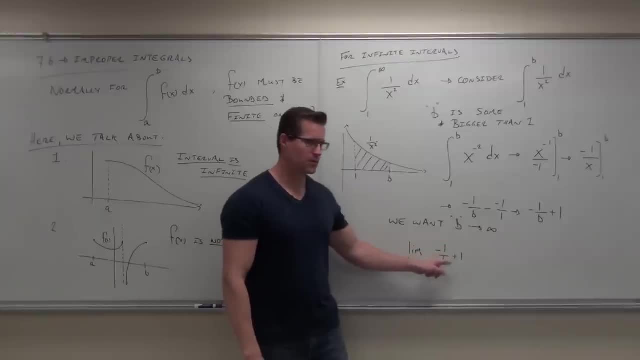 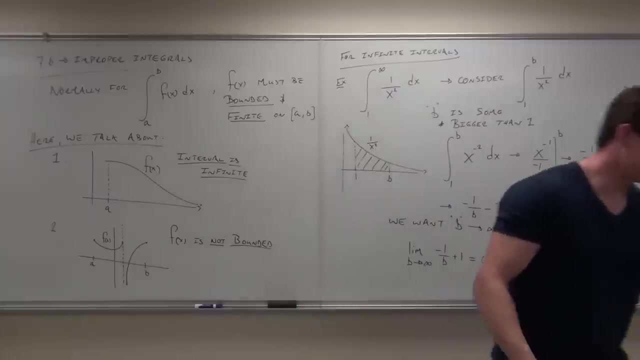 what happens if b goes to infinity here? So can we find the area under the curve from 1 to infinity of this curve, 1 over x squared? That's really cool. How much is it 1.. Yeah, that's the idea. So this idea is we're kind of cheating, we're not really cheating, we're really doing it perfectly mathematically. 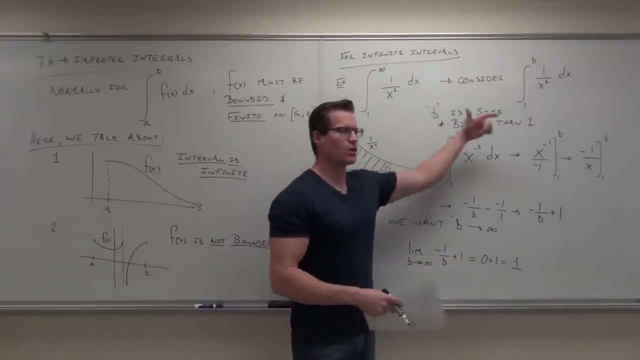 Yeah, that's the idea. So this idea is: we're kind of cheating, we're not really cheating, we're really doing it perfectly mathematically. But the idea is, if you're going to infinity, just call it b. 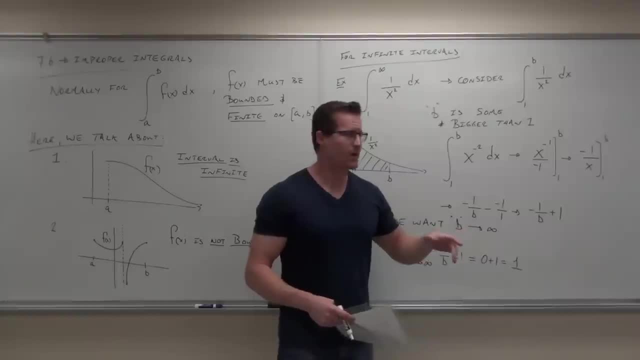 Take a limit as b approaches infinity of whatever the integral is. That way you can actually evaluate. You can't plug in infinity really. You can plug in b. then take a limit as b approaches infinity and that's where we change the problem a little bit. 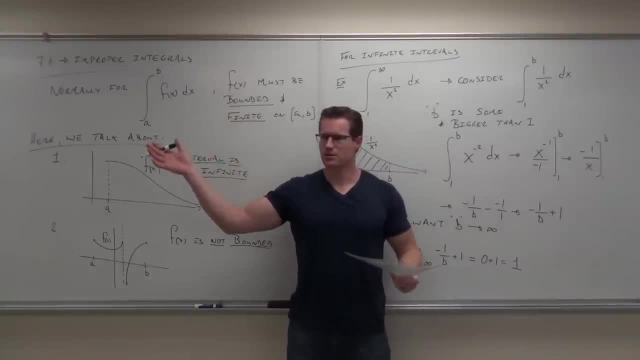 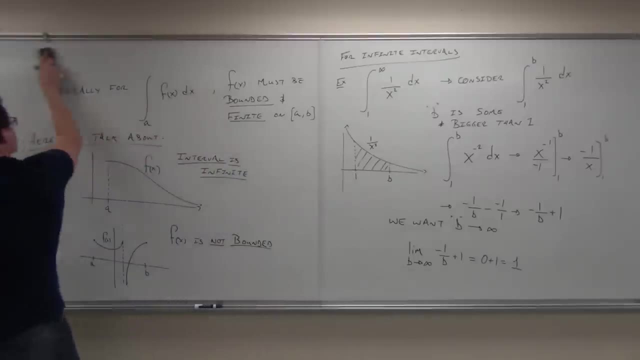 Show of hands. if that one made sense to you, Is it a really difficult concept? Kind of interesting, right? Kind of cool. So let me write some notes out for you on what we're going to be doing. every time Questions- I always forget. 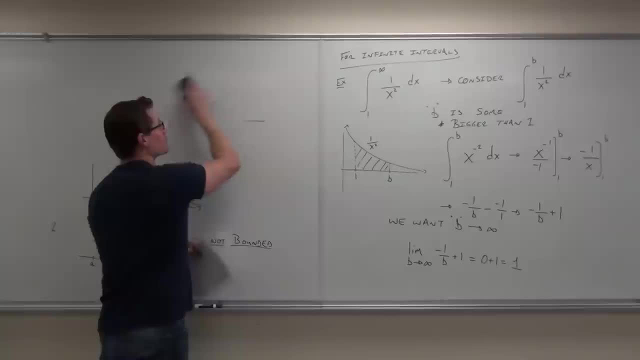 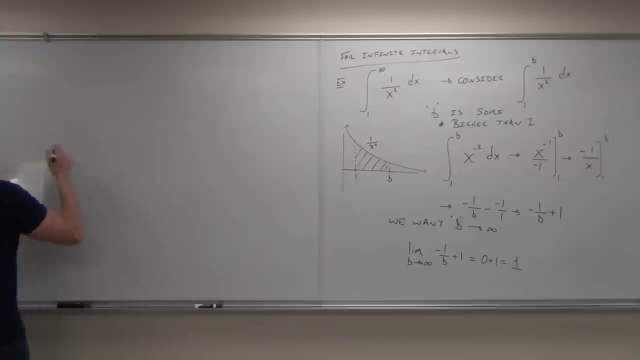 Do you have any questions on this? Okay, good, Did I explain it well enough for you all to understand it? Yes, Okay, We'll deal with the unbounded version, probably another time. So here's what we know. some notes. 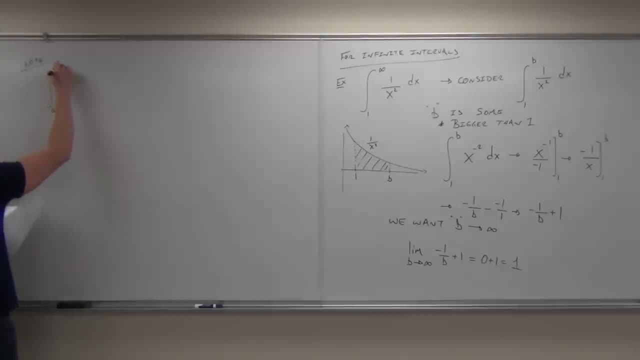 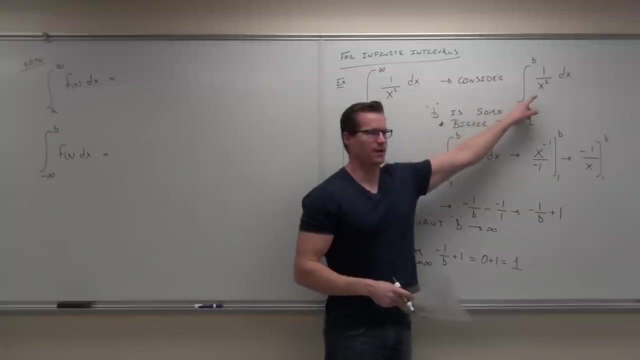 Let's say we had an integral from a to infinity, or we have an integral from negative infinity to b, Out of some function. What we do- we don't really do this every time- okay, Because this, what I've done, this is technically very inaccurate. 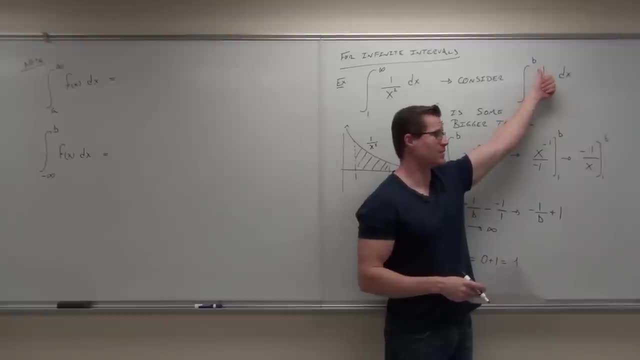 Because what I'm calling this is b, but I haven't said anything. that b is going to infinity. Does that make sense to you? So what we do right off the bat with our improper integrals, after we identify what's going on, 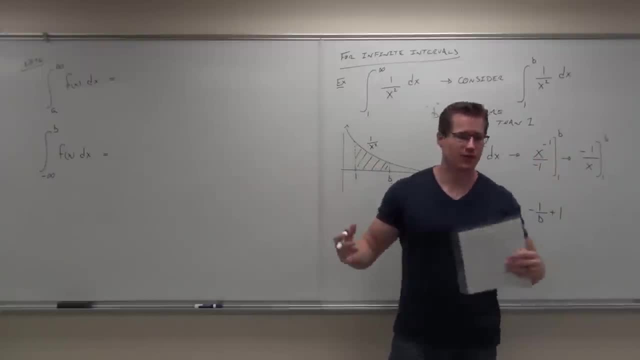 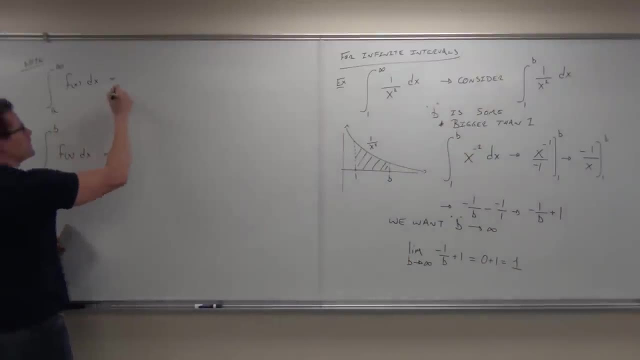 whether it's discontinuity or whether the interval is infinite. we do that first, Then we go ahead and we write out the limit right now. You see, if we're going from a to infinity, then what I'm going to do right now is I'm going to say: 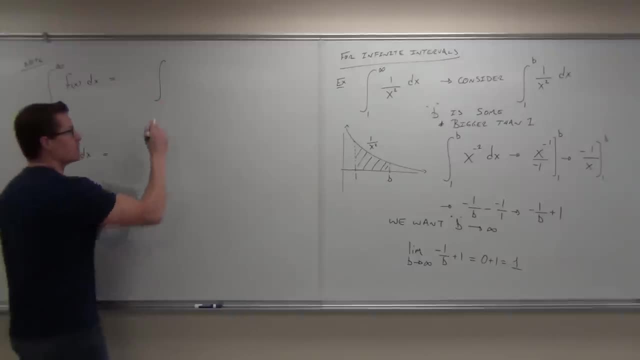 which is the problem, by the way? Is it the a or the infinity? The infinity. So I'm going to say a to b, But in order to do that right away, what you should do is say, yeah, you know what? 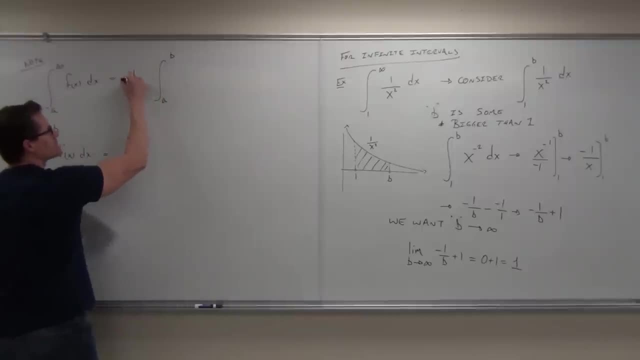 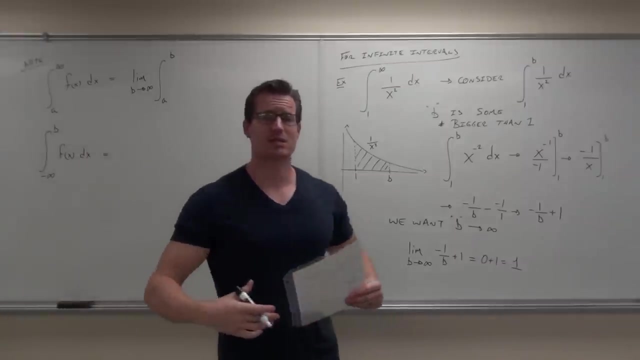 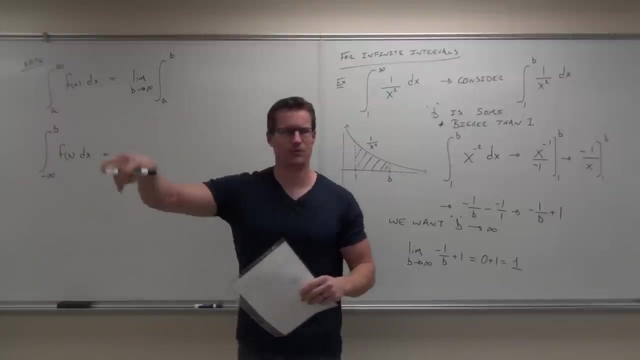 I'm going to take the integral from a to b, but I need to let b go to Infinity If it seems trivial to you. it's not. You're defining what's happening to the b. You have to do that. It's not that I just get to randomly plug in a b, figure it out and then plug in infinity. 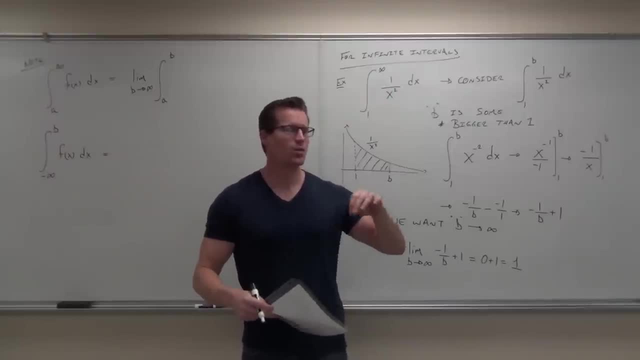 You can't do that mathematically, You do that with a limit. So we say no, we don't get to plug in infinity. Really, what we're thinking about is this: b it's approaching infinity, It's getting really close to it. 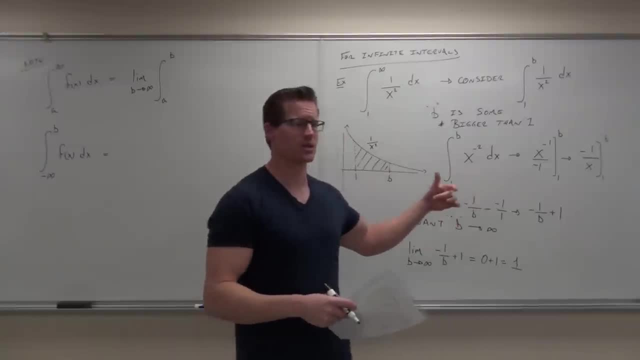 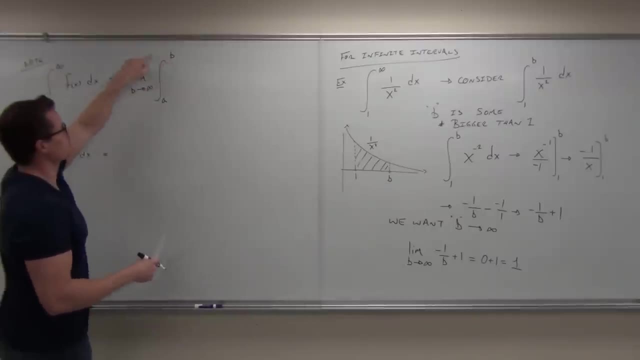 It's plugging in bigger and bigger and bigger numbers until it makes no difference anymore as compared to infinity. Does that make sense to you? So it's not a trivial idea. It's sure. call it a, b, but then define what's happening to b. 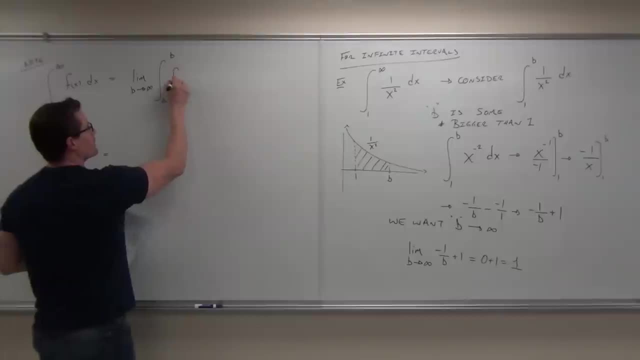 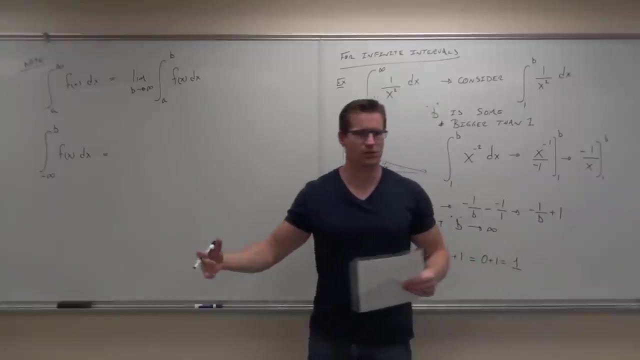 b is going to a positive infinity. You do that with a limit. Now the integral itself- this is where you guys are going to break. The integral itself is doable. I mean, it's everything that we've done so far. 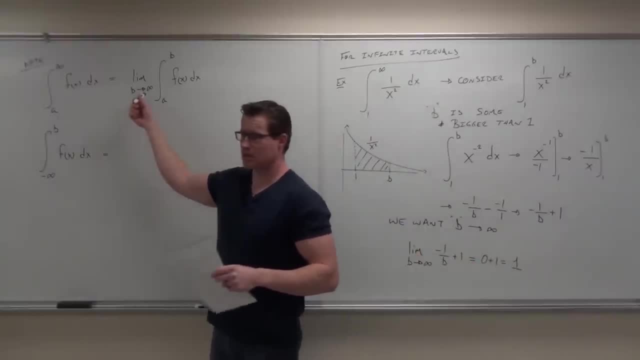 So, basically, the only thing I'm teaching you today is this: That's it That you can do this, That instead of an infinity you put a limit. as b approaches infinity of b, This is still infinity when you think about it. 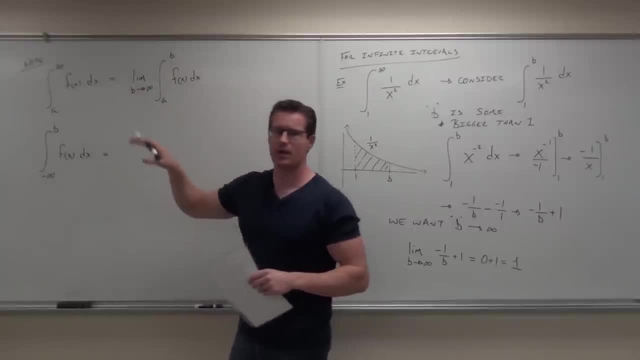 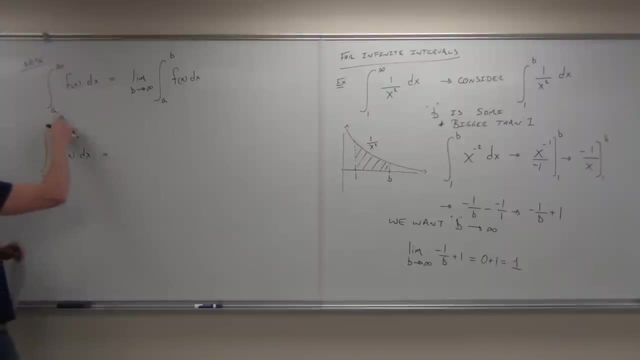 We're just going to make it a little bit more doable so we can actually evaluate this, The integral. That was a lot of words. Did you understand them all? All right, Yeah, Next up, Let's say that we're not going from a to infinity. 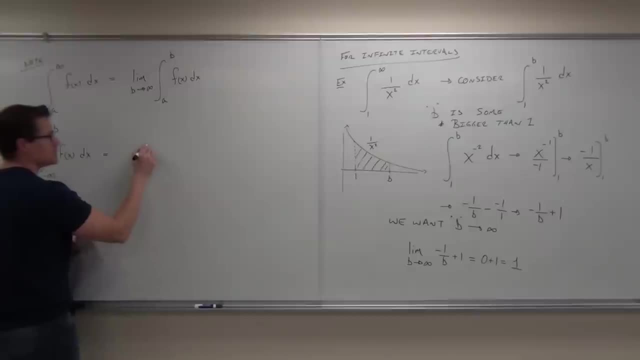 We're going from negative infinity to some b. What's our problem here? Negative infinity, Okay. So the b is not a problem. We call negative infinity our a And then we say, okay, cool, I'm going from a to b, but what's happening to the a? 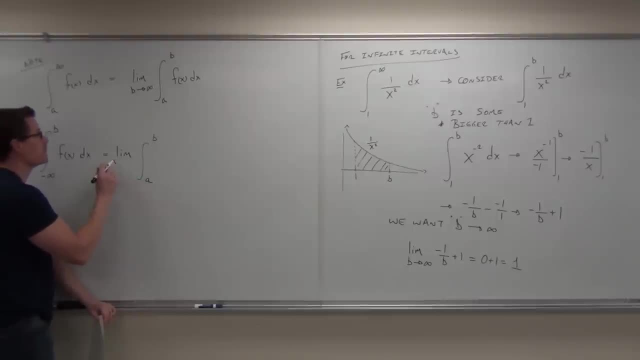 Where's the a going to go? So a Approach is negative infinity. That's right. It should match up. So a negative infinity, a negative infinity, And then the integral. no problem, You'll know how to do this. 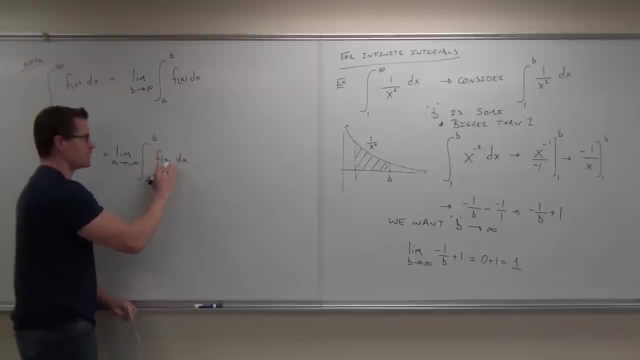 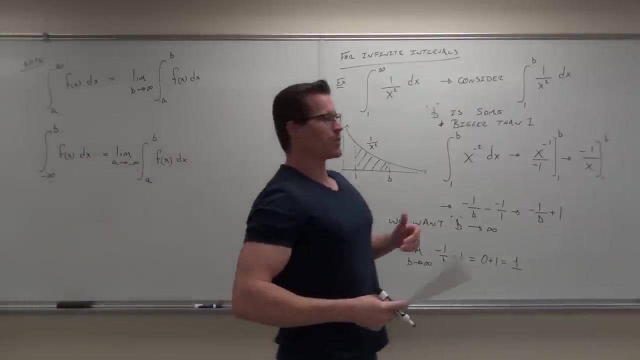 I'm not saying it's going to be easy, but you'll know how to do it, because it's something that we've covered before You guys. okay, so far. Now we're going to come up with two different words here, Two words that I'm sure you've heard them somewhere in your life before. but for integrals. 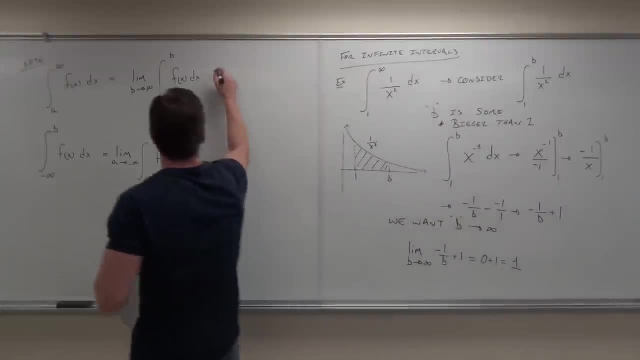 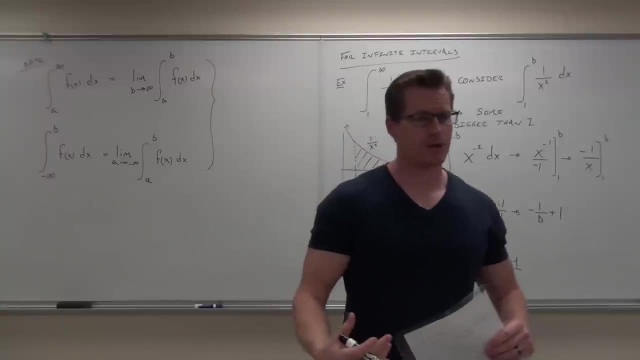 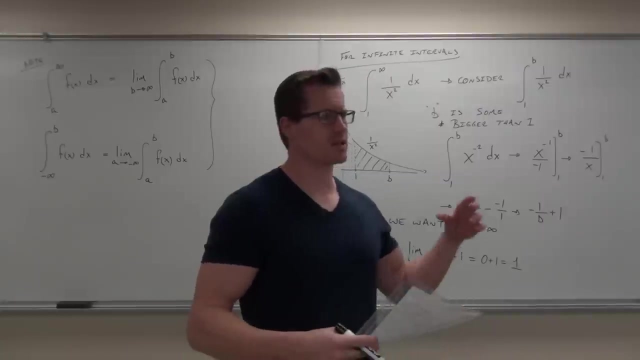 we're going to define them right now. Okay, These limits are either going to be what's called convergent or divergent. Now, if the limit exists, what that means is that you can add up all the little sums and it equals a finite sum. 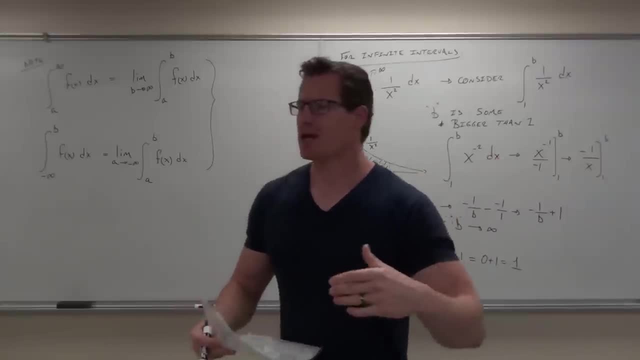 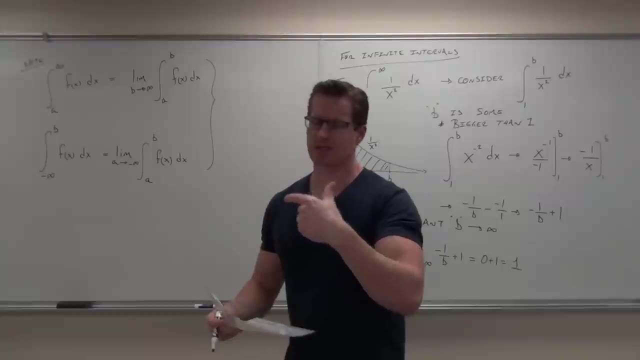 That would be a convergent integral. That means that the area actually exists. If the integral adds up and it keeps getting bigger and bigger and bigger and bigger, well then that integral is not going to exist, That limit won't exist. Actually, the integral probably will exist, but the limit won't exist. 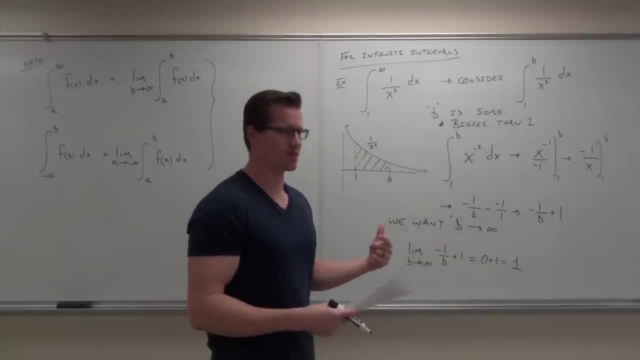 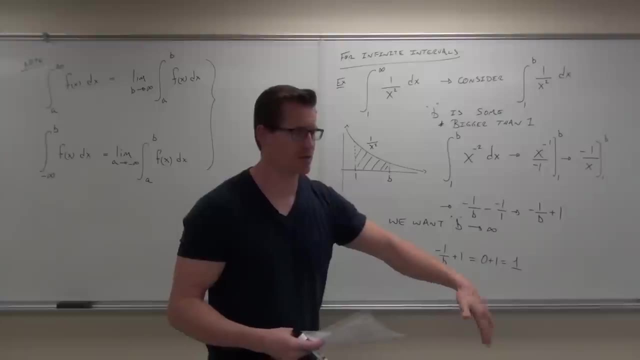 If that limit doesn't exist, well that's divergent. Either it doesn't go to a finite number, it goes back and forth, or it goes always up or always down. It doesn't go to one single number. If that limit doesn't happen, then we call that divergent. 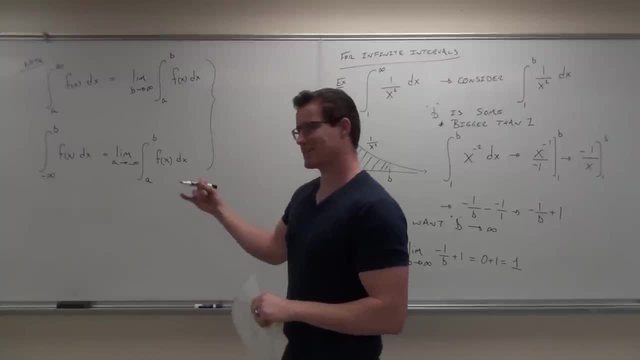 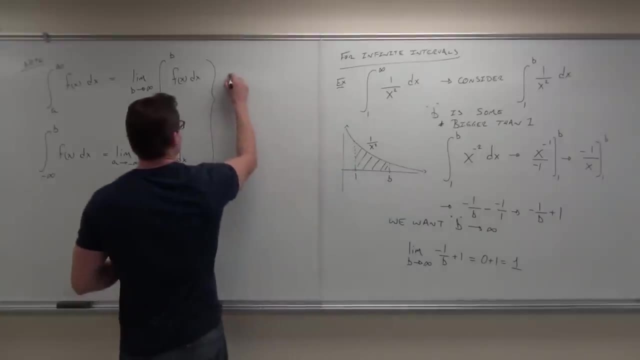 So these things are convergent if the limit exists, divergent if the limit does not exist. Does that make sense to you? Yes, Mel, Yes, So we call these convergent. Yes, If limit exists, we'd say it's divergent if the limit does not exist. 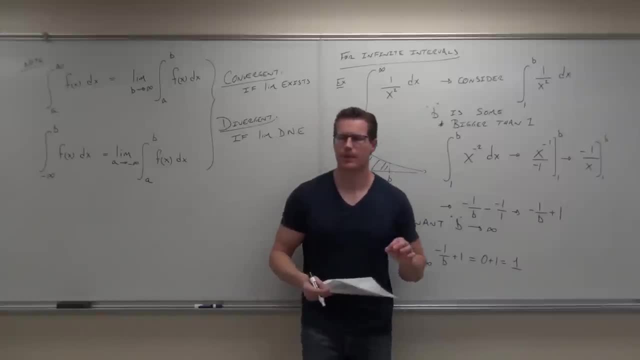 Convergent basically means this. Convergent basically means this: It means that the area that you're adding keeps getting smaller and smaller and smaller and smaller as you're approaching infinity or negative infinity. Smaller and smaller and smaller, to the point where, when you add it, it's so small that 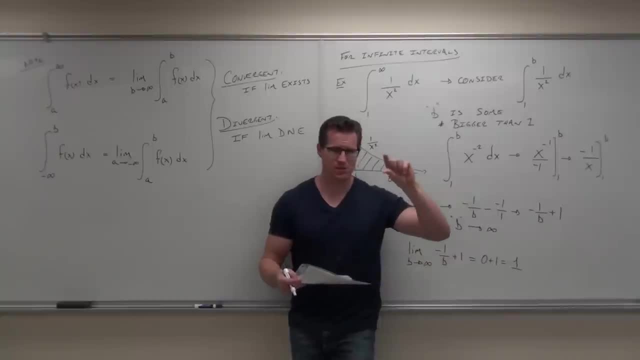 it doesn't make a difference. Does that make sense to you? So it keeps getting smaller and smaller and smaller and smaller Divergent? does this Divergent says it keeps getting bigger and bigger and bigger as you keep adding it, or 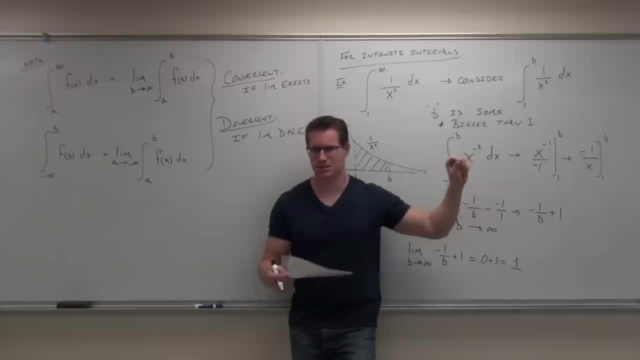 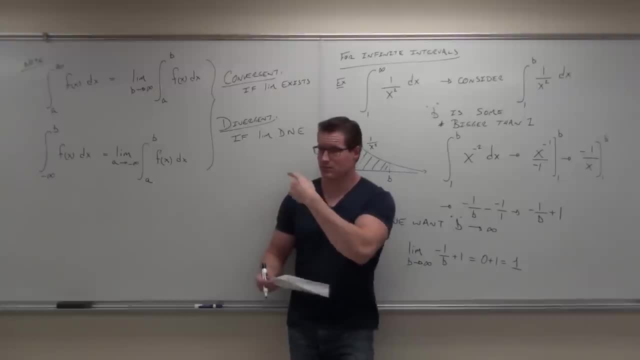 So don't worry too much about it. Basically the idea is: if the limit exists, it's going to be convergent because that idea is happening. It's getting smaller and smaller and smaller. quick enough If it's divergent. if the limit doesn't exist, that means it's not happening. 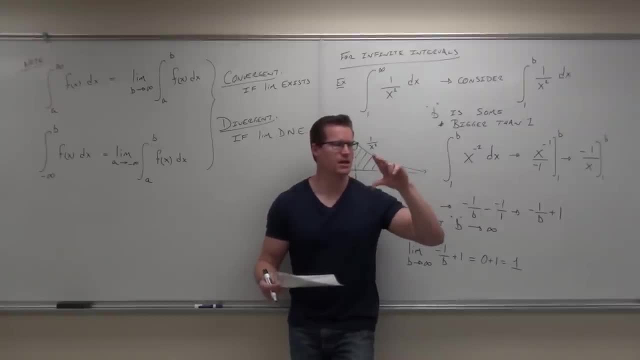 So we're getting bigger areas or we're getting areas that don't go back to one single number. It keeps getting bigger and smaller, bigger and smaller. Does that make sense to you? Okay, Would you like to do some examples? Of course you would. 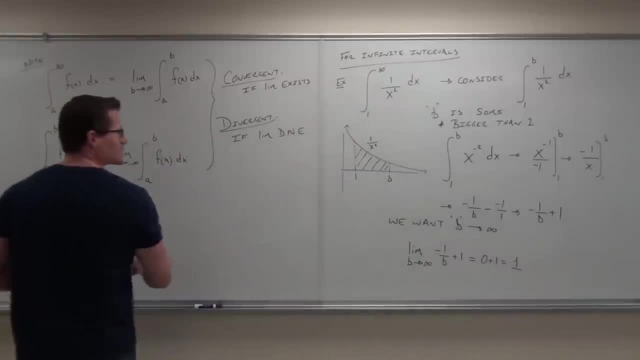 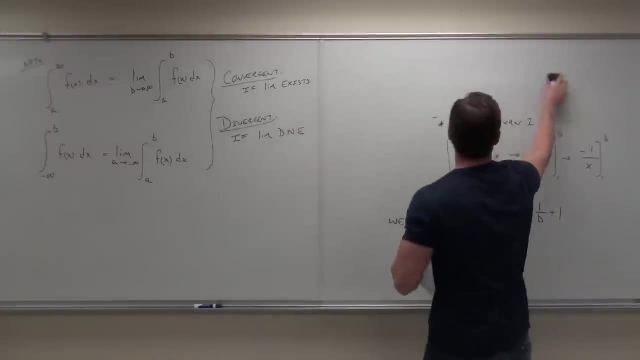 So let's do some. Thankfully, these examples won't take 30 minutes. They're fairly quick Question. Question: Just kidding, Was it on this? No, Just kidding, Oh, you were joking, Funny guy Haha. 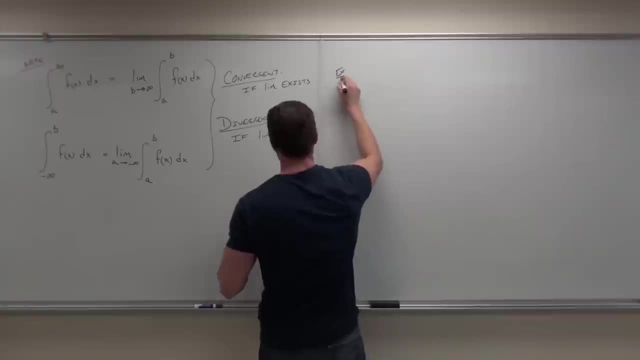 Is there going to be like in case two, where we're taking two limits, Like from negative infinity to infinity Absolutely? Yeah, I'm going to show you how to do every case I can think of. Okay, So this is why this lesson is going to be about three days long. is that I'm going to? 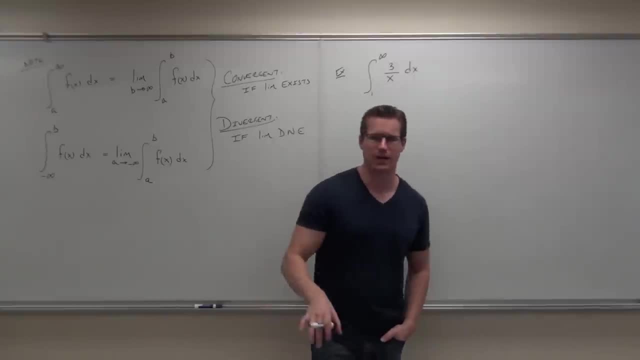 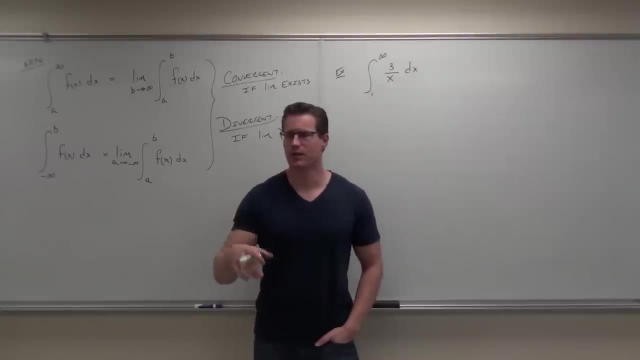 show you everything that I can think of as far as what cases go. Okay, We're starting very easy right now, But we will have limits that go from negative to infinity. We'll have limits that go from negative infinity to infinity, where they cross over an infinite. 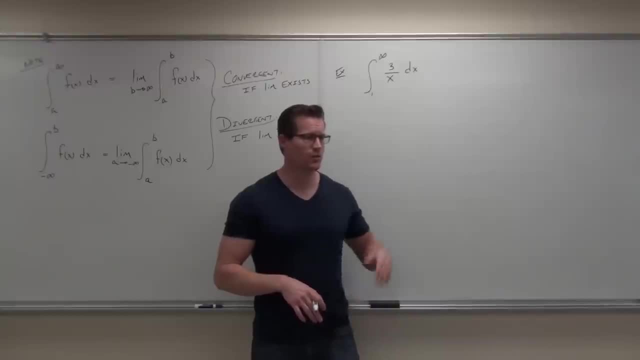 discontinuity. That's about the worst case scenario you can get, Okay. So if you go from negative infinity to infinity and you cross over, if you cross over more than one, that sucks even worse. But if you cross over an infinite discontinuity, then you have to break up that limit, sorry. 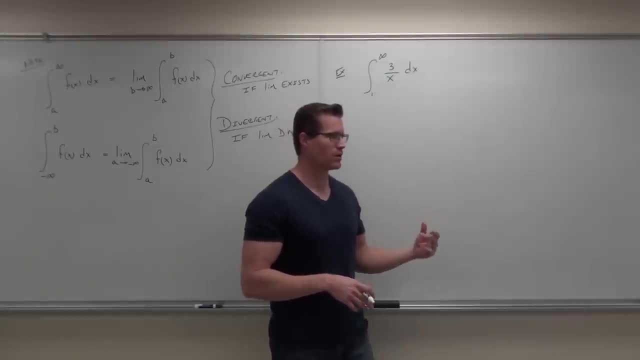 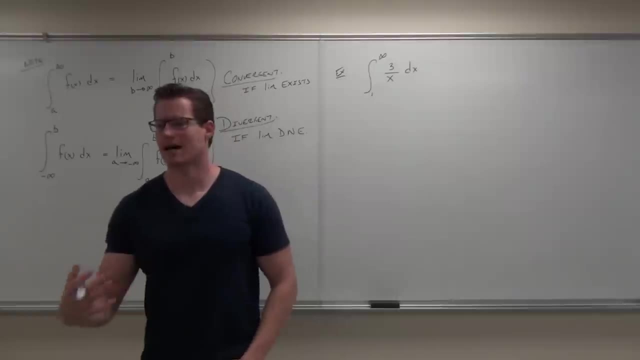 that integral in at least two of them, sometimes more Okey-dokey, Okay. So let's start off very basic. Firstly, we want to identify what type of an improper integral, if anything we have. Do we have an improper integral here? 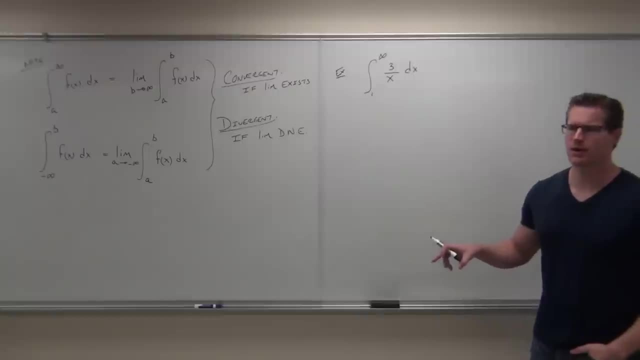 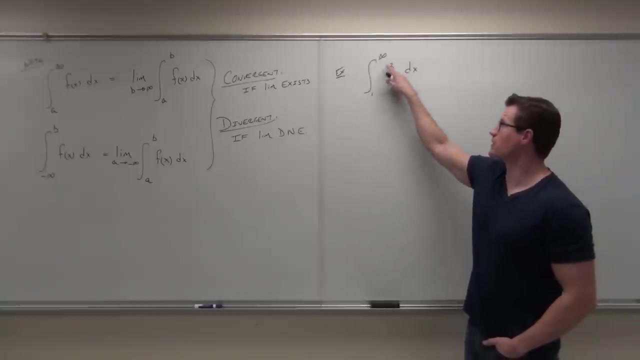 Absolutely Well. firstly, let's see if there's an infinite discontinuity. Are we defined for an entire domain? No, Are we defined for an entire domain? Yes, I don't care about the zero. If I'm not crossing zero, I don't care. 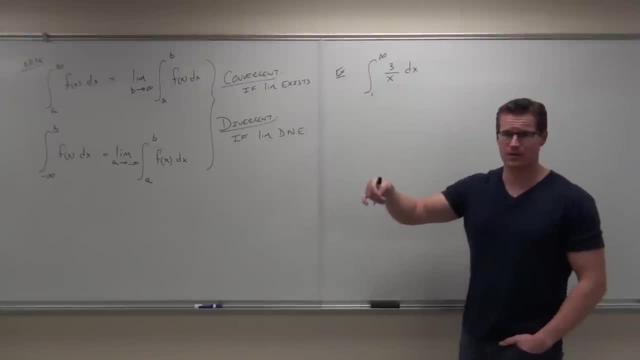 I care just where I'm going to. So, on my interval, am I defined? Yes, Then we're good. There's no infinite discontinuity. I get what I'm talking about. How about the interval? Is the interval finite or infinite? 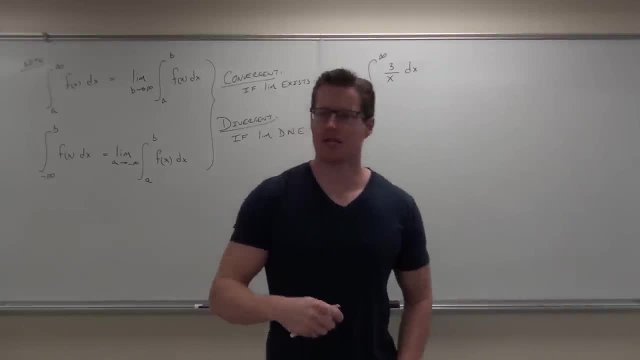 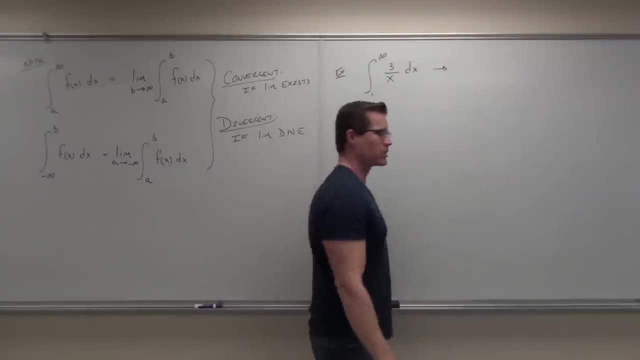 Infinite, So what that's called is an infinite interval. It's one of these improper forms. So if we have an improper form and an infinite interval, let's write out exactly what we're going to do with it. So tell me, how should I rewrite this problem so that I can do it? 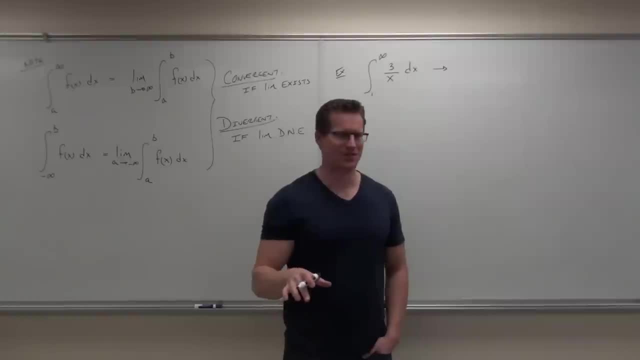 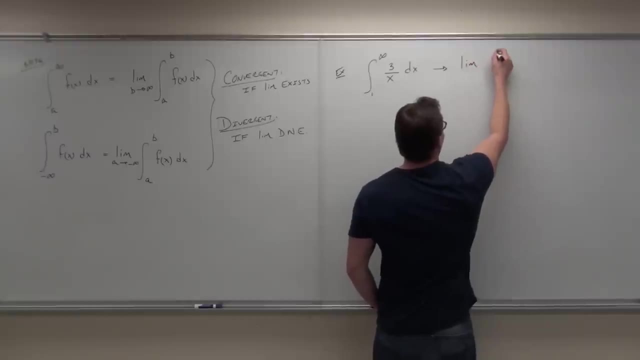 Limit. Okay, So do you need the limit? Yes, I'm not going to check for that or anything on your test, am I? Yes, Of course you do. Of course I am. Limit, Hello, A limit from where to where. 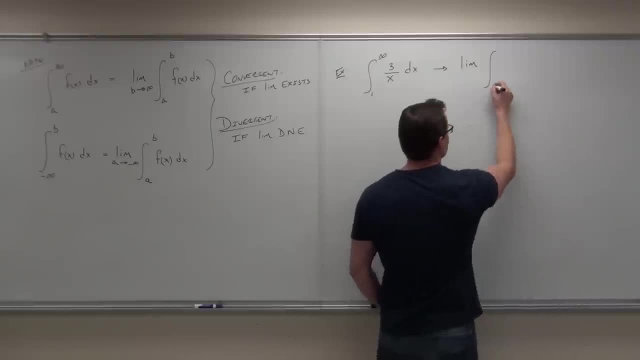 B to A. Oh, say that correctly. From where to where? One to A. One to A. One to B, B- Alright. And then B goes to where A. Perfect, Do we change this? No, You can pull the three out. 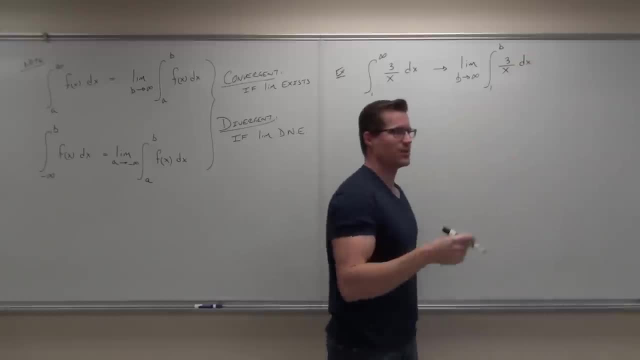 Yeah, you can pull the three out, Absolutely, In fact, because it's a limit, because that's a constant, you can actually pull the three way out here. It doesn't even matter, You can pull it here, pull it here. 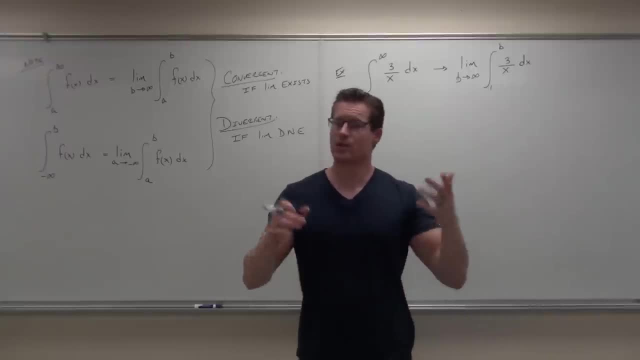 I don't care Wherever you want to go. Does that make sense? Yes, You can pull the three out for sure. Can you do this integral? Yes, They're all going to be doable. Yeah, of course For you. 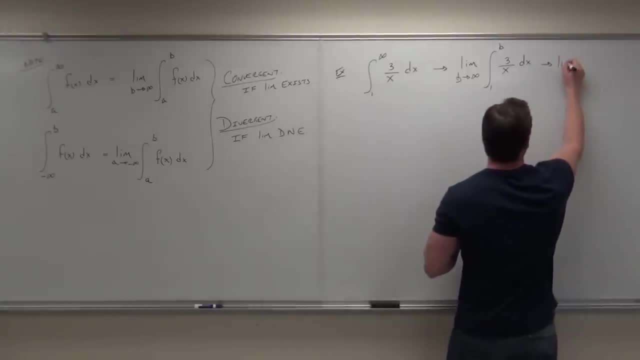 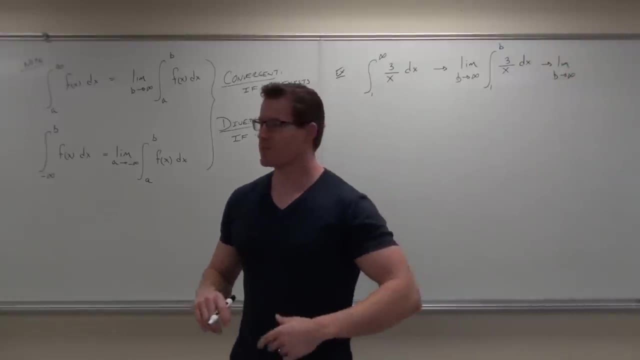 So we have a limit, We have B approaches infinity. I've got to warn you in this section, because we've covered all of our integration techniques. I'm going to be doing a lot of them pretty quickly because I'm going to assume that you 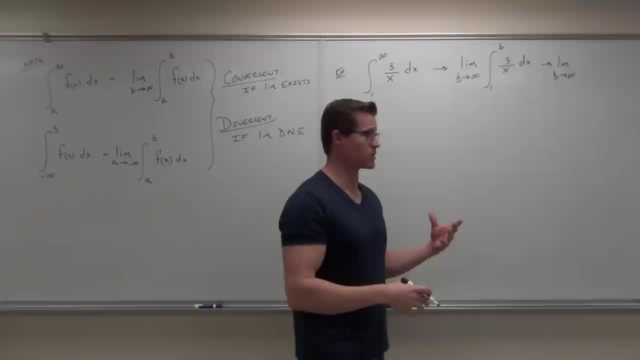 have studied the previous four sections that we've done on integration techniques, okay. So I'm going to cut some steps out just for the sake of time, because we're going to get some integrals that are kind of nasty, Okay, And I'm not going to repeat all of those techniques that we just learned. 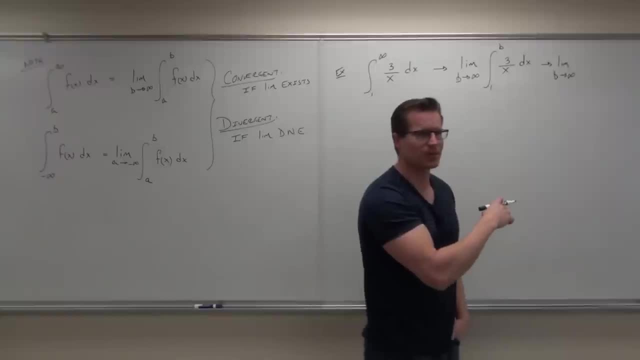 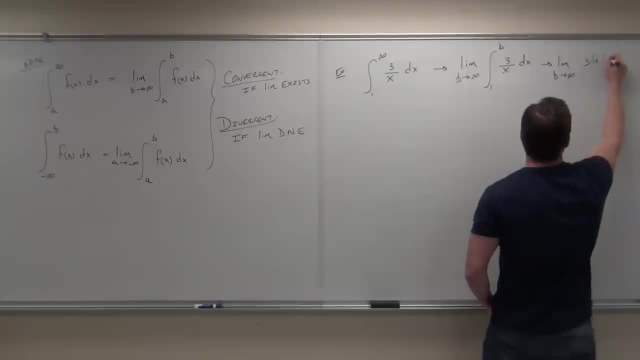 I'm going to use them Here. well, this is a pretty basic one to begin with. So what's our integral going to be here? 3ln, 3ln. Absolute value. Absolute value. x, Oh, absolute value. 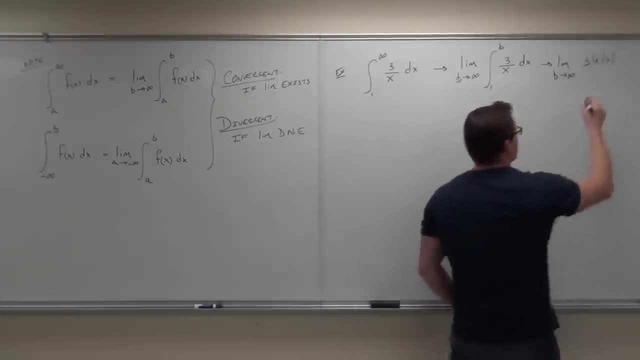 Did you get that From where to where? 1 to b, 1 to b. Now be smart about the absolute value. Look at your interval. Your interval goes from 1 to infinity. Tell me what your interval is: From 1 to infinity. 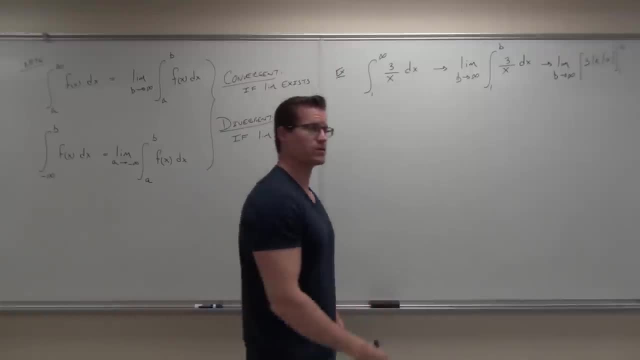 Tell me something about all those numbers. They're all positive. They're all positive. So your absolute value is kind of irrelevant here, but you're going to need to show it. So in our case we've got a limit. 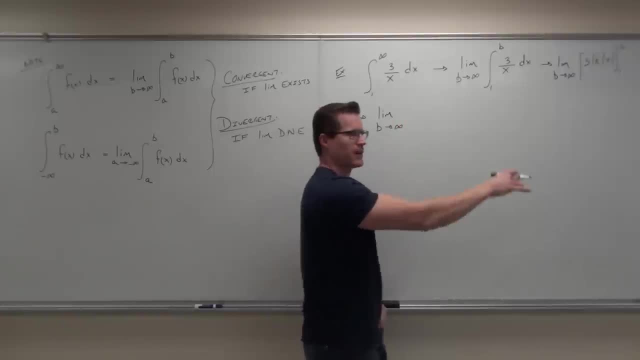 Do you remember something about limits, how we always write them until the very last part where we actually get to evaluate them? Same thing happens here. So we will have 3lnb minus, and you can do this a couple ways. You could pull the 3 out and have a bracket here, or you could have 3lnb minus 3ln1. 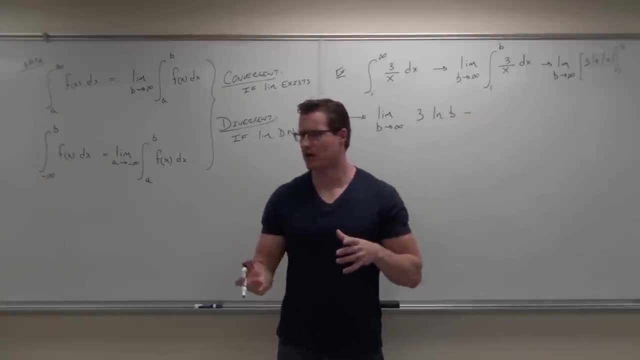 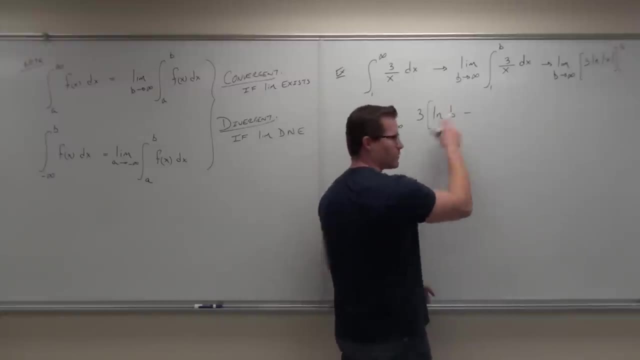 It really doesn't matter, as long as you have the 3 in the appropriate spot, in both places or being factored out. Make sense, It's an algebra. So I'll probably do it like this because I don't want to have to write the 3 again. 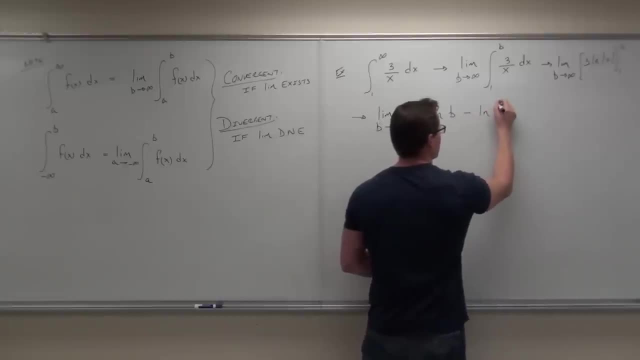 I'll do 3 times lnb minus ln1.. So this is limit. as b approaches infinity, of 3lnb minus how much is ln of 1?? Do you know? Zero, Zero. Okay. so check it out. 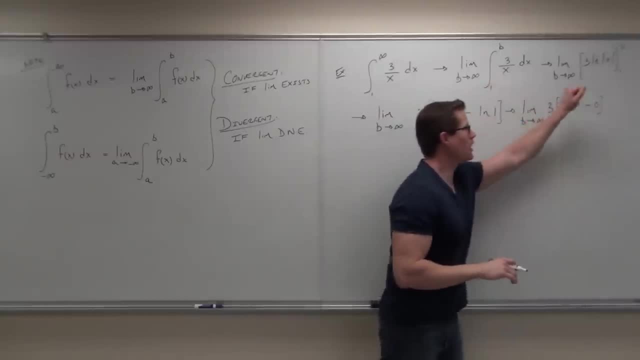 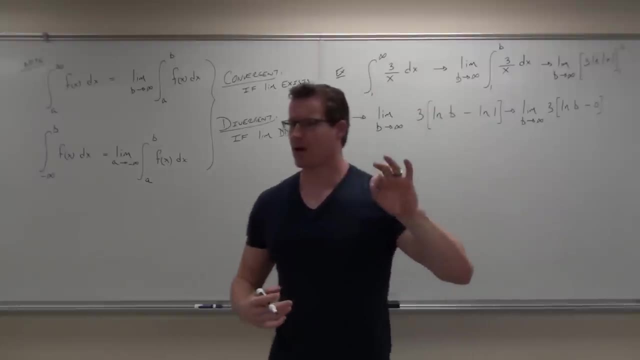 Simple, integral, no problem. We've evaluated it. no big deal. We've simplified it as much as we can to the point where now we're going to attempt to find out what happens as b approaches infinity. Are you guys okay with this one? 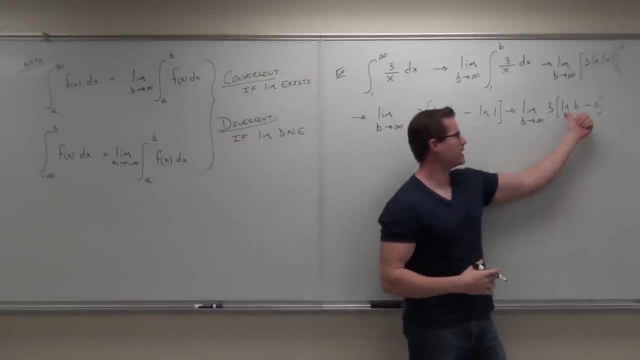 Awesome. So what happens when b goes to infinity? What's ln of b as b approaches infinity? Oh dear, Do you know? Do you know? Yeah, I know, Read it. What's ln of b as b approaches infinity? 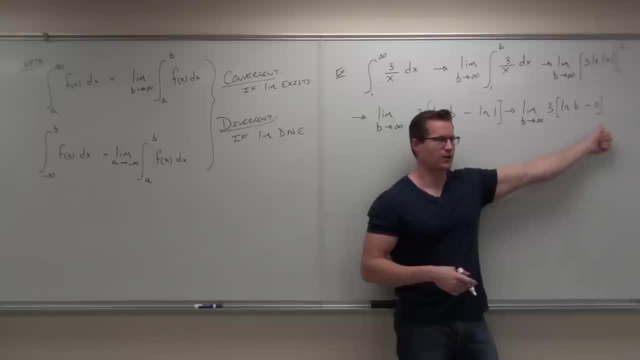 Zero, No, ln of one is zero. How can ln of infinity also be zero? It doesn't make sense. One, It's an increasing function. the entire time It's always increasing. Say what now? Infinity, Infinity, It's infinity. 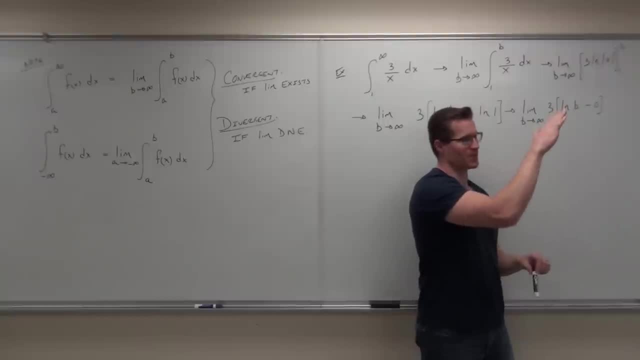 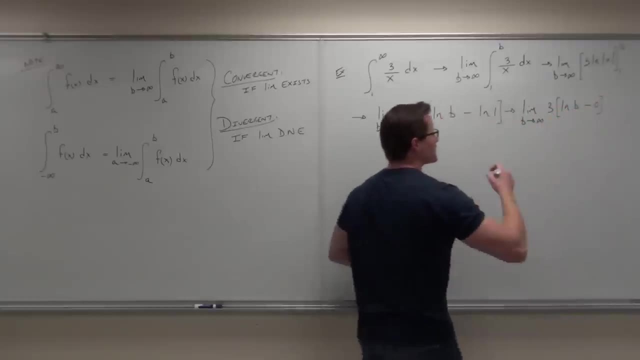 That's right. ln goes like this: Remember ln, Hope you remember. ln Goes to negative infinity as we approach zero. from the right Goes to infinity. as we approach infinity, It's always increasing. What that means is that this is infinity. 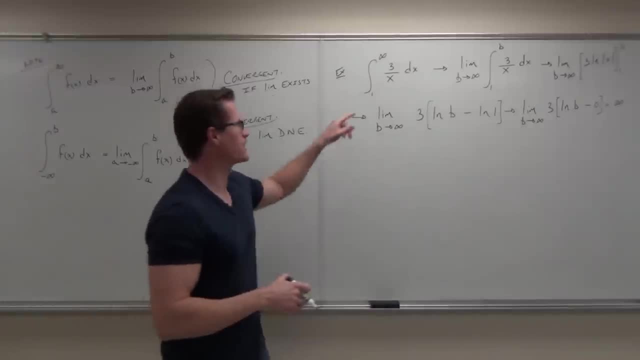 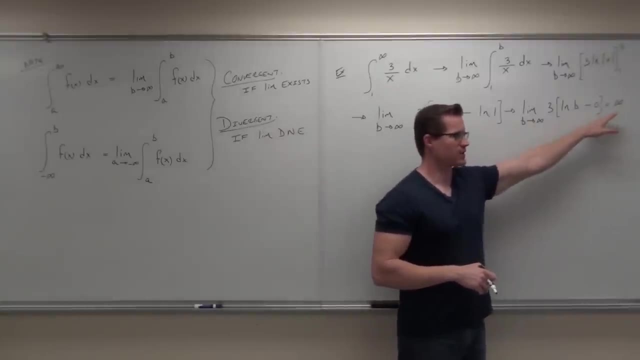 That's infinity. Tell me something about this integral. Is it convergent or is it divergent? Divergent, It's divergent. What that means is that look at this. This limit keeps getting bigger and bigger and bigger, doesn't it? 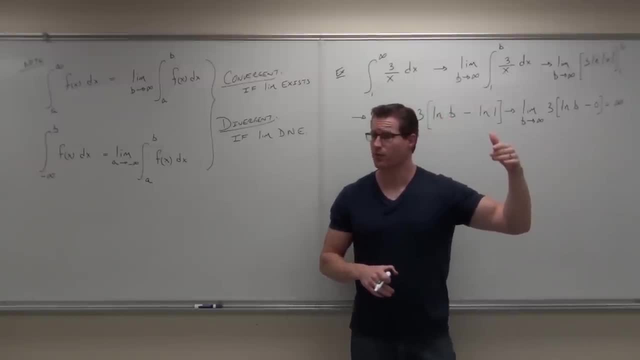 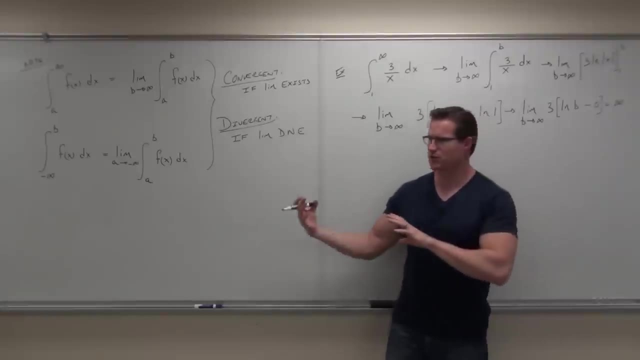 Means the area keeps getting bigger and bigger and bigger. It doesn't go to a finite number. Therefore, our area under this curve, we can't say what it is because it's an infinite area- We call it divergent. You guys see the difference between convergent and divergent. 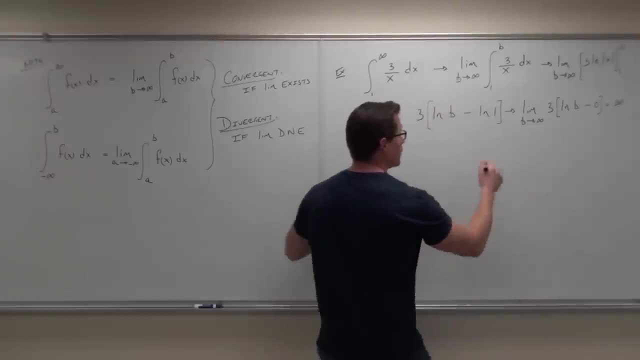 The first one we did. we actually got an area out of it. Second one we did. no, no, This right here says that this is divergent, And I wanted to give one to you right off the bat, That way you see what I'm talking about. 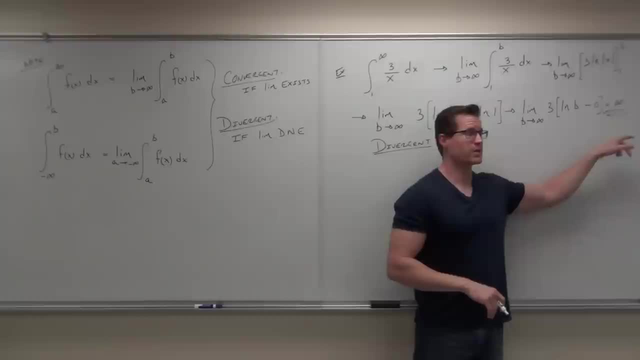 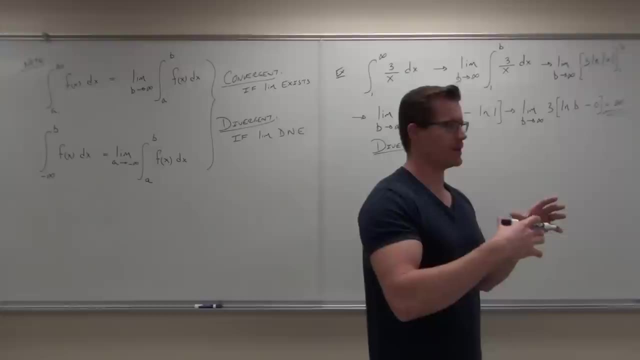 when I say divergent, If the limit doesn't exist or if the limit goes to infinity or negative infinity, then we say that we can't find the area under that curve. It's always getting bigger than some. I can't find it. 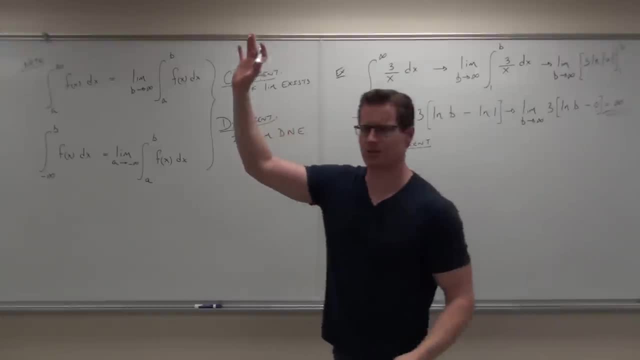 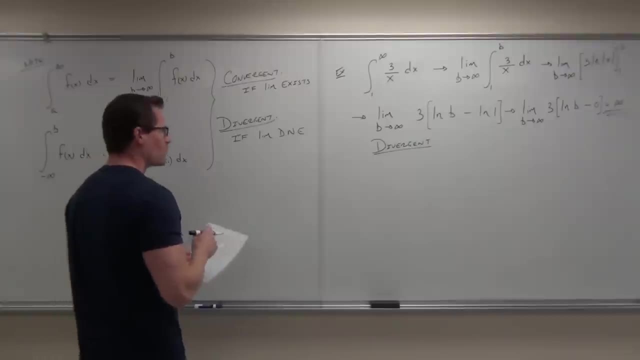 It's a finite number. Show of hands, if that one made sense to you. Okay, can we keep on rolling? Not too bad right? Not yet. at least Let's keep going. What we're gonna do now is we're gonna figure out. 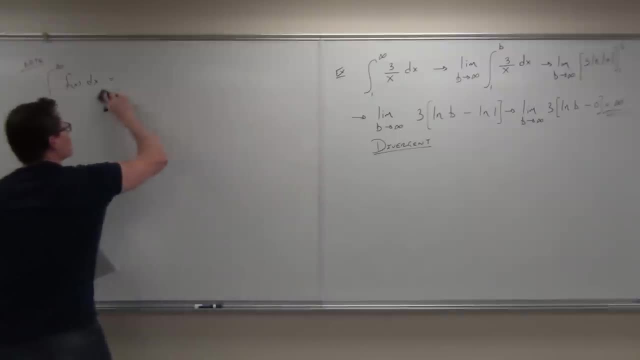 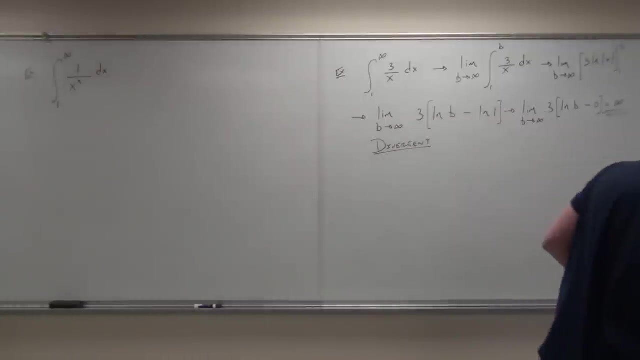 how to do this in general for any power of x. So, instead of doing example after example, let's try this one. Let's go from one to infinity, one over x to the n dx. You know what? I'm guessing that most of you 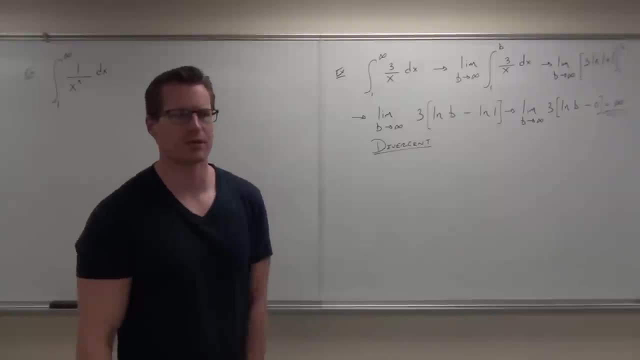 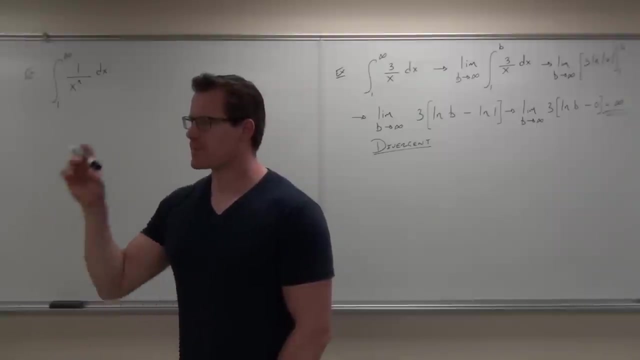 can probably help me out on this one. What's the first thing that I would do with this particular integral Red limit? Red limit, yeah, because tell me what's wrong with it. Do I have a discontinuity or an infinite interval here? 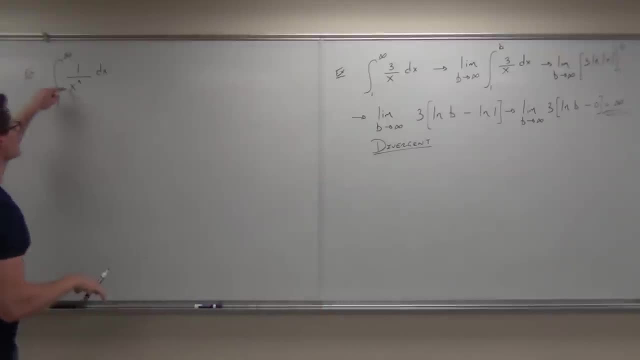 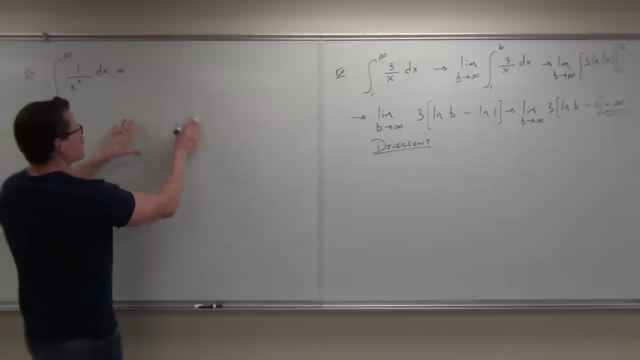 It's an infinite interval. It's an infinite interval. Do you notice how, in this case, the only number that I have wrong with it is zero? still, I missed the zero on my integral, so I'm good. So, yeah, you know what. we just had it on the board. 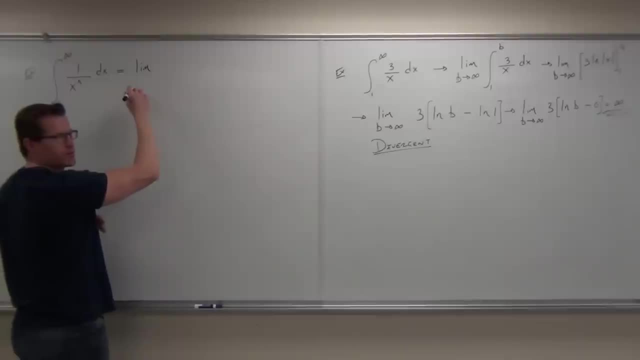 a little while ago. This will be a limit, as what approaches what everybody B, approaches infinity. And then we write from where to where please, One to B, And then One over x. Okay, yeah, okay, we'll do another step. 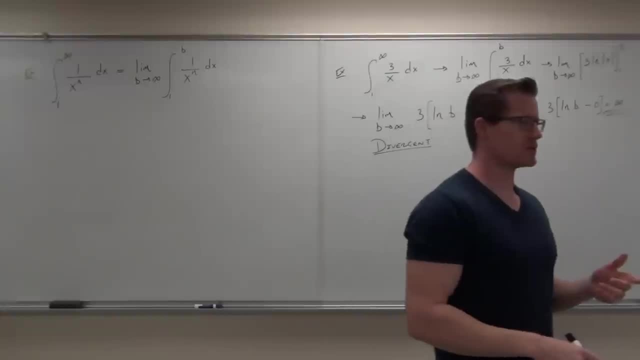 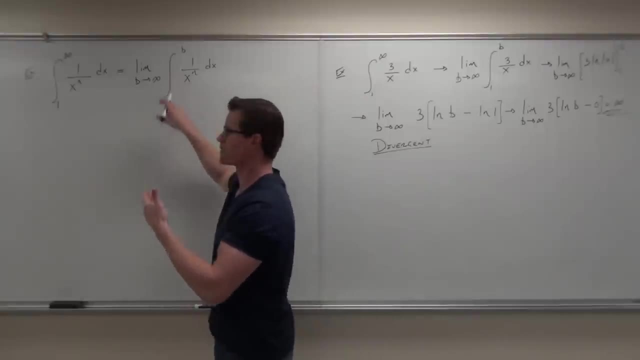 Sure can you guys do that first step. Hello, No big deal, right? You just take care of the infinity, Make sure you have a limit, go into that variable and then take your variable and make it look like it's finite right now. 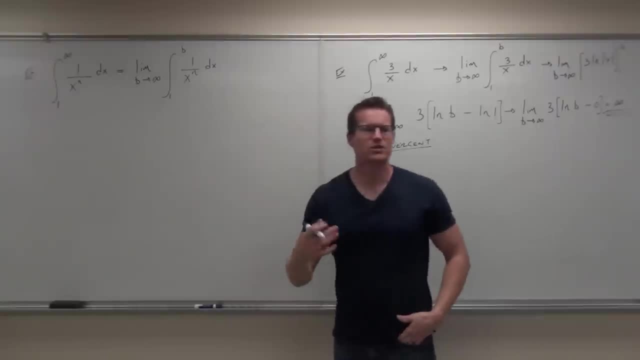 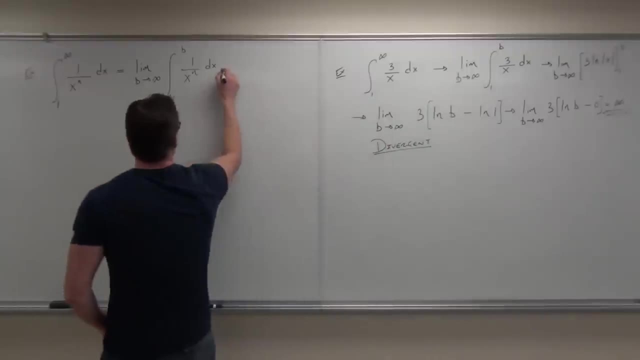 Make it look like it's going to an actual number, just something bigger than one. Now let's go ahead and do this in general. I know that some people don't really like doing things in general, but this is going to save us a lot of headaches later, so check it out. 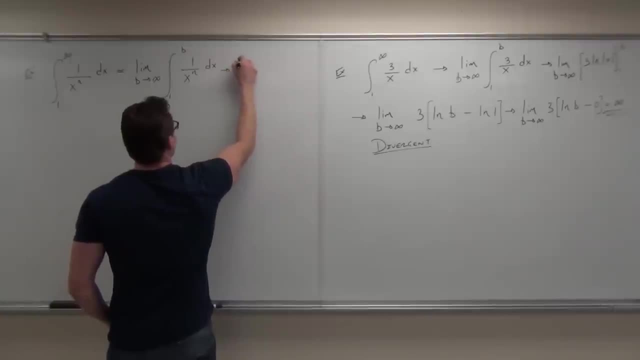 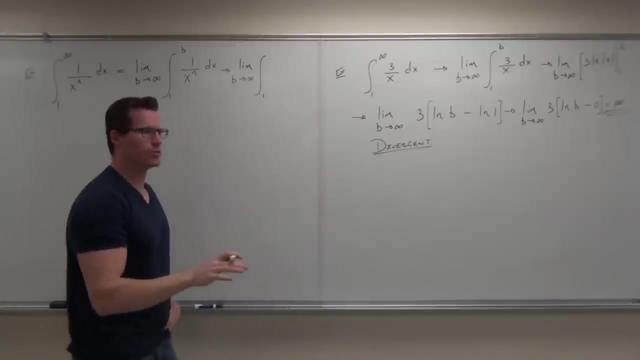 First thing we could do. It's going to get annoying, I know, but you've always got to write the limit. You always have to do that until you've actually evaluated it, so do not neglect that. Are you listening? Yes, 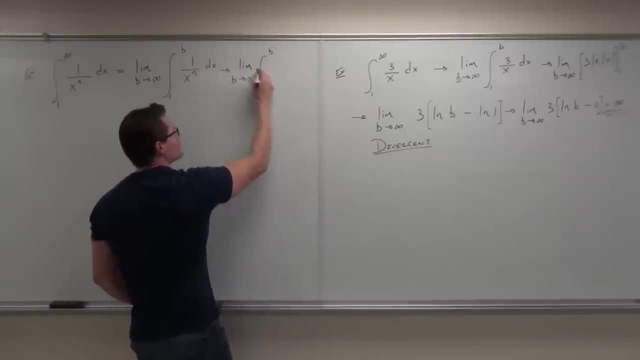 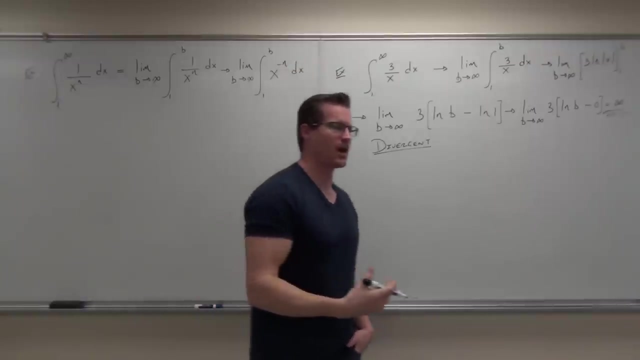 Don't neglect that. Always write it. Now, with one over x to the n, I can write that as x to the negative n dx. You see, if I have x to any power besides one, I can always move that up and I can. 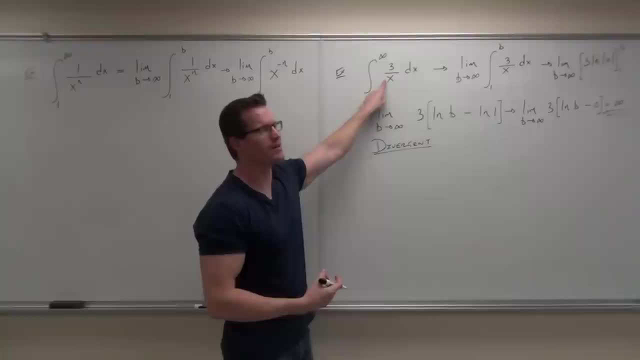 always do this integral. Notice that we already took care of it. If you didn't notice this from before, We already took care of the case. when we have one over x to the first, don't we? We already took care of it. 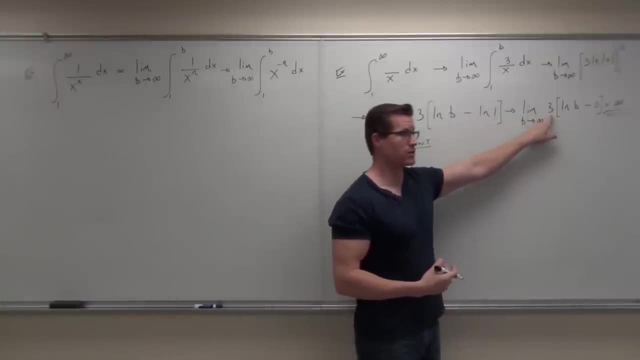 In fact, the three is irrelevant. If the three was a one, you would still have something that's infinite. Do you see what I'm talking about? Hello, yes, no, Yes. So even if this was a one, no problem. 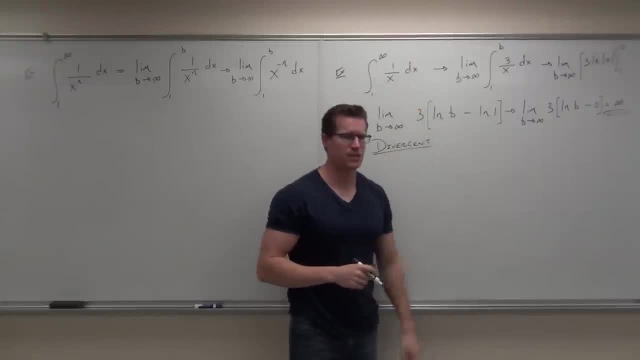 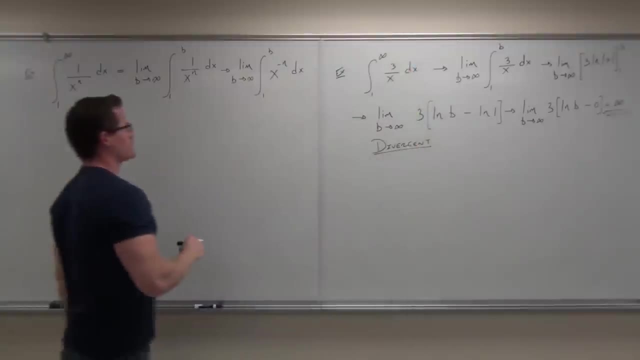 So basically, what's one to infinity of one over x, dx? It's also a divergent, It's also a problem. Okay, so we already kind of dealt with that case here. Let's look at every other case. If we do this, we'll get a limit. 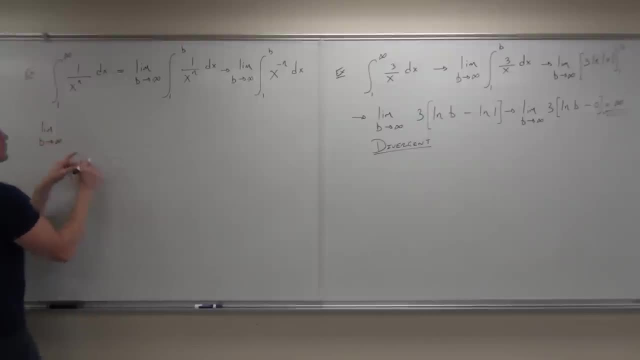 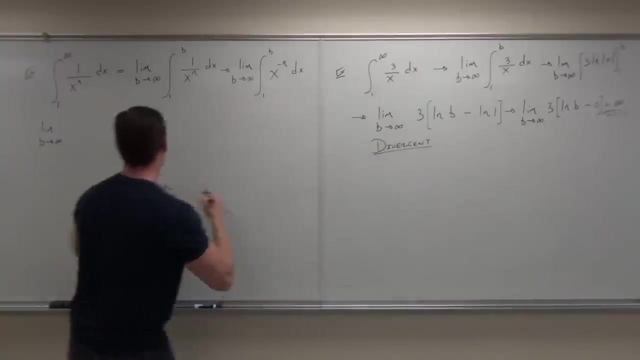 As b approaches infinity. when we do this integral, what do you do with, like x to the third, Or x to the negative? third would be a better. you add one. So this would be x to the negative, n plus one. 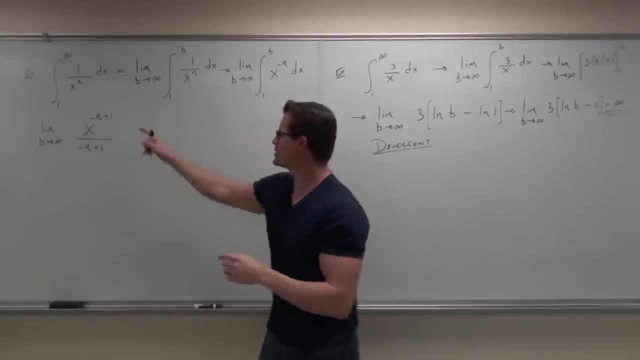 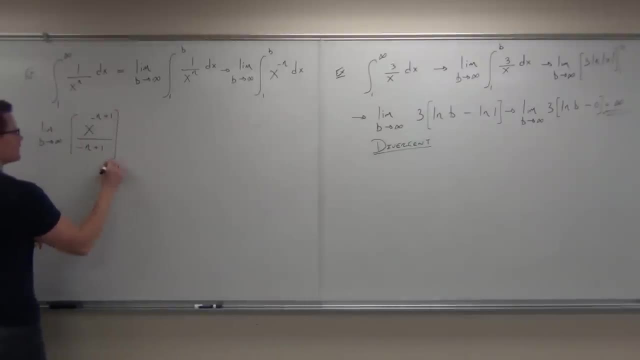 Negative n plus one. Sure, That's exactly what we do. We add one to the remember doing that, We add one to the power divide by the new power. so we do it all the time And then we evaluate it. 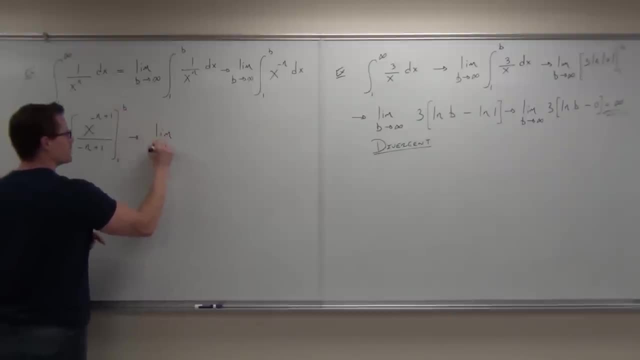 From one to b. Well, if we evaluate it from one to b, we have a limit as b approaches infinity. Tell you what I'm going to change this around, because I like the look of one minus n better than negative n plus one, just me. 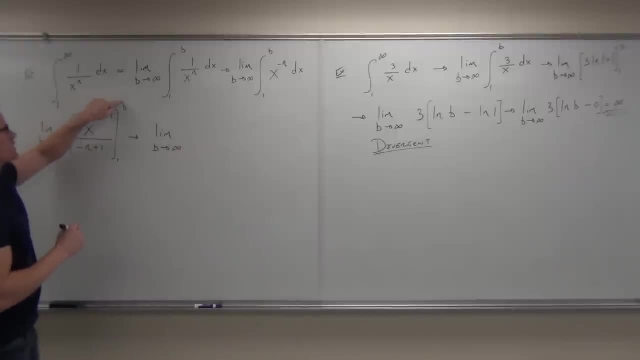 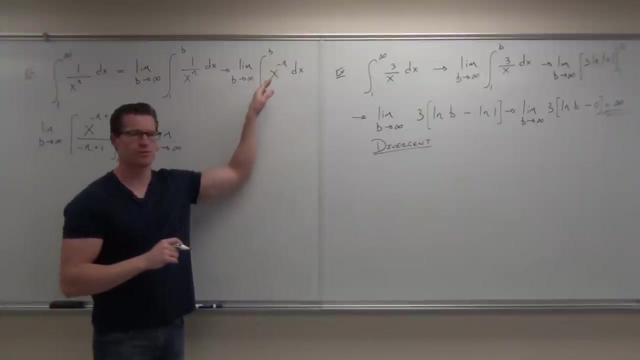 We're going to have remember where the b goes. The b is going to go in terms of not n. n is going to be a constant, okay, And b is going to go in terms of x. So this would be b to the negative n plus one over one, minus x. 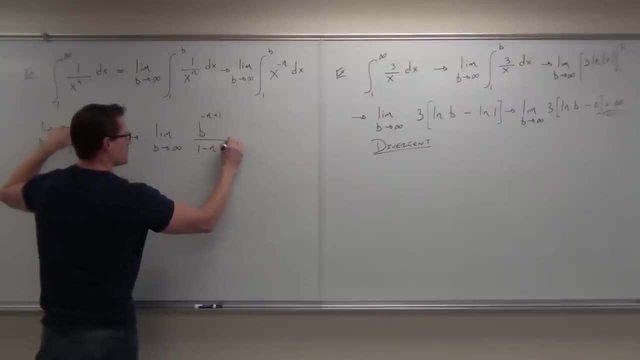 Okay, Yeah, So b to the minus n, minus one to the negative n plus one over one, minus n. Are we okay with that one? I want to make sure that you guys are good with this before we go on any further, Are you? 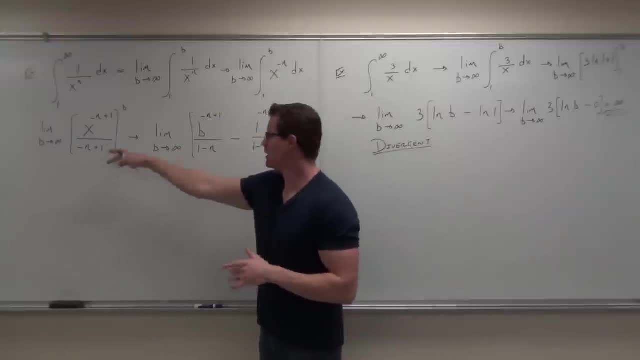 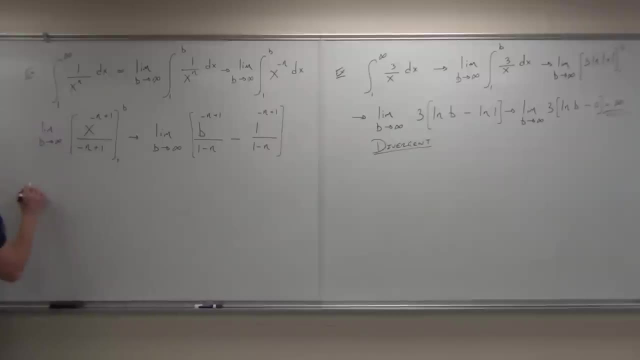 You sure? So hey, add one divide by the new exponent. no big deal. Plug in the b- We got it here. Plug in the one- We got it here. It's got a common denominator. We're going to simplify this just a little bit. 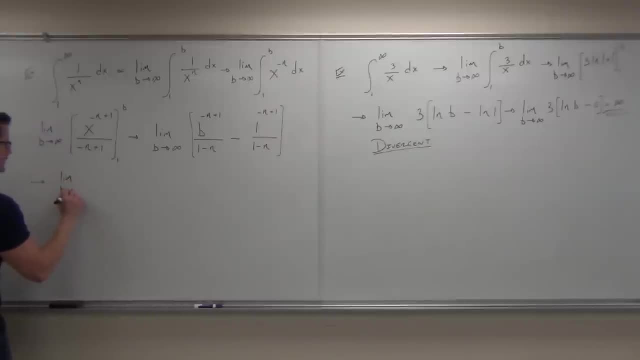 So if we simplify, we've got a limit as b approaches infinity. Well, in here we have b to the negative, n plus one minus one. Notice that one too many, power is still one Over one minus n. You know what we can do also. 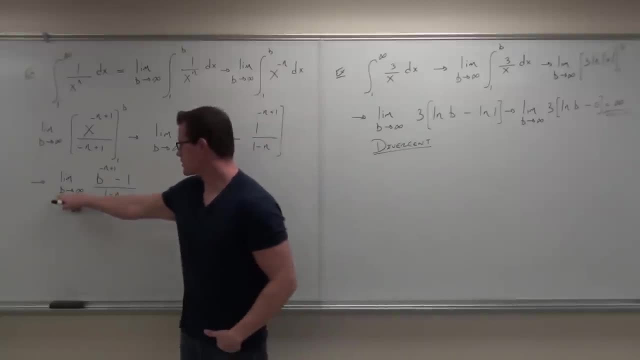 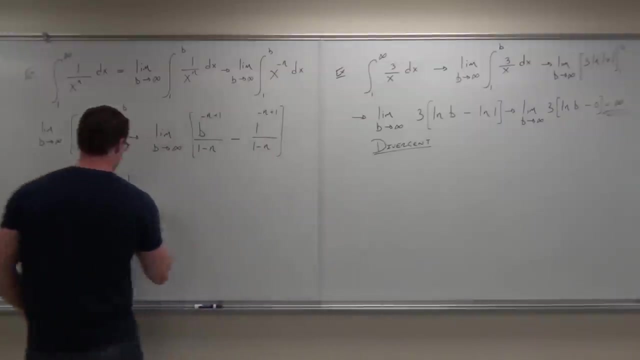 Any time you don't have the specific variable that this is approaching. oh sorry, the specific variable is right here. like b, you can pull out everything in front of your limit, So I'm going to pull out the one over one minus n. 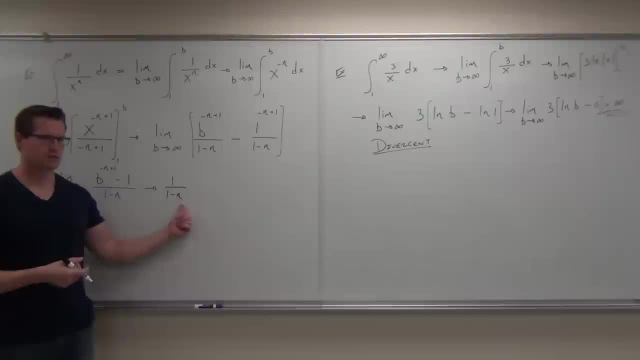 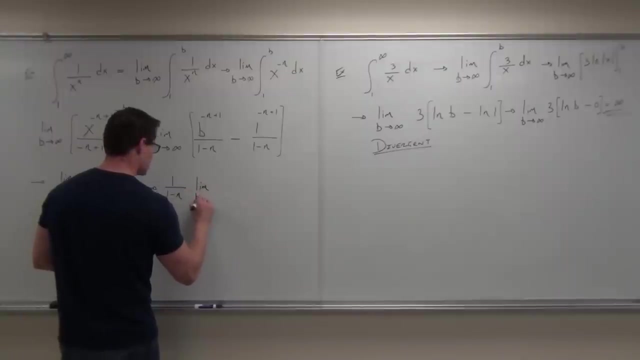 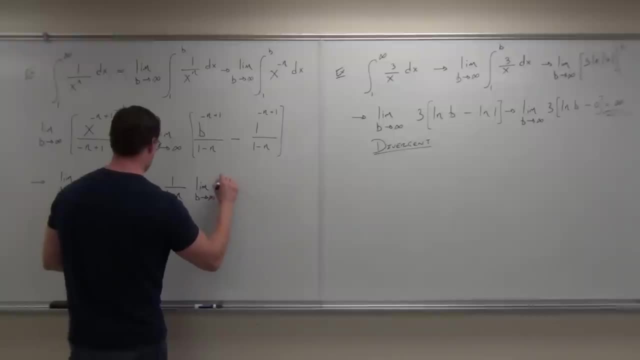 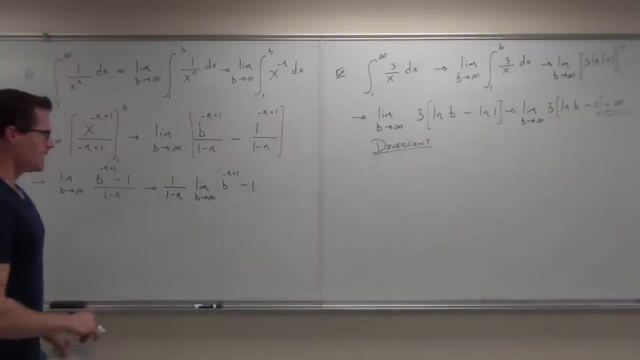 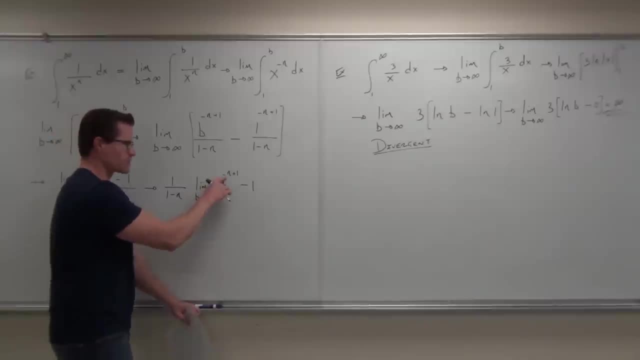 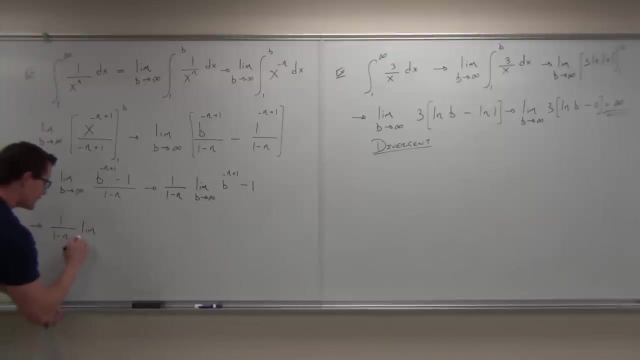 to see what happens next. Are you ready for it? I'm going to force this to factor out a negative. so what I'll end up getting is- and I'll move down here too- 1 over 1 minus n times the limit b to the negative infinity. 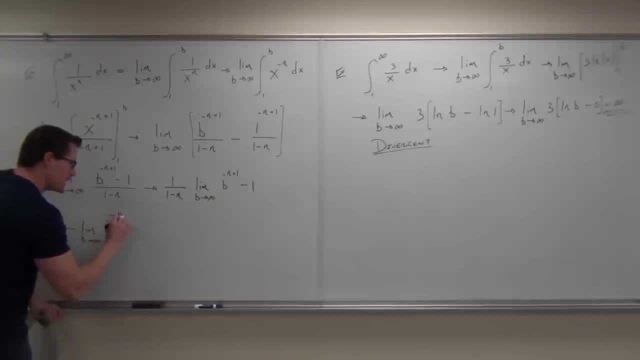 I'm going to force this to be b to the negative, n minus 1.. b to the negative, n minus 1.. Do you guys follow the math on that? Okay minus 1.. Probably need some parentheses here just to show what's happening. 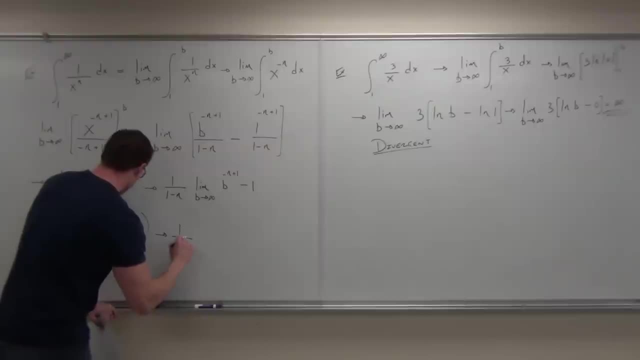 I'm also going to write this as a fraction Limit as b approaches infinity, Because this is now a negative exponent. what I'm going to do is I'm going to write this as 1 over b to the n minus 1 minus 1.. 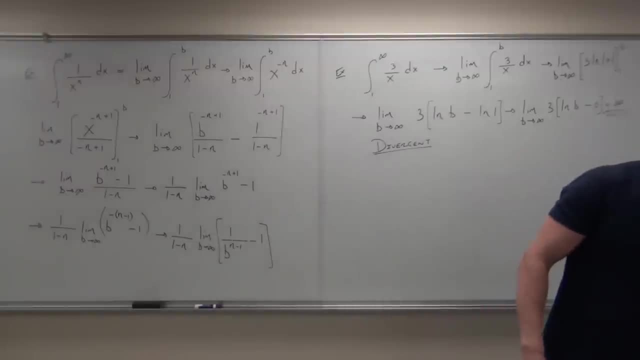 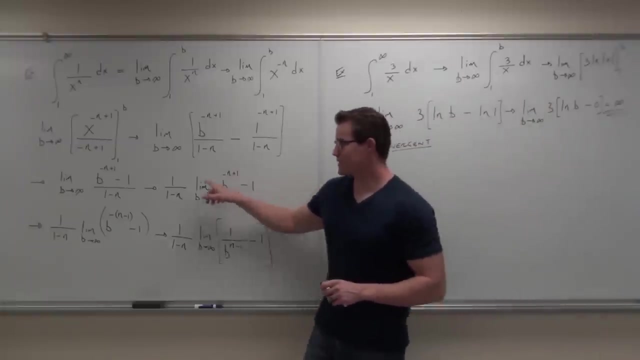 Are we okay with that one? Are you sure Some of you guys are zoning out? Don't zone out now, man, You've got to be with me here, So you okay with that? Factoring out the negative from the exponent. 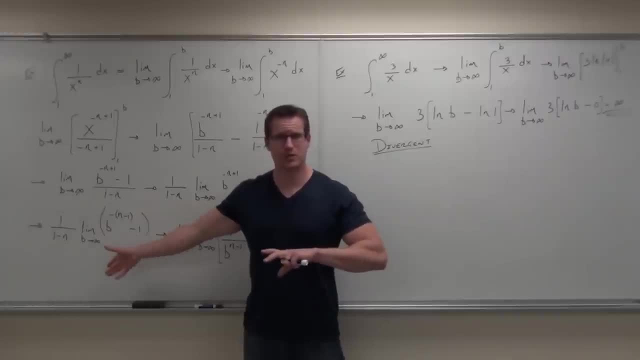 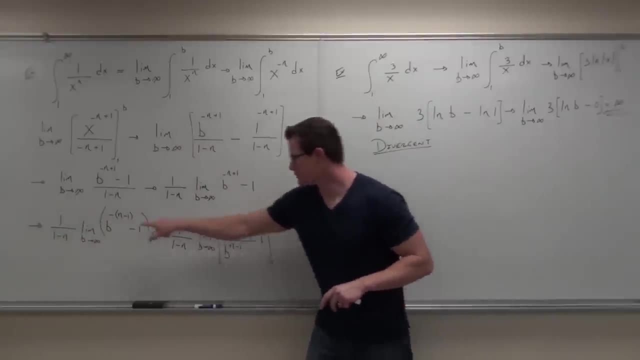 If we have a negative exponent, hey, you can write this as 1 over b to the positive exponent. That's all I've done here. So 1 over 1 minus n, no problem. Limit limit: This is this minus 1 minus 1.. 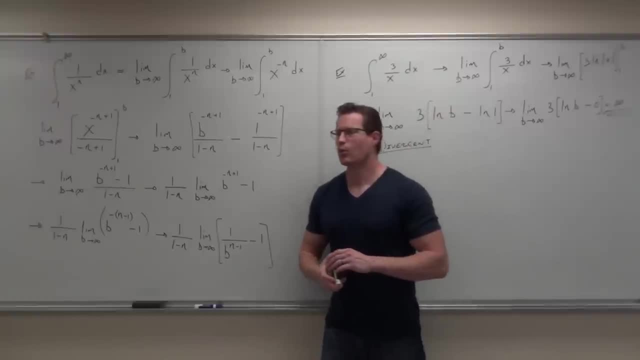 So far, so good. Yeah. Now let's think about this for a second. When is this going to converge, When is it going to diverge? Because we want to do this once and for all. So let's think about this. 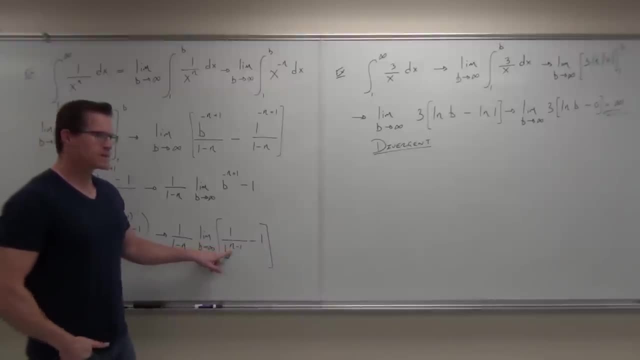 Let's say that n. Let's say that n Is well, how about we get? n is 1.. If n is 1, think back. just stop with me for a second. okay, If n is 1, then this was 1, correct. 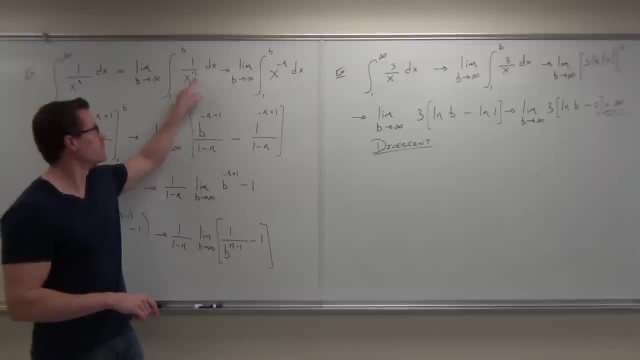 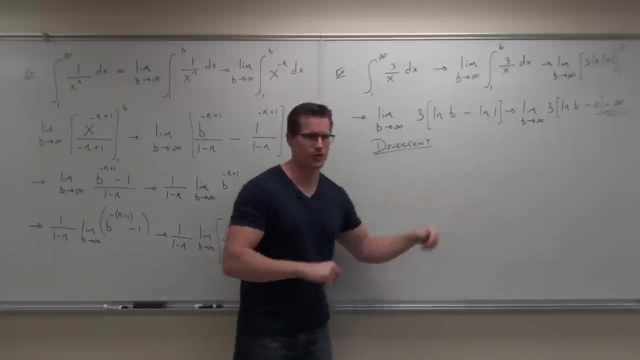 Are you listening? Yes, I need your attention here. If n is 1,, then this was 1.. We've already dealt with that case. We know it's divergent. Does that make sense? So we're going to have anything that, where n is 1, is divergent. 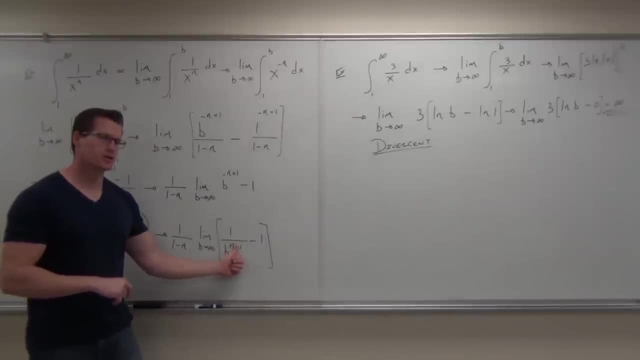 If you got that here, you'd actually get infinity to the 0. It turns out that when you do remember our indeterminate forms, When you did that, you'd end up getting undefined. out of that you'd get infinity. So that would be an issue for us. 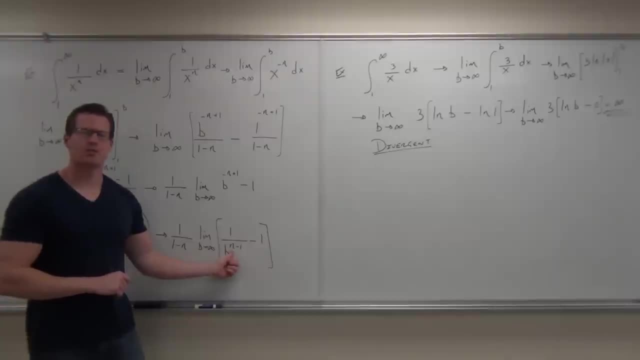 So n equals 1, we know it's divergent. How about n equals 2?? Let's think about n equals 2.. If n equals 2, what's 2 minus 1? 1. This would be like infinity to the first power. 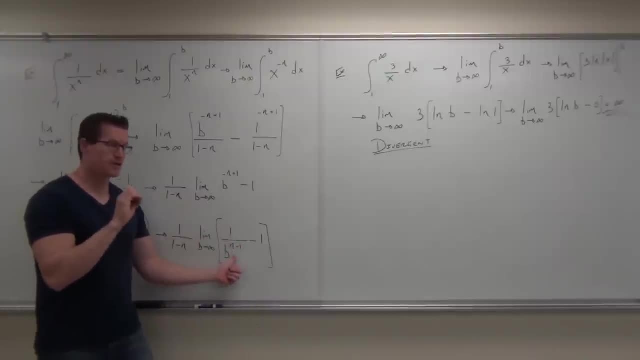 That's infinity. What's 1 over infinity? 0.. This would be convergent. You'd actually get a number out of that. How about 3?? What if n is 3? 2. Same deal, Or 4.. 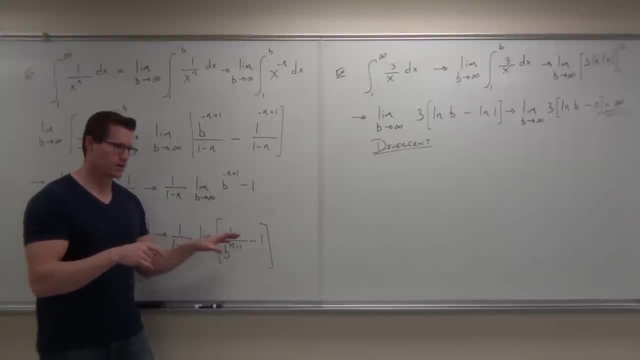 Or 5.. Same deal Now. we already did the 1, correct. What if n was 0, or negative 1, or negative 2?? If n is 0, we'd get 0 minus 1.. How much is that? 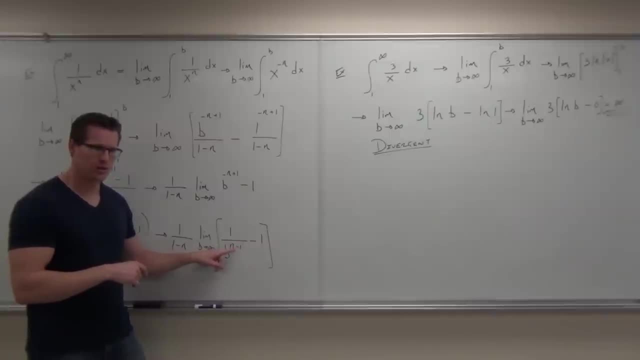 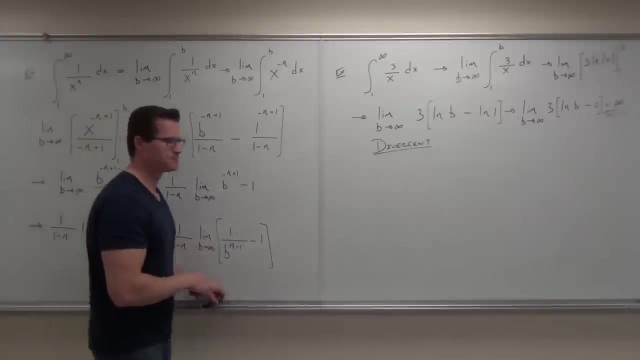 Negative 1.. So, basically, we'd have b to the negative 1, wouldn't we? That would be b to the first up here. That would be infinity. Do you guys get what I'm talking about? So we get this. 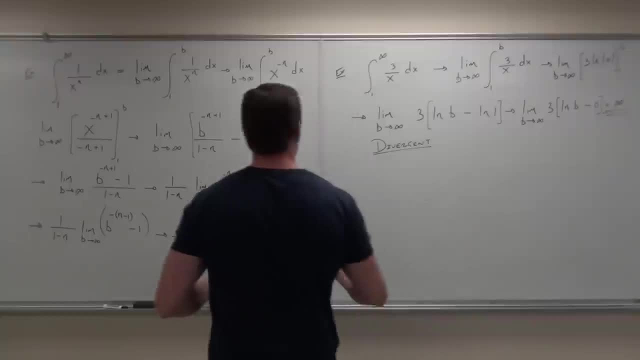 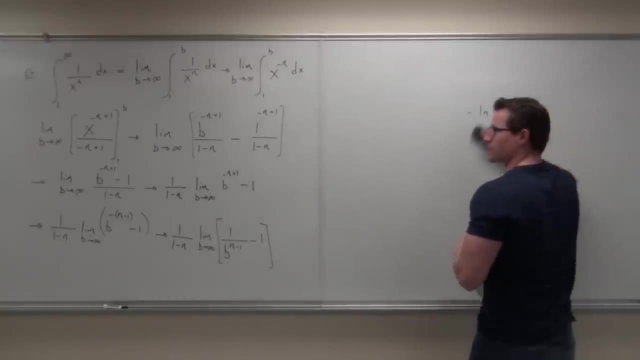 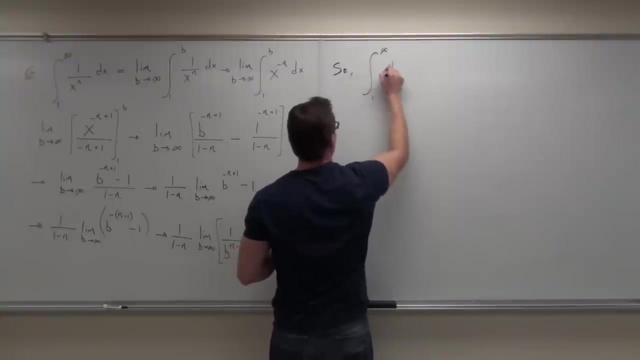 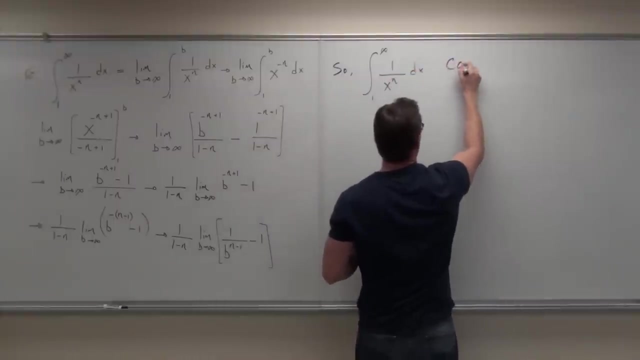 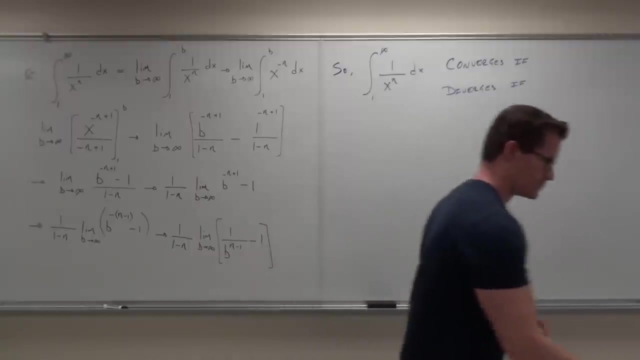 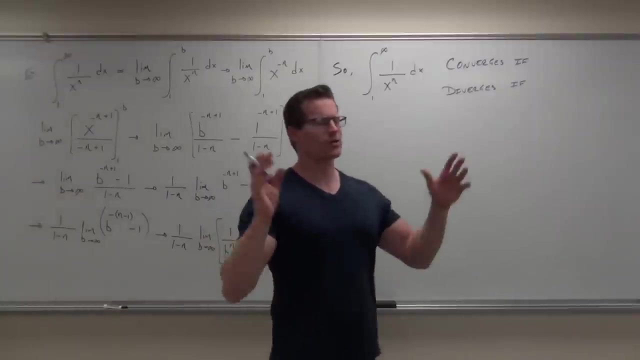 we get this statement. I'm going to write it right up here. So from all this stuff we know a couple things. So let's think about the integral from 1 to infinity of 1 over x2.. I don't care what it is. 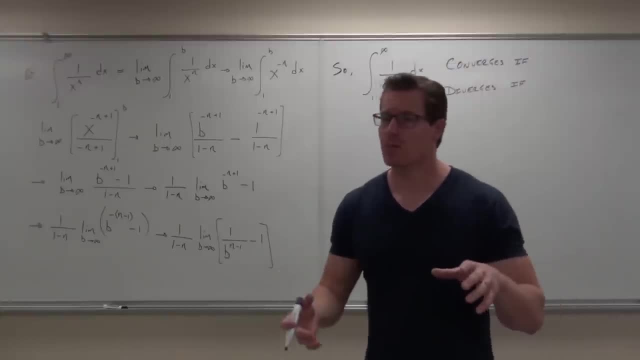 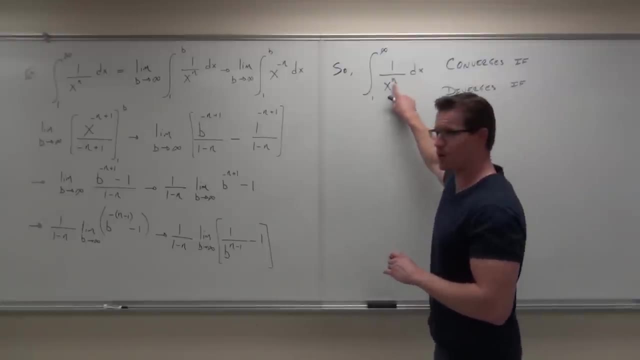 You can do it now without well, you can't evaluate it, but you can see whether you should evaluate it or not. So check it out. Let's say that x was to the first power. We already dealt with that. That was divergent. 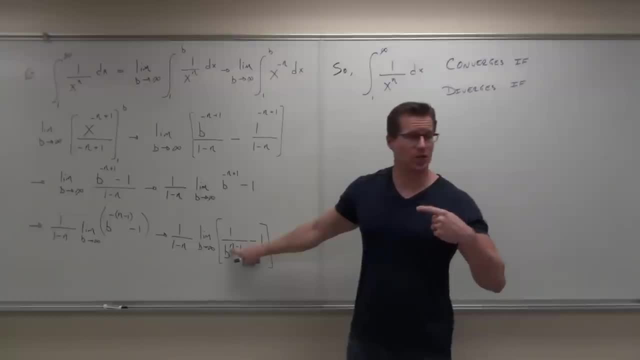 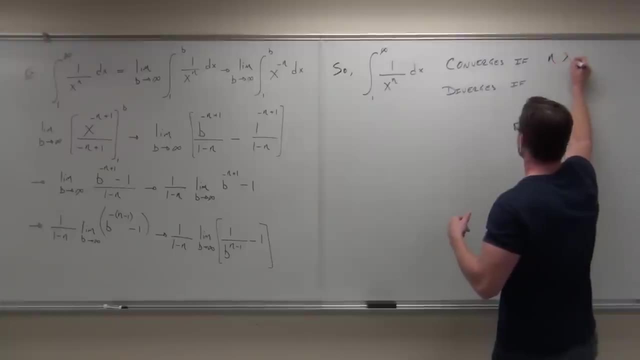 Let's say x was to the second power, So n was 2.. We talked about that. That would be convergent Or 3, convergent Or 4, convergent. Basically this is convergent if n is greater than what number, please? 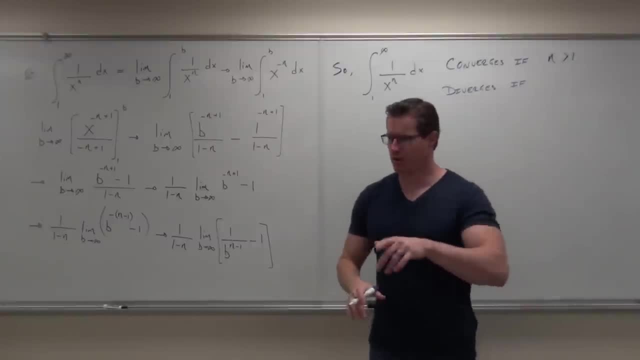 1. 1,, yeah, Not equal to 1,, but greater than 1.. If n is 2 or 3 or 4 or 5 or 6,, then we have infinity to the positive power. Infinity to a positive power would be infinity. 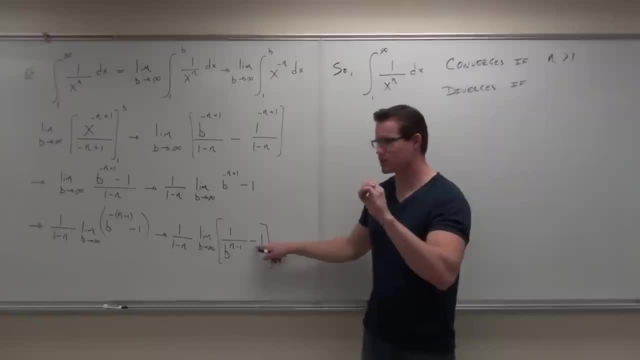 1 over infinity is 0.. 0 minus 1 is negative 1.. No big deal. That would be negative 1 times whatever this is. Does that make sense? Now, that's kind of cool, right? It gives you almost a formula for doing that. 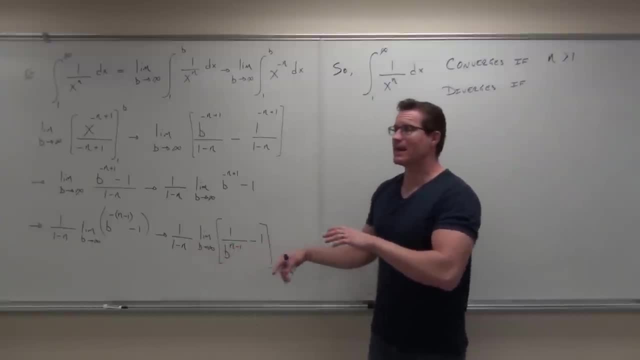 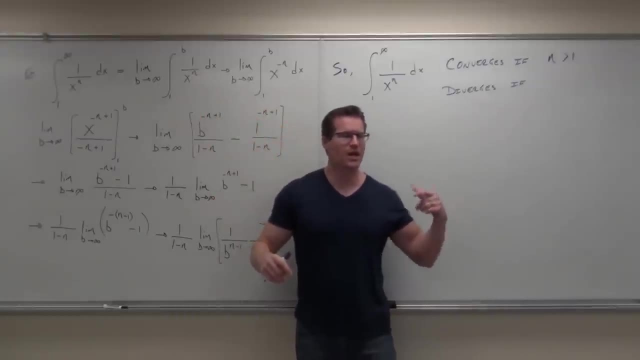 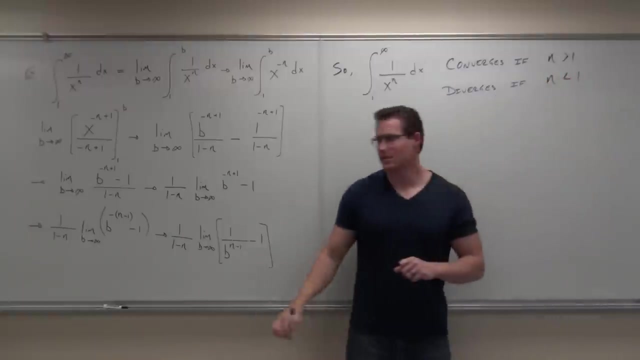 Cool, Now let's say that n was equal to 1.. We talked about that. If n equals 1, I have an ln. We just did the ln That diverged. If n is less than 1, if n is less than 1, we have 0 or negative 1 or negative 2.. 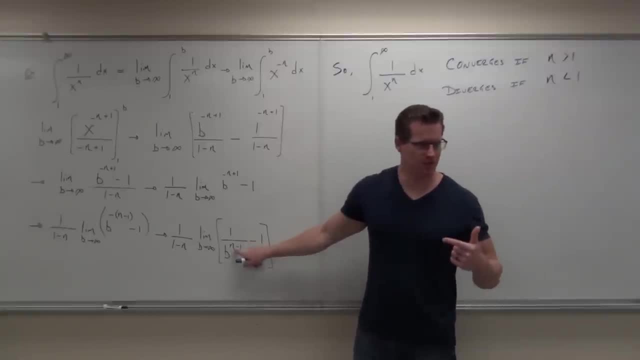 We'd get b to a negative power. Are you with me? b to a negative power is the same thing under 1, is the same thing as b to a positive power. by itself, Infinity to a positive power is infinity, Infinity minus 1, I don't care what you do, it's still infinity. 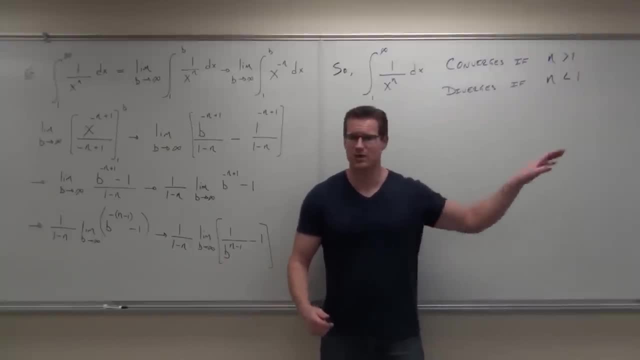 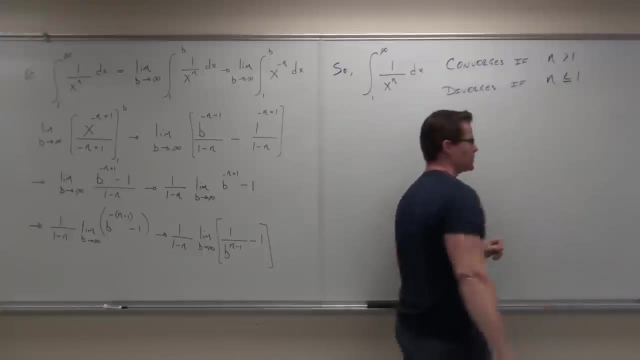 That's an infinite limit. That limit is not going to exist for something that's going to be convergent. So, basically, this convergence of n is bigger than 1.. Divergence of n is less than or equal to 1.. That's the idea. 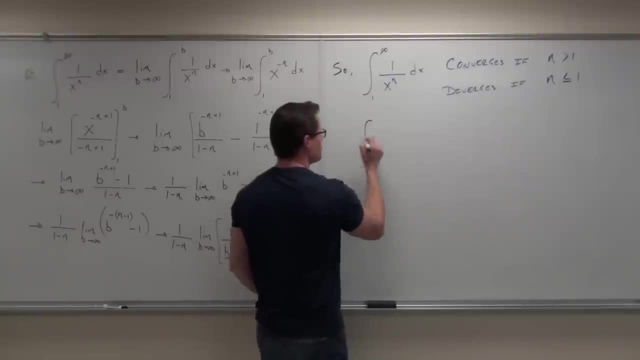 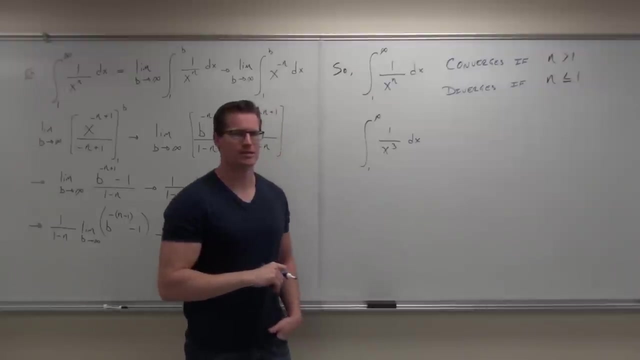 So here's what I'm trying to tell you. If I give you this, should you bother to find out whether this thing has a limit or not. Absolutely, because that's a positive exponent. That's n equals 3.. No problem, It's bigger than 1.. 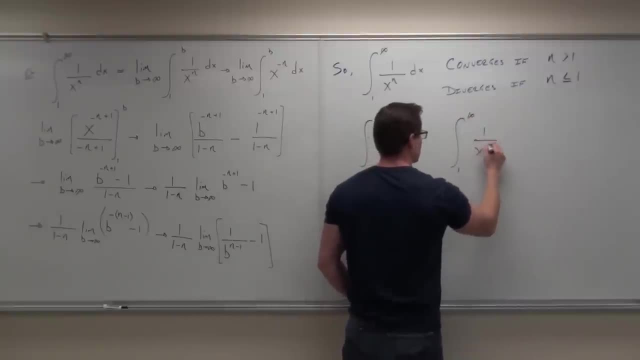 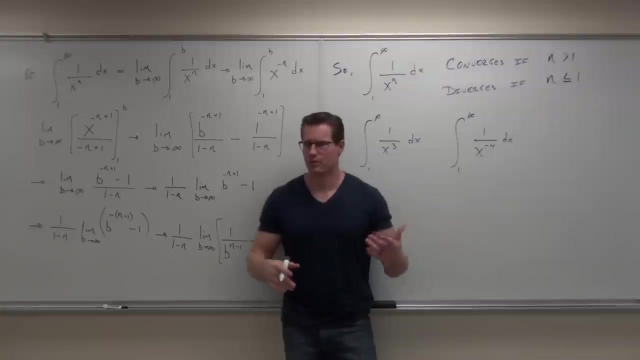 But if I give you this one, would you bother? No, Heck, no, You know automatically that's going to be divergent, For sure. Don't even worry about it. Just say: oh, look at that, n is less than 1.. 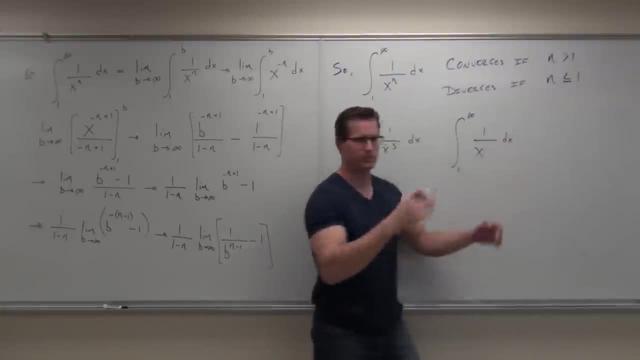 Hello, Divergent. Or if it equals 1, if it's that, don't even worry about it. That's going to be divergent, You with me, OK, so that's. that's kind of a nice little thing that we can do here. 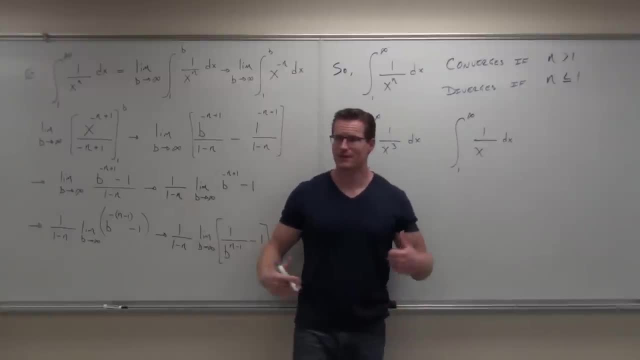 Just look at that. Did it make sense to you, this whole explanation? There's one more thing I was going to say. I don't remember what it was. I don't remember that important. Oh yeah, I know what it was. 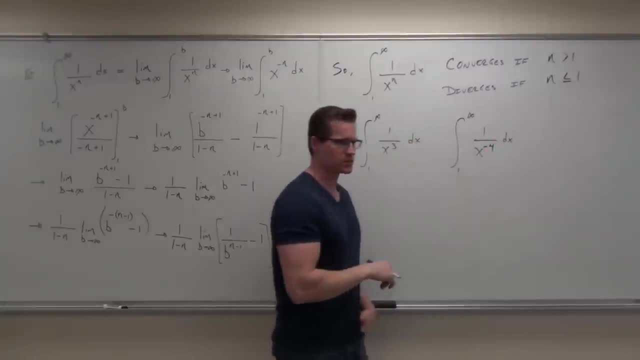 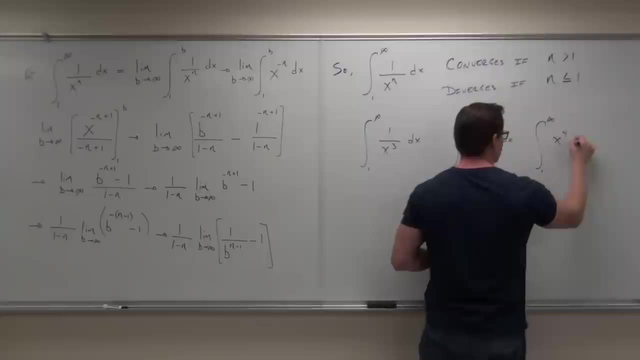 What that basically says is that, because all of these negative powers are going to be divergent, change that into a positive, And what you end up getting is x to the fourth dx, don't you? You get a polynomial. I realize that if I take an integral from 1 to infinity of any polynomial, 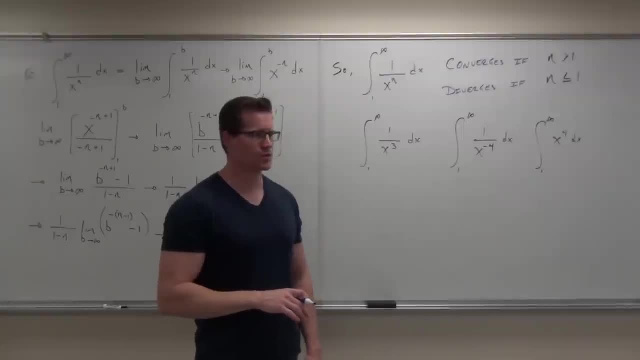 polynomials don't have negative powers. OK, any polynomial polynomials go like this or they go like this. that's their end behavior. It's either positive infinity or negative infinity. Are any of those limits going to be convergent for us? 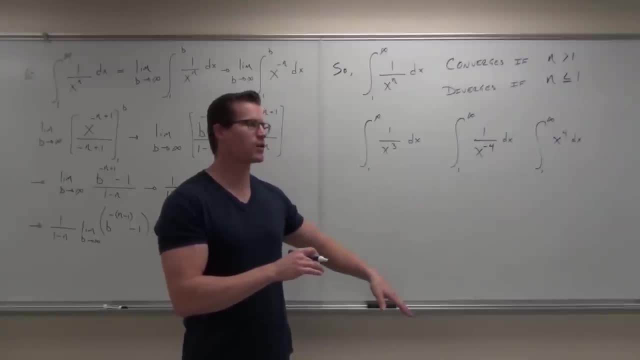 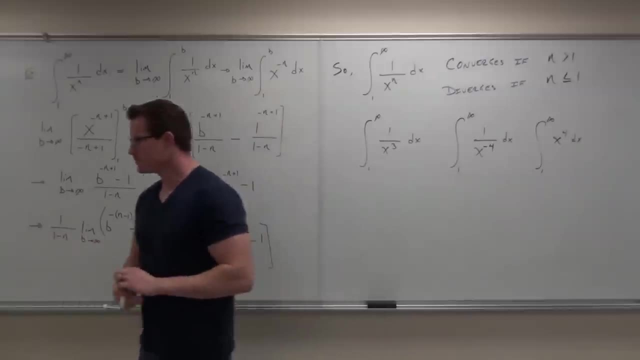 No, They're going to exist, but they're going to be positive infinity or negative infinity. They're not going to exist to a finite number. Therefore, these integrals will all be divergent. Does that make sense to you? OK, 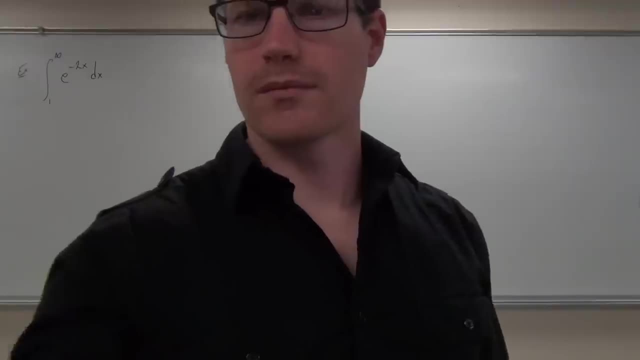 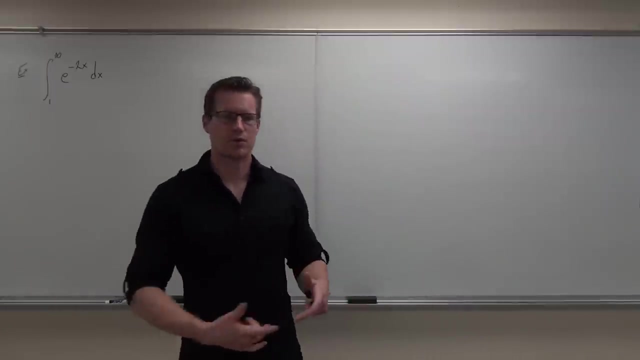 We're going to stop there. We'll continue with this next time. All right, let's get started on our next example. The next example is another case of where we have these infinite intervals, where we're starting in a number, or we're starting at infinity, but we're going. 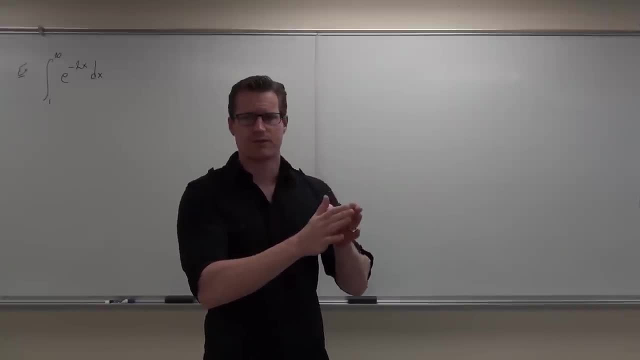 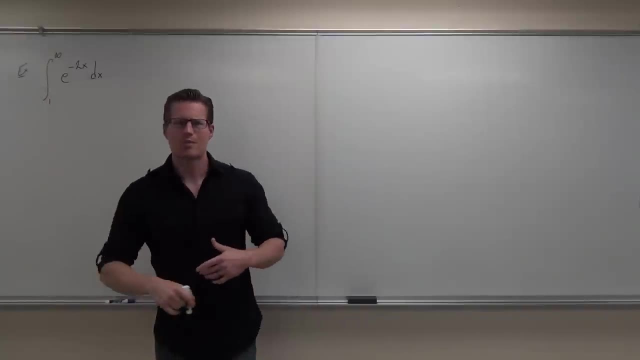 we have one section that's defined, like one part of the interval is defined and one section that's not. So here we have- yeah, we're starting at one, but we're not ever ending. We're going to infinity. Do you remember what we do right off the bat when we have a scenario like this? 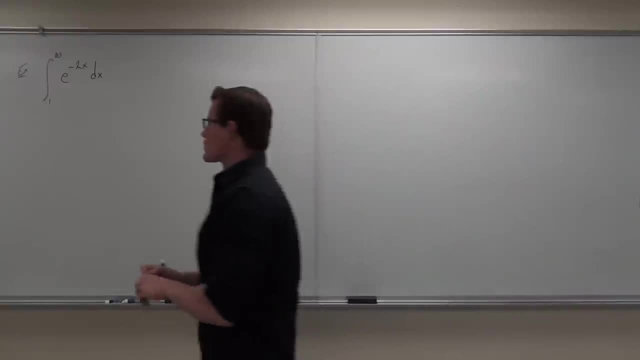 What's the idea? It's a limit. That's right. So what we're saying is that, no, we really can't go to infinity the way we want to, because we can't really plug in infinity since we don't know what it is. 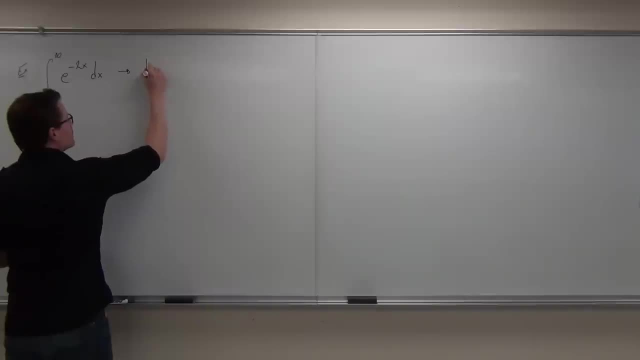 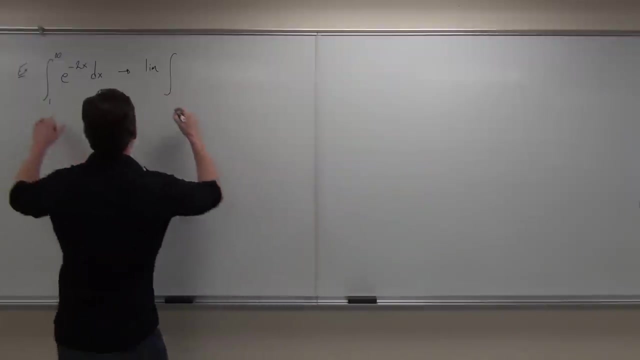 But what we can do is we can say: all right, well, I know I could take a limit from what's our problem here. Is it the one or the infinity? Of course it is The one's great, The infinity. we call that some letter. 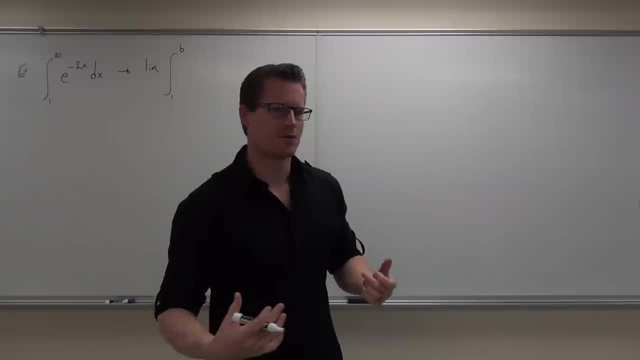 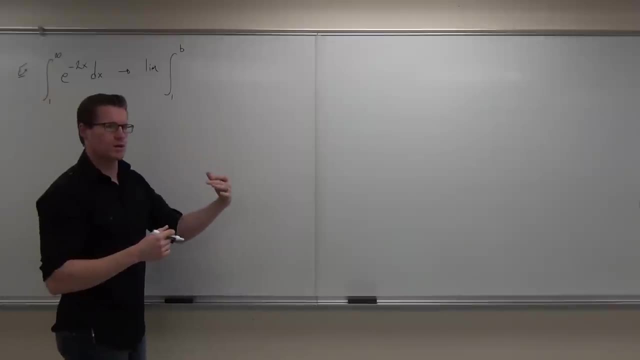 We typically call the upper bound B and the lower bound A. So if your infinity is in the upper bound, call it B, And then what we say is all right. well, this is fine. This now becomes something that we're going to use: a definite integral four where B is a number. 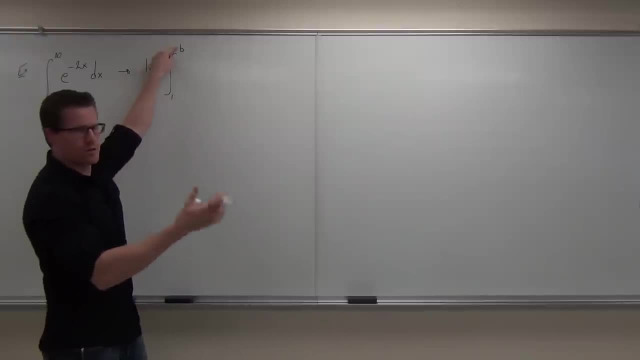 The limit idea says: OK, now you're going from one to some number bigger than one. This is the idea. Then the limit says: OK, now take that number that you're going to, which we call the B, and move it forever to the right. 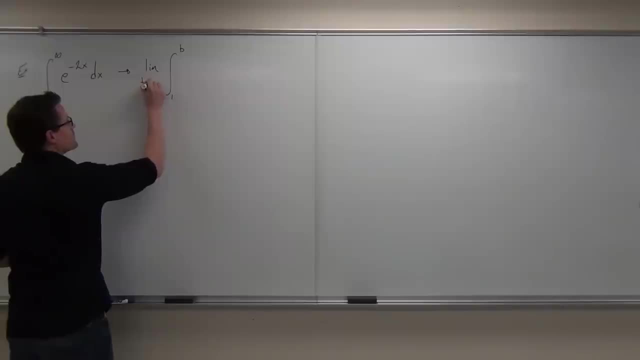 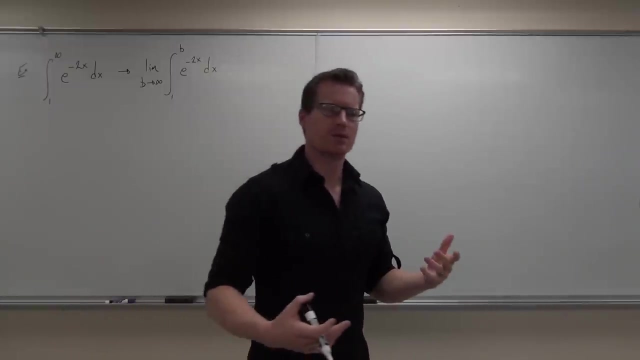 So move it forever towards infinity, And that's why we have to have this limit here And the rest of the integral well, it doesn't change After that. the nice thing about these: well, we know integration techniques. We spent all this time doing it, which is a fantastic question. 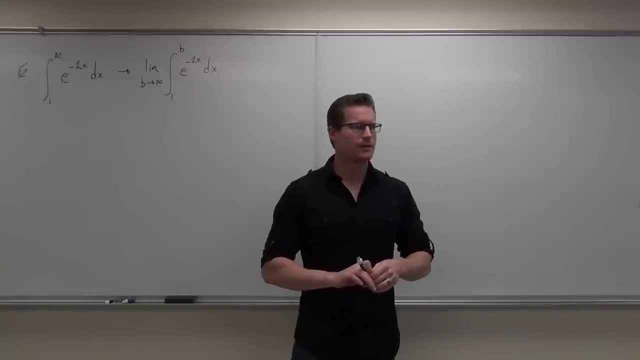 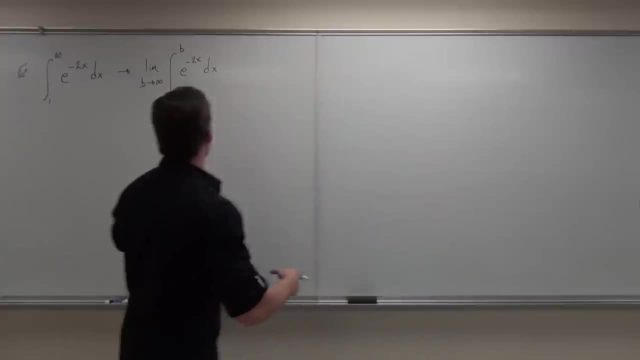 If we just avoid writing that to the end, is that technically incorrect? Yep, Yep, We got to. you have to write the limit You have to have. everything I'm showing you is what you need, Because if you just go from one to B, that doesn't make sense. 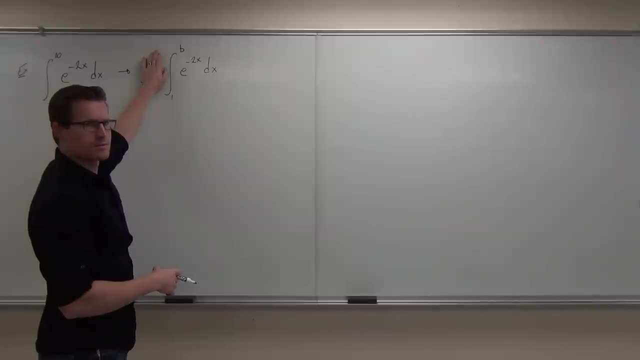 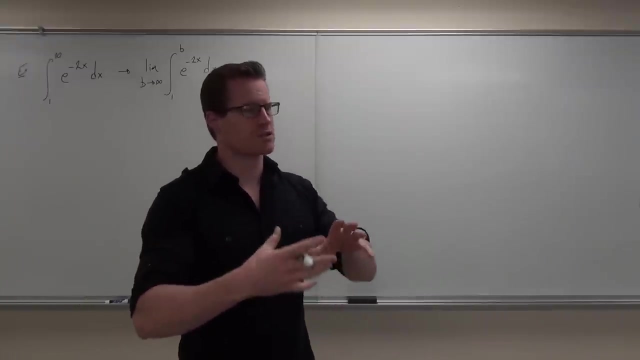 I meant just avoiding the B altogether until you use the actual. You could do the integral first. I prefer you doing the limit. This is what's what's going on here. We're changing to a definite integral where B is just some number to the right of one or whatever number you're given. 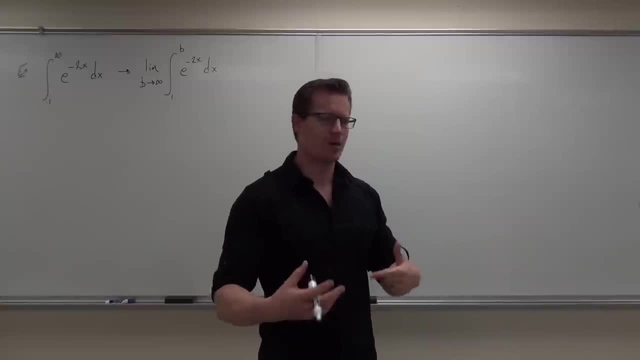 Then you do it, and then you evaluate with B, and then you take your limit. Really, that's a proper form, Super big deal for some people. I don't know. I'd like you to do it this way though. OK, so continuing. 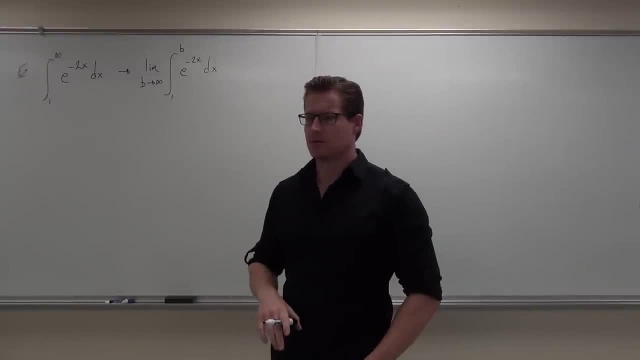 Can we do an integral like that one? Hello, can you do the integral? That's pretty easy. What are you going to do with it? Too bad. I deal with a lot of people who come up with questions going: man, how do I do this? 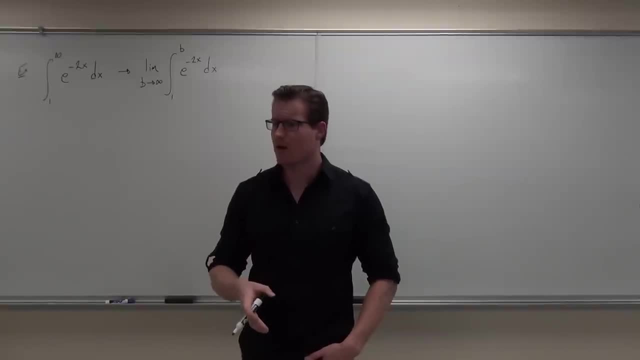 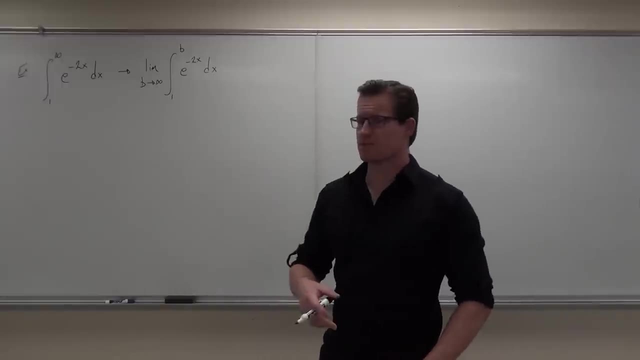 And I'm looking at you guys are making this way too hard, way too hard. Start with the easy stuff. Calculus is supposed to be. well, how can you make it easier? All right. So when we look at this, we're not. we're not thinking integration by parts are off the bat or whatever. 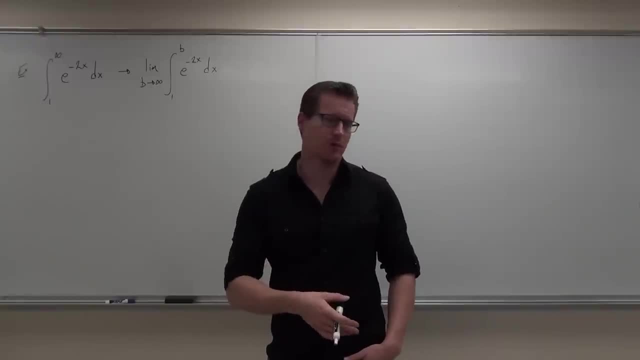 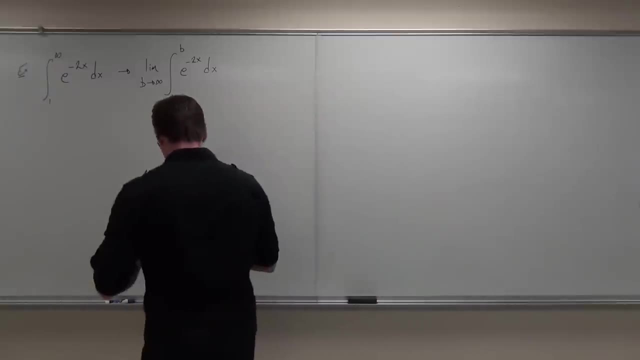 We're thinking: well, do basics, Is it in your integration table? Well, no, Can you do it with a U sub? Yes, Yeah, Do a U sub. then Do something simple if you can. So with us we go: OK, cool, well, we can do a U sub. 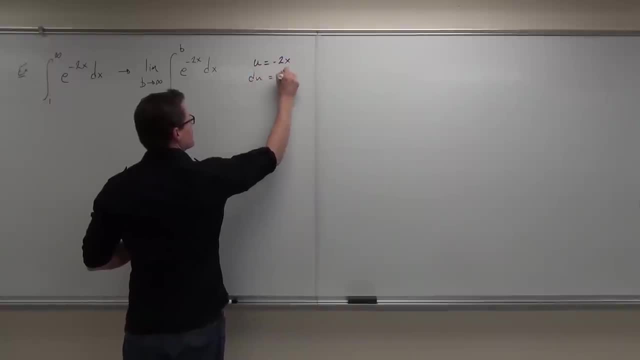 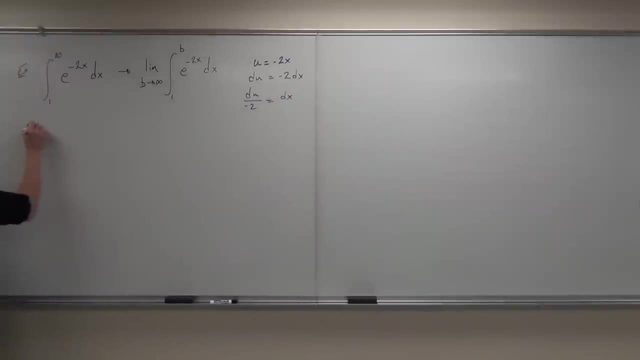 So U equals negative two, X, D, U equals negative two D X, or D U over negative two equals D X, Something really nice. What that means is we get the limit Forgot the limit. We get the limit as B approaches infinity of the integral from one to B. 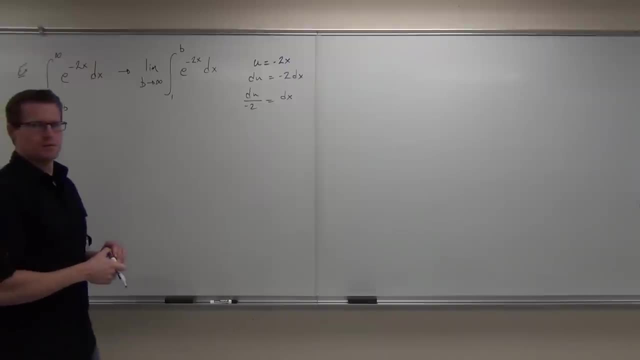 What's going to be on the inside of our integral? E to the U, E to the U, That's right, E to the U, And then D X, No, no, no, no, We got D U over negative two. 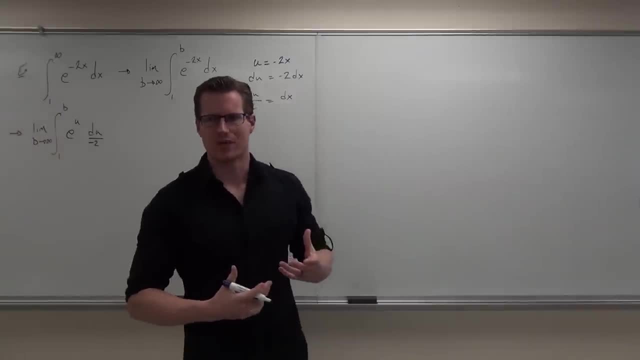 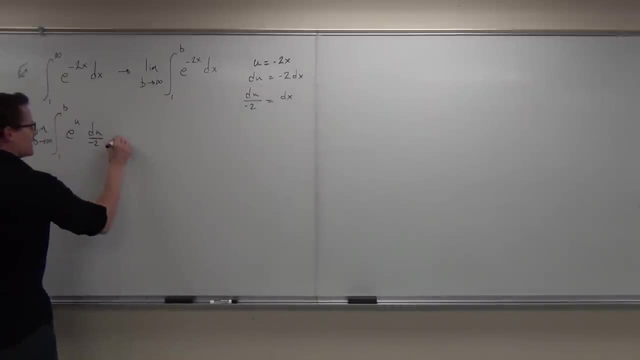 This is actually kind of a pleasant break for us as far as dealing with some simple integrals. isn't it Kind of nice where we know how to do these? They don't take four pages for one problem. What are you going to do now? What do you think? 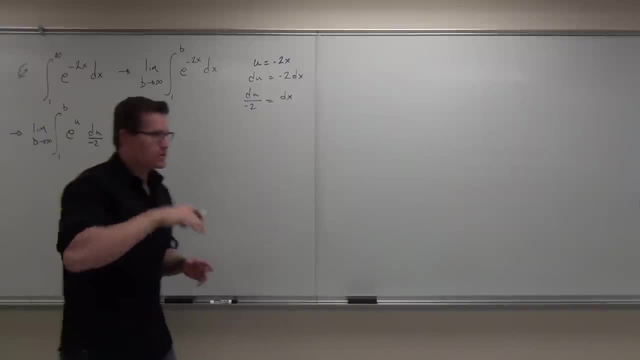 OK, so you know what you can actually do. I don't know if you know this, but you can bring that negative one half to the front of your integral, But you can also do it In front of the limit. So whatever you want, if you want to bring it all the way out front. 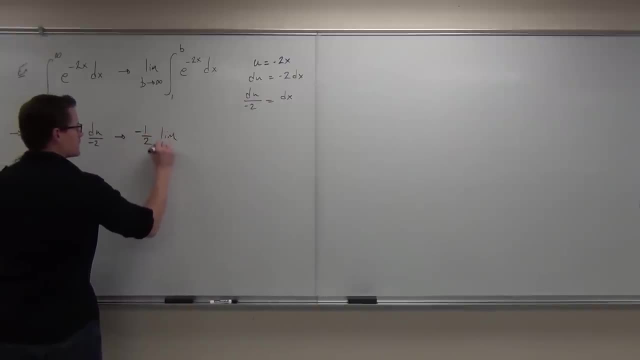 just do negative one half times the limit. as B approaches infinity, I'm also going to do the integral. So we pulled out the the negative one half. What's the integral? Remember this would be gone right. This is our negative one half. 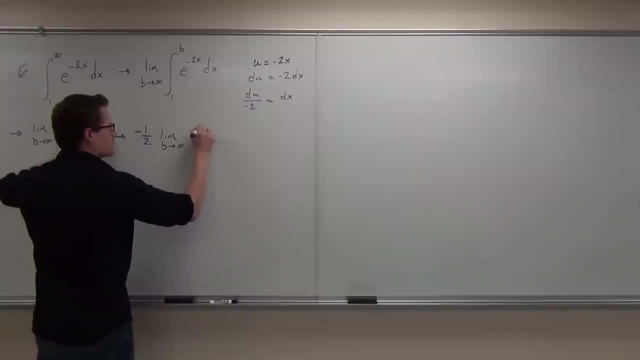 What's the integral of E to the U, E to the U. I love that integral. And then where are we evaluating? From one to B? Yeah, one to B, Notice how, if we pull out that negative one half, it makes what we're evaluating just a little bit easier. 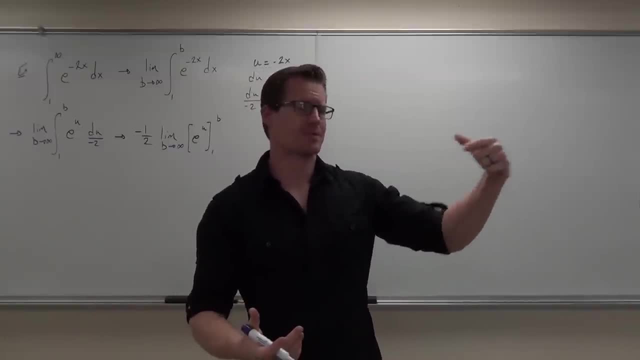 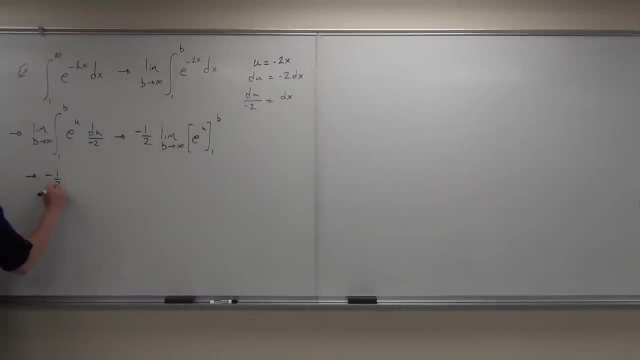 It's kind of nice. We don't even have to worry about that. It's just going to be negative one half times the limit. Quick head nod if you're OK with that. so far. Now we get to evaluate. So what we know is that we're going to have negative one half times the limit. 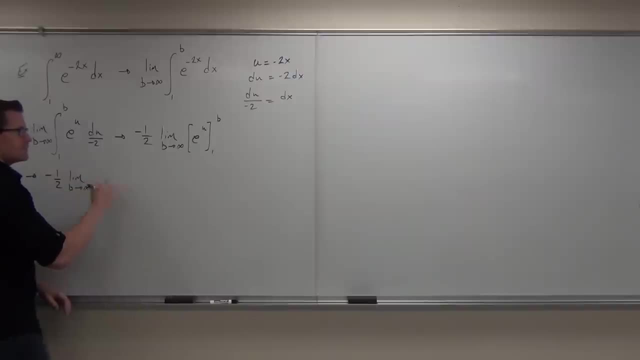 as B approaches infinity. Let's evaluate What goes first, The one or the B: E to the B minus E to the one. Now, if you're going to do this correctly, you do have to be very good at understanding what's happening. 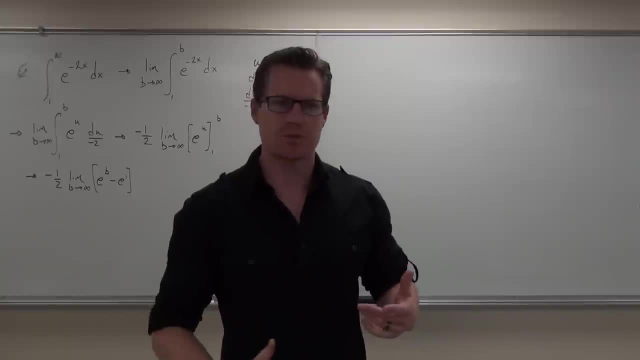 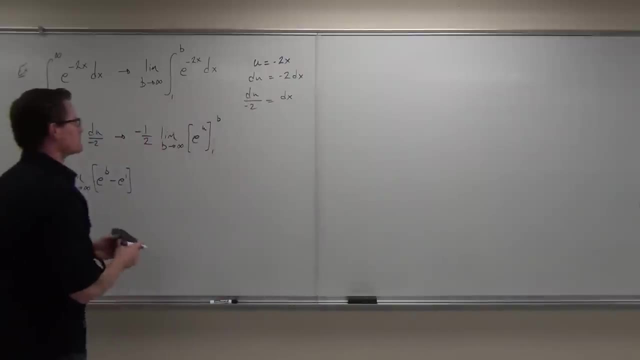 to these functions as you approach infinity. Some of you struggled with this when we dealt with limits the first time. Would I mess it up? What about the U substitution? Oh, my bad, It's actually going to matter to you. I got all wrapped up and talked about infinity. 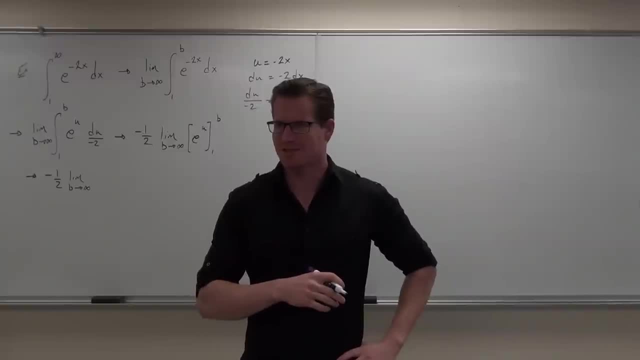 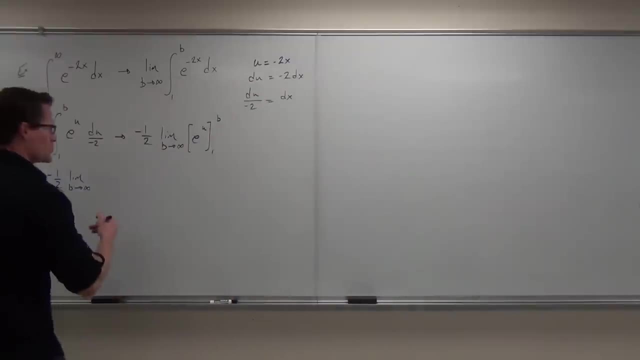 I forgot my substitution, Yumi, I was just testing you. You passed. Fantastic job. What do you do here? What do you do then? OK, yeah, So before we evaluate, you should have caught me earlier. Thanks a lot, guys. 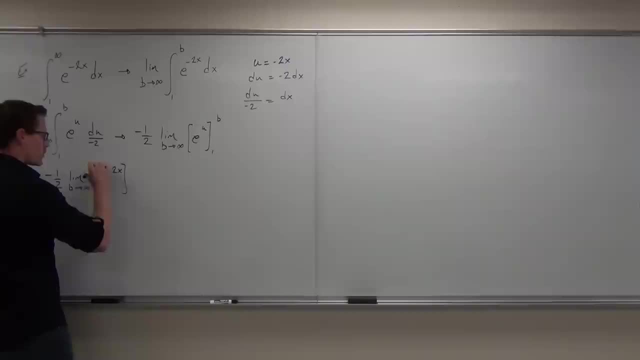 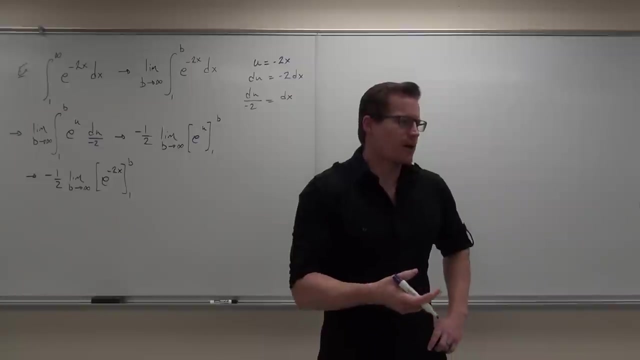 Limit of E to the negative two X. Yeah good, Why is that important? You know typically, typically, what I do in my substitution problems: I change bounds. So if you're used to doing it like I was, don't make the mistake that I did. 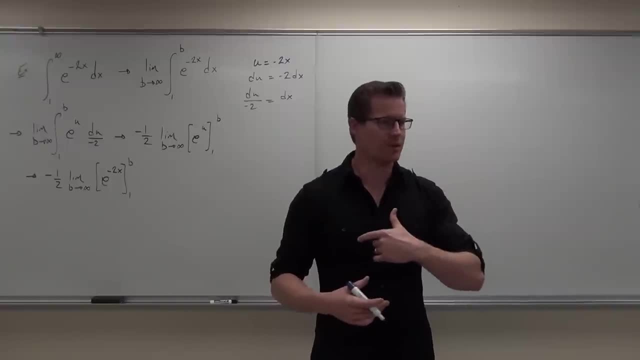 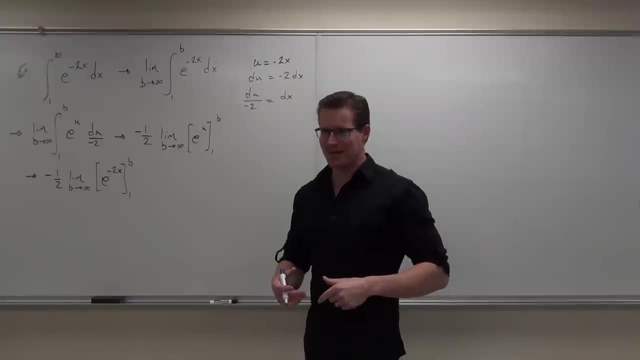 where you forgot to substitute back in for that U. That would have been a really big mistake. I'm glad you guys caught me on that, Did you? did everyone see the mistake that I made? It's on video. Watch it again. You can see the mistake that I made. 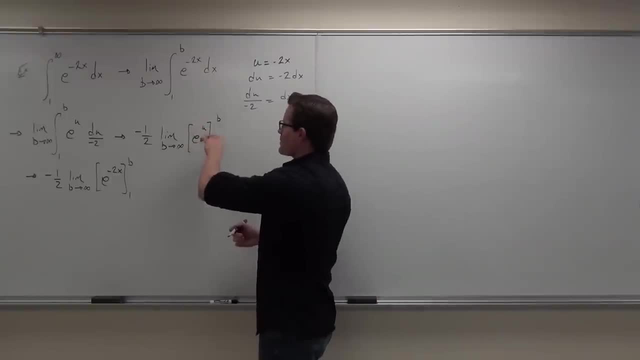 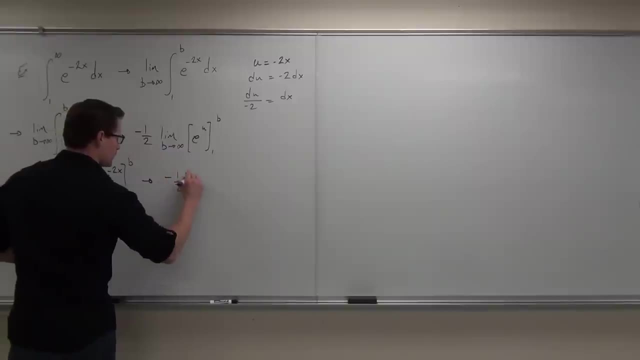 All right, Yeah, Make sure that you're actually doing that substitution back, because if you haven't changed your bounds, that's a must You have to do it. So very good job, Nice catch. So negative one half limit as B approaches infinity. 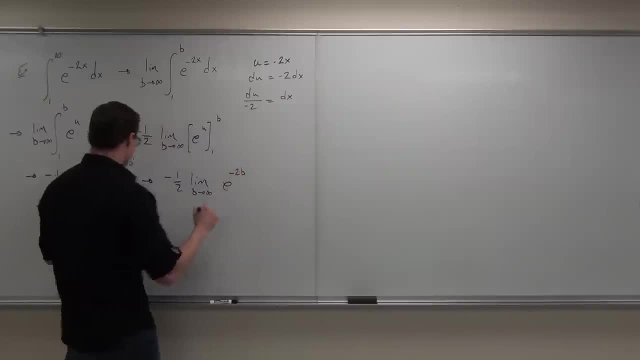 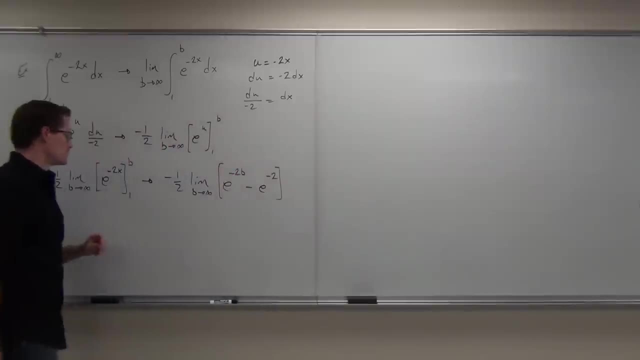 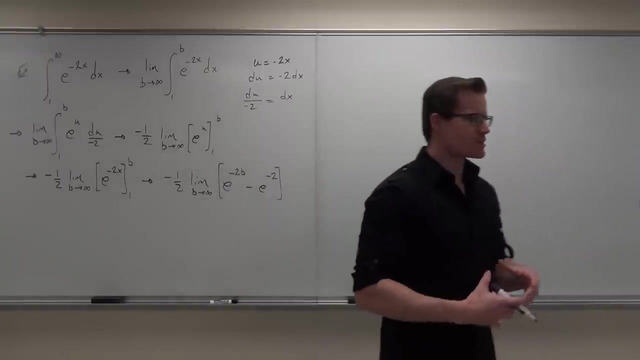 What we end up getting is E to the negative two, B minus E to the negative two. You still OK. so far, Yes, Well, maybe what we want to do is make this so it's a little bit more understandable on what's going on with our function. 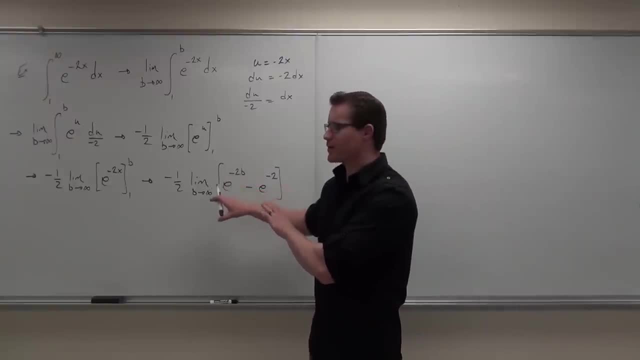 So if you can do it from right here, cool, Go ahead and evaluate your limit from right here. If you're the type of person that says, you know what I really don't like dealing with all these negative exponents that it's hard for me to do. 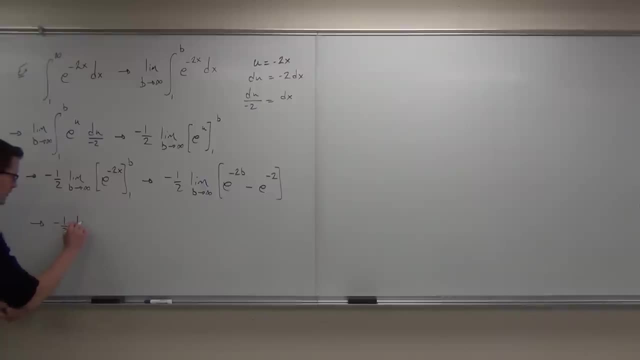 Well then, what I would do if I was you is I'd keep the negative one half out front, I'd write the limit as B approaches infinity, And then I'd rewrite these two things, because maybe that's going to be a little easier. 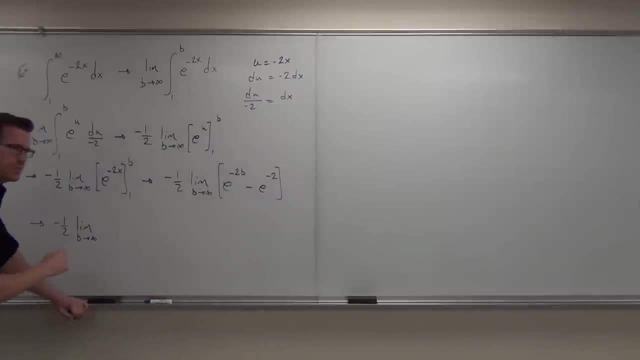 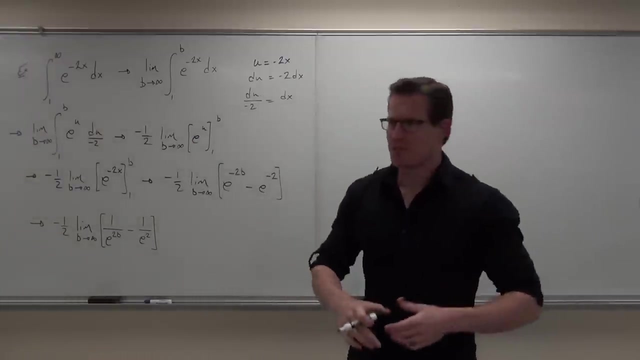 For you. how can you rewrite E to the negative two B? What could you do, Minus one over negative two square? Yeah, maybe that's a little bit easier to see what's happening. now Back to my point that I skipped over an important point to make. 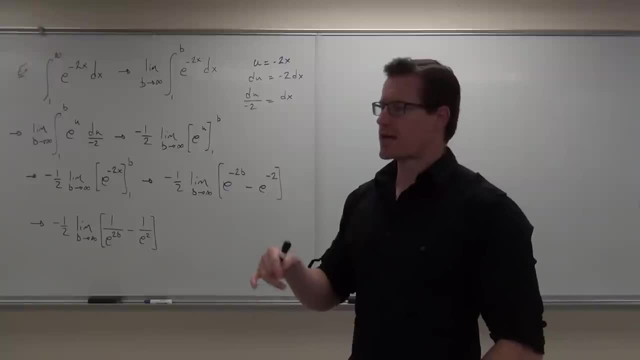 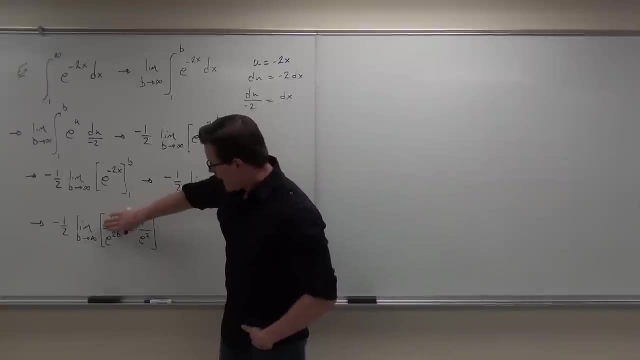 My point is this: You're going to be really good at determining what's happening to your function as you approach infinity or negative infinity. It's really important. It's really important to do that. So, when we look at this, what happens to E, to the two B, as that B goes to infinity? 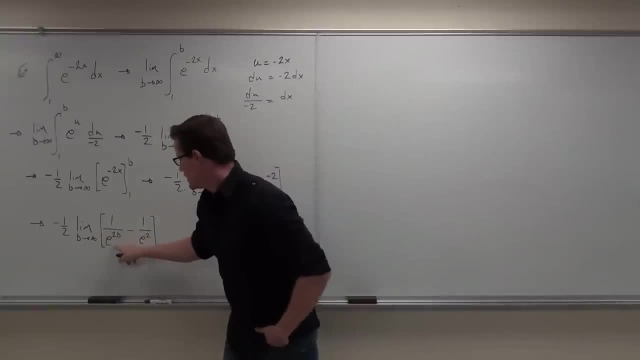 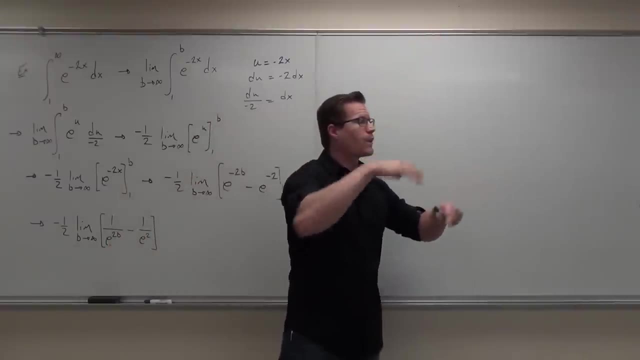 What's happening to that? This little piece goes to infinity. Remember what E looks like? E looks like this. So as X goes to infinity, E is going to infinity. What that means is that if we have one over, So, infinity two times infinity is infinity. 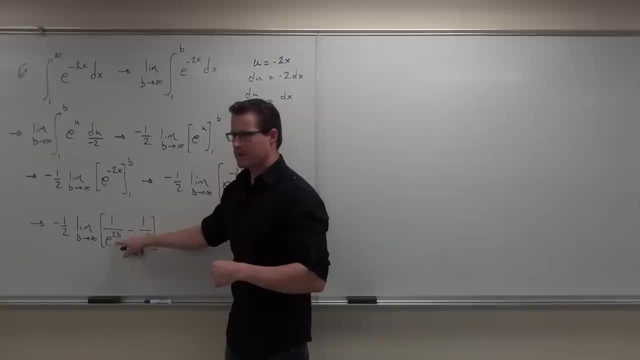 E to the infinity is infinity. How much is one over infinity? Yeah, this thing goes to zero. One over infinity is zero for sure. Now, what's this thing go to? This is B squared Nowhere. This is it. 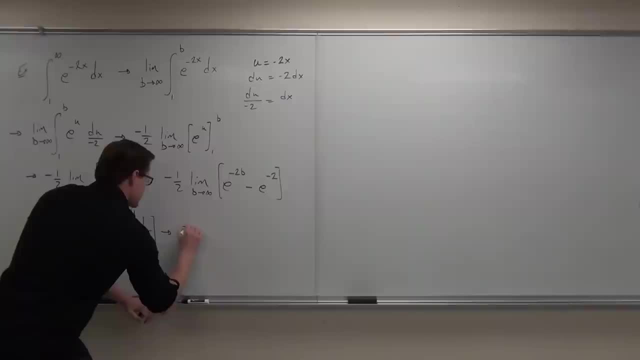 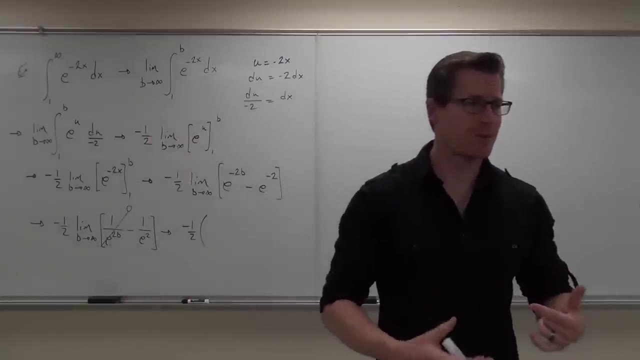 It's a constant. So what that means is that we're going to have this negative one half times. Notice how, when I evaluate the limit, when I evaluate as B goes to infinity, I stop writing limit, but I don't do it until I actually evaluate it. 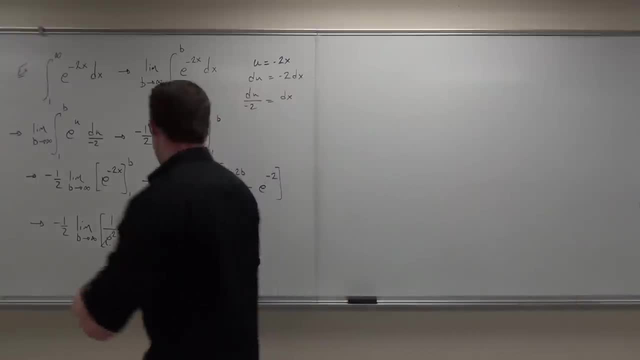 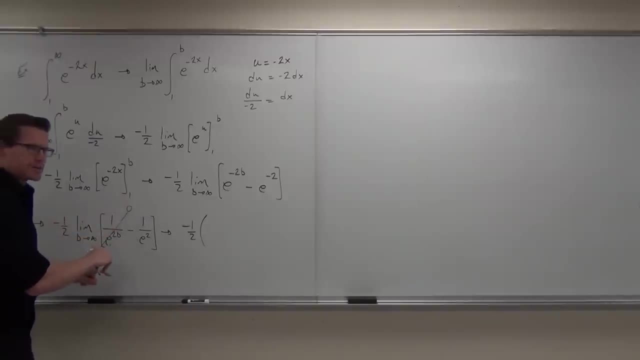 You guys clear on that one. We do have to have it every single time until we get down to: Oh, yeah, OK, When B goes to infinity, this thing goes to zero. Then in here we have what: OK, Zero minus one over E squared. 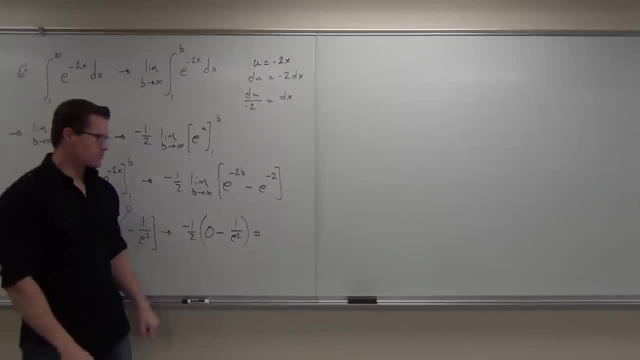 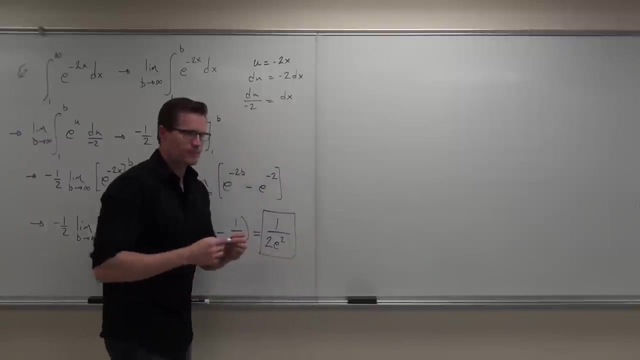 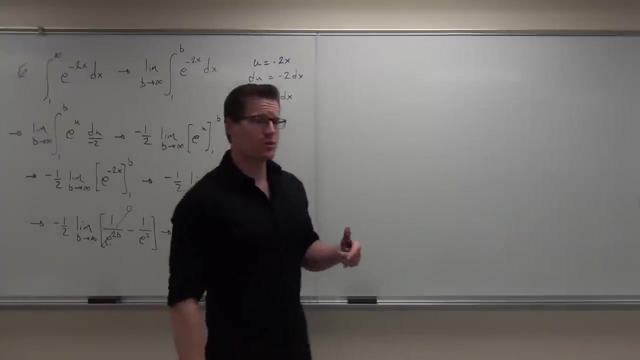 Which is equal to- let's do it- Negative one half times zero, minus one over E squared. How much are you going to get? Negative, positive, Positive one over two. Negative two over two E squared? What I find just amazing about this is that what we really did here is we found the area under a curve. 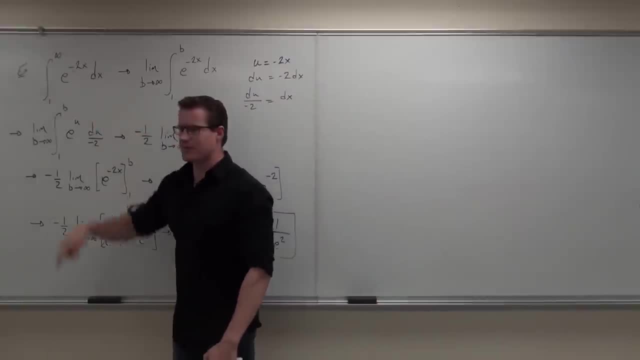 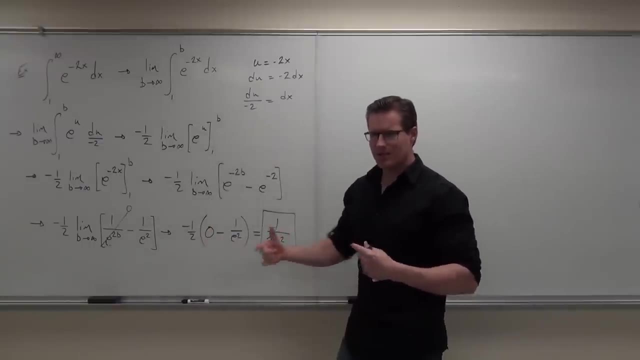 What curve, This curve. We've got an area under this curve from one to infinity. So start at the number one and going forever, And we got a legitimate area underneath. that thing Isn't that interesting. It means that we're getting so close to probably zero as we go to, or some numbers. 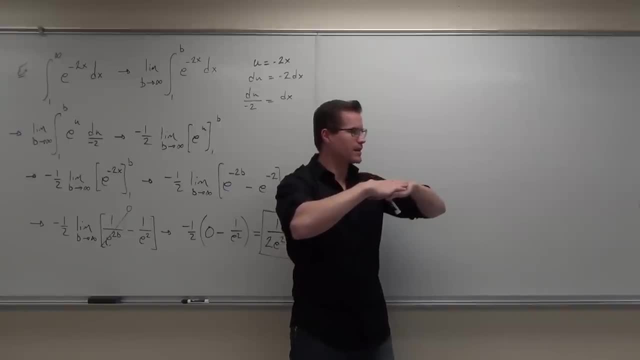 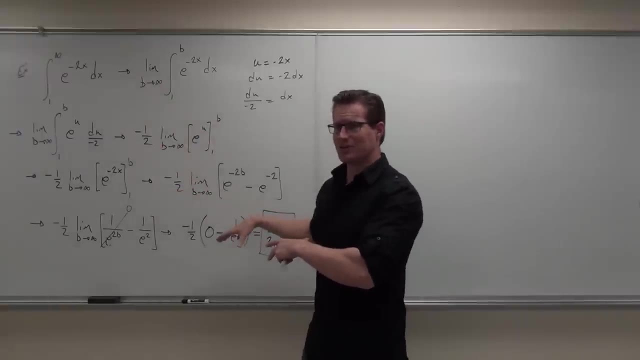 go to the right that it doesn't make any difference when we add that. That's kind of that's cool to me. I don't know why that's cool, but it's so cool. Does it cool to you that we can add something up from one to infinity and get an actual number? 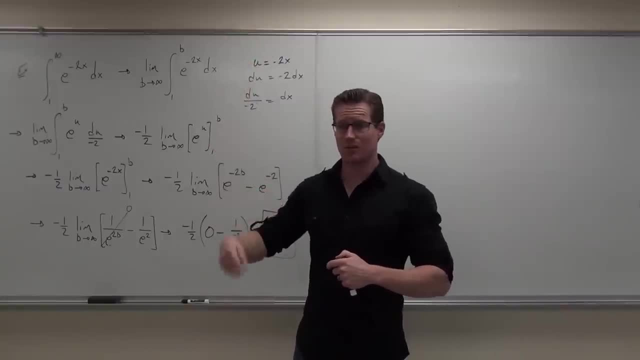 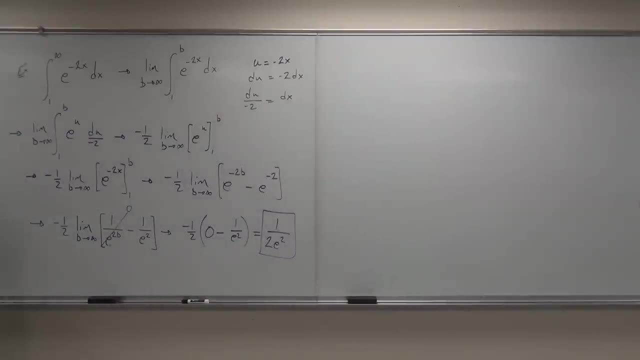 By the way, did the example make sense to us? Good, You guys want to keep going. We're going to make it a little bit more difficult as we go. Well, not more difficult, but more involved. I suppose I want to give you some different cases. 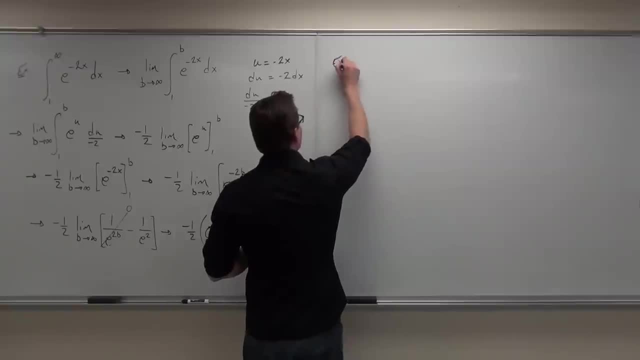 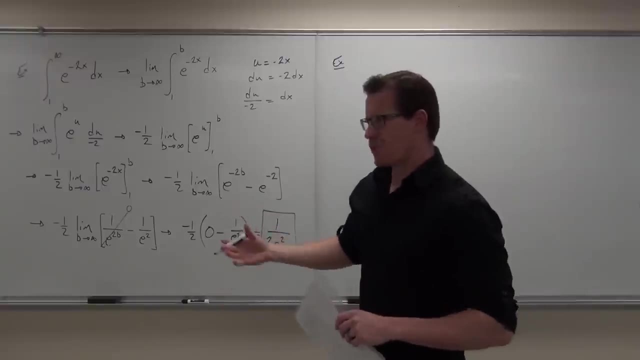 So let's continue. So I guess, long story made real short. the integrals are going to be very similar to what you've done before. One is you need to identify what type of improper integral we have, whether we have an infinite interval or an infinite. 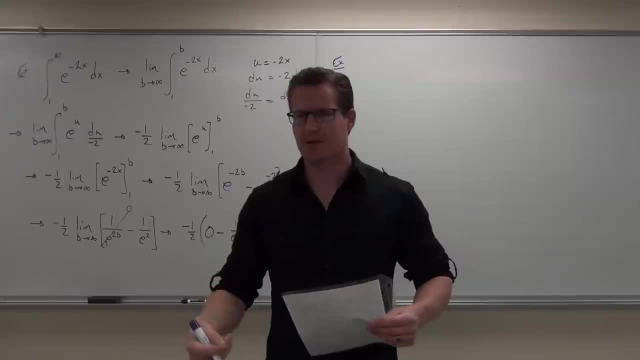 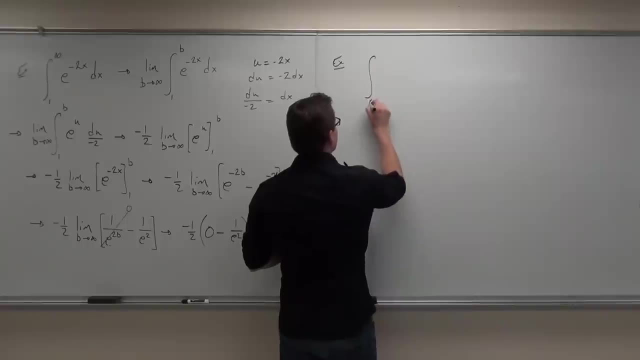 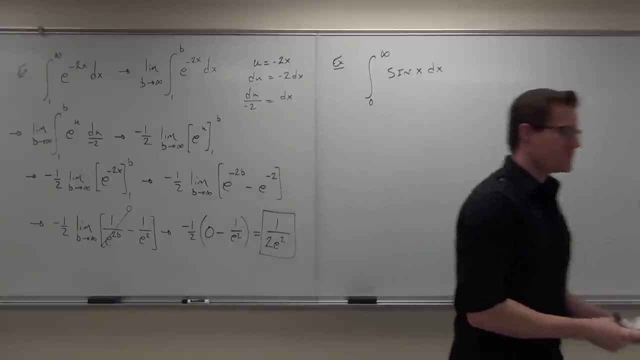 I'm sorry, emphasize the wrong level- an infinite discontinuity there. So, whether we have a discontinuity or infinite interval, So in our case here, when we get this one, What do we got? Do we have an infinite discontinuity or do we have an infinite interval? 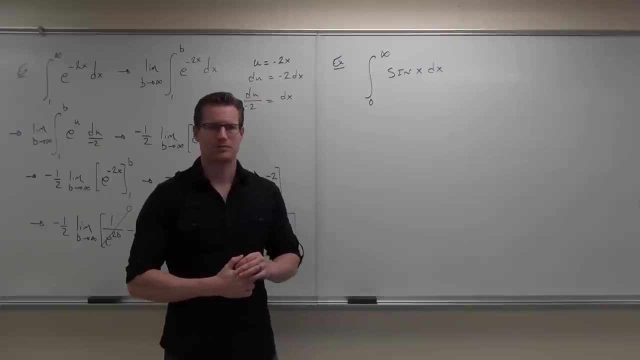 Which one? Both, Neither One or the other. What do you think? Do you know? I want you to think about sine. Are there any problems with sine? ever Do you ever have a discontinuity on the function sine? Never. It goes like this forever and ever. 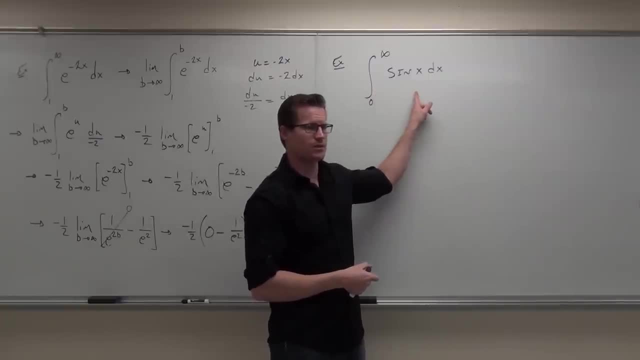 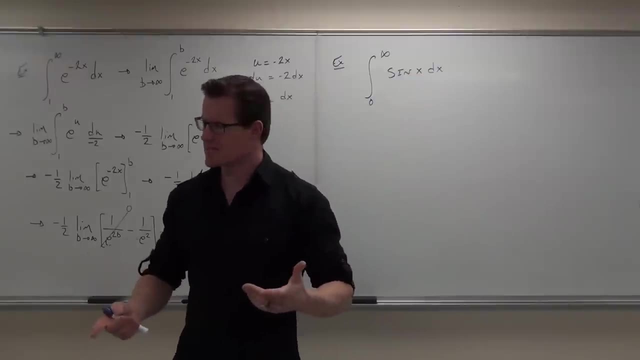 So from zero to infinity, are we going to have an infinite discontinuity? No, we're good. It's going to be defined for this entire range of numbers, because it's defined for the entire interval of numbers. Does that make sense to you? 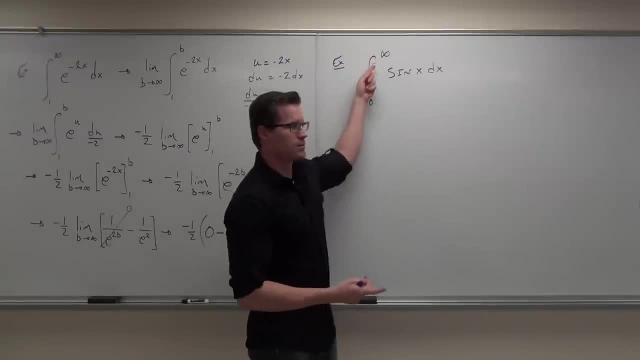 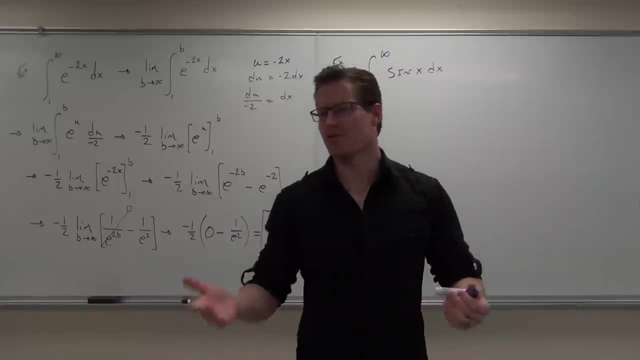 Now we do have a situation here. We have: we've got the infinity. This would be called an infinite interval. So I want you to do the first step. Write this as, instead of going from zero to infinity, we're going to go from zero to what? 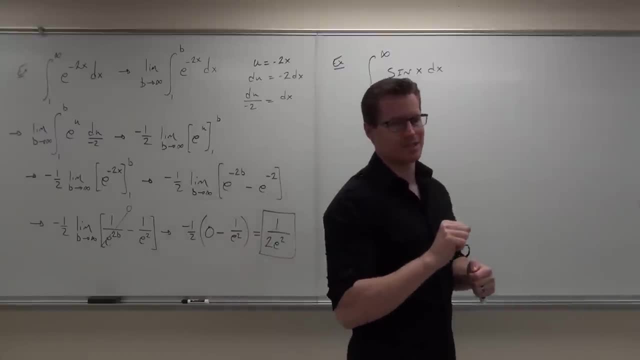 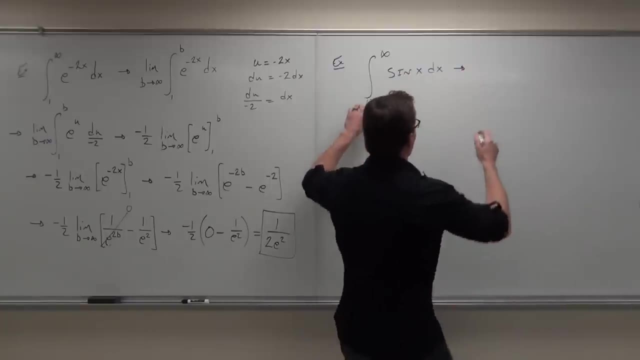 And in order to do that, we add this little thing in front of our integral What is it OK? so you should have done that already or be doing that right now. So we think about this and go: no, no, let's just start at zero. 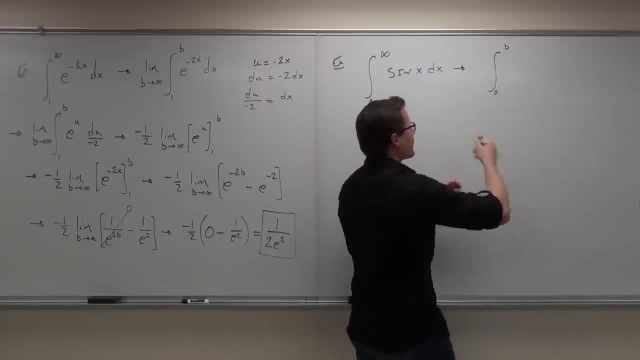 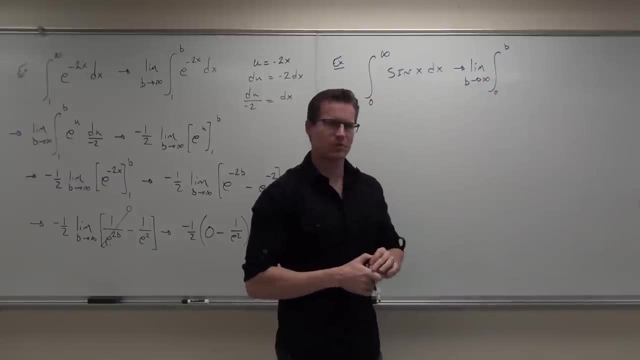 Because that's good. But let's go to some number just to the right of zero, And then let's take that number and push it to infinity after we've done the integral. So we're not really cheating, but we're kind of manipulating our integral properly. 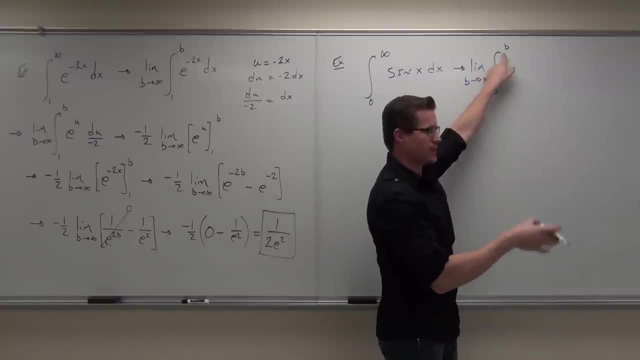 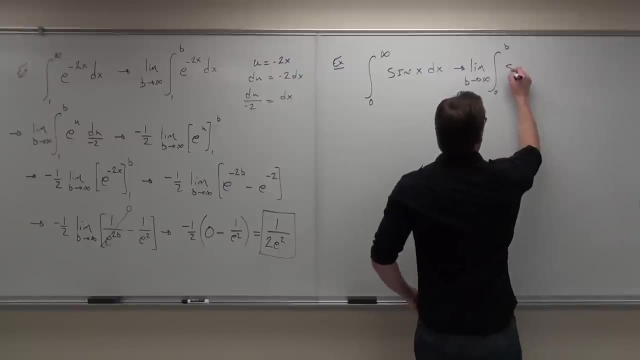 So we're saying, hey, let's go from zero to B. That way it's definite, It's a definite integral. This says now, at the very end, take your B and push it to infinity. That's the idea. Now I know that we've. 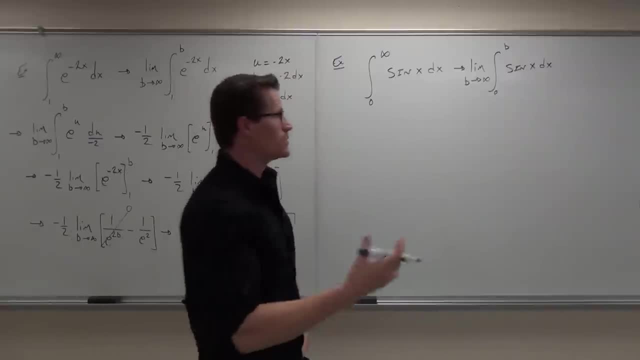 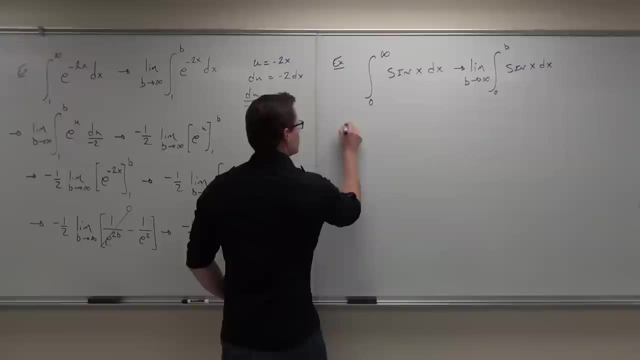 been doing some really difficult integrals, so don't make these harder than they actually are. Don't do anything fancy for the integral of sine x. What's the integral of sine x? Awesome, So we're going to have a limit as B approaches infinity. 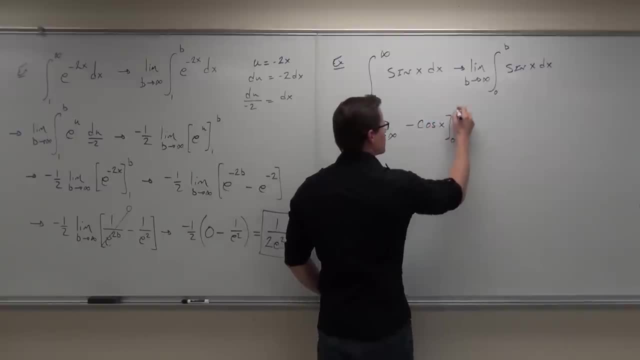 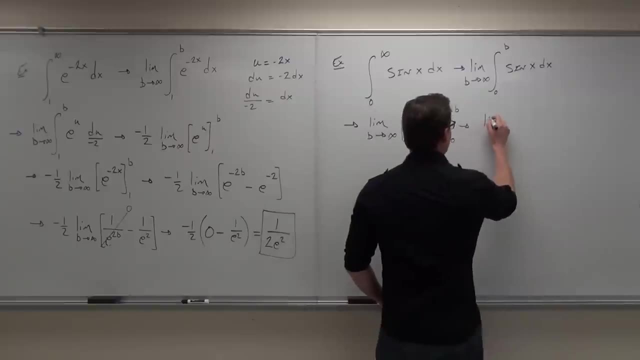 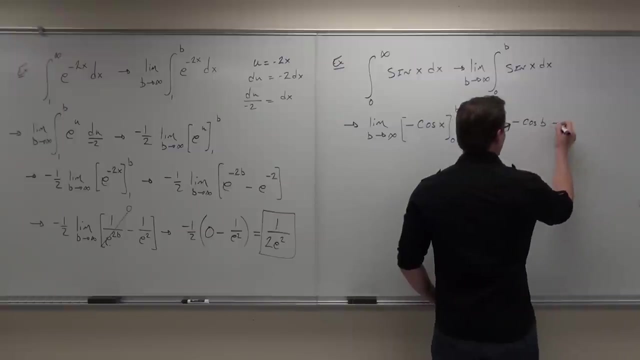 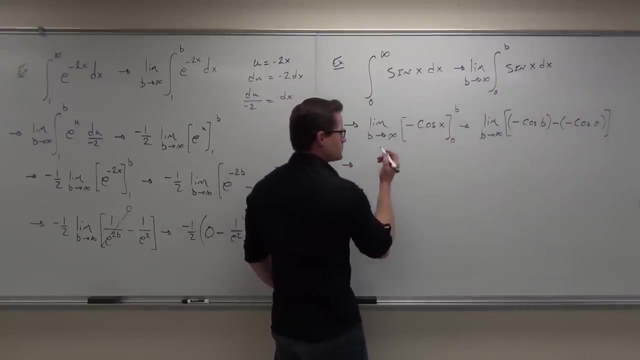 Negative cosine x from zero to B. Let's plug them in. We're going to have a limit as B approaches infinity. Negative cosine B: OK, minus negative cosine of zero. Let's see what we get out of this thing. So negative cosine B plus cosine zero. 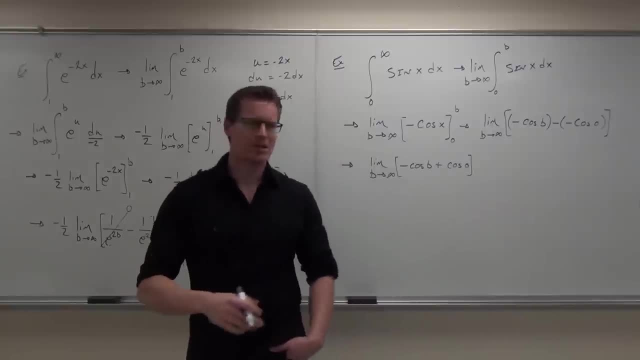 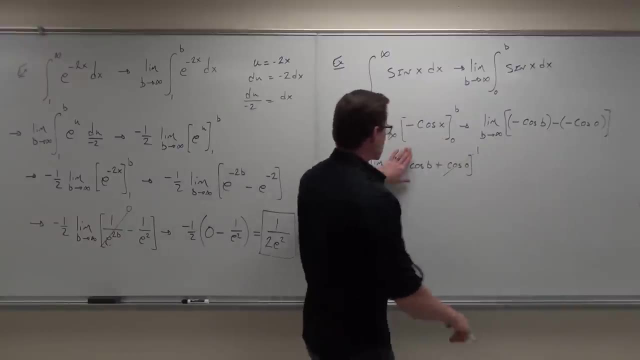 Let's start with the easy part. What's cosine zero? How much is that? So we know this is going to be equal to one. Now think about negative cosine B. Think about just cosine B. What is cosine B as B approaches infinity? 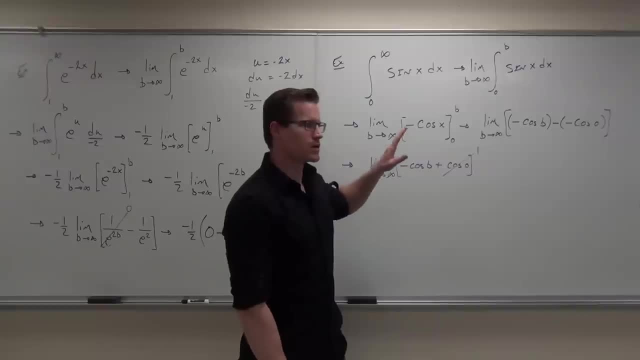 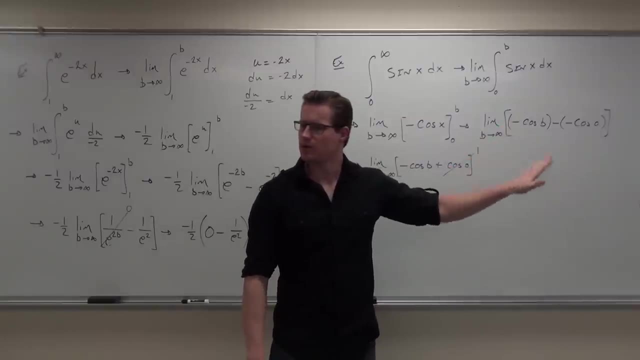 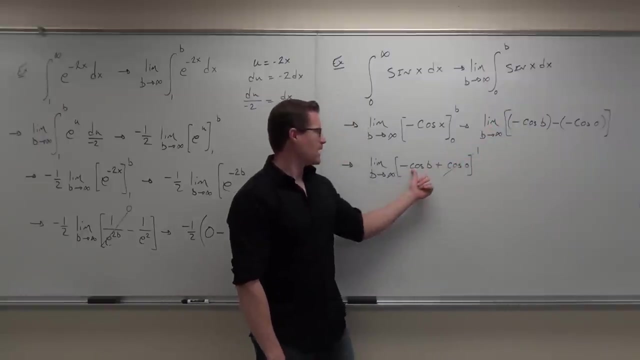 What is it Cosine, Cosine does, negative cosine, Negative cosine does? Does it ever go to a number? No, it's going to go up and down, down and up, Forever and ever and ever, correct? So my question is: as cosine- sorry, as B- approaches infinity? 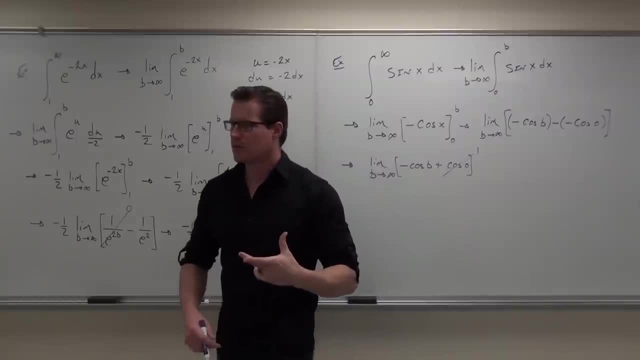 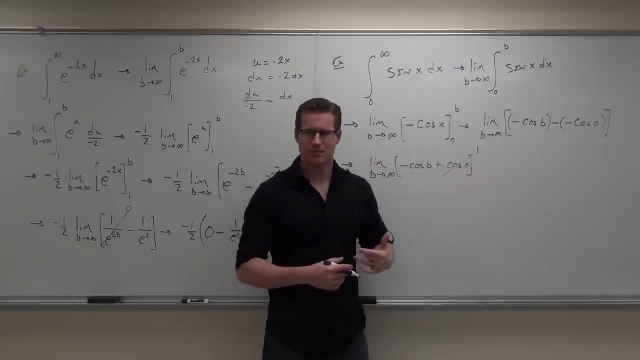 does cosine B ever go to a single number? It goes through lots of numbers. It goes from a range of negative one to one. So if it doesn't ever go to a number, does the limit exist? It's divergent. This limit doesn't exist because cosine does this forever. 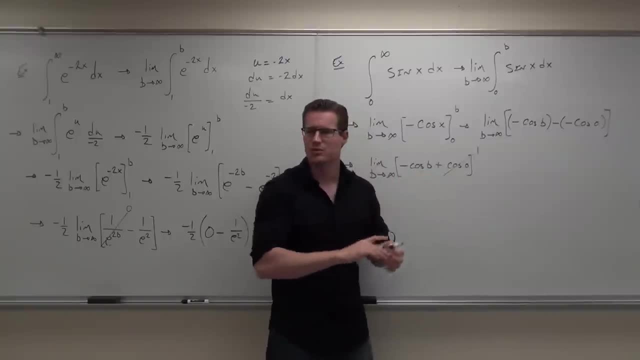 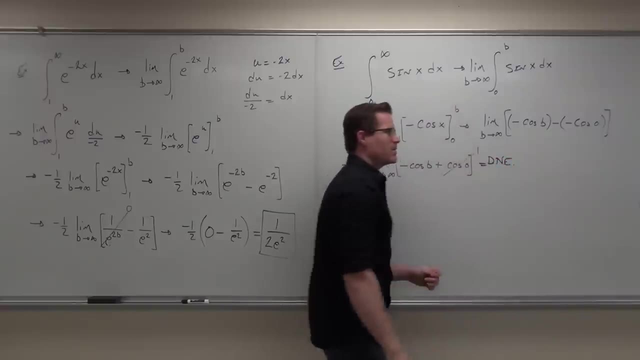 It doesn't ever go to one or negative one or some number between there. This is A DNE type of limit. If you get a limit that does not exist. what do we know about the area here? What do we know about that? 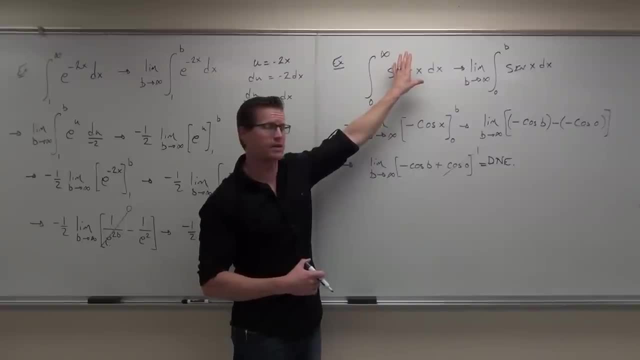 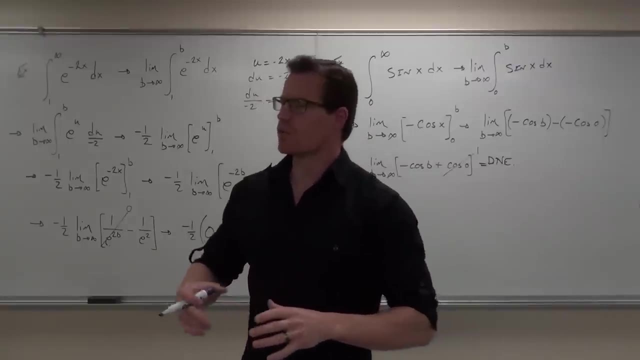 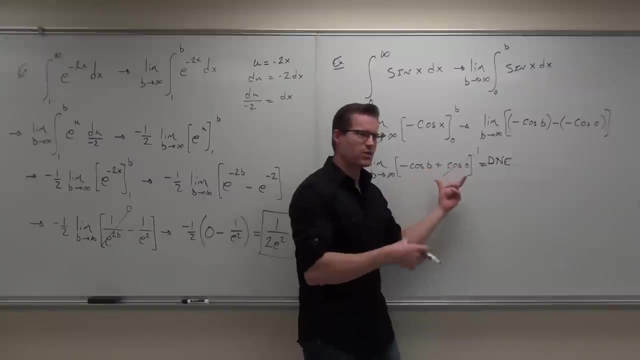 Is it going to be a convergent integral, where we can find an area, or a divergent integral where we can't find the area? So this is what I meant about those cases. So where we had convergent or divergent, If we have an integral that equals some function, that when we evaluate 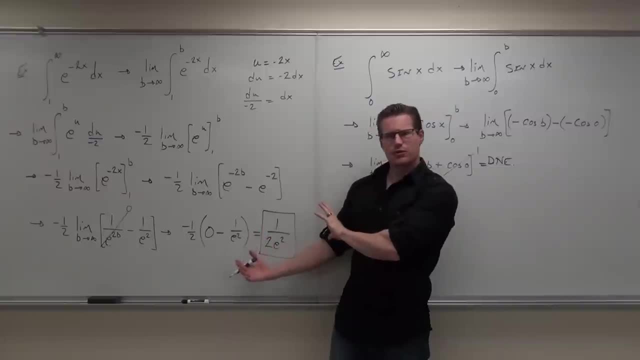 we get a single number, Like we did here, This would be convergent or divergent. So if the limit exists, it's actually equal to a valid number like this one. We have an integral that's convergent. Our improper integral would be convergent. 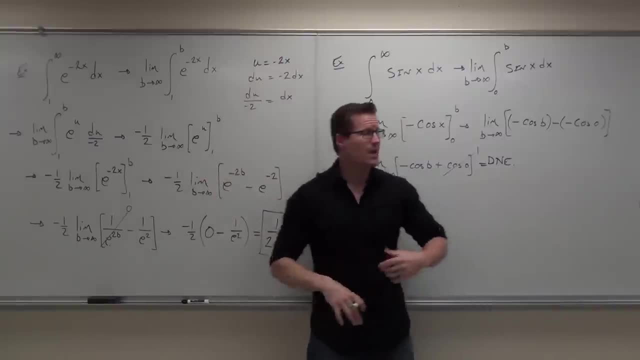 Convergent means the limit exists If you get an integral, so that when you evaluate with our limit here we get something that doesn't exist, like this one. It doesn't actually get to a number or something where we have infinity or negative infinity. 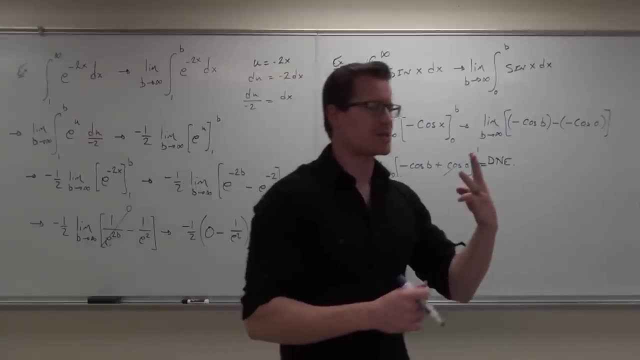 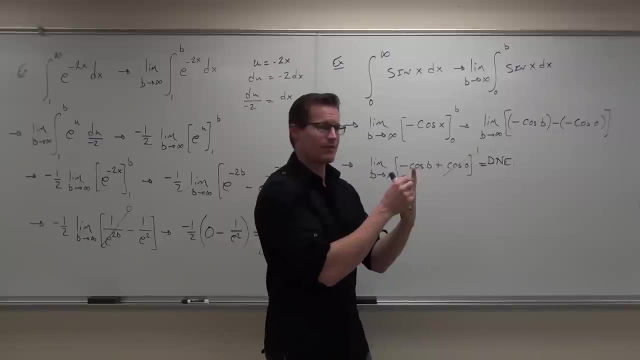 That's when we get this divergent. So there's basically three cases. The cases are: we get an actual number with our limit, We're good. That meant convergent. The other two cases are divergent, where we have a limit that does not exist. 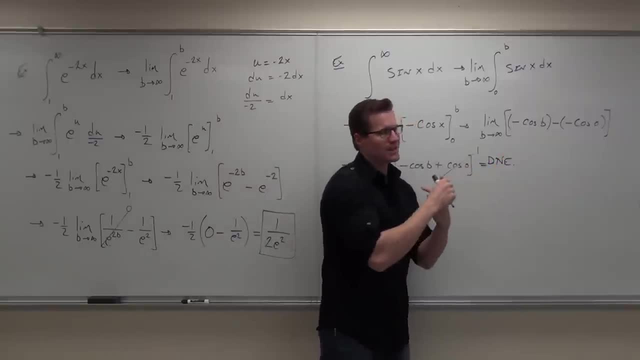 because it doesn't go to a single number, like cosine doesn't, or where we get an infinity or negative infinity. that limit It exists kind of, but it's not an actual number that we call convergent. It's just ever growing or ever decreasing. 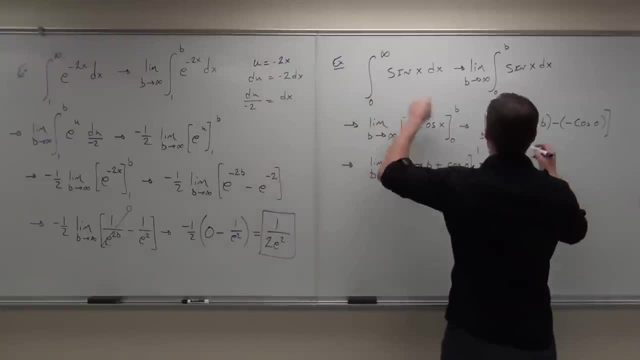 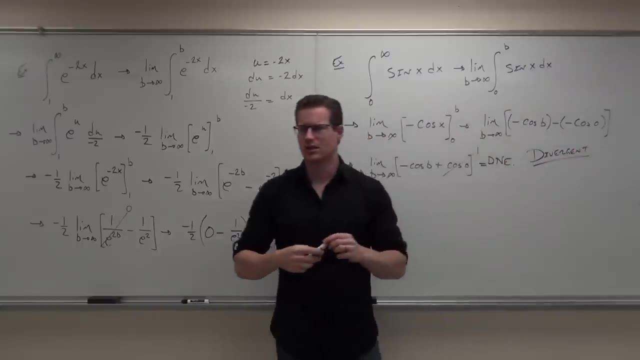 So if you look at the idea, OK, so here we say this integral is Divergent. You know, you might have guessed that just by looking at the function itself. Look at sine. Does sine ever go to a solid place? 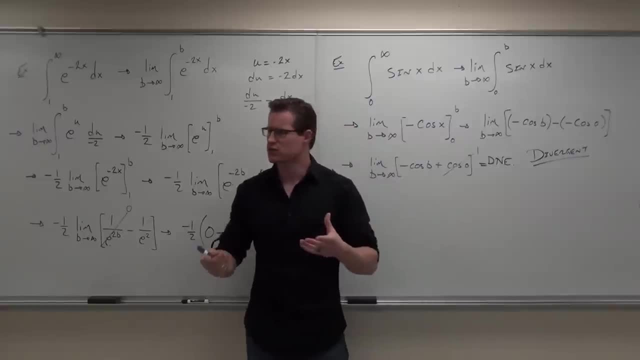 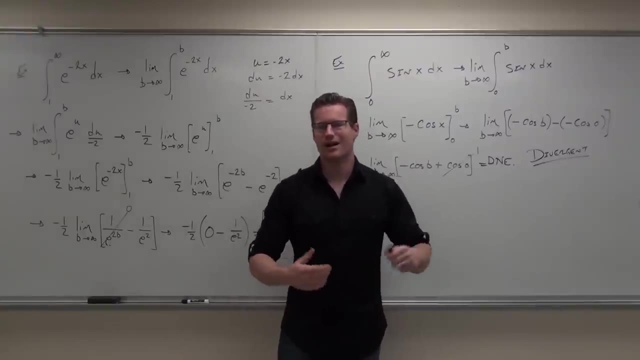 Really, it's always going back and forth. So if you thought about what integrals actually mean, integral means area under a curve. So if we're thinking about hey, you know what, I want you to find the area under the curve from zero to infinity of sine. 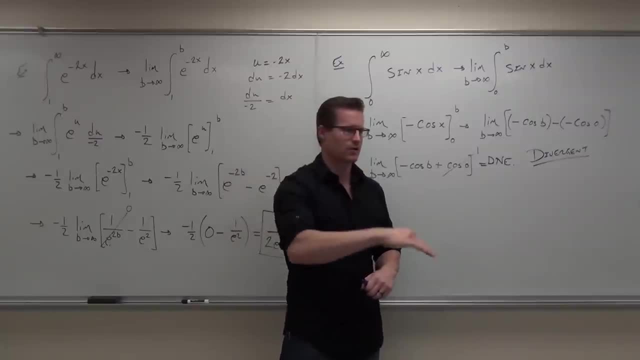 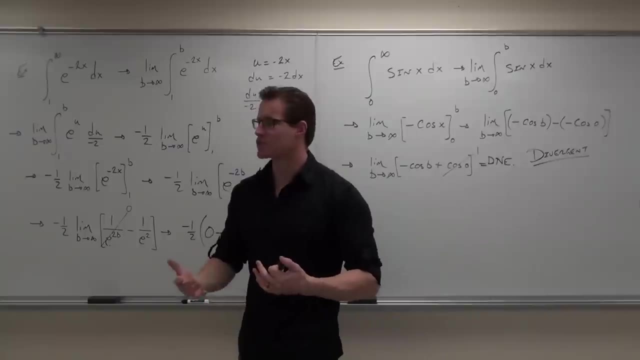 You're going: all right, well, there's going to be an area, then very little area, then more area, then very little. What's going to happen there? It's going to go forever like that. You're never, never going to be able to tell me how much the area actually is. 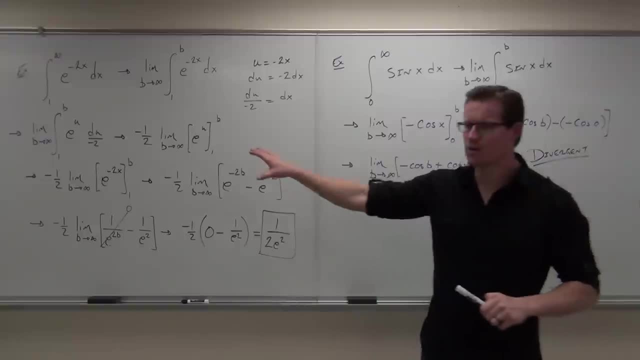 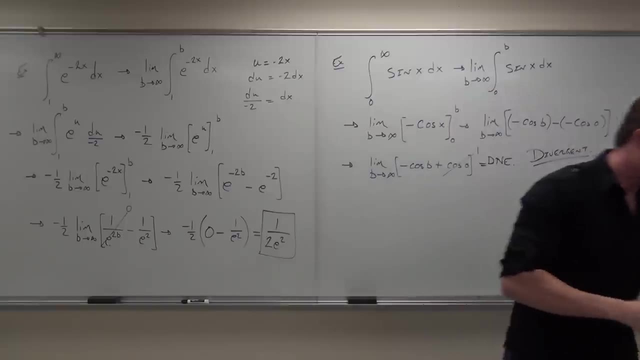 So far, so good. OK, cool. Have I explained these too long enough for you all to understand them? I'm going to ask you now, before I erase them, Any questions on these before we get going. OK, so it doesn't exist. 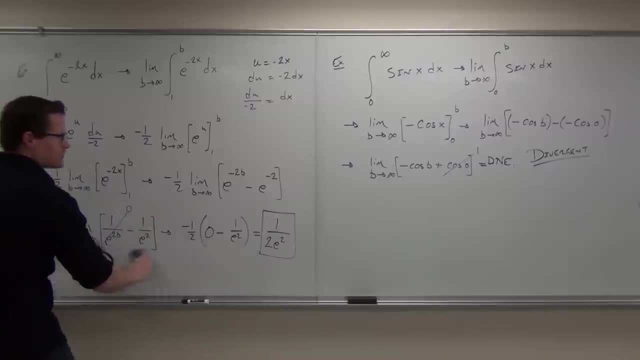 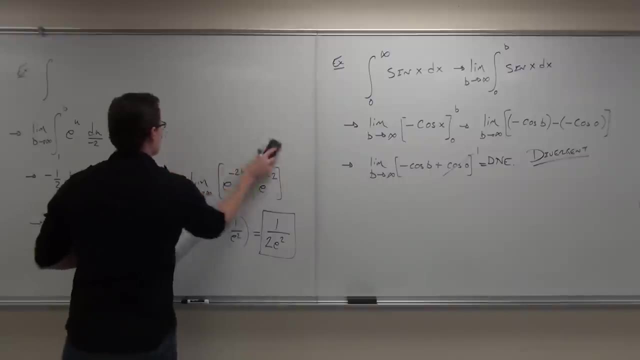 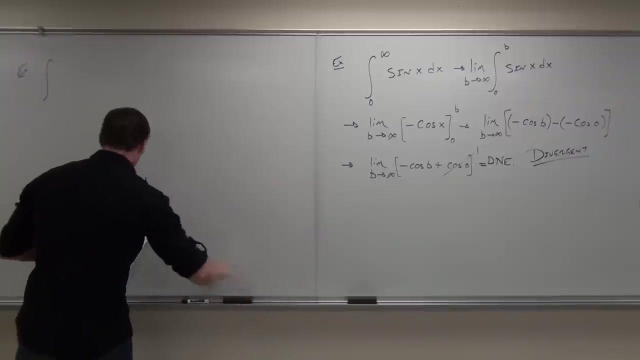 It's divergent. If the limit does exist, it's convergent. We're good to go. We can actually find the area. That's very cool. Let's continue. Can we ramp them up a little bit? These ones can get kind of boring if we do simple integrals all the time. 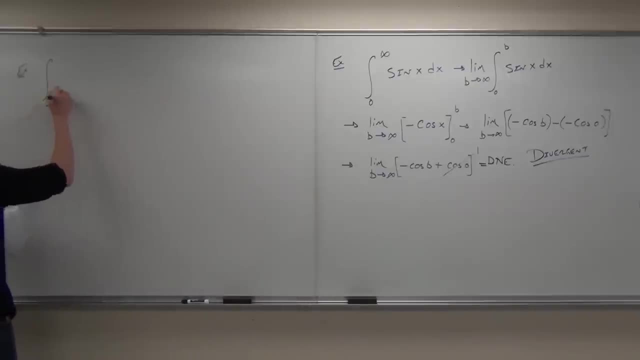 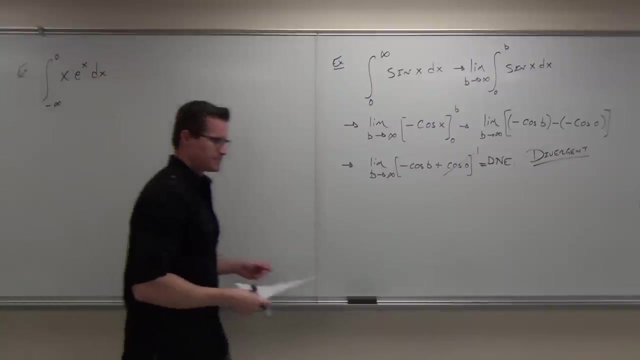 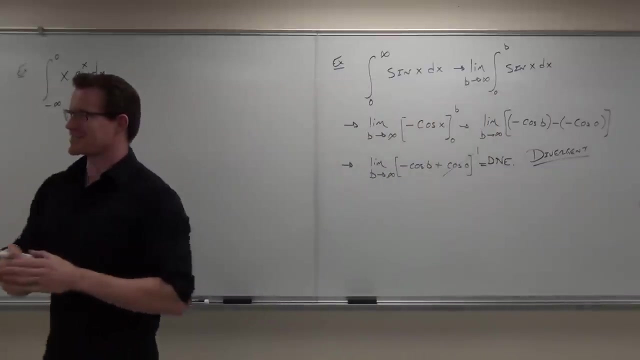 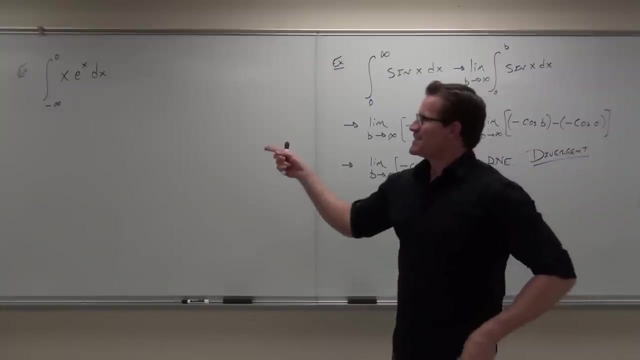 So let's see how this works with something a little bit funner. OK, first duty. First duty we got is to define what type of area left, Because I said duty, You guys watch too much Scrubs. Anyway, what was I saying? 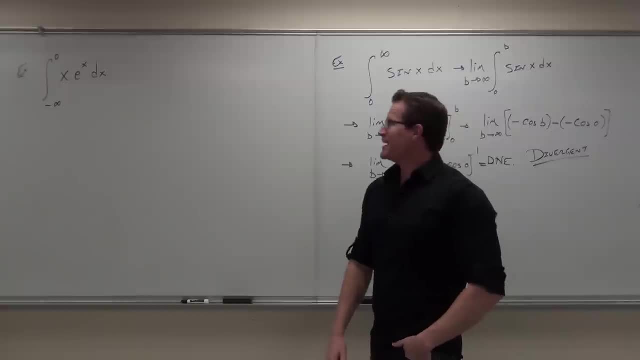 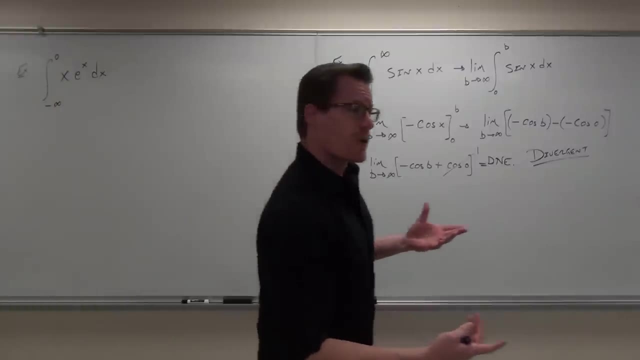 First duty. The first duty Should be the second duty. Anyway, first duty is to find what type of improper integral we actually have, Whether it's an infinite interval, whether it's an infinite discontinuity. Here this is all defined for the entire domain. 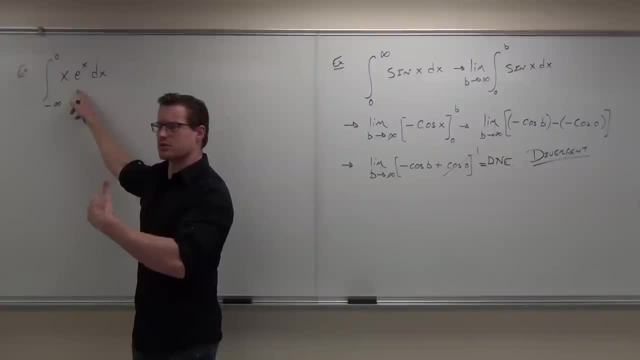 x times e to the x. we're good to go. We have no issues here. So it's not an infinite discontinuity. Those should be kind of obvious to us. when we get them You'll see them. What we do have is an infinite interval. 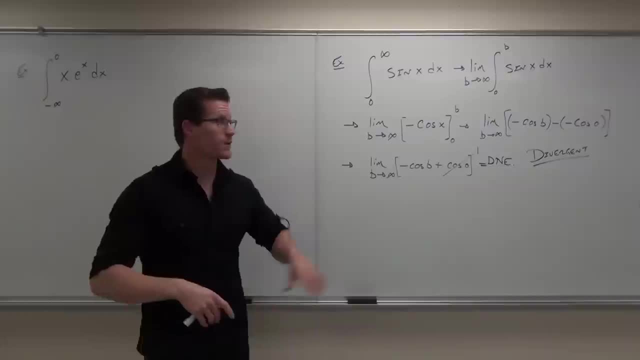 We actually start, though, at negative infinity. So we're going to do something very similar to this idea, Only I'm not going to be going from a number to v, I'm going to be going from. how would I write this? 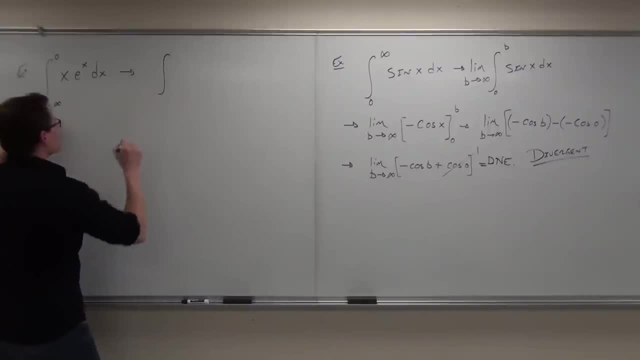 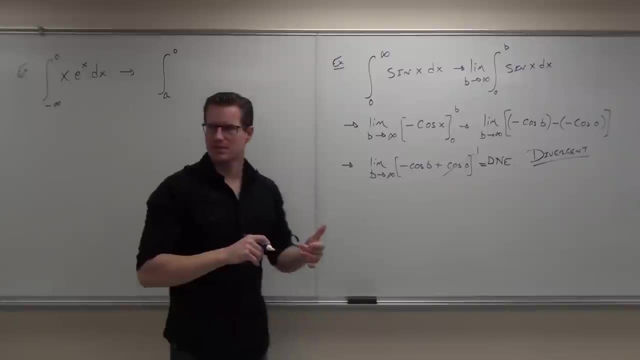 A OK. so because our lower bound is an infinity, I'm going to call that a Zero. I'm good with a zero. We're just going to go from a to zero. Does that make sense to you? No? Now, of course, we've got to define what we're actually doing here. 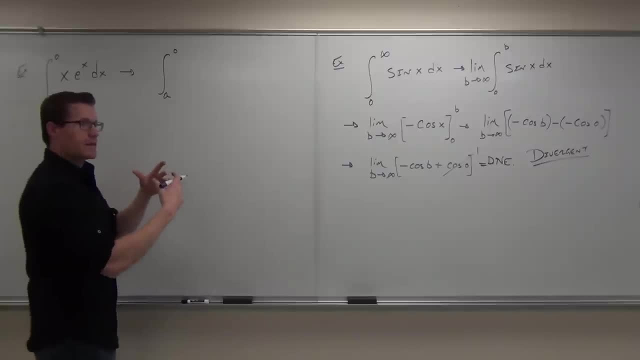 So I can't just go from a to zero and not define what a is doing. What's a doing? Approaching negative infinity? Good, Let's make sure we get that negative infinity in there, And that means the only way we can do that to let a approach negative infinity. 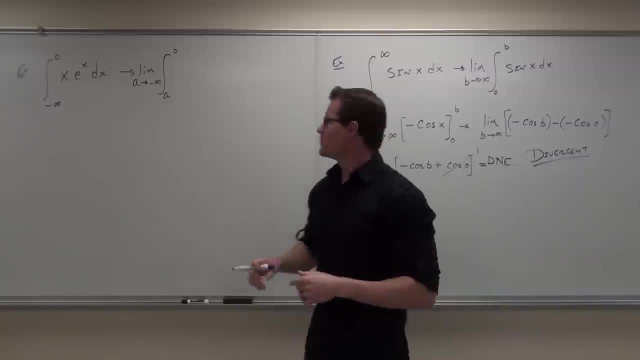 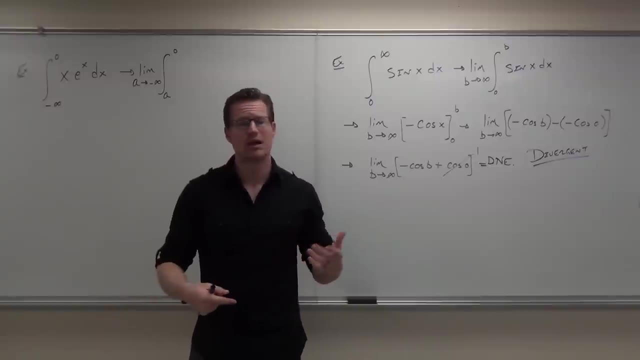 is with this idea of a limit. Quick head nod if you're OK with that one. So typically we call our upper bounds b's, We call our lower bounds a's, if they are positive infinity or negative infinity respectively. After that, what's really cool again? 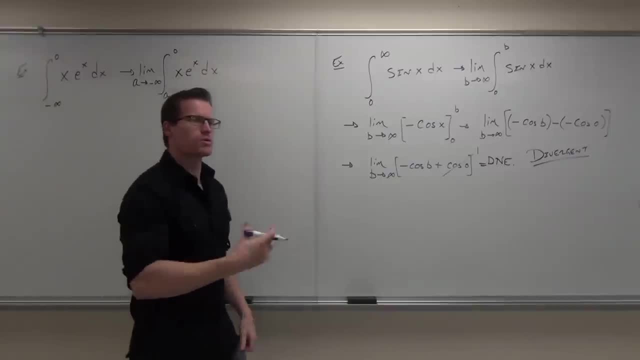 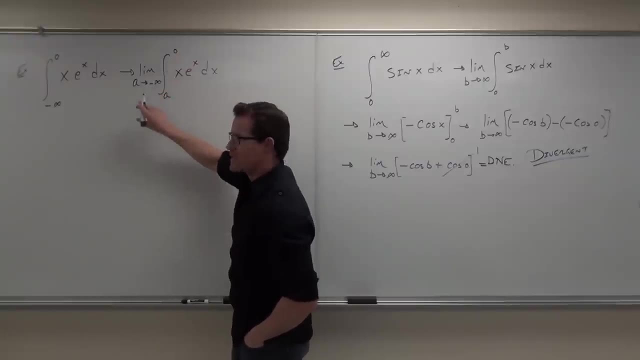 is that we know how to do all these integrals. So let's go through this integral. Right now is the time we go: OK, well, cool, We define what's happening here, We now have a definite integral, And then we're going to let a go to negative infinity. to take this idea of negative infinity to zero. 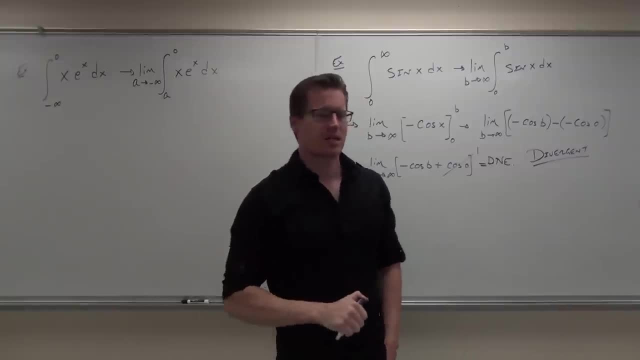 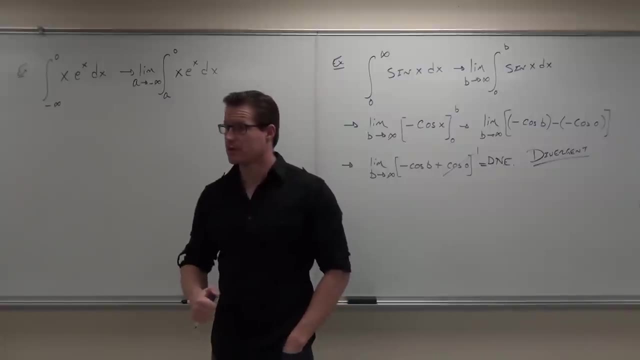 But we just got to worry about this right now. So the integral of x e to the x dx. Let's go through what we know. Does it fit the integration table? No. Can you do a substitution with it? No, Could you do a substitution if I did this? 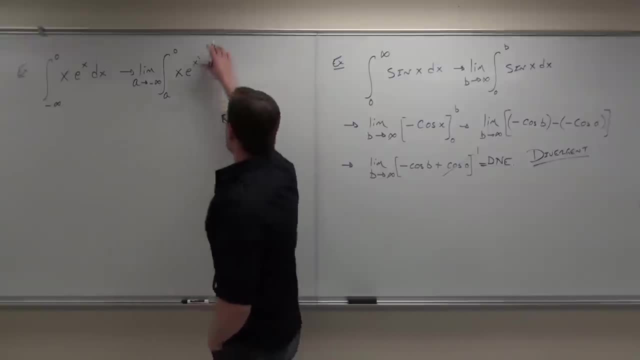 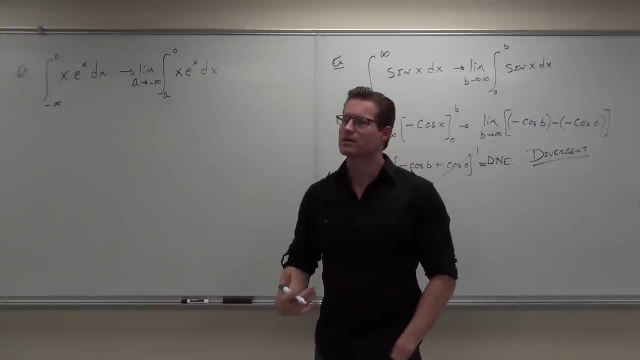 Yeah, That would be nice. So that's what we would do in this case. If I don't have that, then no, we can't do a substitution. Can you do integration by parts? Yes, you can, It's a product. 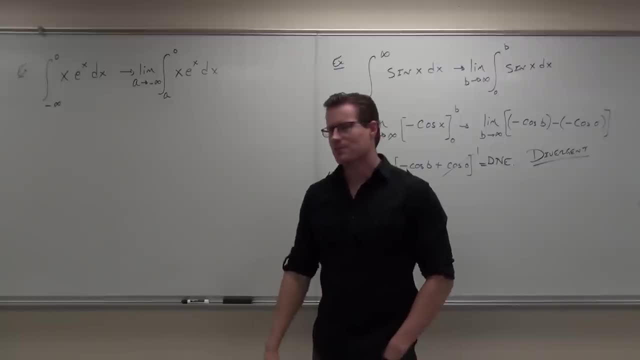 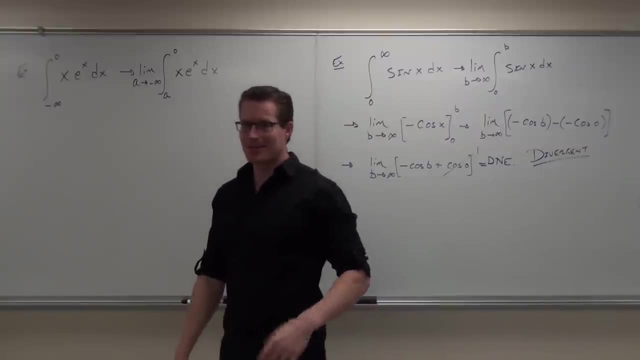 We can do integration by parts with it. So let's do integration by parts. What would you pick? What would you pick for? Do you remember how to do integration by parts? It's been a while, So this is one of those things that you should kind of do from time to time on your own. 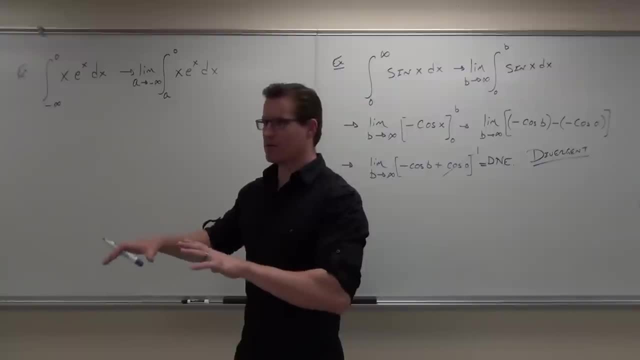 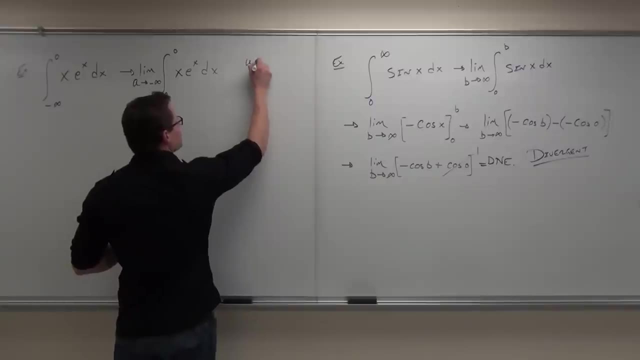 whether I give you homework or not, because we haven't really covered that in a long, long time, Right, But it is part of this chapter. So what would you pick E to the x? Yeah, u is x. Remember how to pick u. 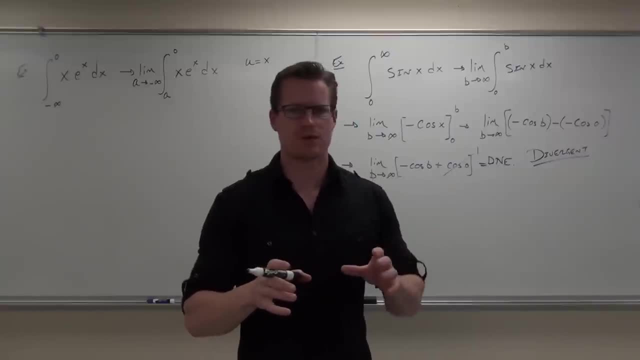 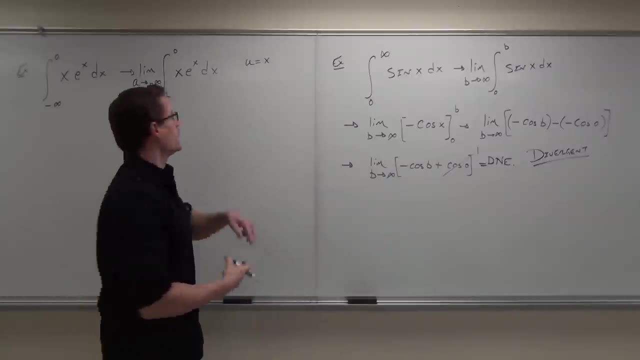 You want to pick u and v this way. You want to pick so that you can do the integral of what's left over very easily, or that the derivative of u becomes easier. So here I'd say, hey, can you do the integral of x? 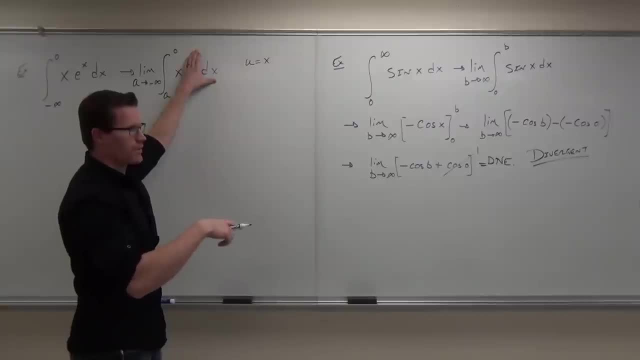 I can, but it gets worse. It gets x squared over 2.. I don't want that. Can you do? the integral of e to the x, Uh-huh. And the integral of e to the x is E to the x. 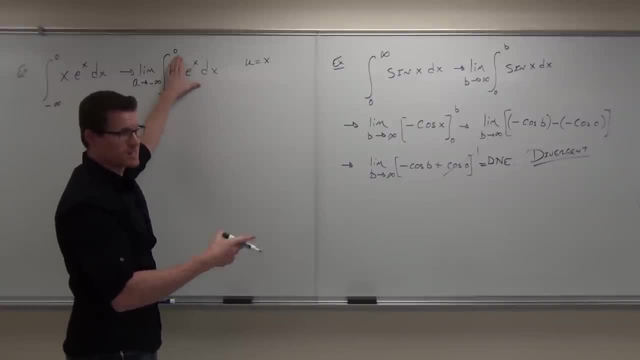 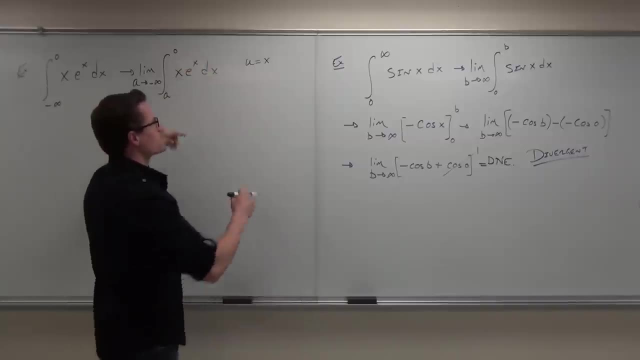 Okay, that's nice. Can you do the derivative of e to the x? Yes, That's e to the x. It doesn't get nicer. Can you do the derivative of x? One, That's one that's nicer. So our appropriate choice here is u equals x and then v equals. 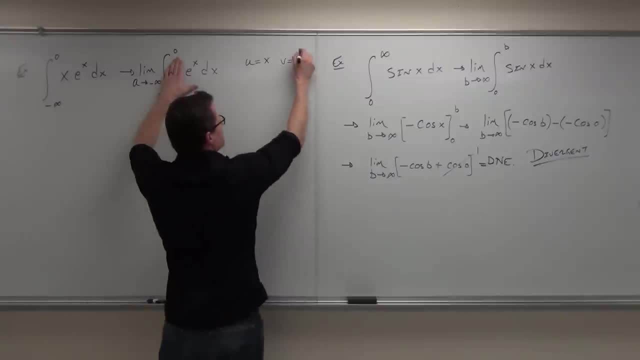 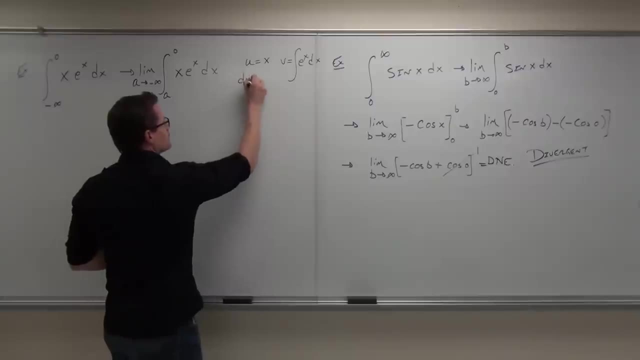 we always teach this. I say, hey, cover up your u. v is the integral of whatever's left over. So du equals dx, v equals e to the x, because that's really nice. And then do you remember the formula for doing integration by parts? 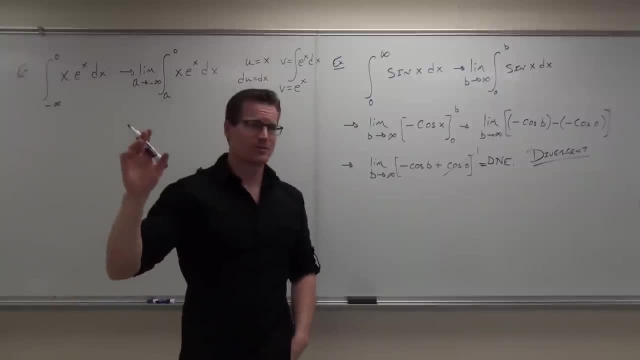 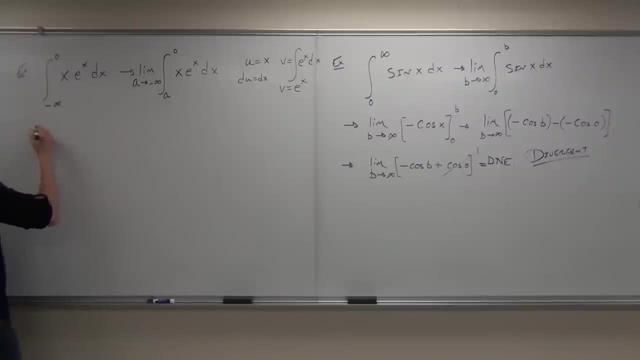 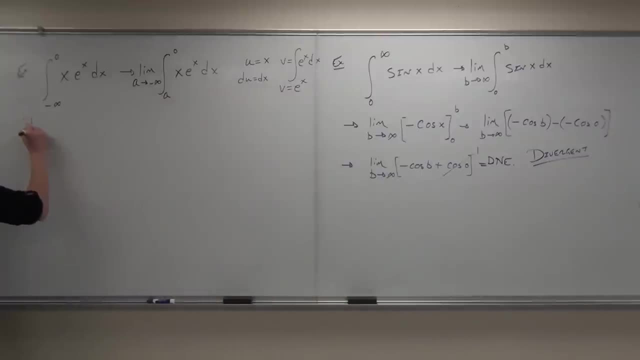 because that's really still what we're doing. Okay, so we've got a limit, We've got a approaches negative infinity. That's right Now. in this limit, we don't have the integral anymore. We have, well, our integration by parts says we do a? u times v. 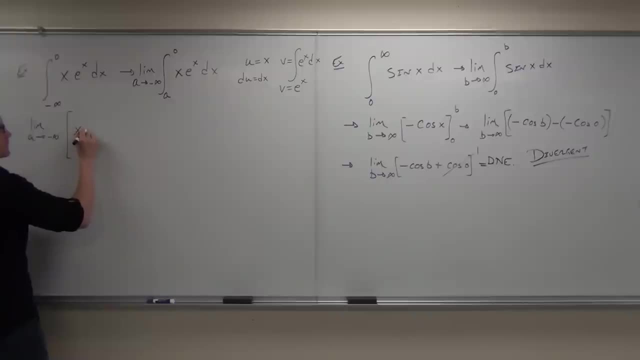 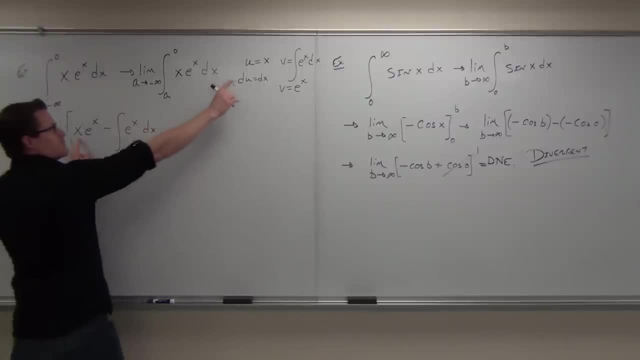 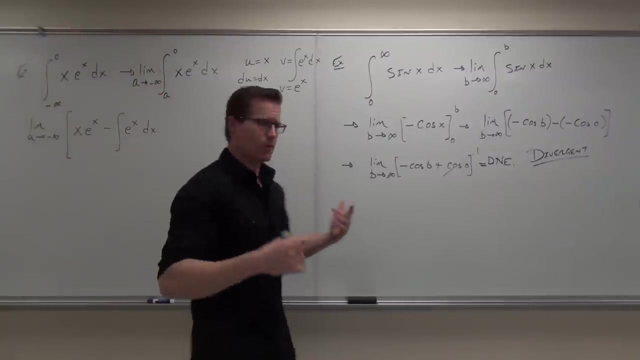 v, dx, v, dx, Good, So u times v Minus the integral of v, du. But du is dx, So we have integral of v, and then du is our dx. Chopin should be okay with that one, By the way. for those of you who are thinking: well, what about our bounds here? 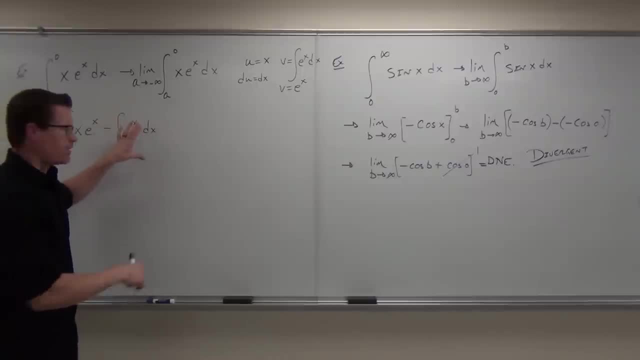 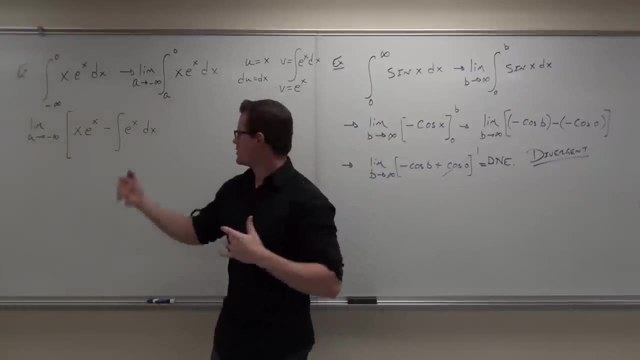 Don't worry about it. You're going to evaluate later. Don't evaluate this integral right now. Wait until you do it. Then evaluate the entire thing from a to 0.. Does that make sense to you? If you try to do it here, it just makes it too hard. 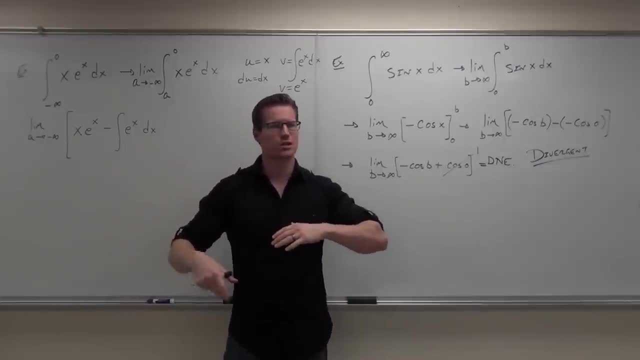 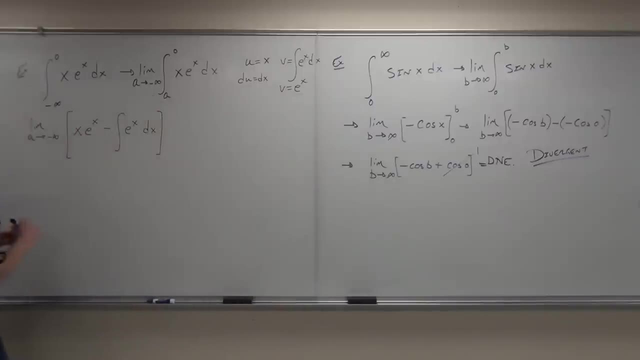 Okay, so wait, Wait on it for a second, to the very end, until your integral is actually done. You got that, Otherwise you're really working overboard. So I am going to put this here. I'm going to put the a to 0, so I don't forget about it. 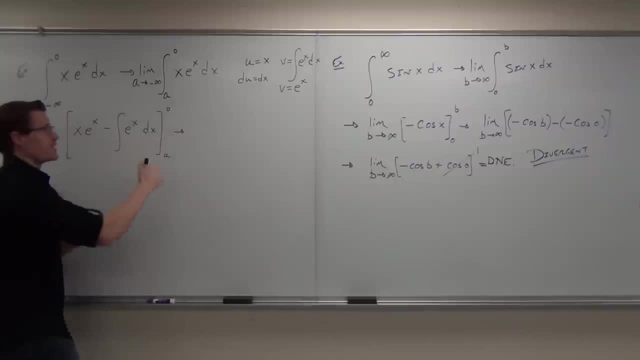 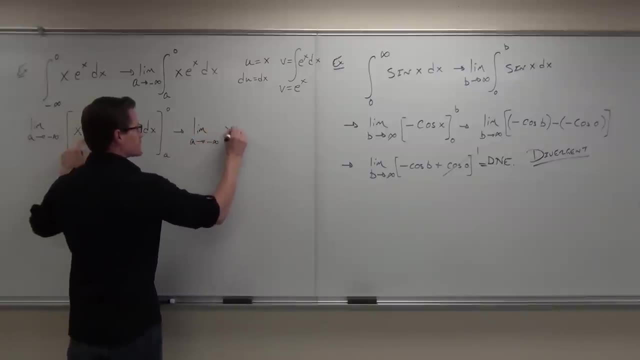 But I know I have one more step in here to do before I actually evaluate that. So I'm going to have a limit As a approaches negative infinity. I have x. I've got e to the x. This is why integration by parts works. so nice for this. 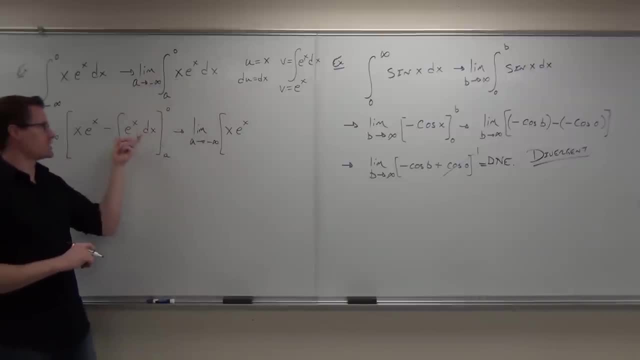 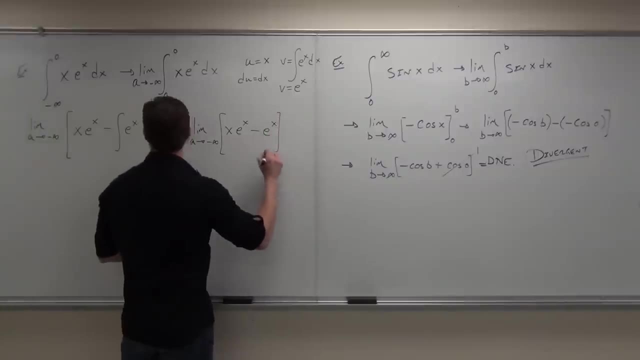 We reduce the power of our x by 1 degree. If we've done that, that means the rest of this integral is really nice for us. What is the rest of that integral for us, Minus what? From a to 0.. 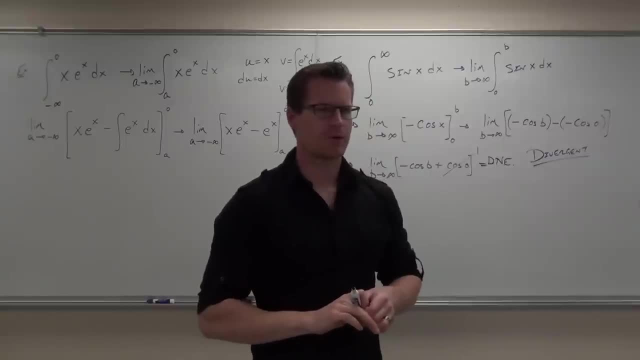 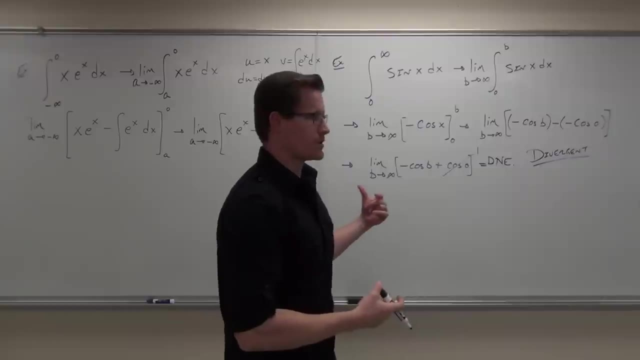 What are we going to do now? What do you think We could simplify? We could factor. if you want to Sure, you could factor this. You could do it right now if you want to. It doesn't really matter to me how you do this. 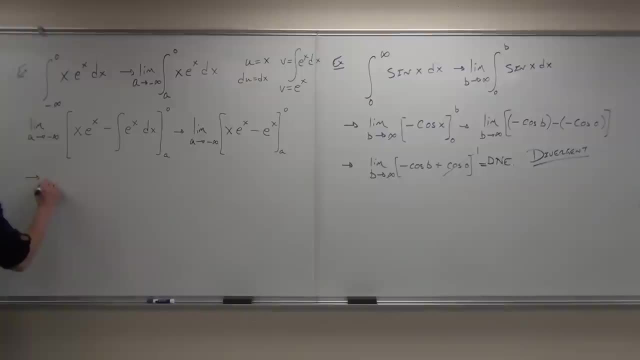 If we do decide to factor this- since you guys said that we'll have a limit, As a goes to negative infinity- of what e to the x times 1. x minus 1. Perfect, OK, well, now let's go ahead and evaluate that. 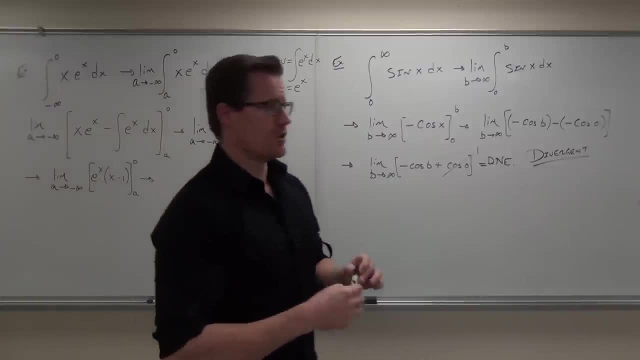 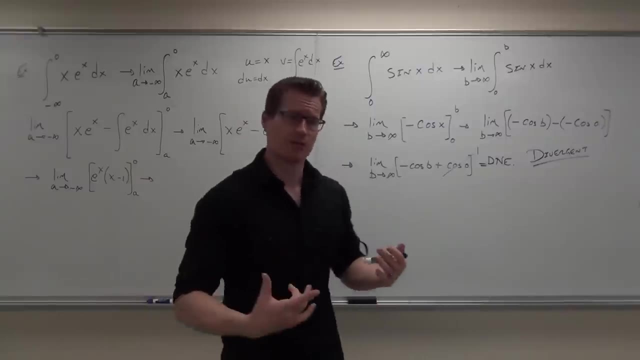 So what we've done so far is the first thing we do. we identify that we actually have an improper integral. We find out the type, whether it's the infinite discontinuity- we haven't even talked about this yet- or an infinite interval. 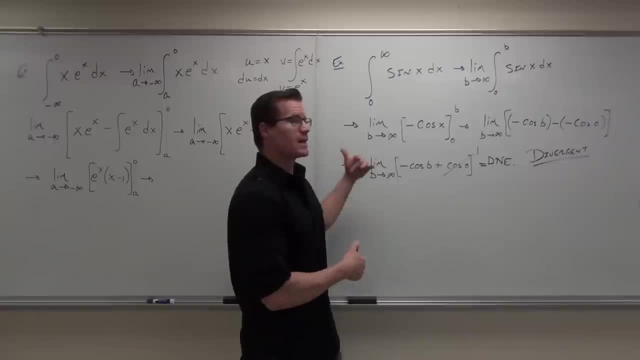 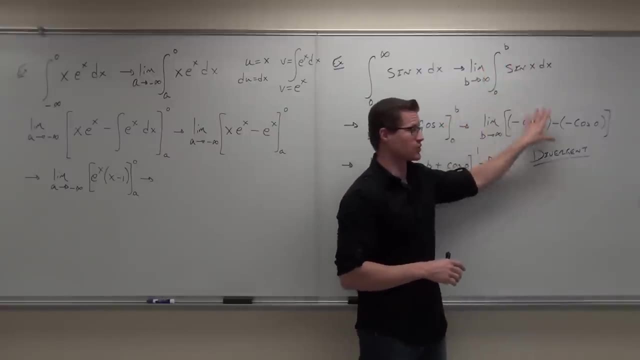 If it's an infinite interval, no problem. When we know how to do that, let's just take a limit And instead of the infinity, we'll make it definite, for, like the right now, It's a definite integral. right now, That means that we can actually do it. 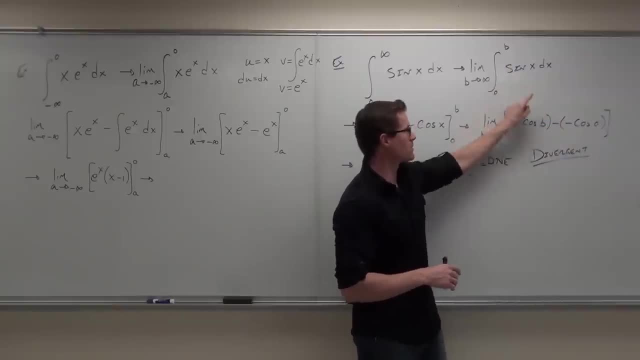 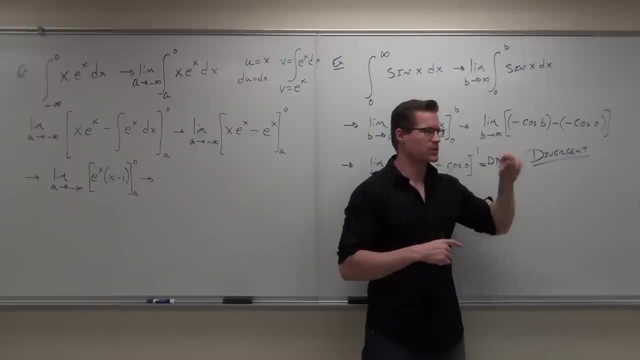 OK, by the fundamental theorem of calculus this actually works. So we do this, so that this is actually possible. Then we realize, oh, but you know what? B wasn't actually definite. B was this number that we want to now move to infinity. 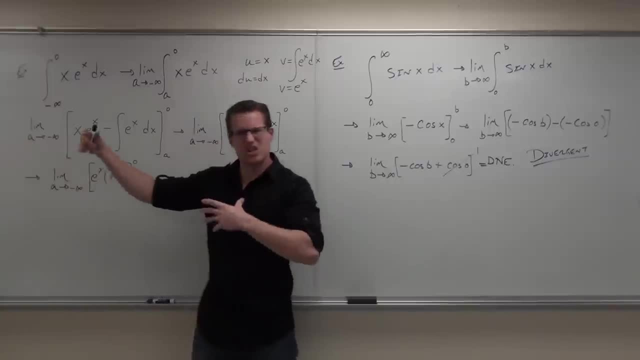 Or A was this number that now we want to move to negative infinity. So we're cheating a little bit. We're calling this a definite integral when we know it's not. but it uses the fundamental theorem of calculus to actually do the definite integral and then says: now use the limit idea. 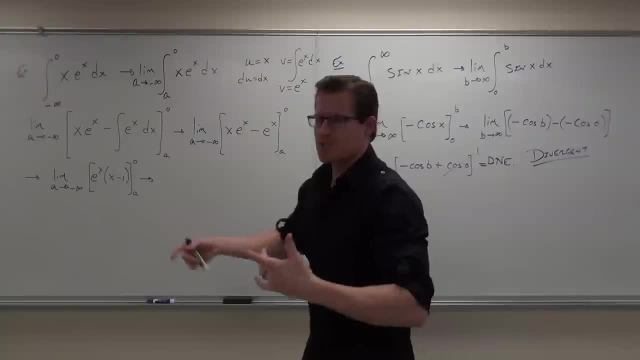 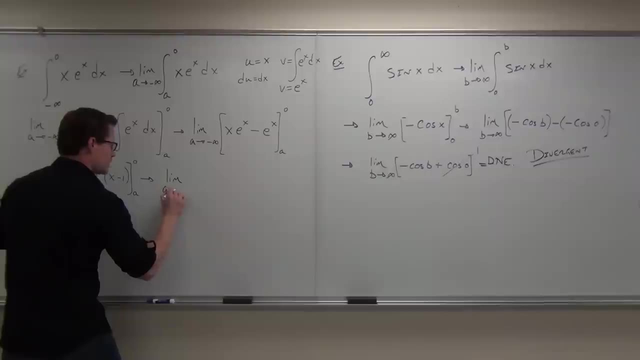 Now move that number to infinity or negative infinity. Hey, just evaluate the limit. So when we do, we're going to evaluate the integral but then evaluate the limit. So A is going to eventually go to negative infinity. We got to plug it in first and see what happens. 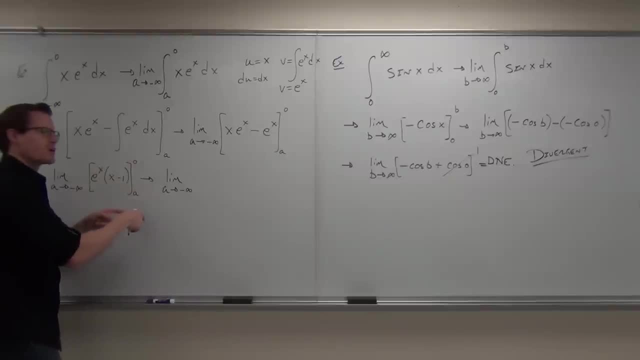 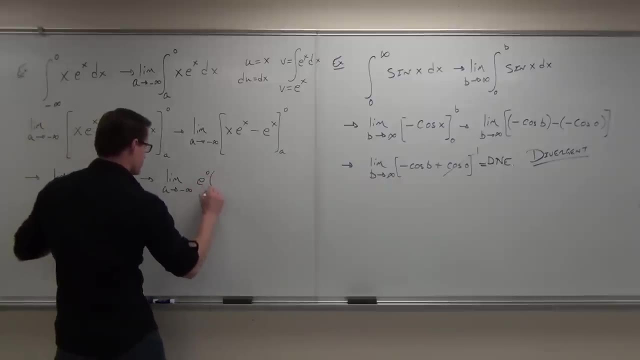 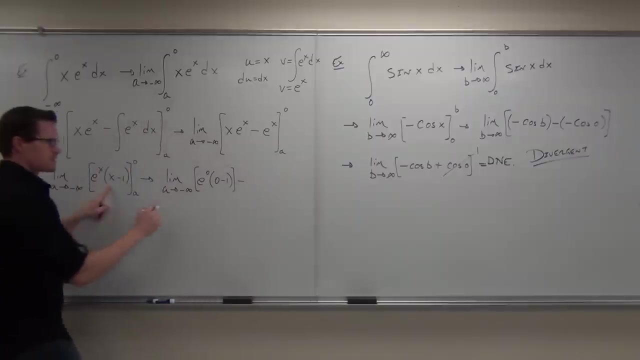 Which number do you plug in first? Make sure you do that. OK, make sure you follow the rules for evaluating your integrals here. So we have E to the zero Times zero minus one Minus E to the A times A minus one. 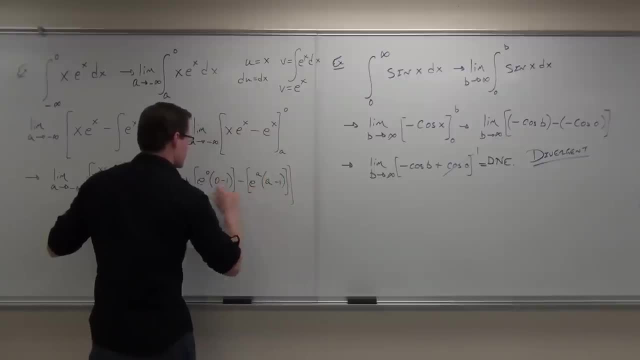 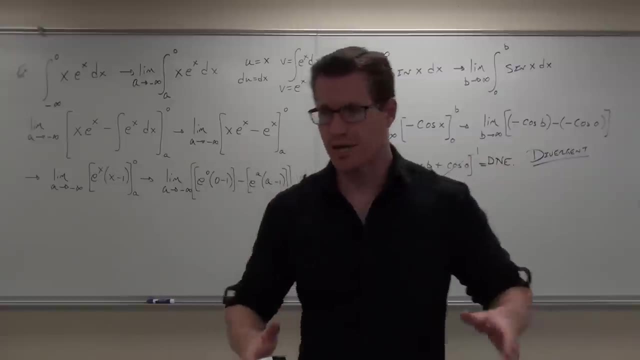 OK, let's simplify some stuff here right now, because there's I have no idea what's going on with this. I just got to. I got to simplify this because right now it's a little bit too confusing for me. Do you guys see what I'm talking about? 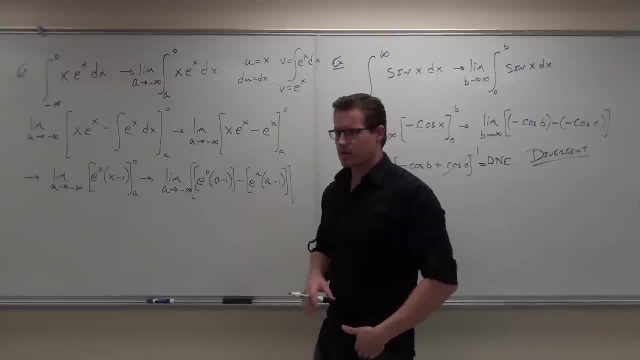 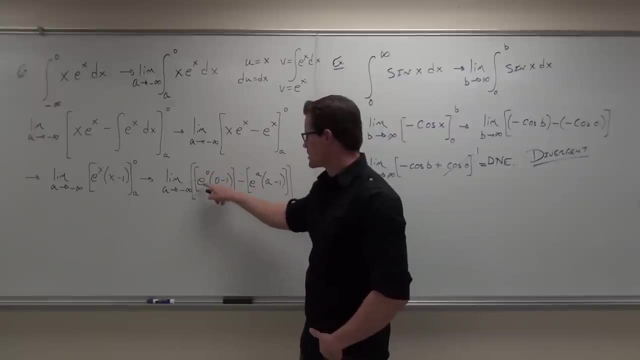 A little bit too much going on. So what can we do with this thing? E to the zero is how much One Good? Zero minus one is One. So this whole piece is one times negative one. This thing goes to negative one. 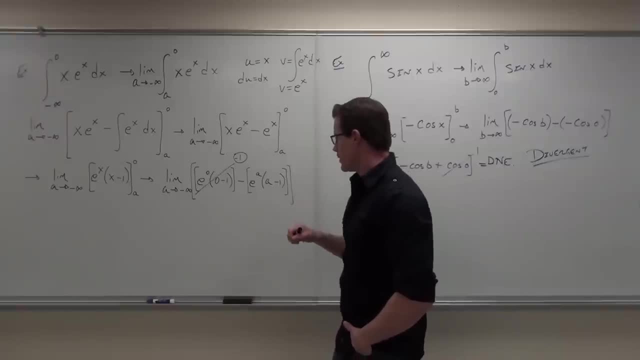 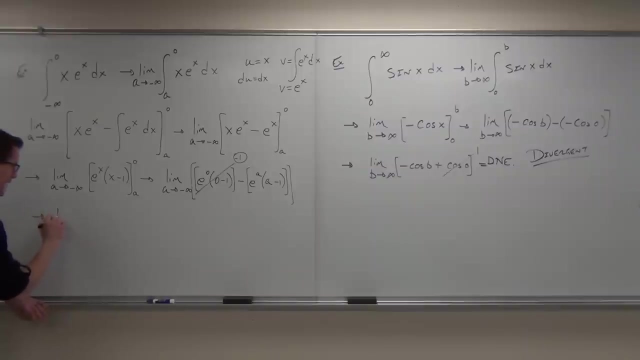 Very good. Also, I'll tell you right now what's going to have to happen here, because I have infinity and infinity. I'm probably going to want to distribute this real quick, So it might have been nice if we hadn't have factored that. 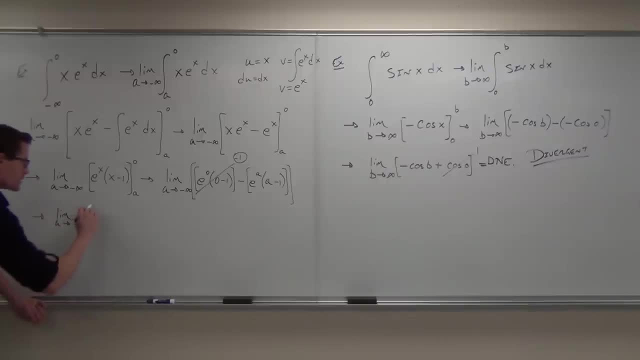 but you know what? Not a big deal. We can take care of it right now. So in our limit we've got negative one. We're going to have minus A times E to the A and then plus E to the A. Can you check my work? 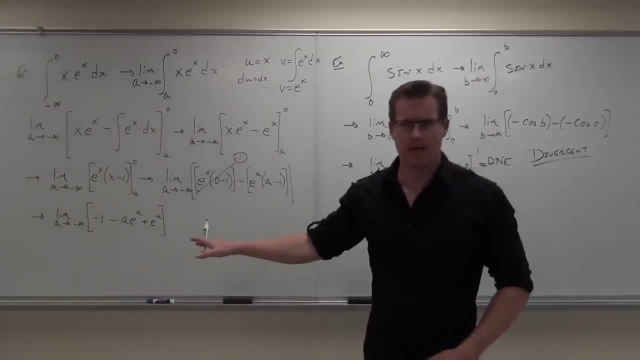 I want to make sure that my algebra is correct too. Can you check that to see that I'm OK on that one? Are we OK with that? So I've distributed this. So this is A E to the A minus E to the A. 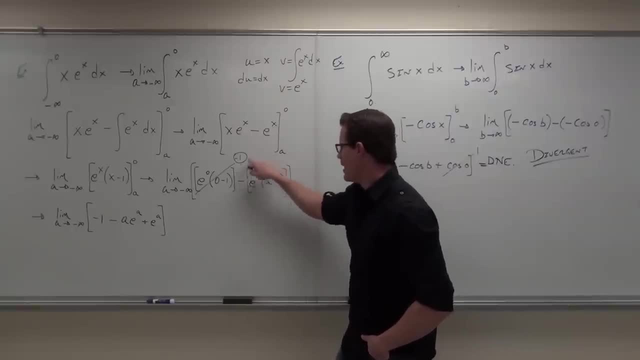 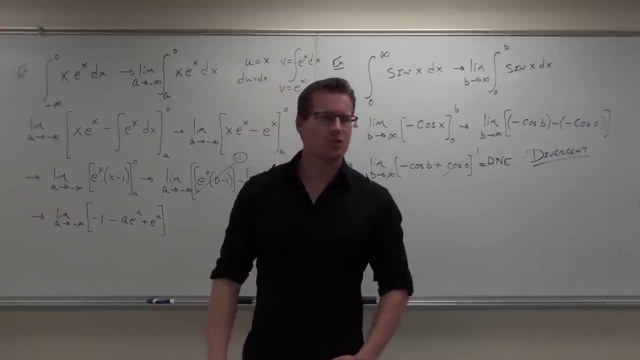 but then my negative changes the sign. So minus A E to the A and plus E to the A. So I'm OK with that so far. Now let's think about what's going on here. Do not neglect your knowledge of limits from your chapter six step that we've done. 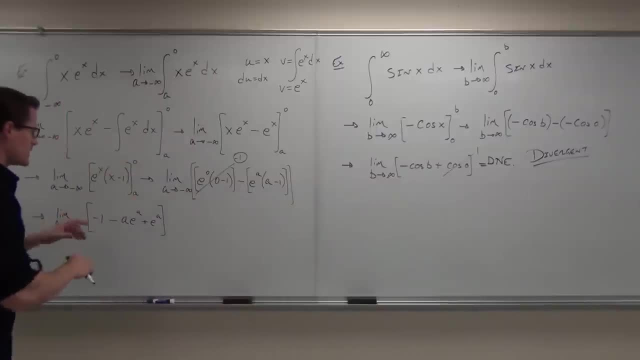 You've got to really follow that. So, if we look at this part of this is really easy. So check out the negative one. What's that going to go to? That's easy. Check out the E to the A. Oh, let's think about this. 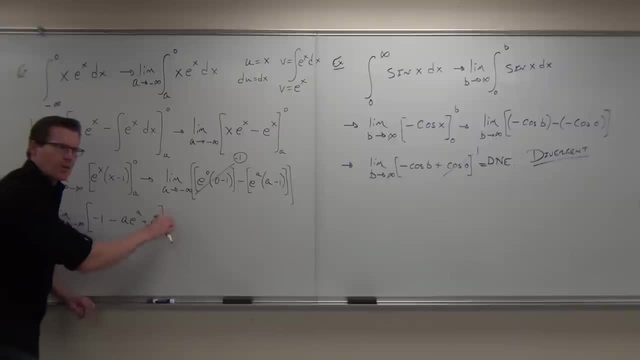 E to the A when A approaches negative infinity. So, basically, what's E to the negative infinity? Zero, It's zero, That's right. So this is one negative one. This is zero. That's fantastic. Now please listen carefully. 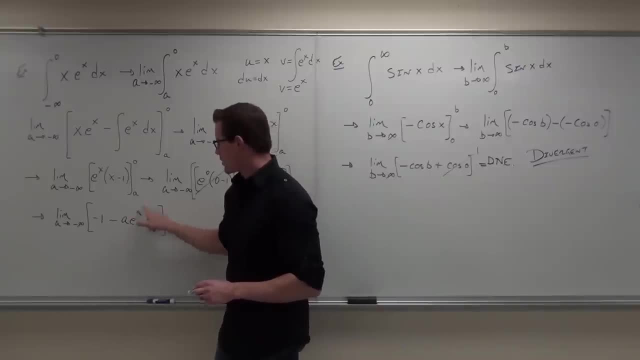 This is A times E to the A, correct? We already know that this part is zero. E to the negative infinity is zero, But this is negative infinity. So we have an infinity times zero. That's an indeterminate. Remember that. 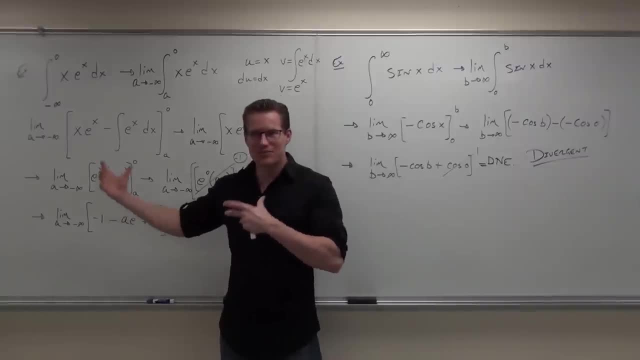 Oh it's coming back. This is exciting. It's an indeterminate. Look at how much stuff is involved in this. Had you not done indeterminate forms, you couldn't do this problem. Had you not done integration by parts, you couldn't do this problem. 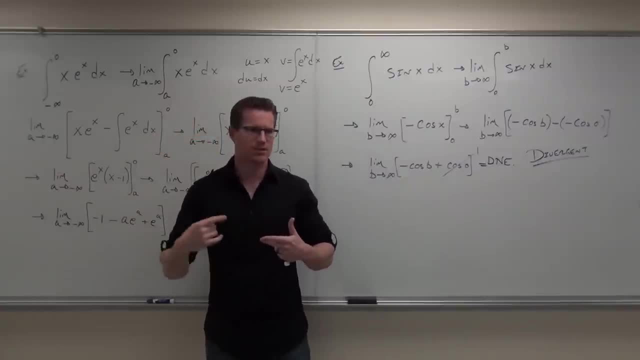 And now we have a proper integral. So we've got lots going on in this stuff. This is why this calculus builds so nicely for us. But you've got to remember it All right. So it's not like other classes where you can forget a section and you're probably OK. 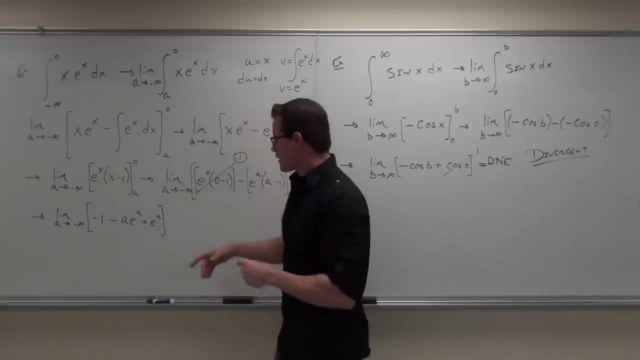 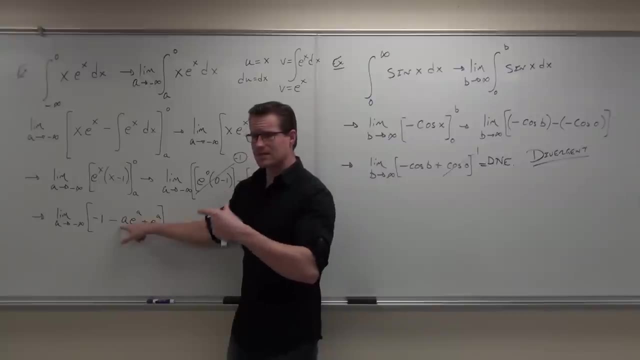 You need everything to do these problems sometimes. So for us we go all right. well, cool, This is easy Negative one, This is easy Zero. But this one, well, that's an infinity times zero type of indeterminate form. 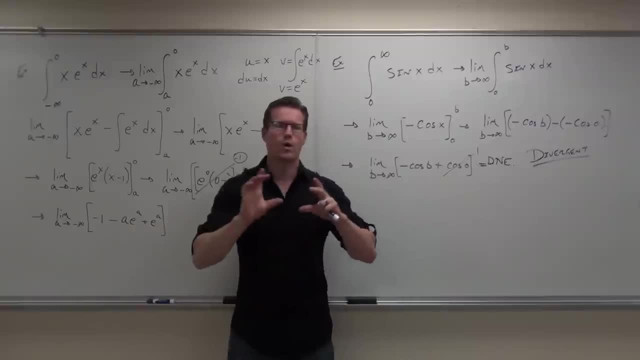 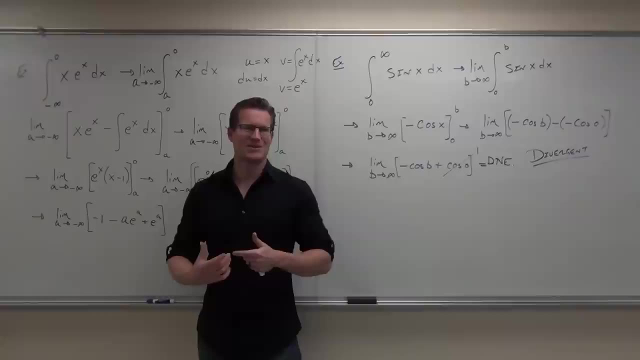 What that means is, when we have an infinity times zero, we've got to rewrite one of those in order to get an infinity over infinity or a zero over zero. In either case, we can use L'Hopital- Remember L'Hopital. 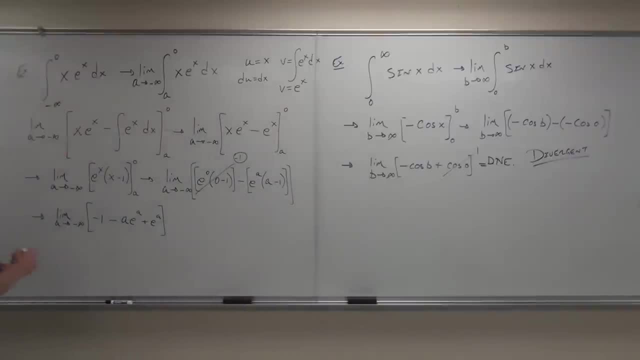 Favorite word in limits: L'Hopital. So I'm going to do something here. I'm going to separate these. What I know is that this is cool, This is negative one, This is also zero, So I'm going to do this. 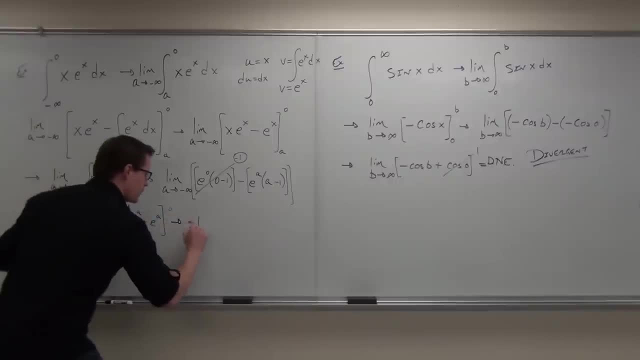 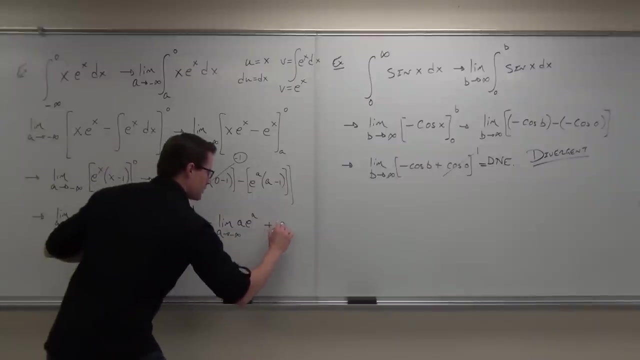 I'm going to separate these limits. I know I'm going to have negative one. I'm going to have minus the limit A times e to the a as a approaches negative infinity plus zero. So basically, I just want to focus on this guy. 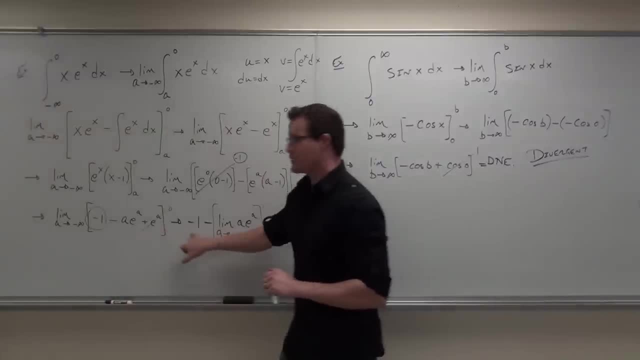 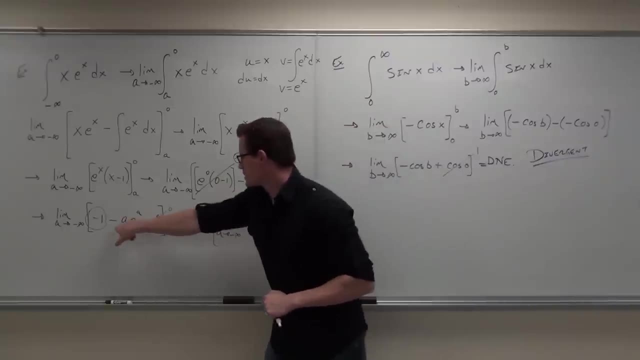 I want to see if you guys are OK with the math on that. Are you OK on where the negative one came from? Yeah, that's this limit. Limits are simple: Y, addition and subtraction. This is zero. No problem, I'm just focused here. 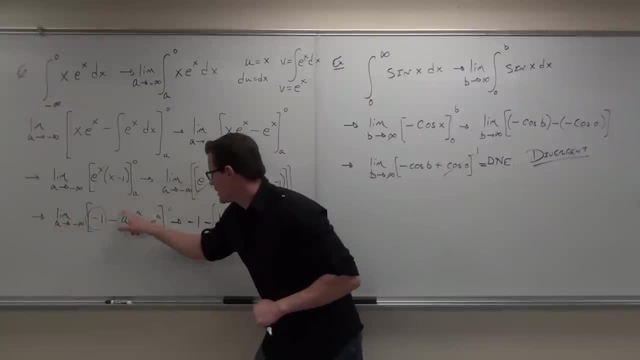 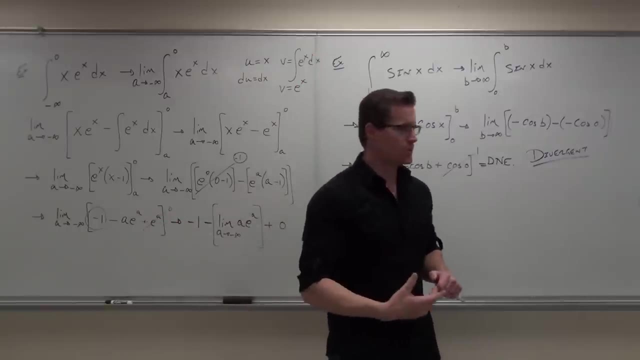 My minus is right here, So I have a limit as a approaches negative infinity of this guy, Just that guy. I hope you guys feel OK with that one Now if you don't remember how to do these zero times infinities or infinity times zeros. 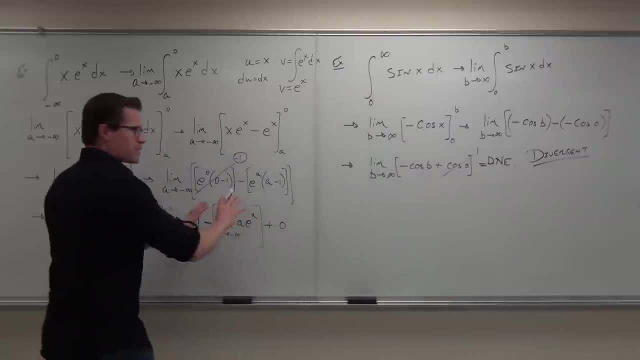 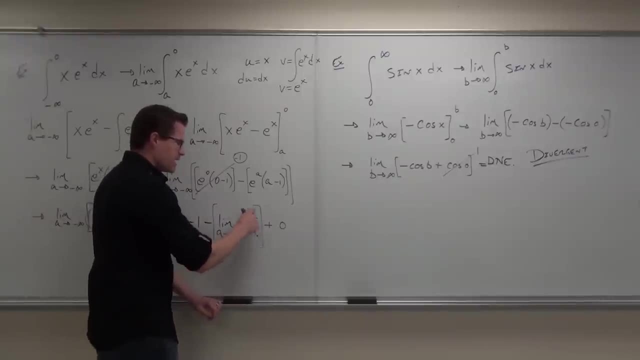 rewrite this as a fraction. So take one part of this and move it to a denominator. Now, what I know is that it's going to be easiest if I move this e to the a, to the denominator, So I'm going to take a little little break here. 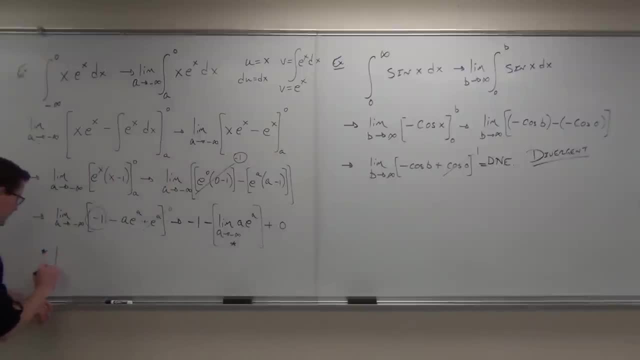 We'll call this asterisks. The limit as a approaches negative infinity Of a times e to the a can be rewritten as a limit as a approaches negative infinity. I'm going to keep the a. I'm going to keep the a right where it is. 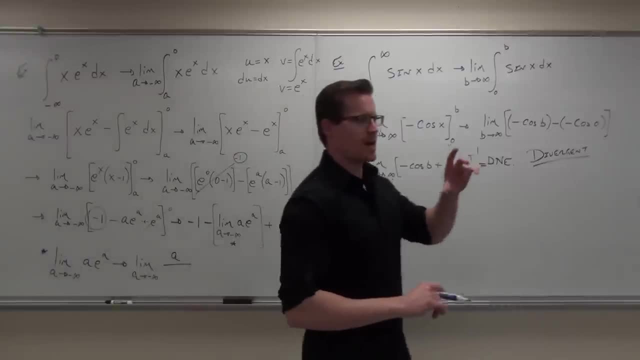 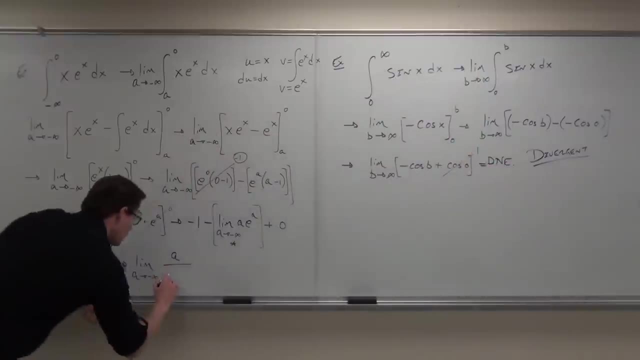 But the e to the a. I want to rewrite that. Can you tell me how I'm going to write a times e to the a as a over something to the negative? Yes, In your heads is this the same as this stuff? 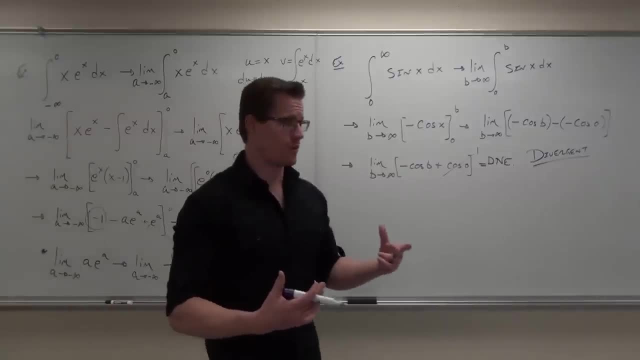 Now check it out. Remember whenever we change something in our limits. I don't know if you do remember it was a long time ago, But if you don't remember, rewatch the end of chapter six, OK, on the video and it will show you all this stuff. 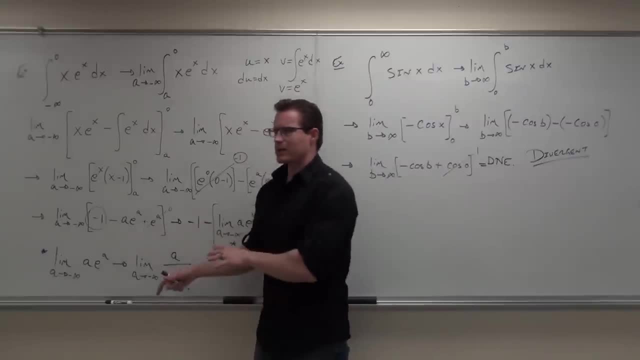 This was the indeterminate forms. Whenever you do something algebraically, you reevaluate it and you see what actually happens. So if we reevaluate this, how much is a as a approaches negative infinity? Now, how much is e to the negative? a as a approaches negative infinity. 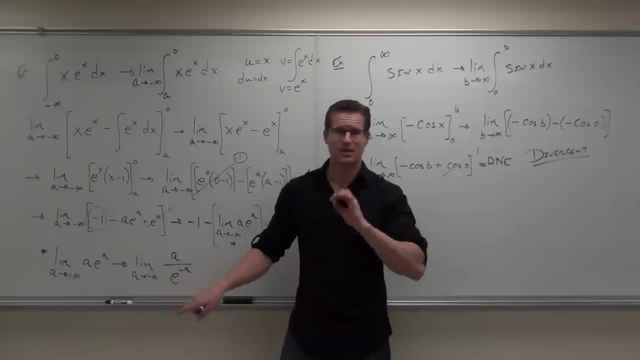 Remember a negative times. negative is a positive. How much is this? It's infinity. So we have a form of infinity over infinity. Does that make sense? This is a prime candidate for L'Hopital. Yay, L'Hopital. 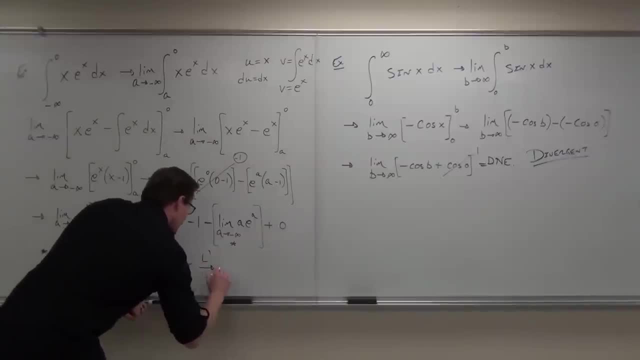 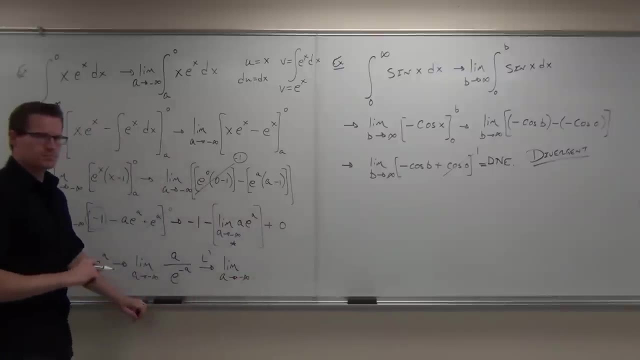 It's a fun word, even So. L'Hopital, Can you explain to me please how you do a L'Hopital's rule? What do you do? Take the derivative of the top over the derivative of the bottom. 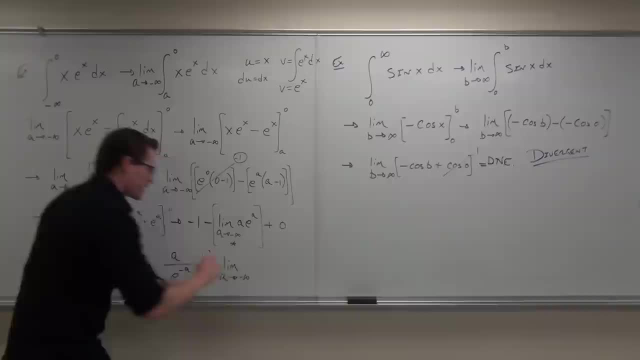 Cool. Is it a quotient rule? No, No, Derivative of a numerator is. This is why we left the a where it was OK. If we hadn't, if we made it one over a, our a power would grow and our e power would not decrease. 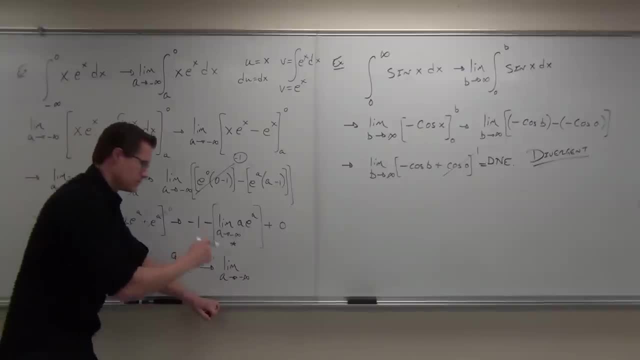 So that's why we left the a where it is, because the derivative of a is- That's beautiful- The derivative of e to the negative a. Can you tell me what the derivative of e to the negative a is? Negative e to the negative a. 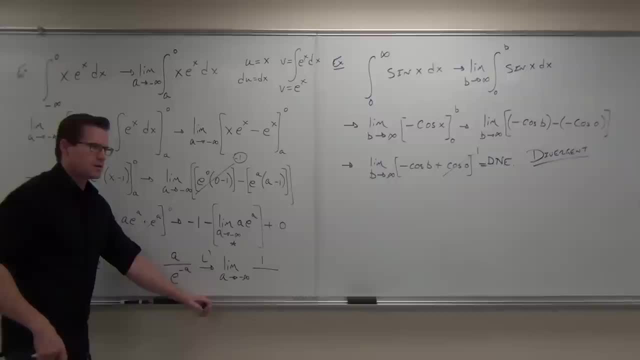 Some of you said e to the negative a. some of you said negative e to the negative a. Which one's right? Negative e to the negative a. What gives you that? Chain rule, Chain rule. Oh my gosh, we have a chain rule in here. 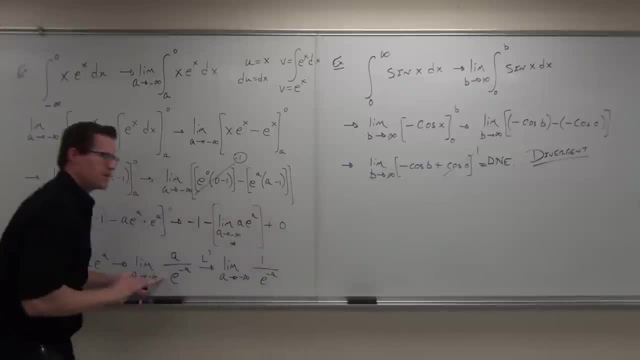 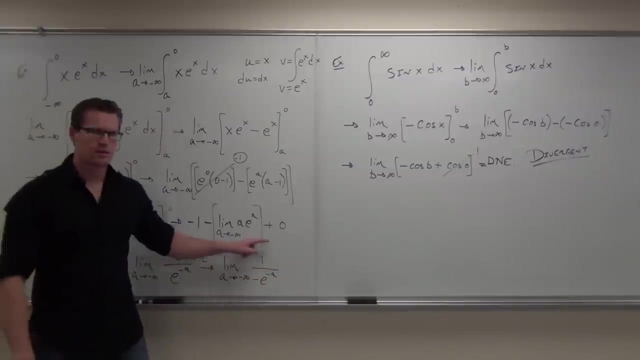 So derivative means you leave it alone. You leave e to the negative a alone, but you multiply by the derivative of whatever function's inside there. This is a function of a Derivative of negative a is negative 1. Now can you evaluate this limit? 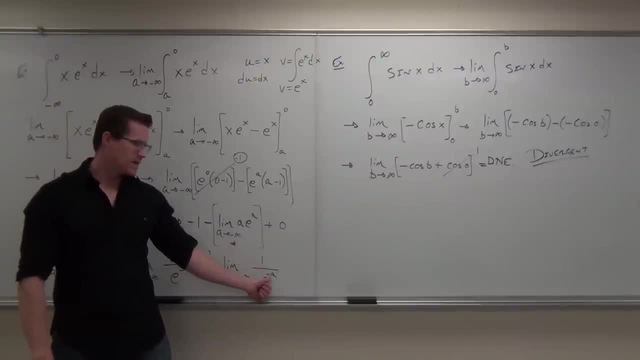 Yeah, Sure, How much is e to the negative? What was that again? e to the negative. a as a approaches negative infinity, Oh my gosh. So check it out. If a goes to negative infinity, you get negative infinity there, right? 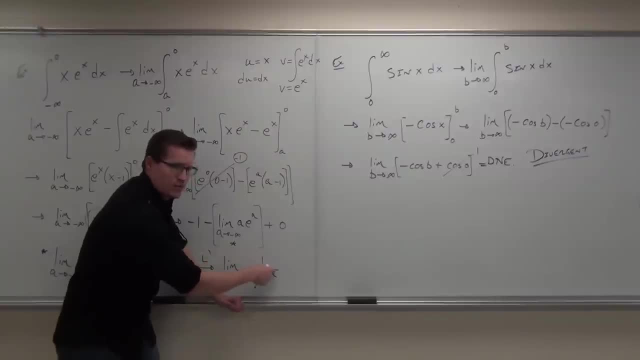 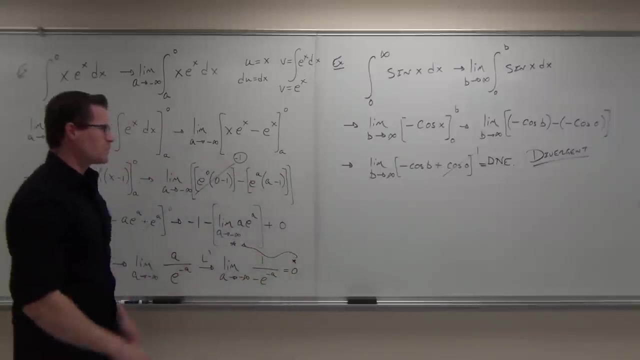 Negative, negative infinity is Positive infinity. e to the infinity is Infinity Negative infinity. I don't care what it is. If it's a number over infinity, you get how much Zero. This is zero. Now, this is our asterisk, so we'll move it right back up here. 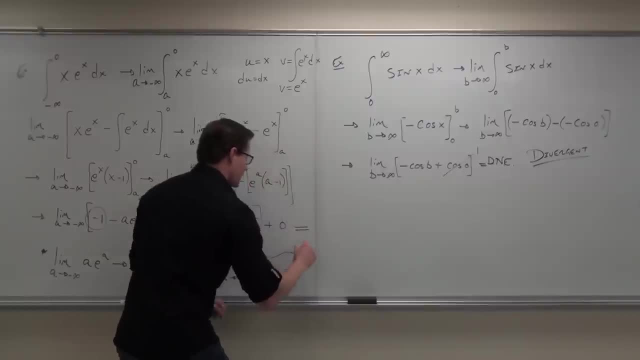 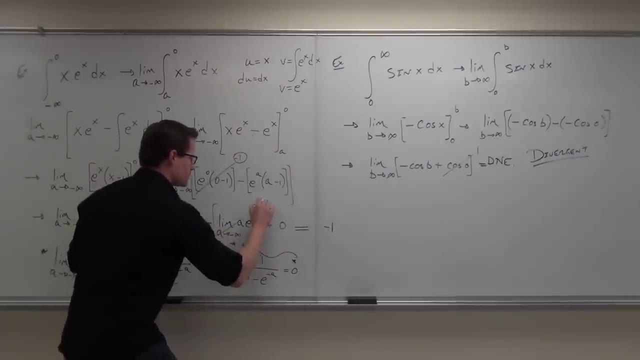 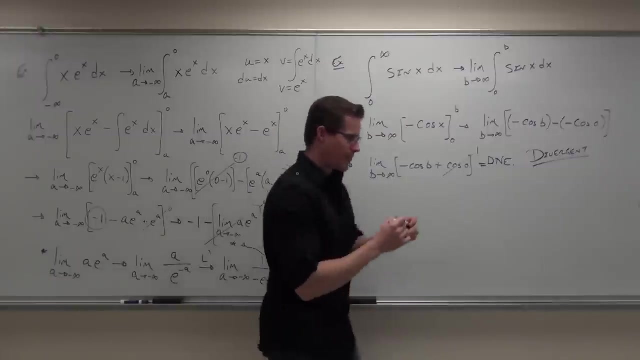 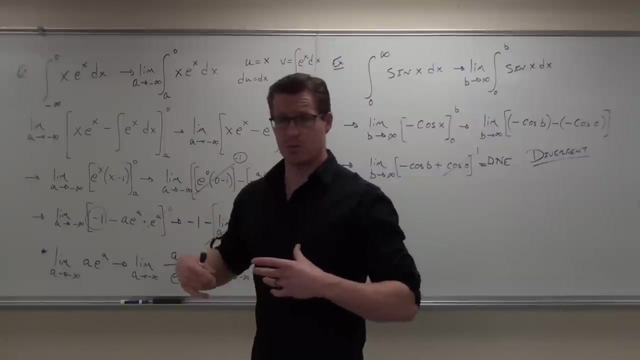 So what our limit is is: what do we have left on this thing? Negative 1.. Negative 1.. This whole thing went to zero. What's really? I don't want you to forget what we're actually doing. okay, A lot of people in calculus they end up learning how to do this stuff, but not really what you are doing. 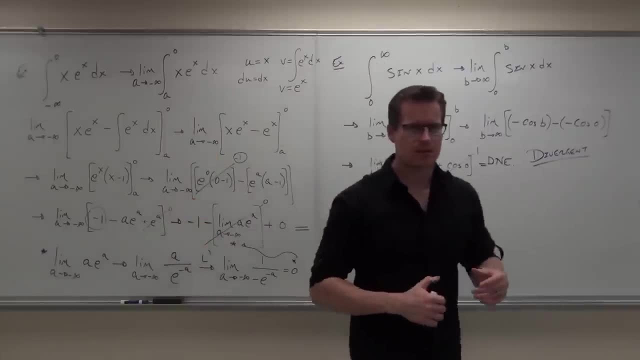 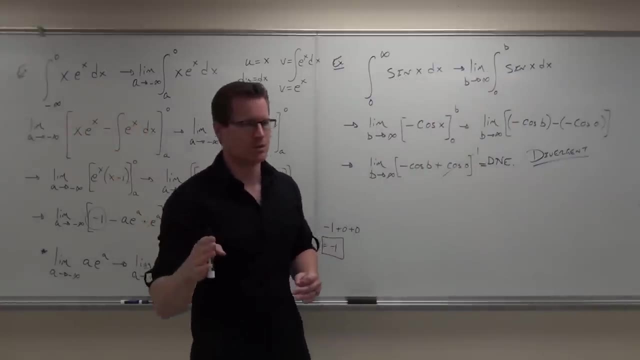 What do we just do here? What do we find? Area under this curve from negative infinity all the way up to zero. And how much is it equal to Interesting? That means it's below the x-axis. That's what that area means. 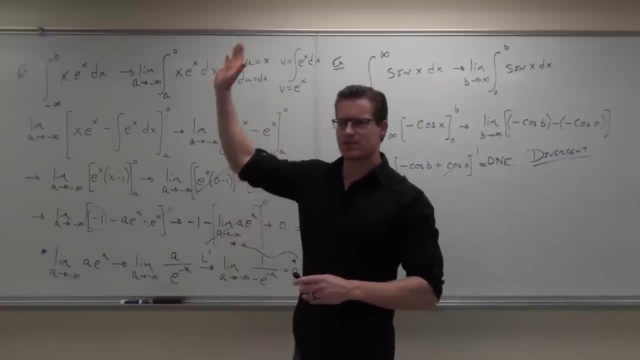 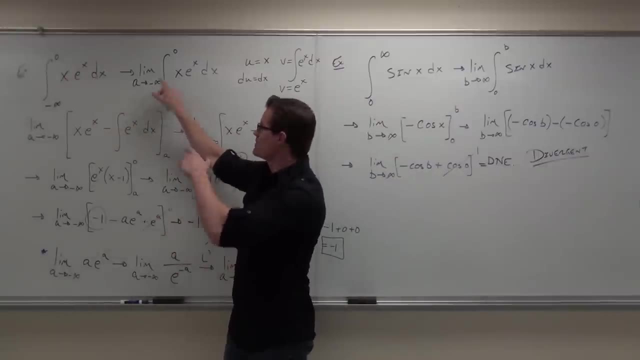 The majority of it is below the x-axis. Should we actually be okay with this example? So we do, hey, infinite interval, no problem, Make it definite, Just define what's happening. This means that we can actually do the integral by integration by parts or whatever we have here. 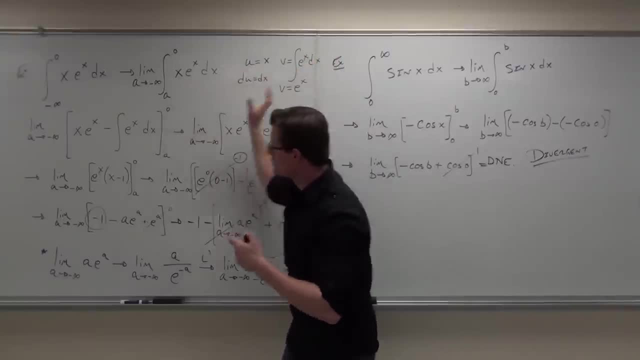 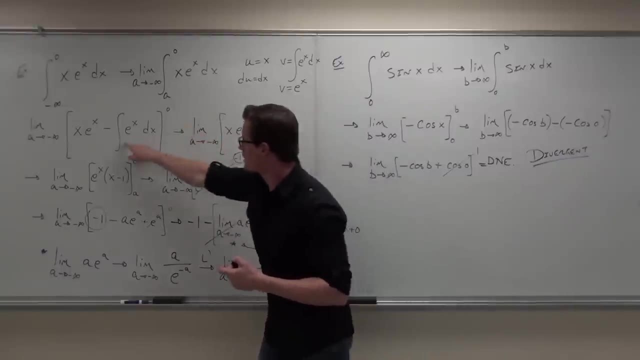 Integration by parts. So u is x, v equals integral to the rest. Do integration by parts: u times v minus integral of v to u. Evaluate that thing once you've done the complete integral, Not right here, but after you've done the whole thing. 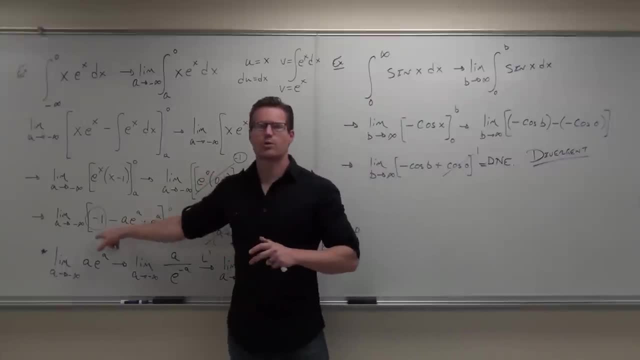 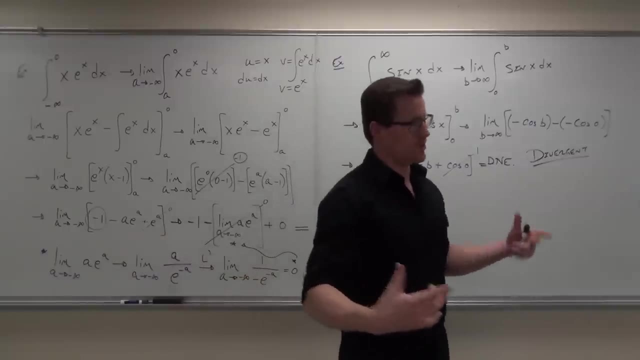 Evaluate it, then simplify it and then work with your limit. Haven't you covered all this stuff before? Yeah, Oh, and nothing's really new, Nothing, It's just putting it all together now. Sure, you're okay with it. 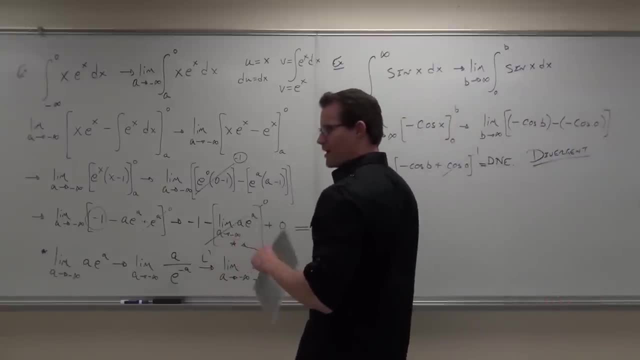 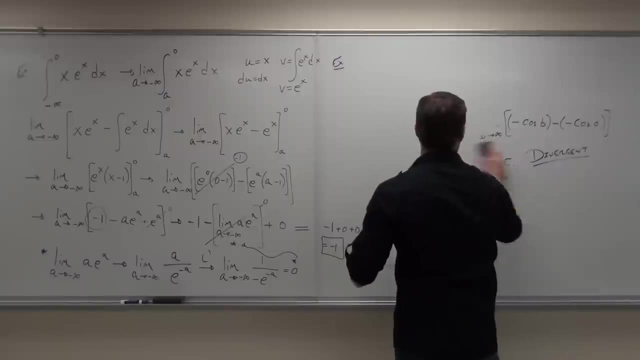 Yeah, Okay, Can we move on a little bit? Yeah, Finally on a roll. These problems don't take 45 minutes. a problem like before, which is nice too. You're going to love that on your homework, I'm sure. 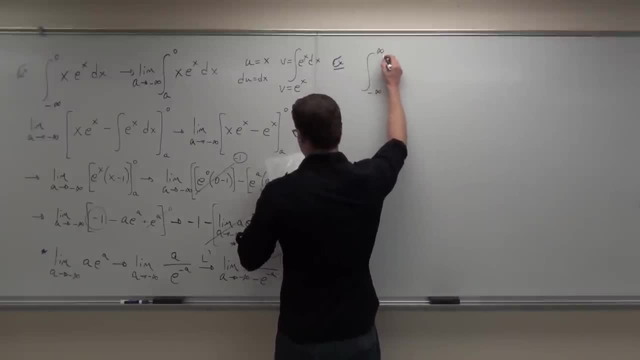 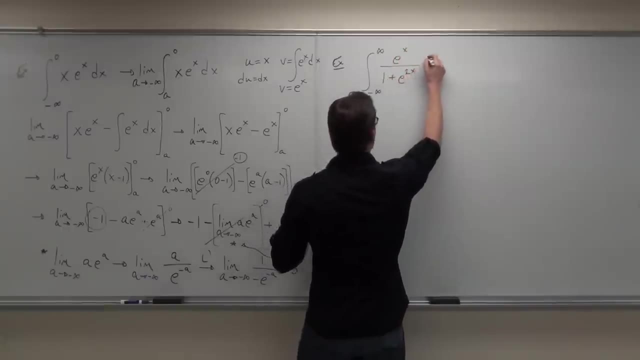 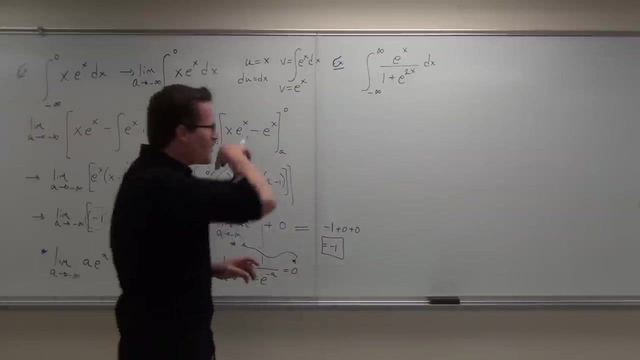 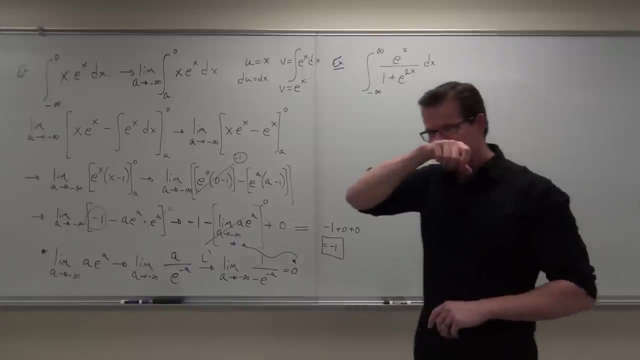 Well, except for this one, What K K K, Why? Why do we do this? Why do we want to murder us? Oh my gosh, Let's think it through. Let's think this through. First thing, are we defined because we always check this first. okay, 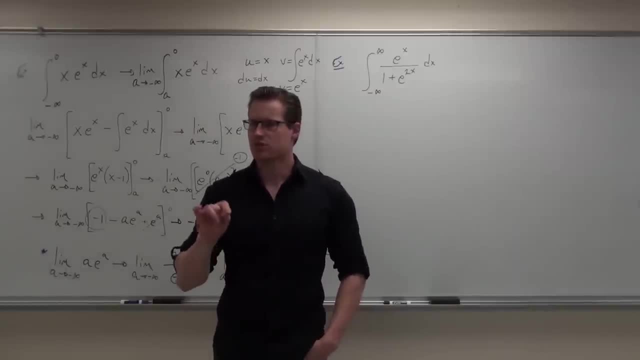 Look at your function inside of your integral. Is this function defined for your entire interval? If you say no, then you better give me a number that doesn't work here and you better rewrite it. So if you just guessed at it and said mm-mm, because it looks funny, probably not the best thing to do, all right. 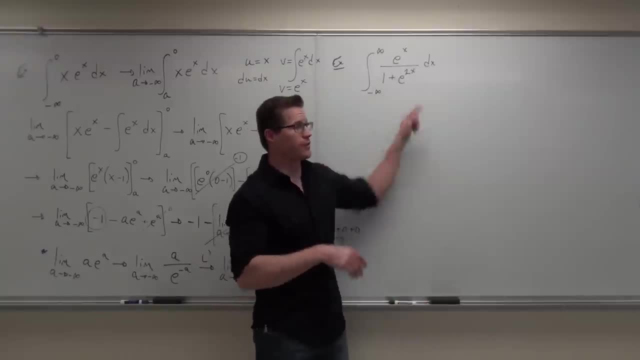 So why don't you think about it? Is there anything that gives us a problem in this function? Is e to the x defined everywhere? Yes, Yes, So this is fine. Is e to the 2x defined everywhere? Yes. 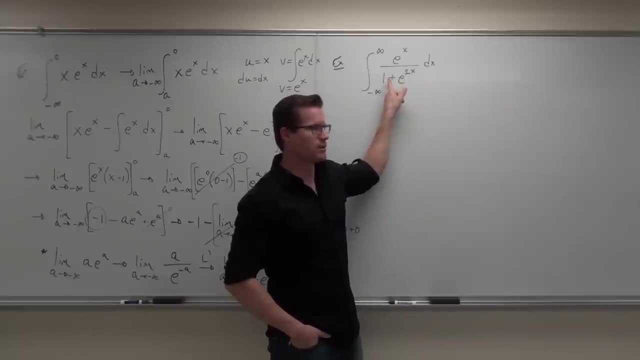 And if I add it to 1, do I have a problem in my domain? No, No, This is defined everywhere, but that's what I'm asking you to check. You've got to be good with finding domain. This is why your teachers taught you how to find domain. 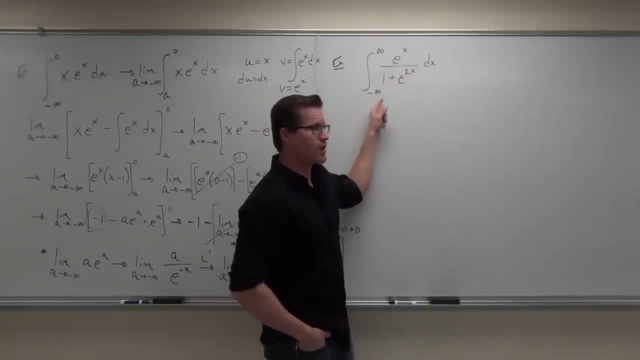 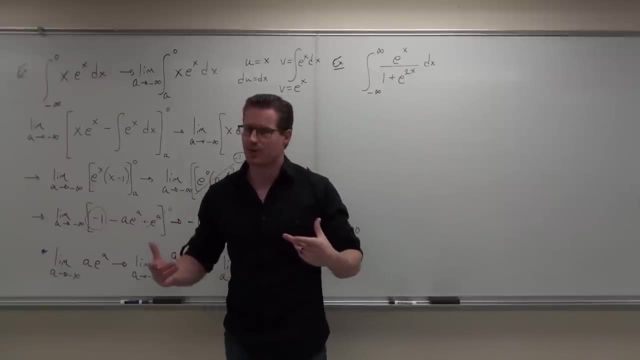 So you go. oh, you know what? My domain here is all real numbers. Therefore, on my interval of all real numbers, I'm good to go. I don't have to worry about any infinite discontinuities, because there are none on this function. 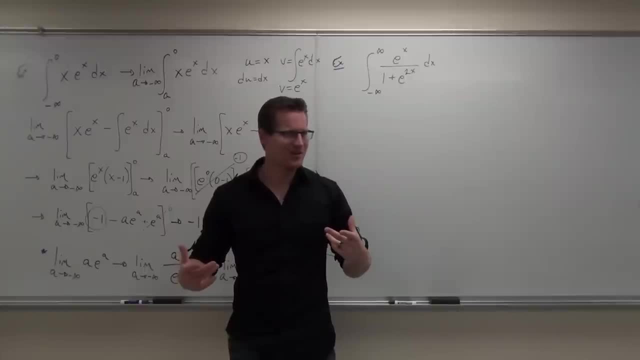 I know I just talked fast, but did that make sense to you, Are you sure? There's nothing that makes this 0 or negative. Therefore, if this is always positive, it's being squared. so no problem, it's positive. 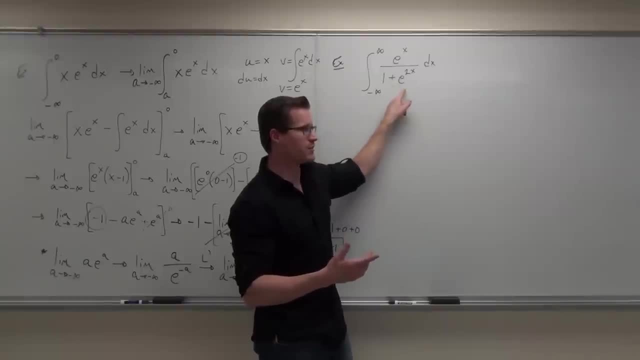 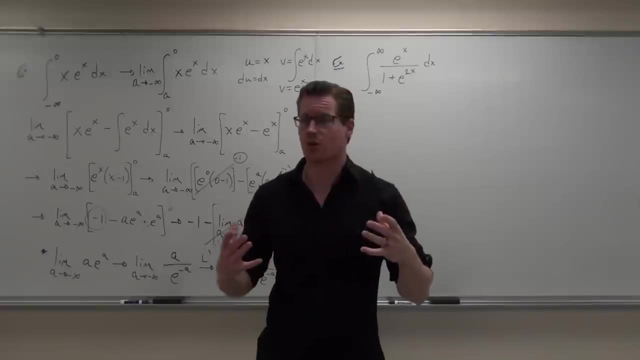 If this is always positive and I add 1 to it, it's still always positive. It can't ever be 0. It can't ever give me anything. I don't have any problems. This is always defined. They're both always defined. so my entire rational function is always defined for an entire interval. 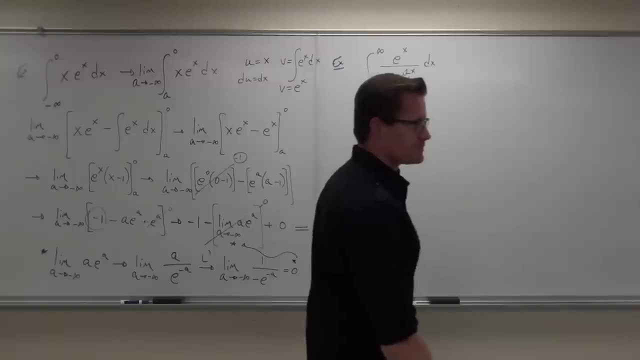 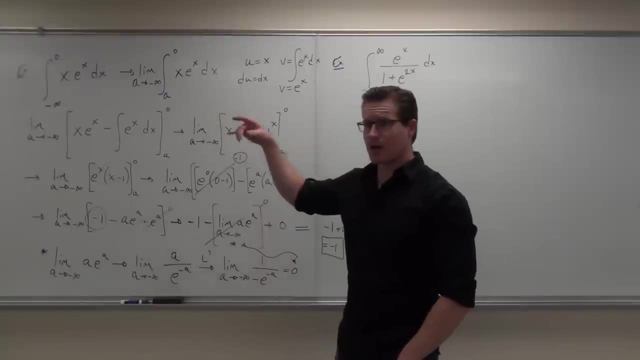 Now the problem is that: what's the problem here? What's our problem? Negative infinity to infinity? Yeah, it's this idea of: oh my gosh, we've got this double infinite interval where I'm not going from negative infinity to a number like 0.. 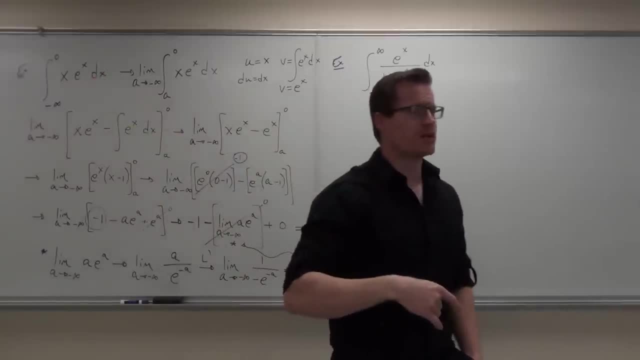 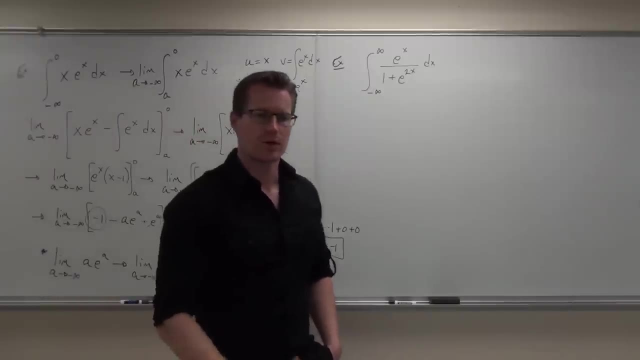 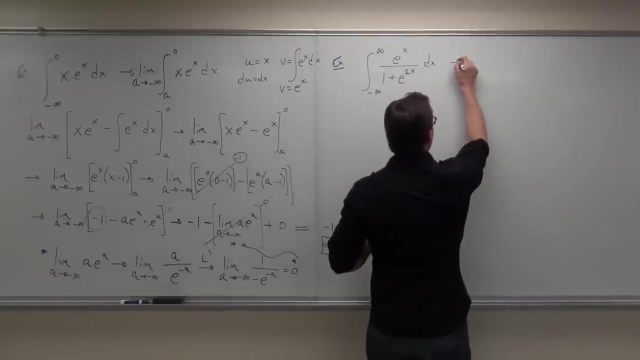 I'm not going from 0 to a number like infinity, I'm going from negative infinity to infinity. So what in the world are we going to do? Simulator to infinity. Yeah, You know, what we're going to do is, instead of thinking of this as one big integral, 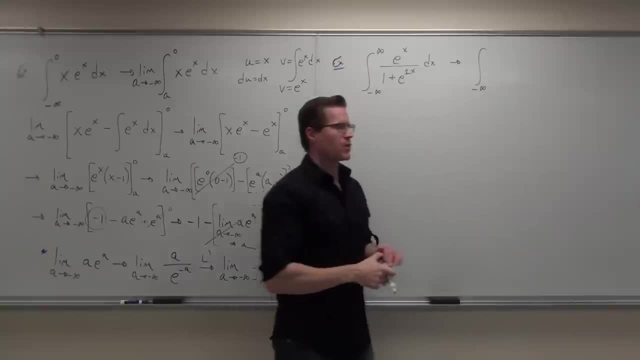 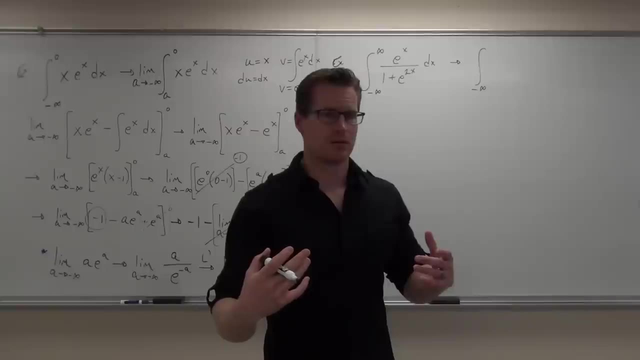 let's think of it from negative infinity to. I don't care what number you pick, it's going to be the same. whatever you want to pick Now, I'm probably going to pick the easiest number I can think of to plug in. 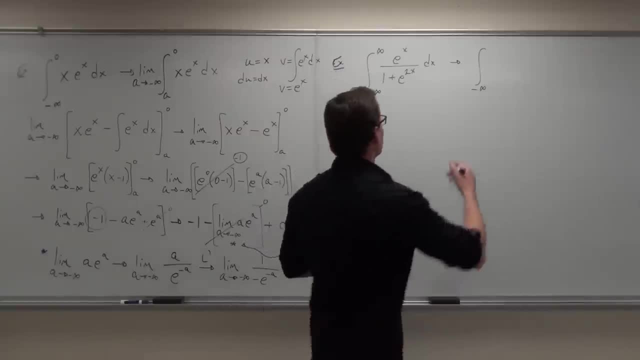 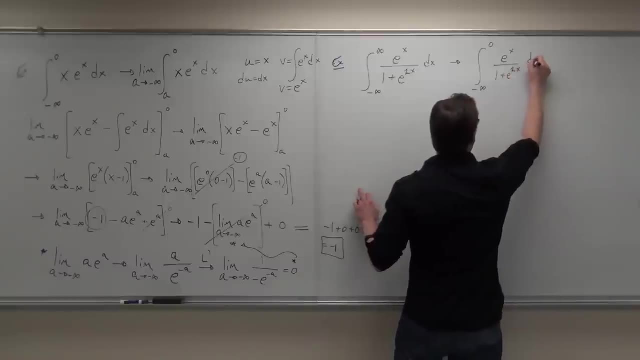 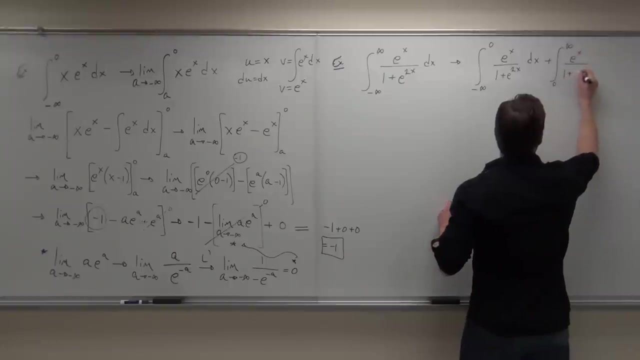 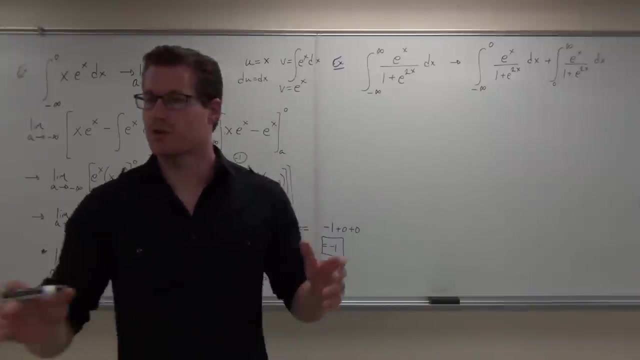 I'm going to pick 0, because 0 for me would be the easiest number to plug in. You guys know, hopefully from your Calculus 1 class, whenever you took it, that you can actually separate integrals like that. 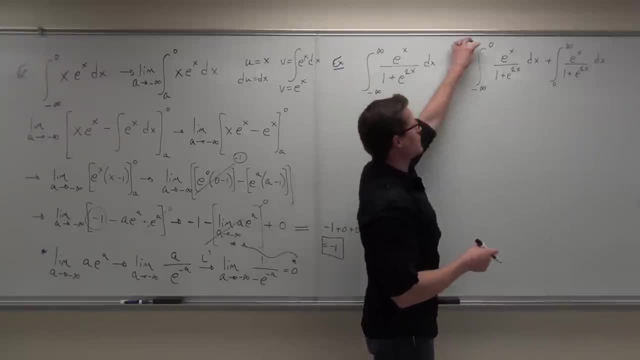 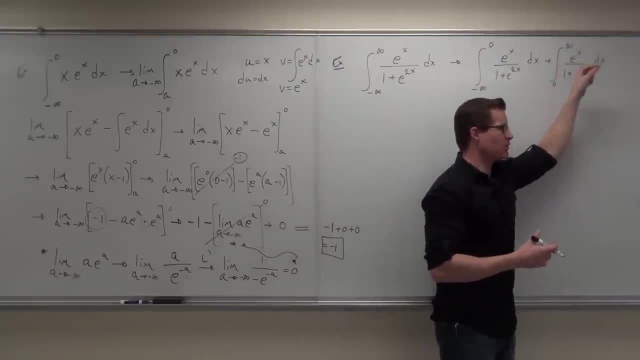 You start from wherever your a is, introduce some intermediate number c and then go from that number c to where your ending is. So your ending value is b. So instead of from a to b, we go from a to c and then again from c to b. 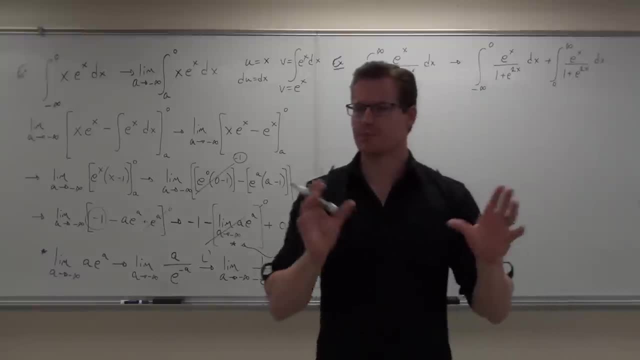 and we add those integrals together. That's legal to do As long as you have no problems in between there. that's legal to do. Quick head note, if you're okay with that one. Hey, have we seen stuff like this? 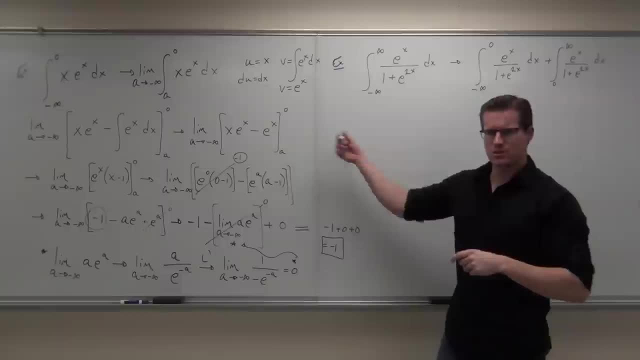 Yeah, Have we seen stuff like this? Yeah, Can you guys do the next step for me? Write out what you would do. Change these into our limits for us, okay? Remember that lower bounds typically change to a's. upper bounds typically change to b's. 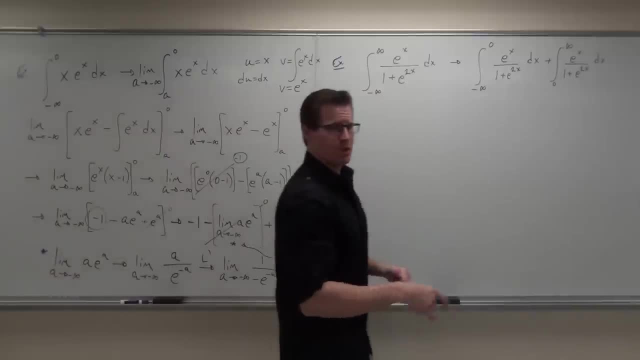 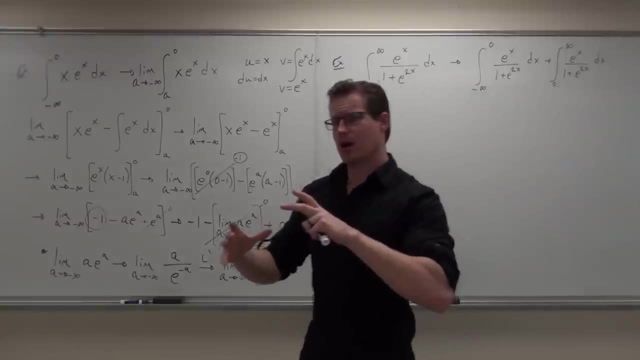 So go for it. What is nice about this, though, is that we don't have to do the integral twice, Since we're just rewriting the same thing. our integrand right there hasn't really changed. We'll just do the same idea for both of these integrals at one time. 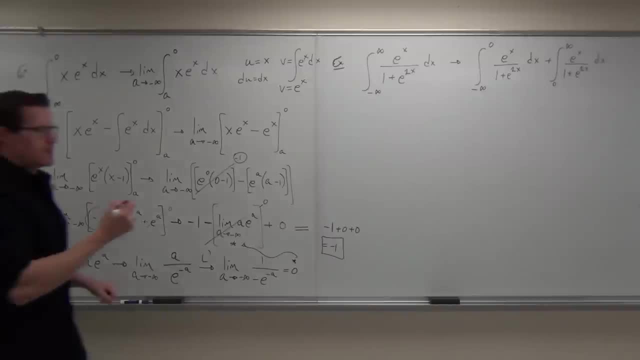 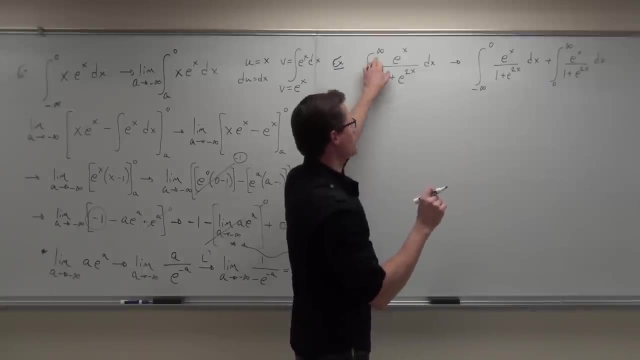 So here's what I'm asking you to do. I'm asking you to firstly understand that when I have this type of integral, where it goes from negative infinity to infinity, you do have to do this with two integrals here. You have to separate it. 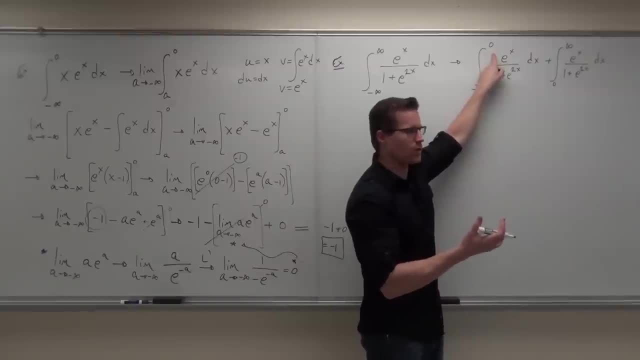 So we have to have at least some solid bound in between there. Call it 0,, call it 1, whatever you want, 0 is going to be easier to plug in. Remember that we do have to evaluate these sort of things, right. 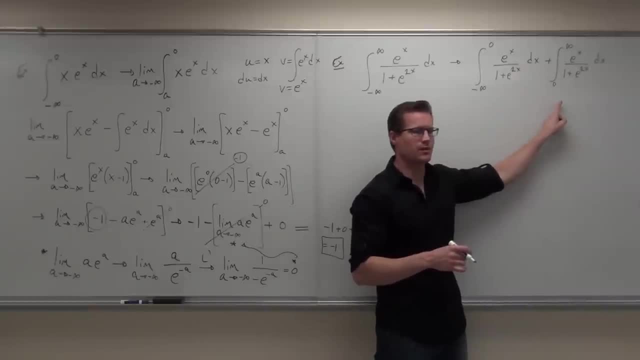 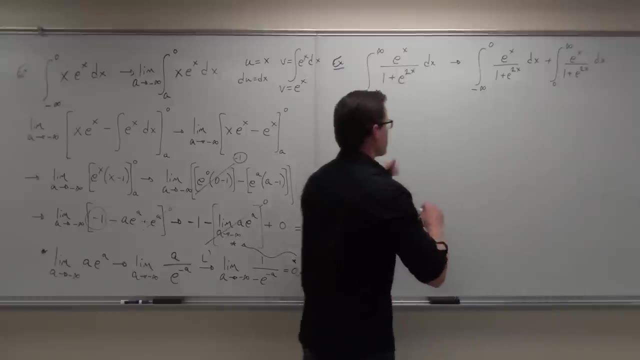 So we're going to have to plug in this number twice. 0 is going to be easier to plug in than negative 7 or something like that. You will oddly get the same answer out of that, but it's going to be easier to plug in if you have a 0. 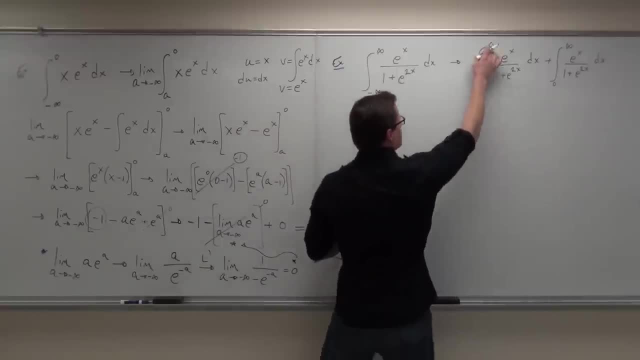 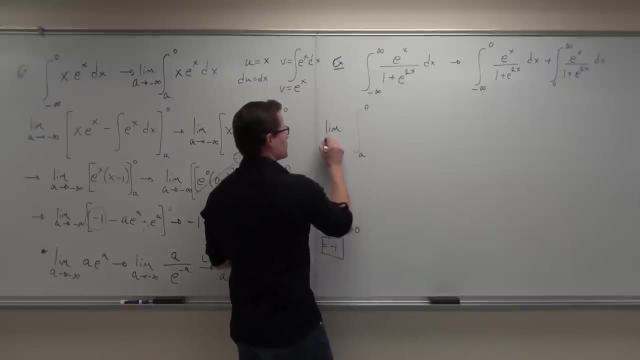 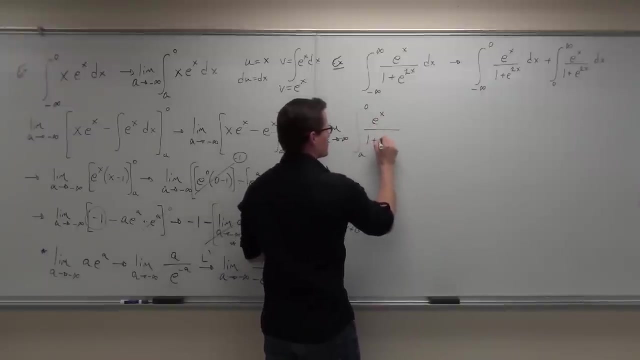 So we'll have, instead of going from negative infinity to 0, what's my bounds of integration going to change? to a is 0.. Now I'm going to define it Limit as a Perfect. The inside of my integral, my integrand is not changed. 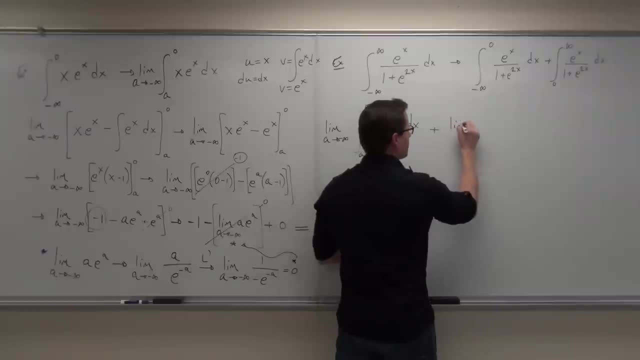 Plus what's the next thing? I'm going to write, Plus the negative As b: How far is infinity Good? Well, if I've called b positive infinity, the 0 doesn't change with infinity. I'm going to call that b. 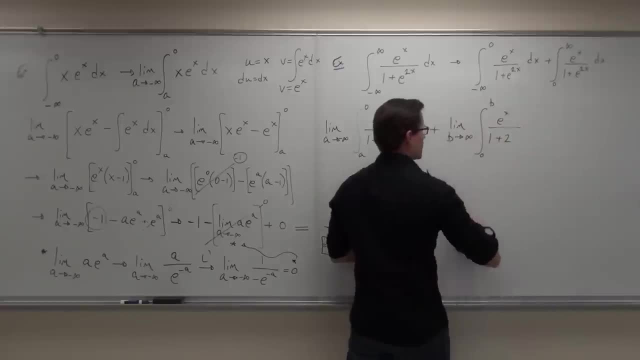 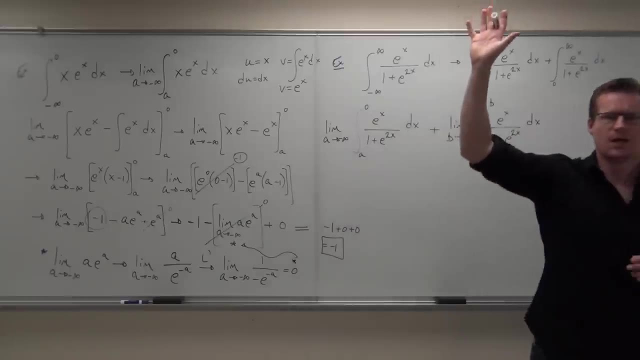 e to the x over 1 plus 2x. That's not right. e to the 2x. Okay, quick show of hands if you feel okay with this idea. Just a combination of two ideas that we've had before, And here's the nice part. 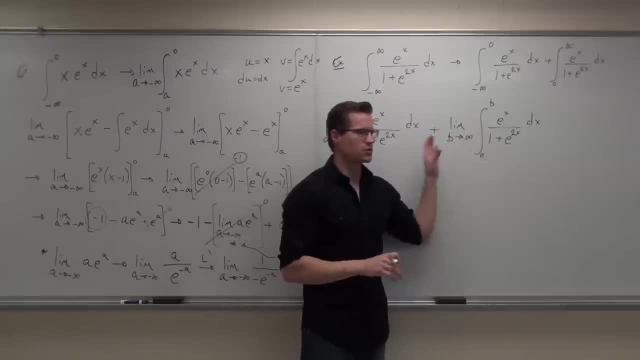 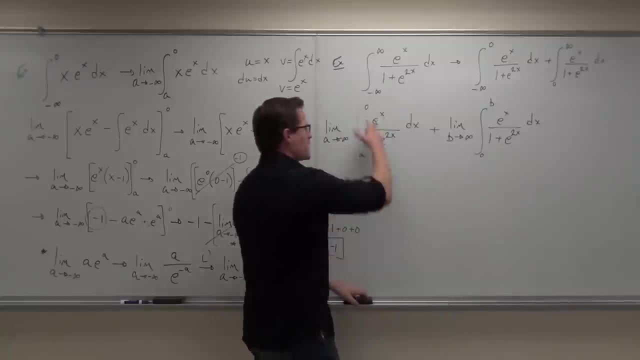 Once you've done this, I don't want you to do each of these integrals independent of each other. Understand that they're exactly the same. You guys get it So off to the side. I'm not even going to worry about the a to the 0.. 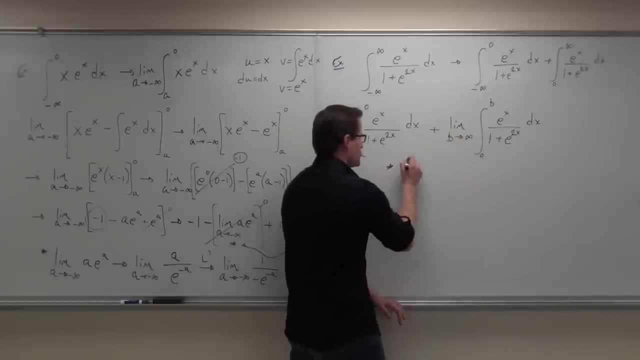 I don't care. I'm not going to worry about the 0 to b. I don't care about that. I'm going to just do the integral of e to the x over 1 plus e to the 2x. Let's just do that. 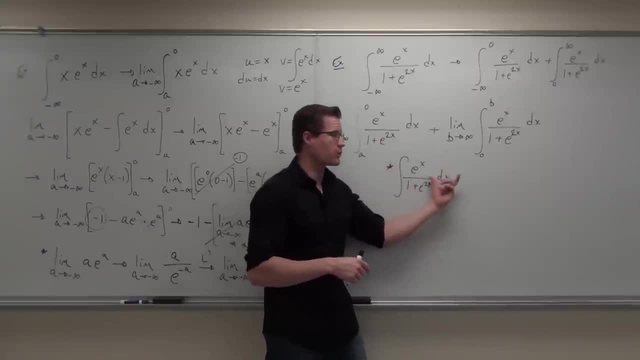 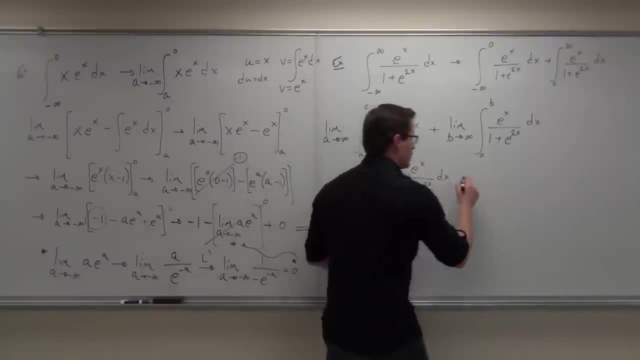 Take this idea and run with it afterwards, And then we'll evaluate whatever we get twice, from a to 0 and then from 0 to b. Do you understand that idea? So just do the integral. off to the side Now. hopefully you can do this integral. 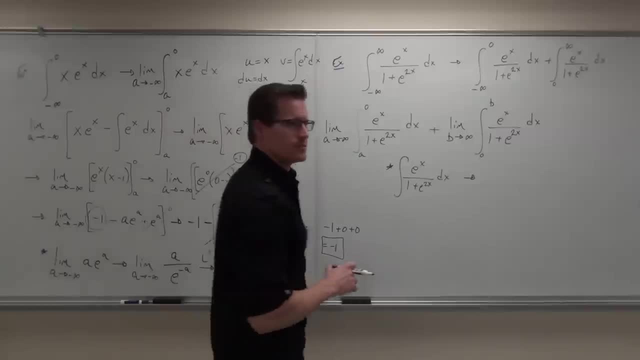 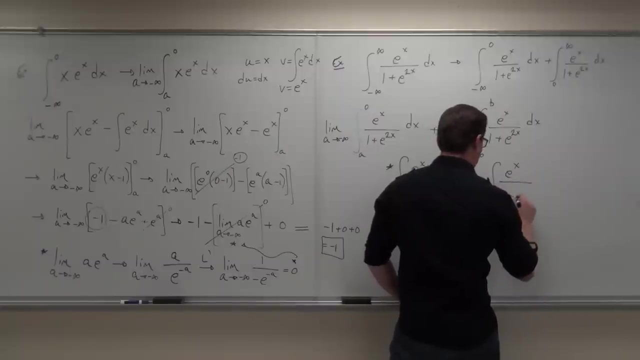 Let's walk through it. Is it a substitution? If you say no, okay. If you say yes, explain that to me. u equals e to the x. Oh my gosh, Someone's good at substitution, True, Yes. 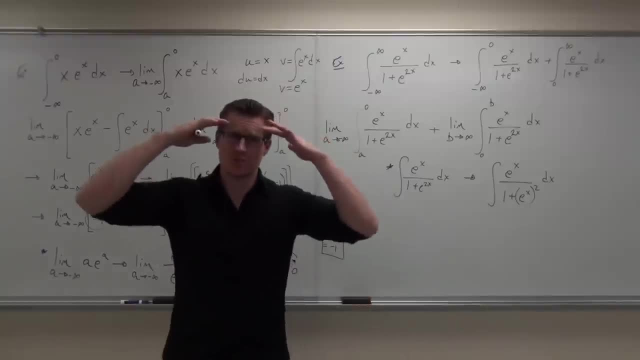 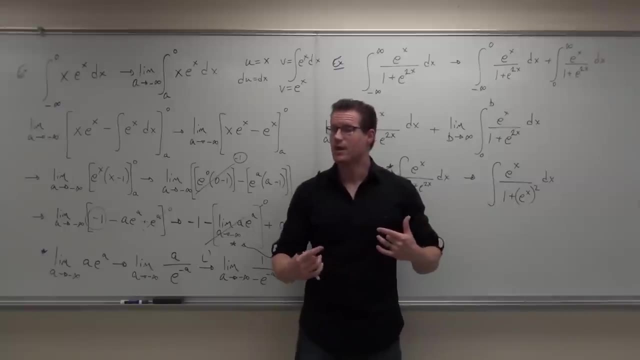 Hey, let's be smart about this. Don't jump to a conclusion of I don't know how to do it, Rewrite it. Think about these things. Think of: can you find a derivative somewhere in your problem? If you can, then you have a substitution here. 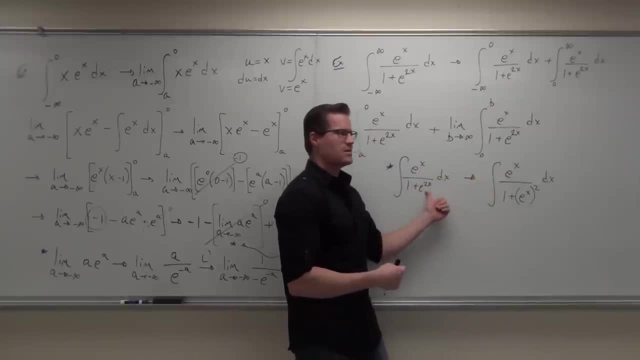 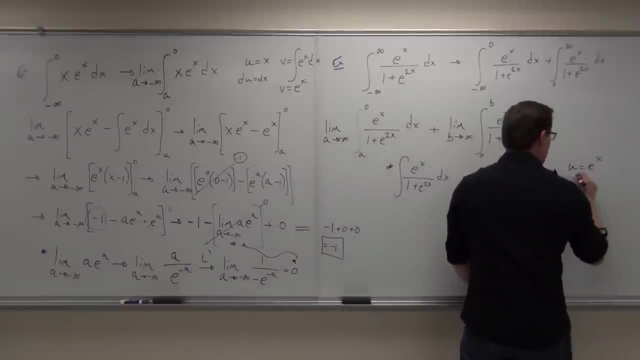 So e to the x, not a problem. Ooh, e to the 2x. Now let's think about that as e to the x squared. If that's the case, a substitution of u equals e to the x. Man, that works nice. 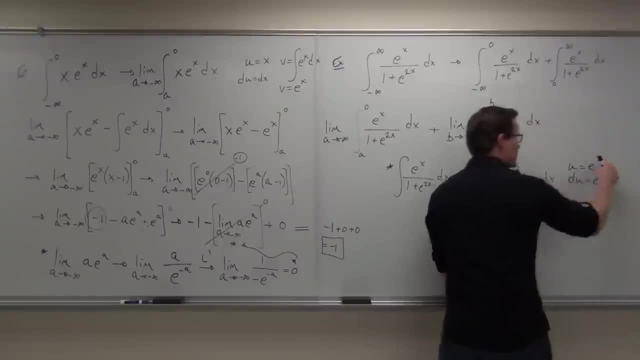 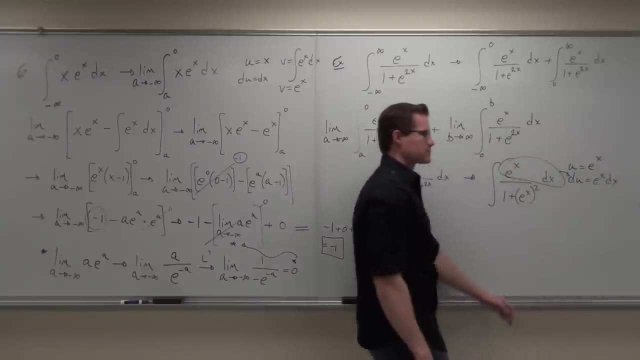 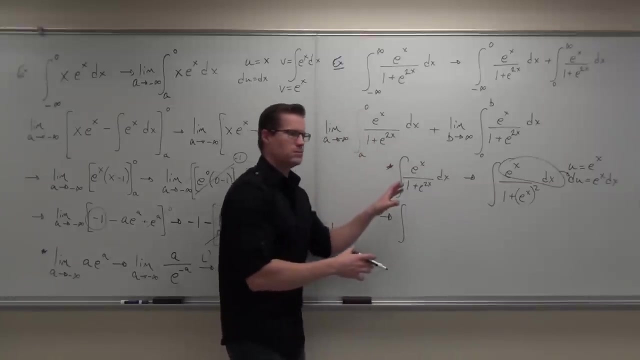 du equals e to the x dx. The derivative of e to the x is e to the x. Check this out. Here's e to the x dx. Here's du. It's right there. You guys following me on this one? OK, so integral. that looks really hard right now. not so hard. 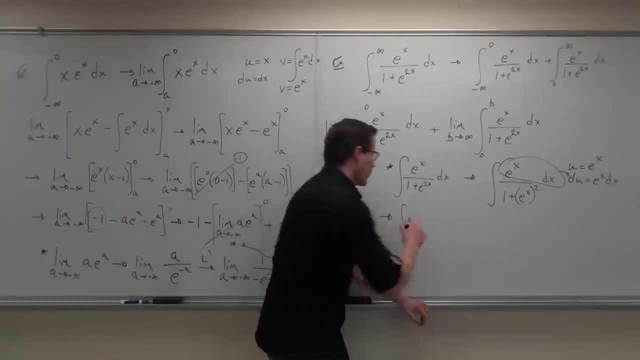 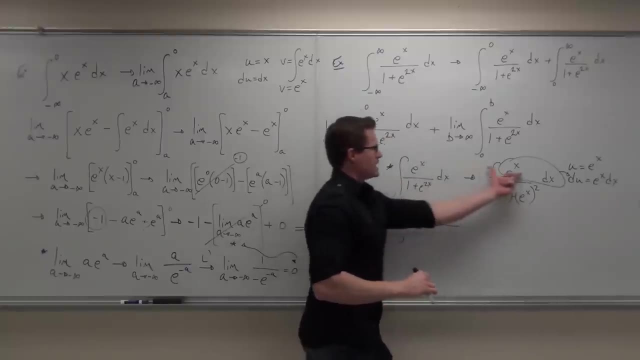 Tell me what's going to be in the integral. Tell me 1 over 1. 1. OK, so this goes away. This is basically. you can write du. even if you want to, I'll show you that You can write du, because e to the x, dx is du. 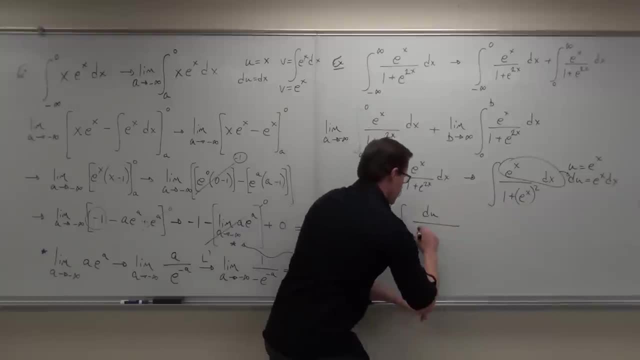 e to the x dx. is du over what? 1 over 2 squared Now, if you don't like the du being there, OK, call it a 1.. Put the du over here. I just want to make sure that you are OK doing our substitution. 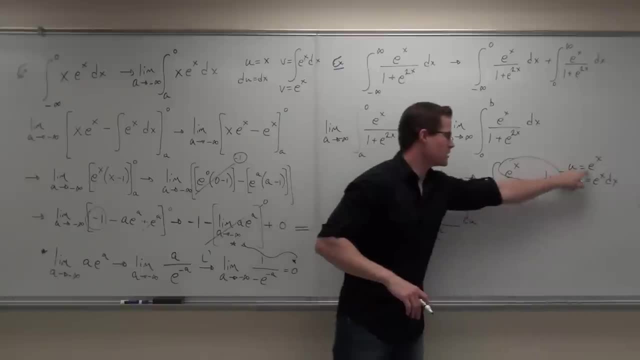 e to the 2x is e to the x quantity squared. And then doing u equals e to the x. Hey, no problem, This is 1 plus u squared. du equals e to the x dx. We've got a 1 du. 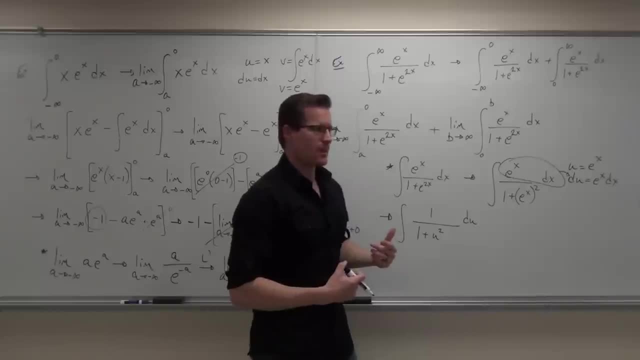 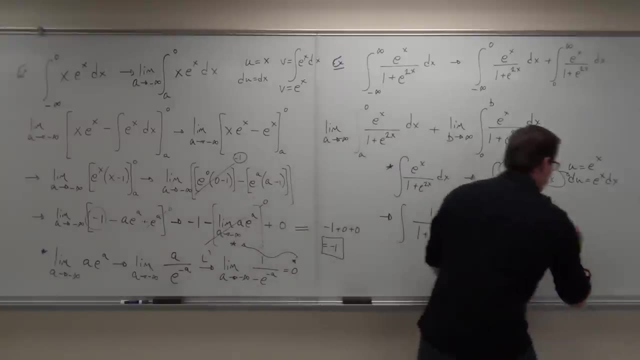 Show hands if you're OK with that one. Now you've got a couple options here. You can do this the hard way or you can do this integration table way. The hard way would be a trig sub. The hard way would be, and this would be just fine if you want to do this. 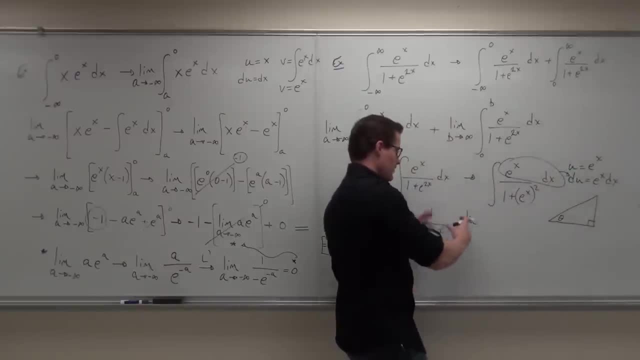 Remember doing this: Even though you don't have a square root, you can put one in there. You do square root of this whole thing. squared, You would have square root of 1 plus u. squared, You'd have u and you'd have 1.. 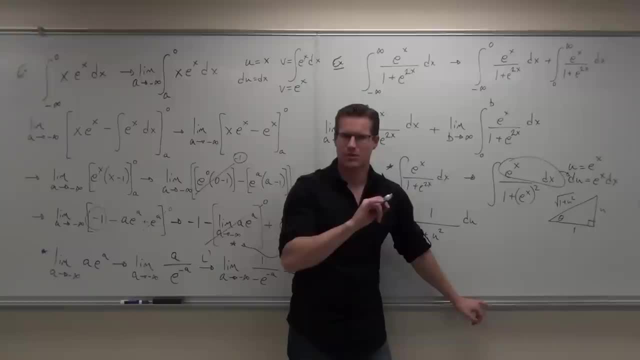 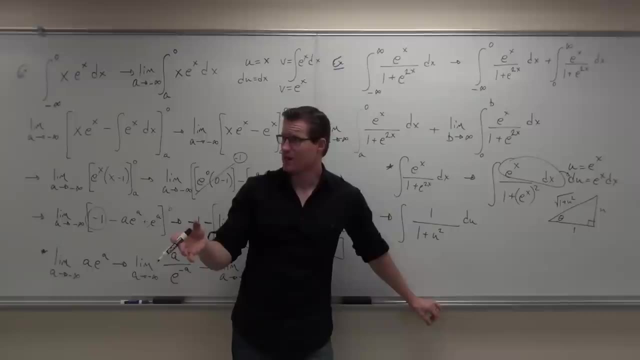 You would have tan theta equals u. Does that make sense? You do it that way, Or you could recognize that this right here is actually in your integration table. Now, when we're doing trigonometry- I'm sorry, when we're doing integrals. 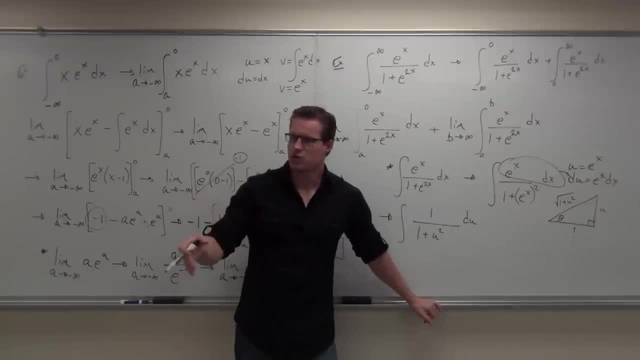 the first thing we should be looking for is our integration table. right, We should make things harder than they have to be. We should try substitutions and integration table first. Well, if this is in our integration table, that's brilliant. How much is it? 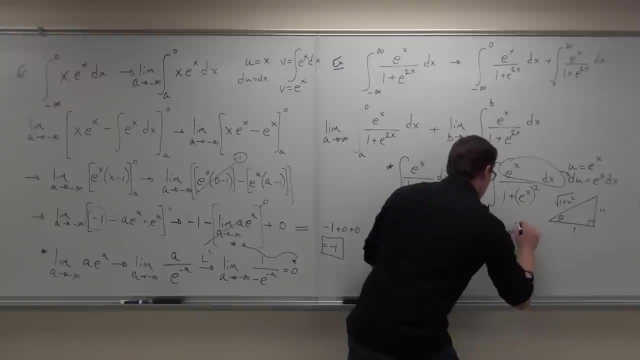 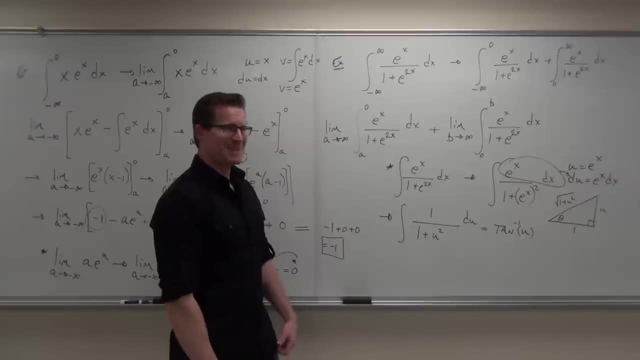 Tangent inverse. Tangent inverse of u: Tanverse, Tanverse, Tanverse Made up a new word: Tanverse, Tangent inverse of u. Yeah, absolutely, That's exactly what that is Now. let's not make a mistake. I did before. 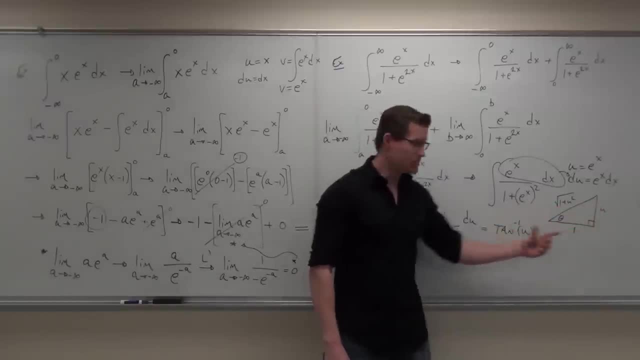 By the way, would you guys know how to finish it off if you did the triangle? Let's say you didn't see this on your test. Could you do that? Sure, You know. trig sub Tan theta equals u Du equals secant squared theta d theta. 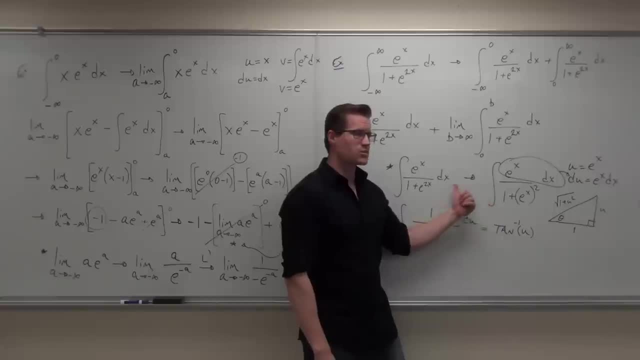 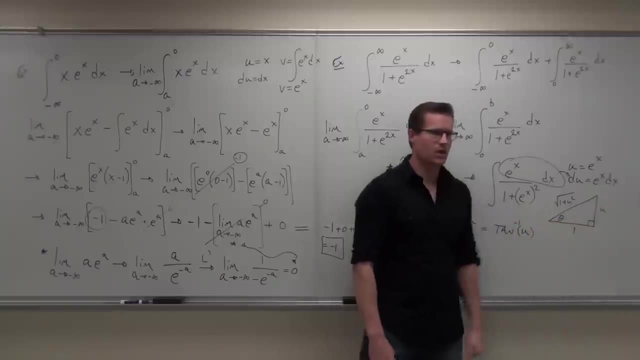 You'd have a little bit of work to do here, but what you'd end up getting is a secant squared theta over secant squared theta. You'd get 1.. The integral of 1 is theta. Theta equals tan inverse of u. 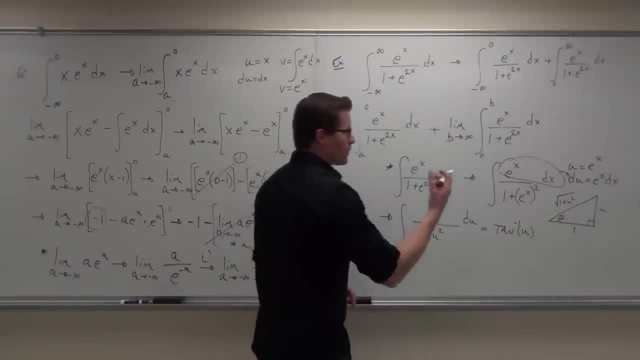 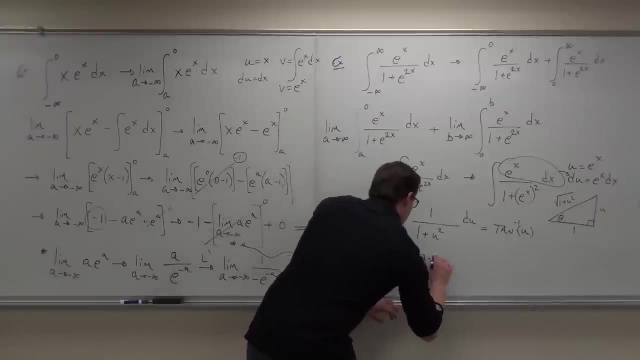 Bam, it's right there. It's exactly the same thing that we would get. So tan inverse u. What's the next thing I'm going to do? Substitute, Very good. So if I substitute, I get tan inverse. 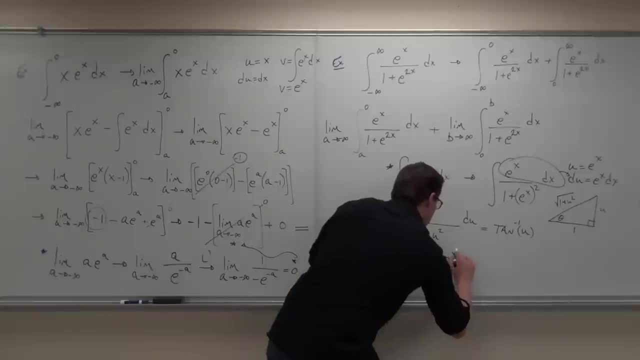 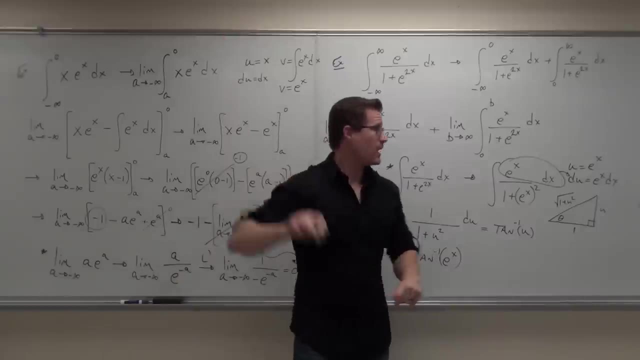 Oh. tan inverse of what? E to the x, Perfect. Tan inverse of u, No, no, no. Tan inverse of e to the x. So your parents would be okay with that. so far. Now I'm going to rewrite this because I want to be a little bit more clear than what I'm being here. 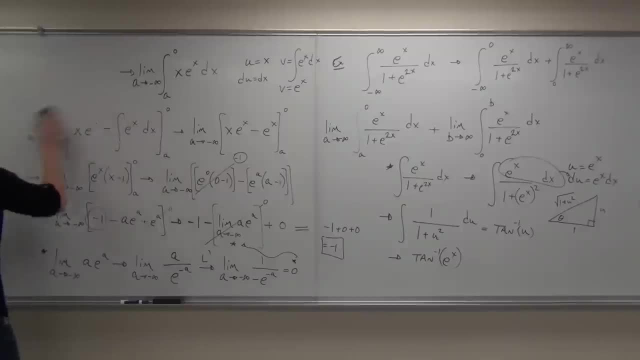 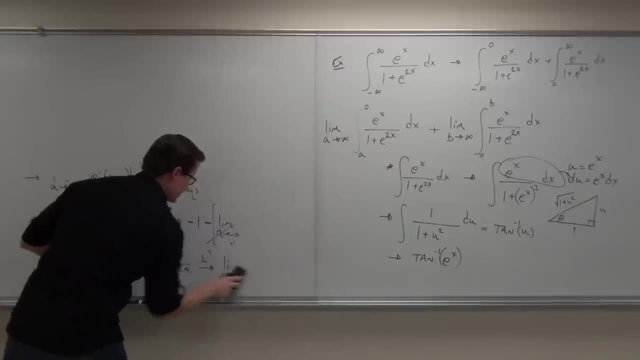 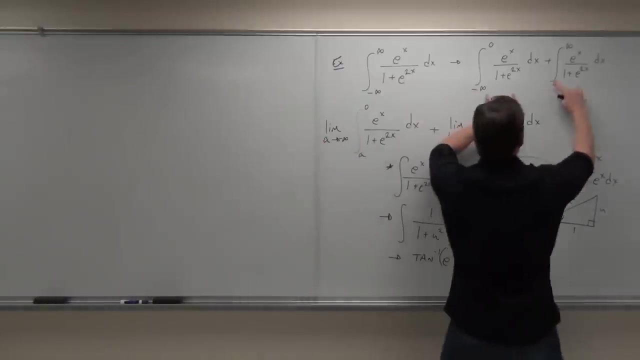 So do you have any questions on this side? No, All right, I'm going to show you exactly what's going on with this thing here. So what we ended up getting was these two integrals, And then we change them to, okay, some definite integrals, so that we can actually evaluate them. 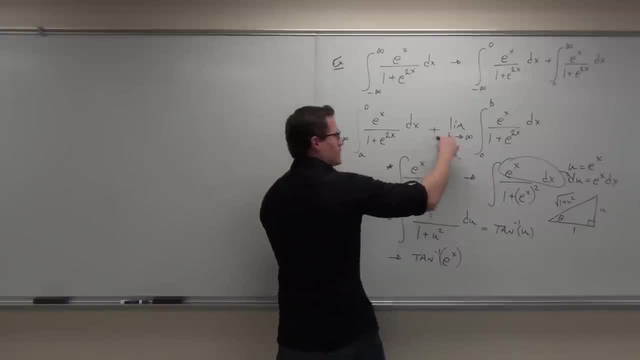 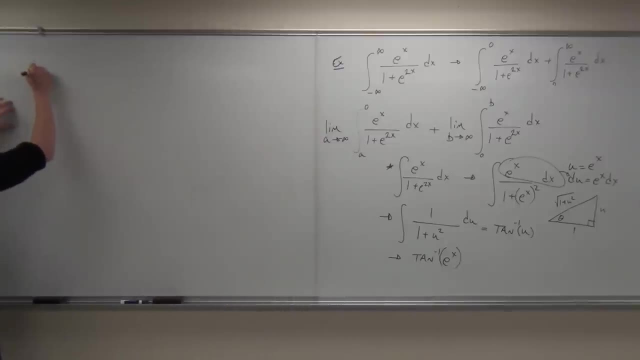 But we made our limits so that these bounds go to negative infinity and positive infinity respectively. So I'm going to rewrite this piece, Then we're going to look at what happens in conjunction with that. So we had a limit as a approached negative infinity. 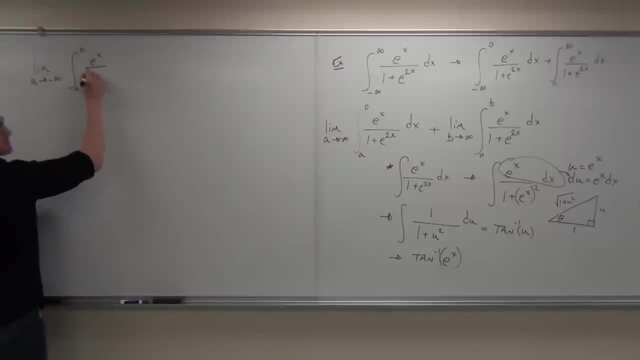 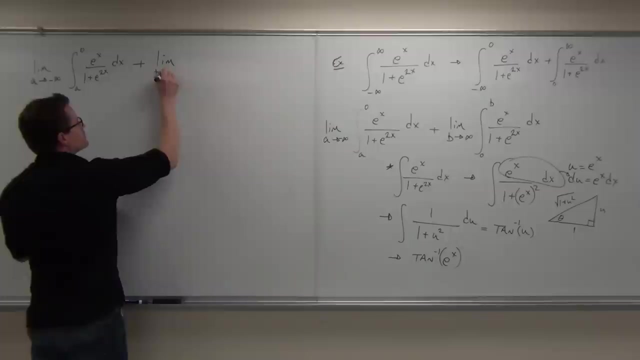 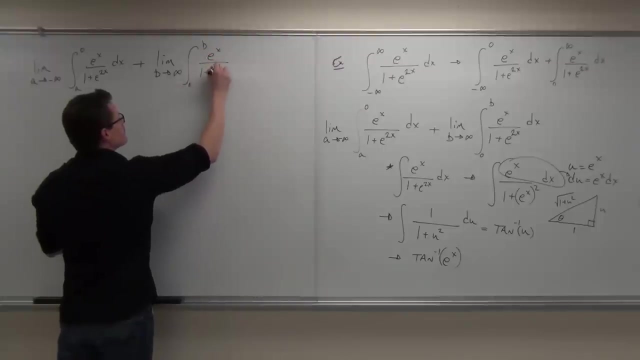 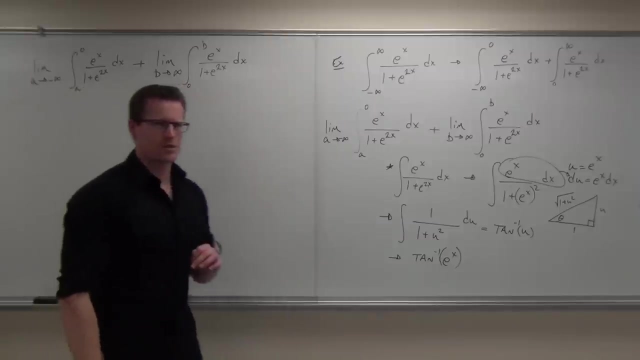 The integral from a to 0,, e to the x, 1 plus, e to the 2x, e to the 2x, dx, Big plus limit as b approaches positive infinity 0 to b of the same integrand You guys okay with that so far. 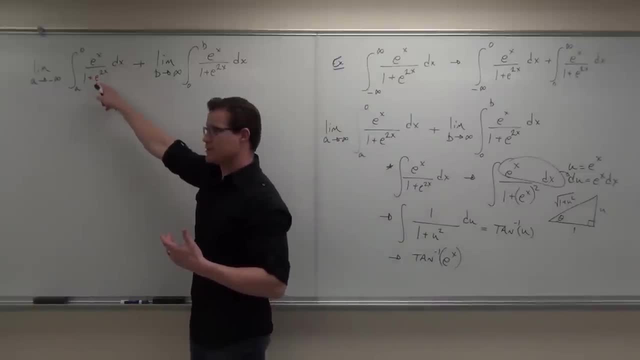 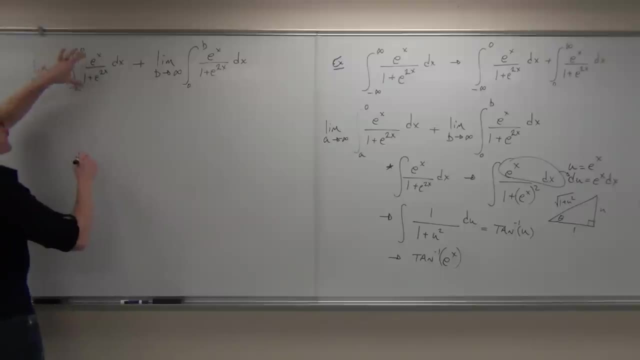 Now we've already done the integral of e to the x over 1 plus e to the 2x. How much did this integral give us? So let's just change those. Let's change those parts. So if I know that the integral of e to the x over 1 plus e to the 2x is actually tan inverse of e to the x, which it is, 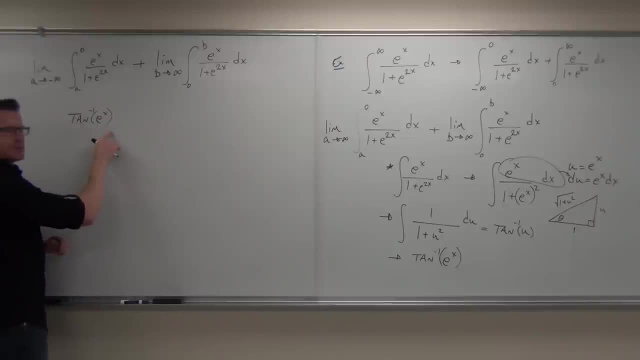 Can you tell me where I'll be evaluating this thing from a to 0.. Sure, Is that pretty straightforward to you guys? To me it makes perfect sense. I want to make sure it makes perfect sense to you. So we say, hey, this integral is this thing. 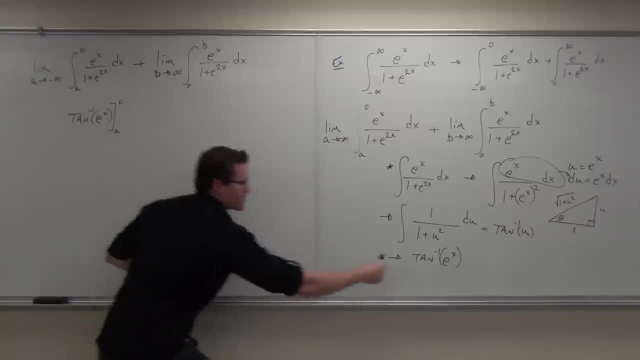 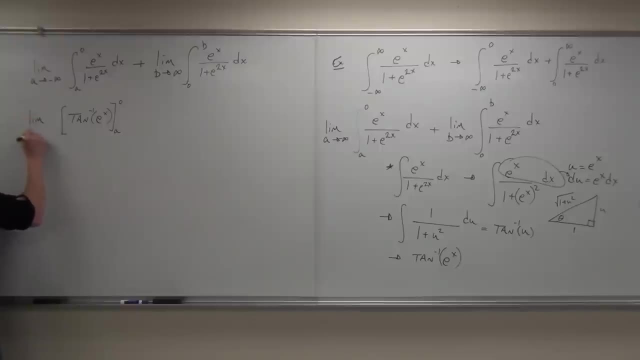 Therefore, if I want to evaluate this integral from a to 0, I just evaluate this thing from a to 0.. From a to 0.. Now, I can't forget what The limit, The plus, yes, but I also can't forget this limit. 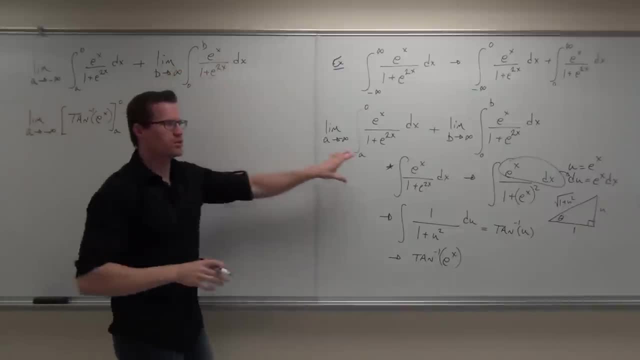 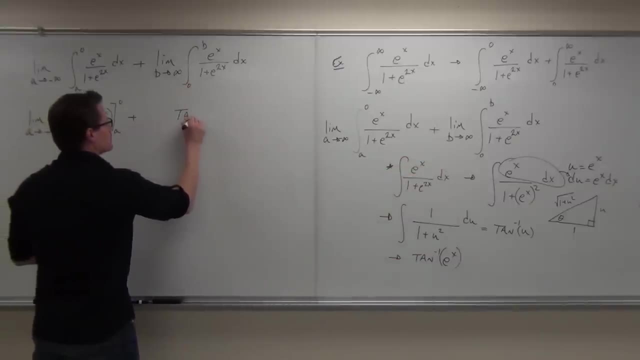 Plus. Now I get the same integral, which is why I'm only going to do it once. It's silly. if you do it twice, It's the same thing. This integral is also tan inverse of e to the x. I'm going to evaluate that from where to where, please. 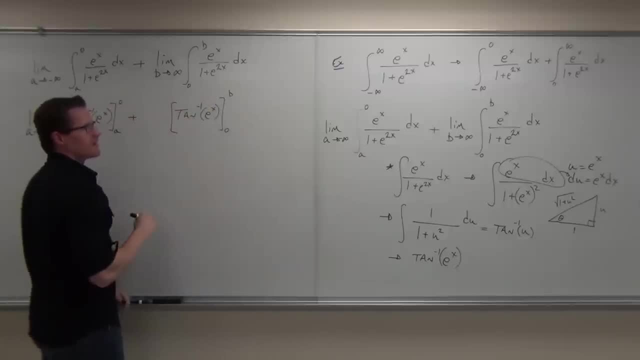 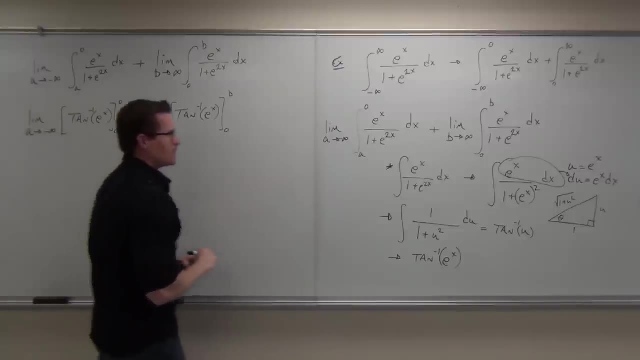 From 0 to b, And I'm not going to forget the. There's only one right answer here: Limit, Limit As b approaches infinity. Okay, what I want to know is: can you make the jump from doing our integral here to evaluate our integrals here? 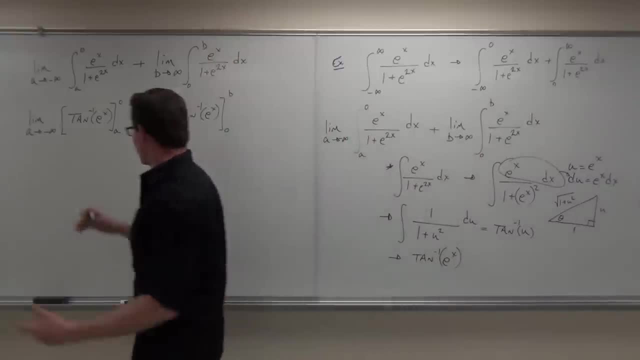 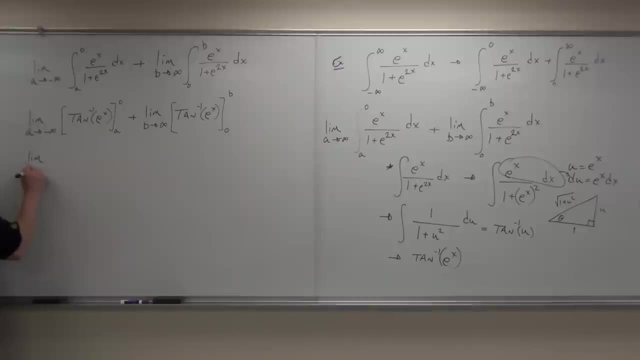 Show me if you can make the jump. Okay, what do we do now? So are we still going to have limits? Yes, Right now. Yes, Yes, Have you evaluated the limit yet? No, Right now. what we're doing is we're. 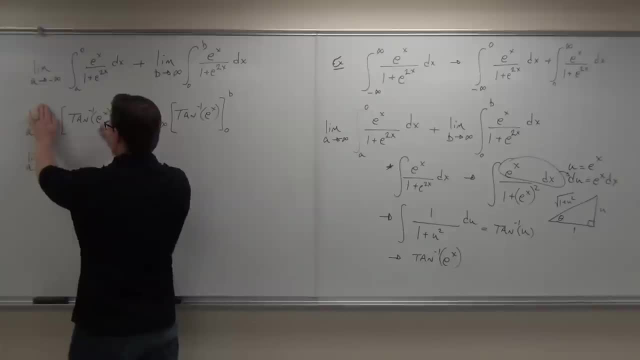 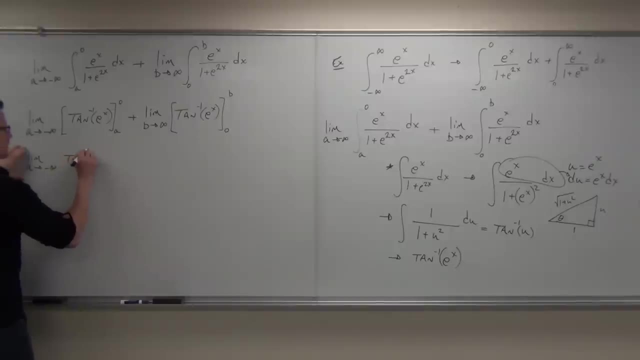 Look at it. Look at it: If I didn't have this limit, I'd still have to evaluate, wouldn't I? Because you haven't done the limit yet. So I'd still be plugging numbers in. So I'd have tan inverse of e to. 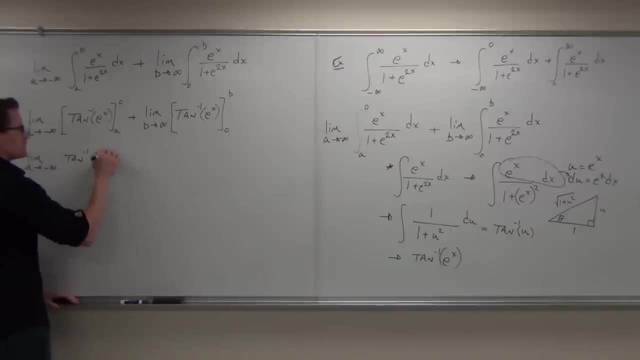 What comes first, the a or the 0? The 0.. The 0 comes first, Minus tan inverse of. That's very common for people to make that mistake. It really is. They go. oh well, 0 always comes. 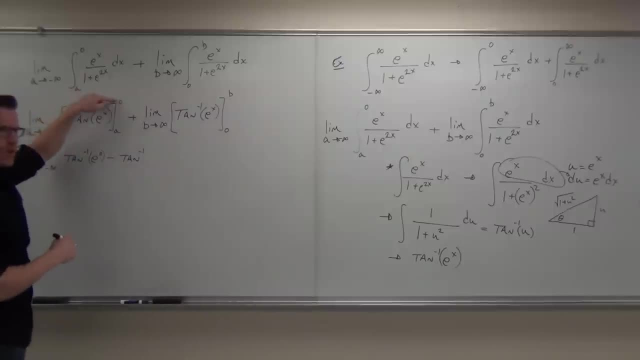 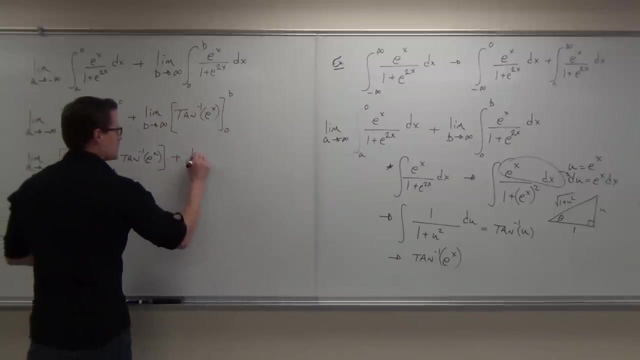 No, no, no. The top bound, Your b, always gets evaluated first And then you do your lower bound. So if you guys feel okay with that one, Are you sure Okay? so here's one Big plus limit as b approaches infinity. 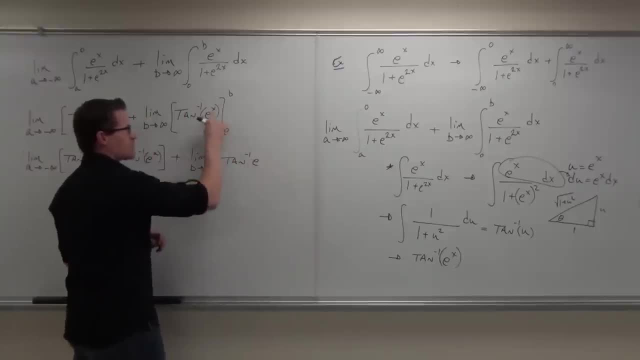 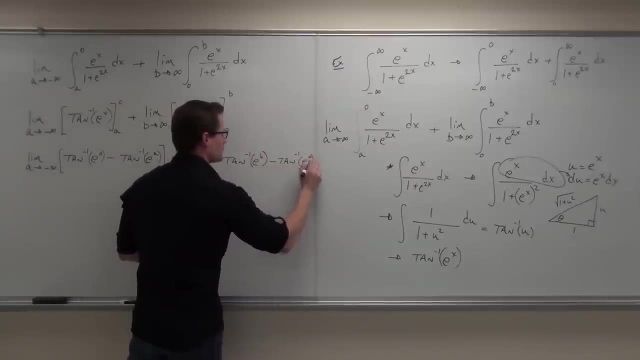 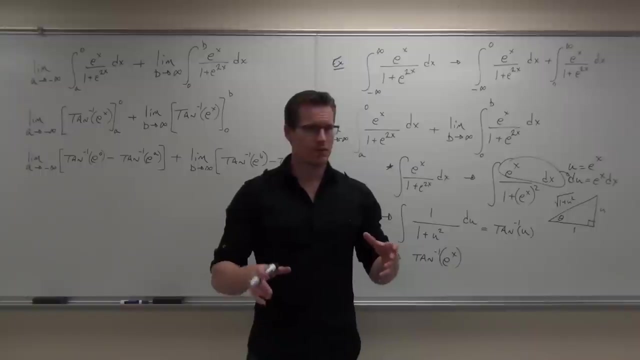 Tan inverse. Let's try this again: Tan inverse of e to Would it be 0 first, or b first, b Minus tan inverse of e to the 0.. Now, are you guys okay with that one? Notice why we still have our limits. 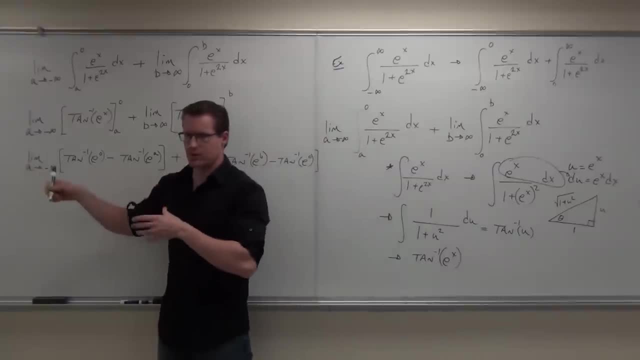 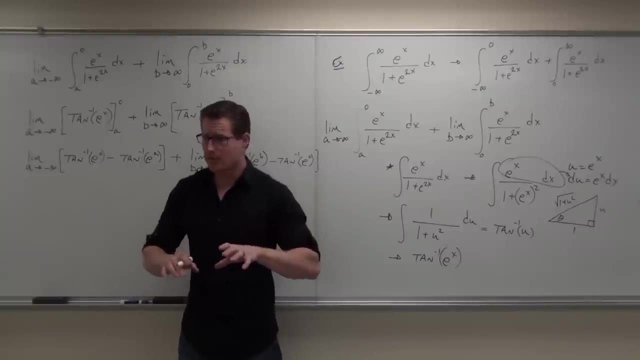 Have you let a go to negative infinity yet. That's why you still have your limit. Now we get to let a go to negative infinity. We let b go to positive infinity, So we're going to stop writing limits right now. 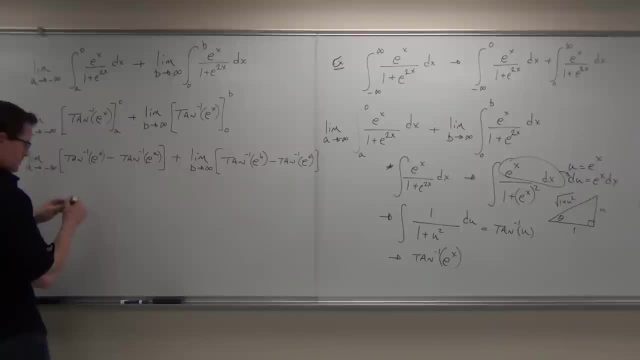 Let's think about this: How much is e to the 0?? Hello, 1.. So this is 1.. How much is e to the a as a approaches negative infinity, 0.. Very good, This is 0.. 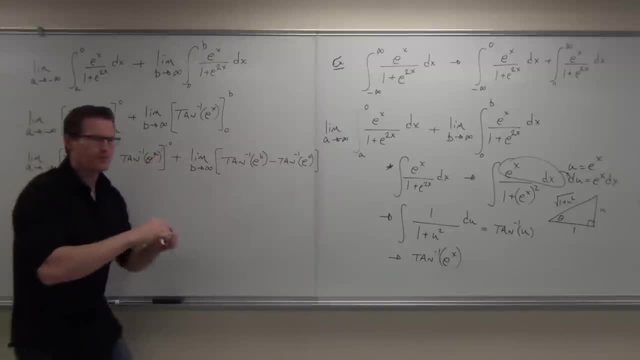 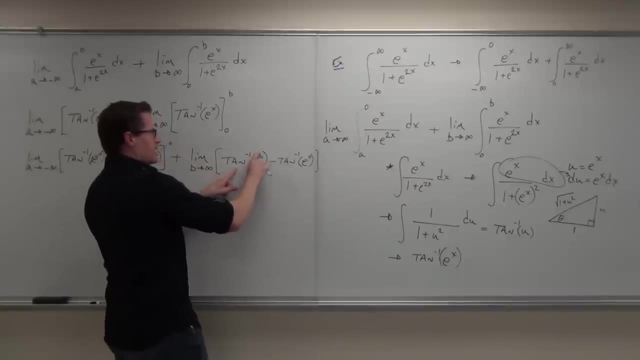 As a goes to negative infinity, e to the a. This is e to the negative infinity. e to the x goes like this: So, as negative infinity, we're going to 0.. How about e to the b, as b goes to infinity? 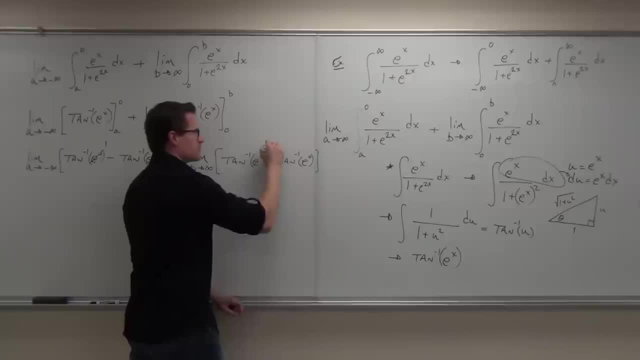 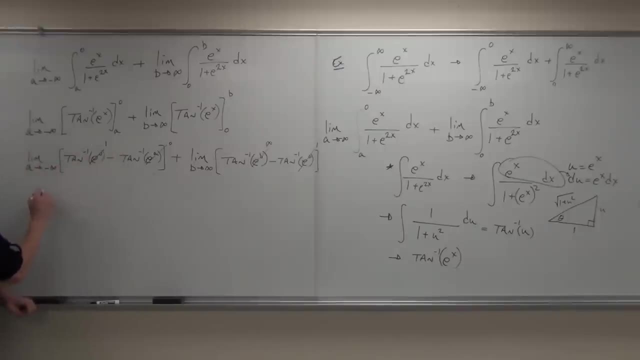 How much is that going to be? Infinity? Very good. e to the infinity is infinity. How about e to the 0, again 1.. So now that I've let these go to their appropriate places, I stop writing the limit. 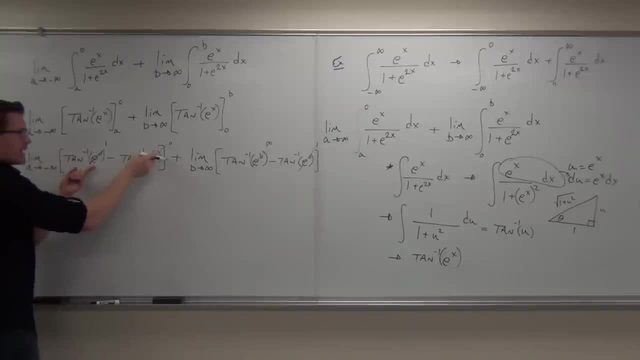 This was a value in limit. I said, hey, look at that. e to the a, as a goes to negative infinity, that's 0. And this one's going to be infinity. So we have tan inverse of 1 minus tan inverse of 0. 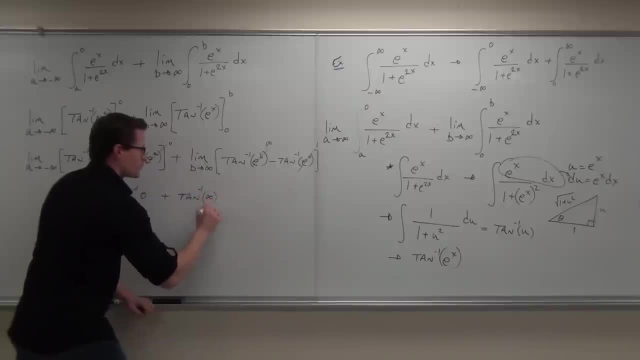 plus tan inverse of infinity- That looks a little weird to write, but we'll write it- Minus tan inverse of 1.. Now we've got to be good at tan inverse. Let's see what happens. We're almost done with this thing. 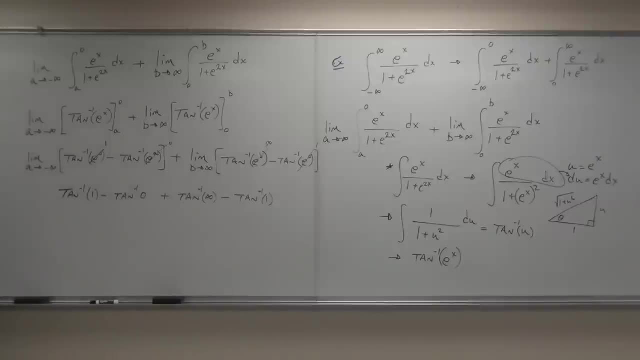 How much is tan inverse of 1? Pi over 4.. Pi over 4.. Very good, So this piece pi over 4, says tan of pi over 4 gives you 1. Therefore, tan inverse of 1 is pi over 4.. 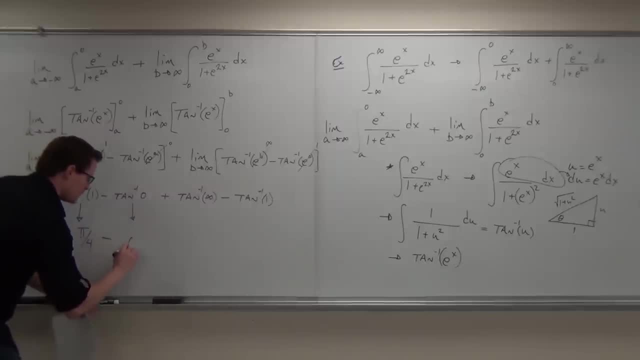 How about tan inverse of 0? 0.. 0.. Tangent of 0 gives you 0.. Therefore, tan inverse of 0 gives you 0.. Plus how much? oh, this is an important one- How much is tan inverse of infinity? 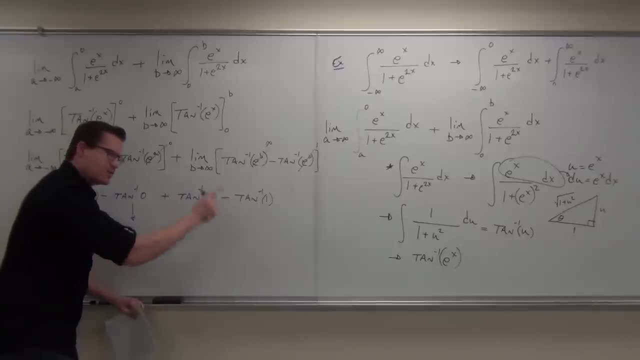 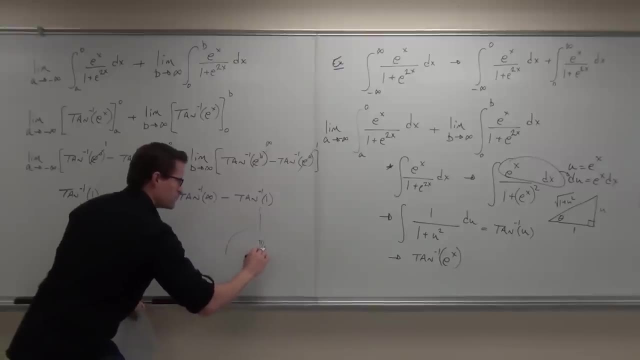 So basically, tangent of what value will give you infinity? 9. Well, pi over 2, will Remember. tangent looks like this at pi over 2.. That make sense. So if tangent of pi over 2 is asymptotic, then we have an infinity. 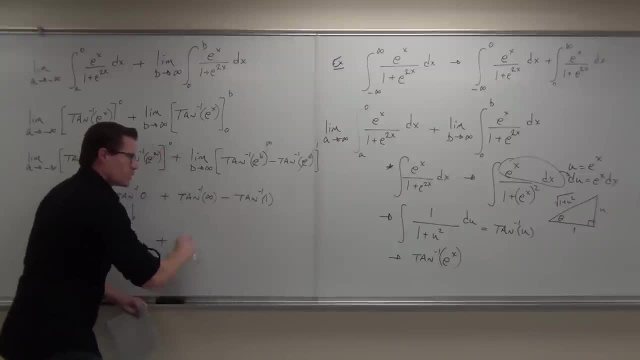 So therefore, tan inverse of infinity is pi over 2.. It's a little weird because we can't actually plug in infinity, but we think of it like that. We think of how can I get really close to infinity with a tan inverse? 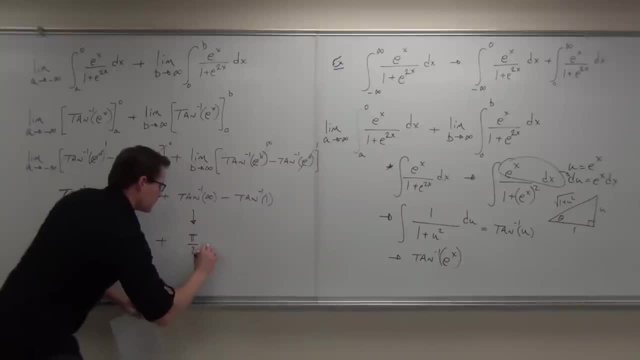 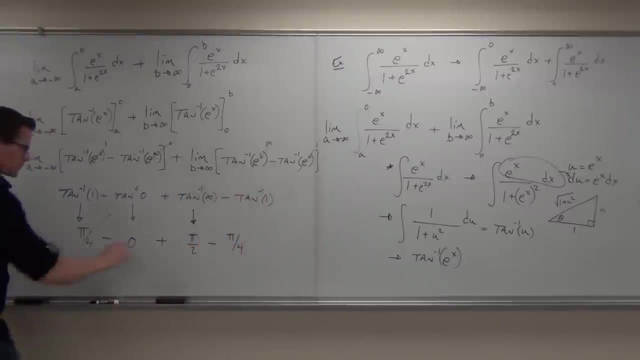 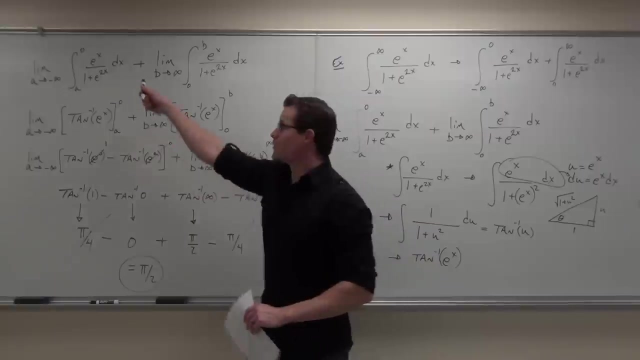 It's pi over 2.. We already did this one: It's pi over 4.. What's our final answer? What floors me? what's really cool is that we have this function right with e to the x in there. 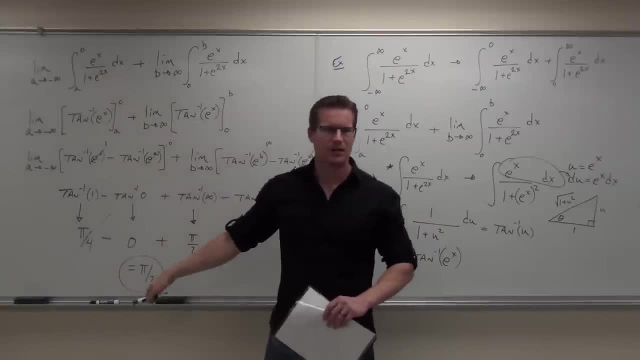 e to the x over 1, plus e to the 2x, and somehow we get a pi over 2 out of that thing as a solid area. Isn't that kind of cool. Yes, So, Spencer, that made sense to you. 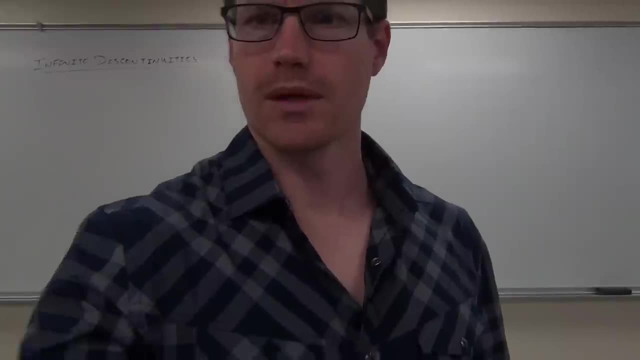 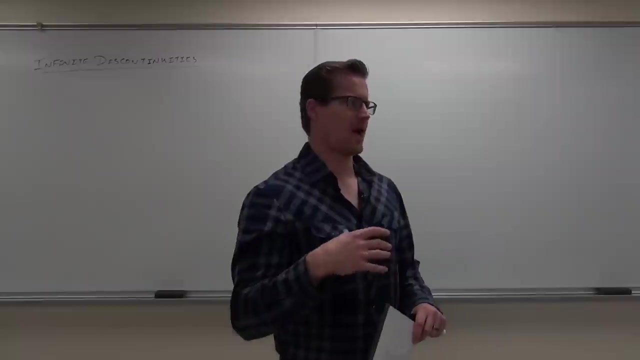 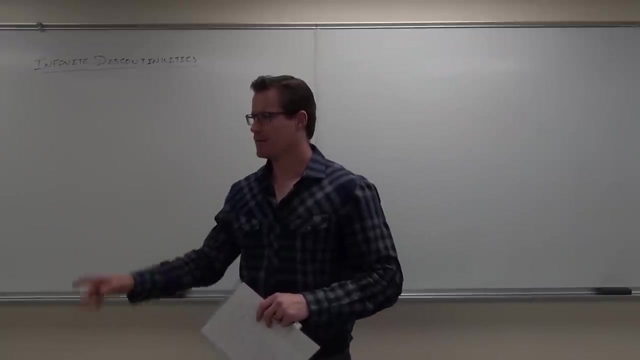 Good deal, All right. so the last little bit that we've got to cover in this section is, instead of an infinite interval, we've got to find out what happens with an infinite discontinuity. What that means is that, instead of going from like negative infinity to a number, 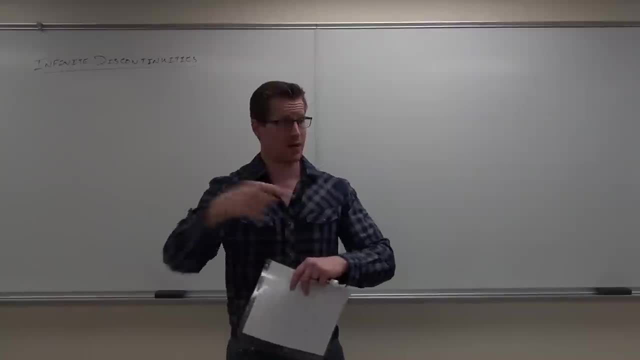 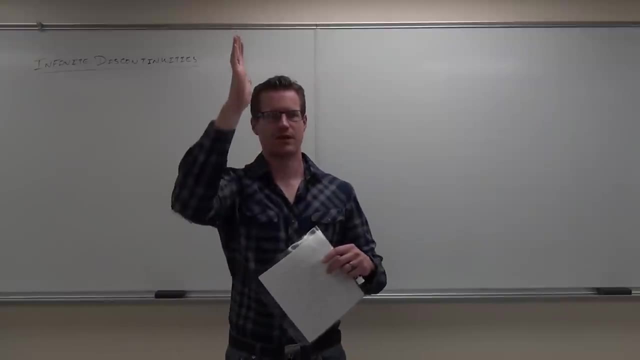 or a number to infinity, or even remember the last time we had negative infinity to a positive infinity somewhere within our interval. whatever it is, our function's not bounded. What that means is that we're going to infinity or negative infinity along the y-axis. 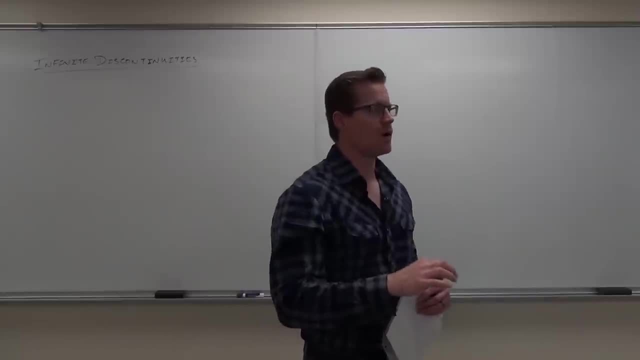 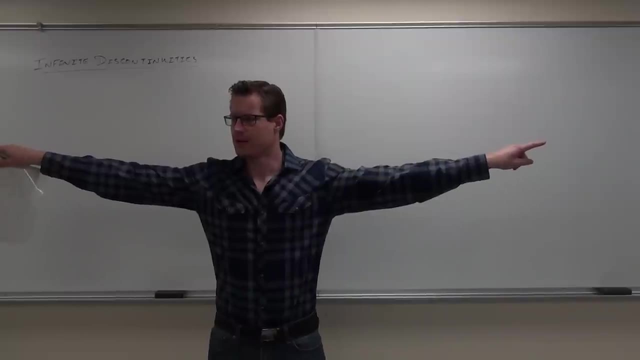 So basically, we just have an asymptote somewhere along the interval on which we're trying to integrate. Do you guys see the difference in the idea? Yeah, Infinite intervals go this way for infinity. Infinite discontinuities go this way to infinity. 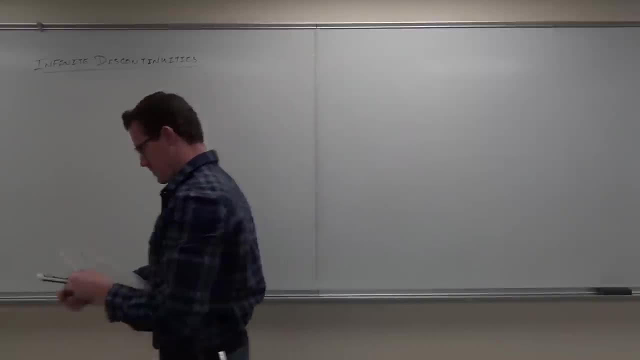 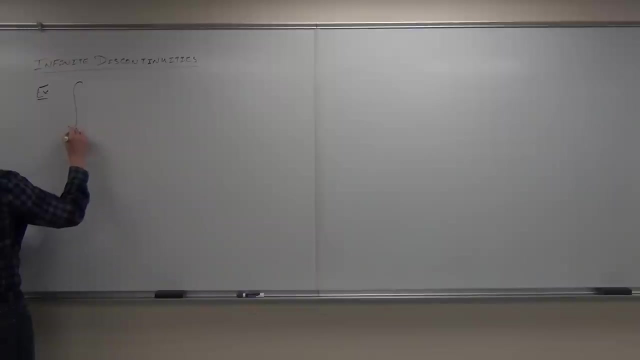 The function is actually going to infinity. Let me give you an example and it's going to clear everything up. So first example: Let's say I want to go from 0 to 9, find the area of the following function from 0 to 9.. 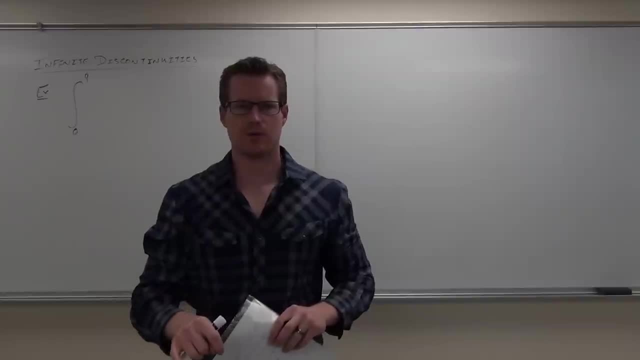 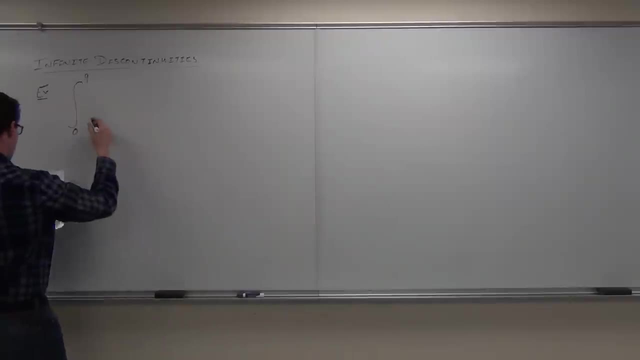 Now right, there is that an infinite interval or a finite interval, Finite Sure, that's great. So we don't have to worry about the limit of b going to infinity or a going to negative infinity. We're not worried about that. 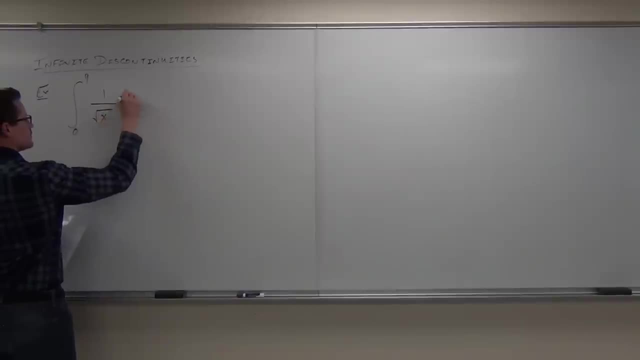 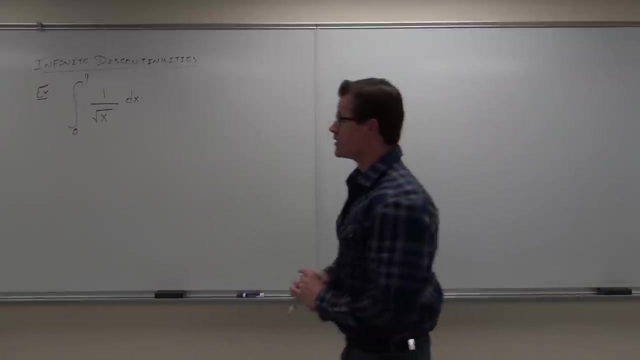 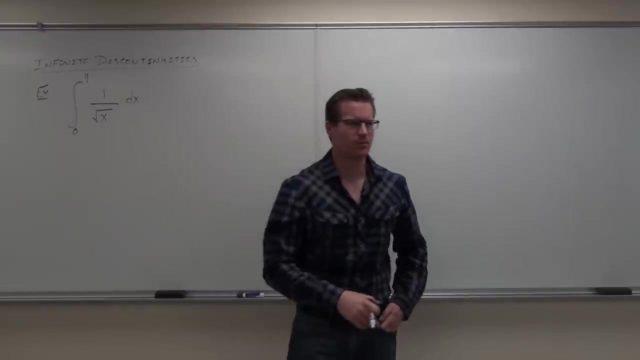 However, remember the first thing I told you to check when you're talking about your definite integrals is: well, look at your bounds of integration and see if your function is defined for that entire interval. Is it defined for our entire interval? No, 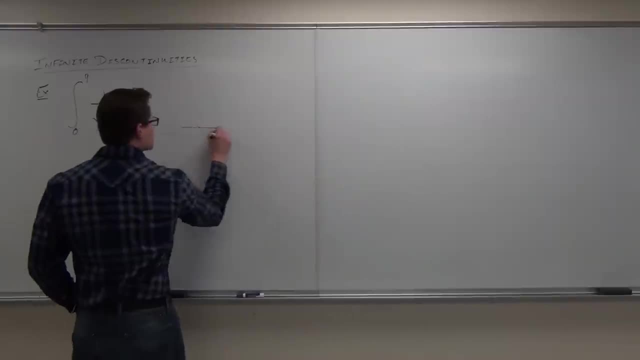 No, In fact, what's happening here with this function is this thing looks a sketch here. looks kind of like this Where, as we go towards infinity- yeah cool, we're going to get you know- smaller and smaller values. 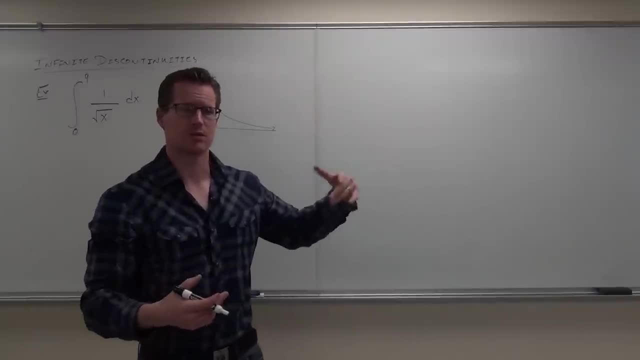 because we have a fraction over a number that's growing. Even though it's a square root, it's still a growing denominator. Does that make sense to you, However, as we get towards 0, what's happening as we get towards 0?? 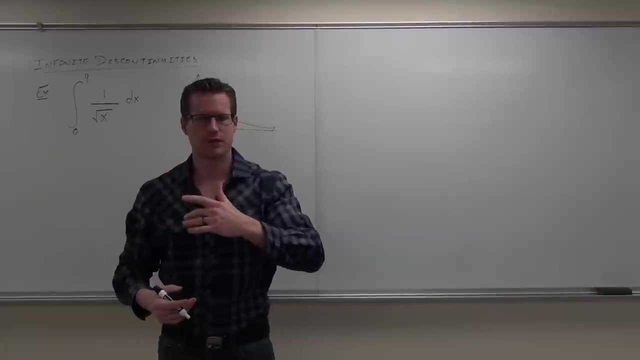 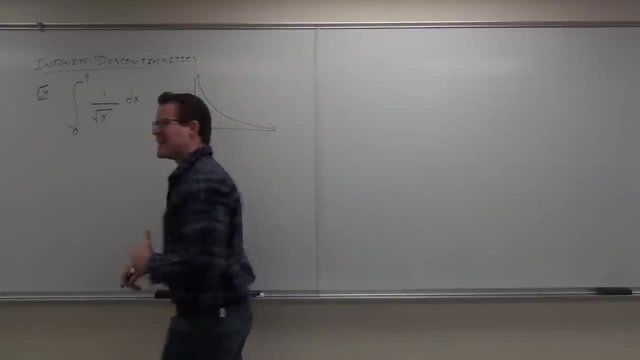 It's going up, It's going towards infinity, because when we're dividing by smaller and smaller numbers, we're getting this away. Well, we've got an undefined zone here And that's an issue. So as we get closer to 0, we have this issue. 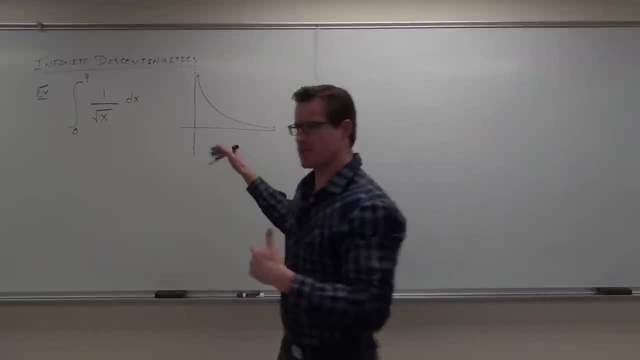 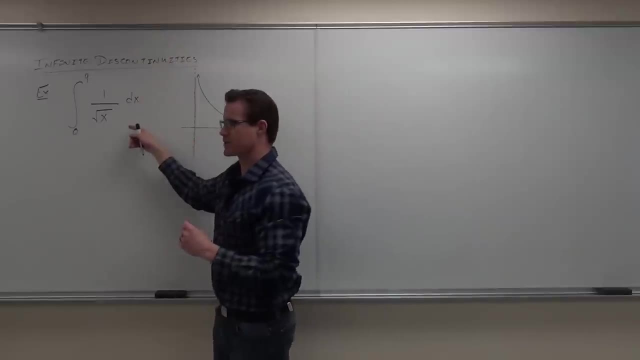 We have what's called an infinite discontinuity. It's not continuous, It's going towards infinity. The function is not bounded. So if I can just be okay with this one, Okay Now on the left side of 0, well, we have nothing, because we can't even plug in negatives, because we've got a square root. 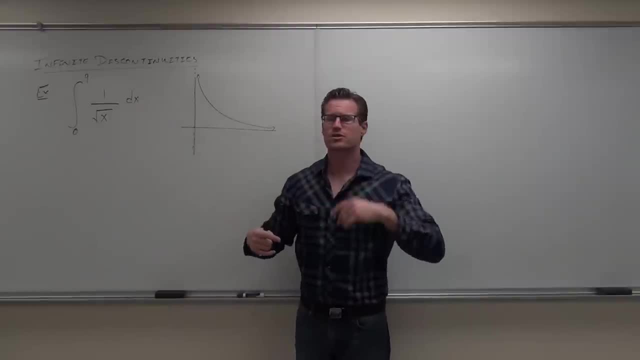 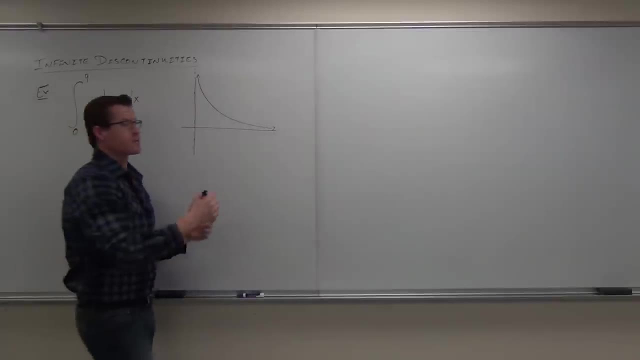 So this is basically what our graph looks like. You got it, Yeah. So here's our idea, Instead of going from 0 to 9,. what's the problem here? Is it the 0 or is it the 9, or is it somewhere between there? 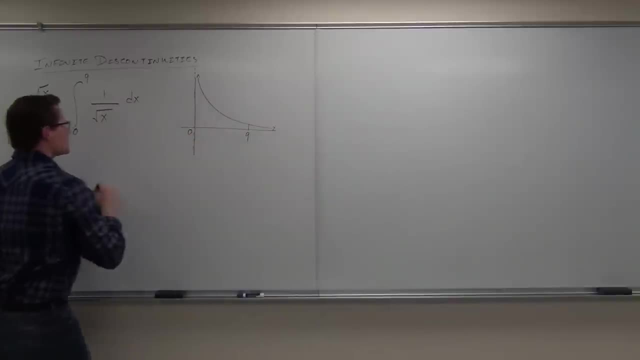 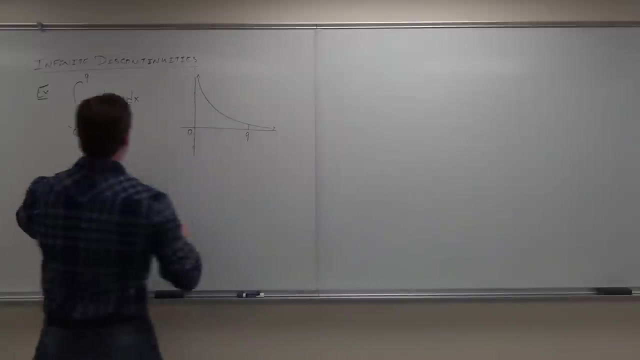 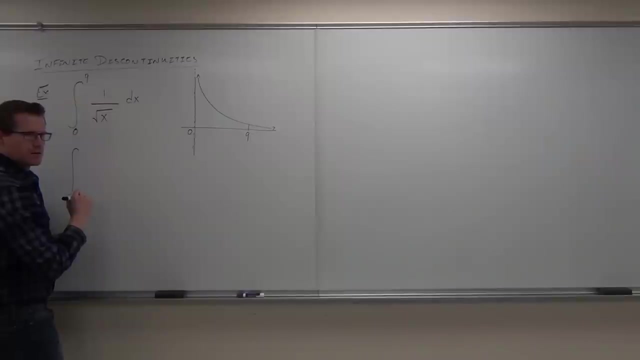 It's the 0.. It's the 0. The 0 is the problem. So tell you what. We're going to use, a very similar idea to what we did last time. Instead of going from 0 to 9, maybe we'll go from. I'm sorry, what was the problem again? 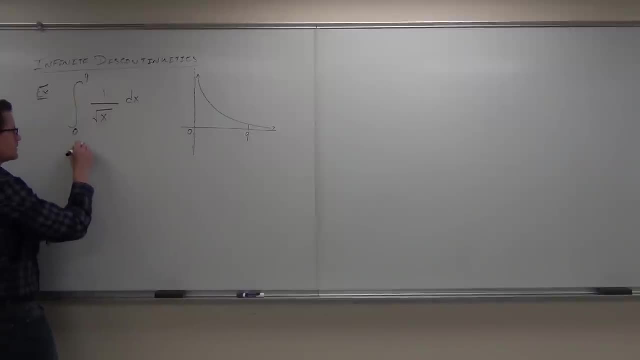 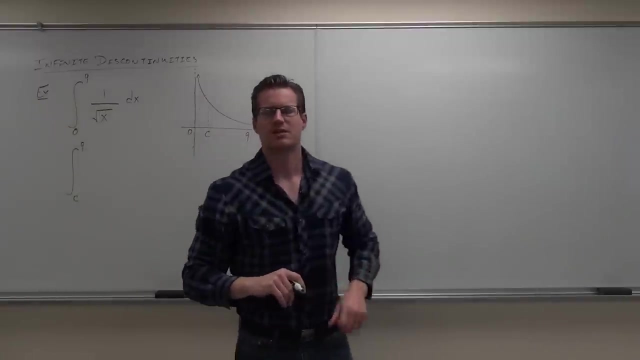 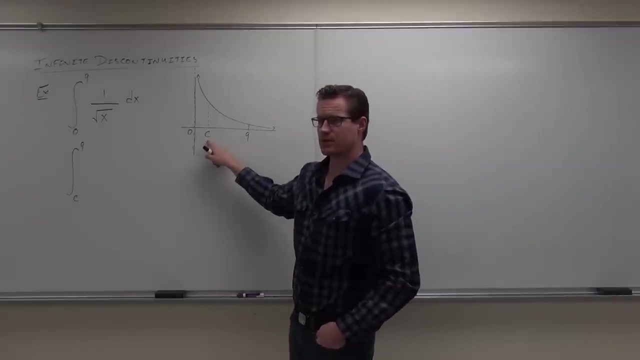 0 is the problem, or 9 is the problem? 0 is the problem. We'll go from C to 9. And we'll make C some intermediate value. Tell me something, Hey you ready? Tell me something. If this was a number like 1, could you integrate this thing very easily. 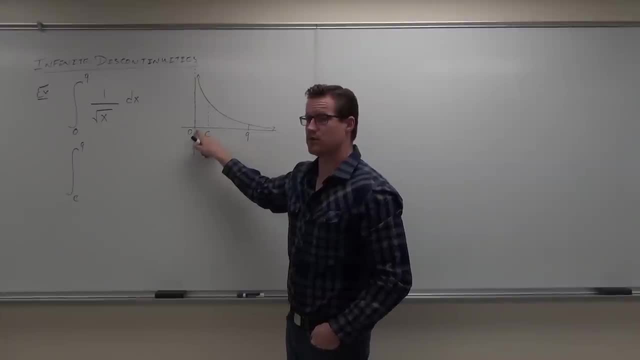 Piece of cake. If it was like 0.01, you could still do it. 0.0001,, you could still do it 0,, not so much. We're going to have a different idea. So it's really similar to the idea of: well, we can't actually plug in infinity, but we can plug in a number, right? 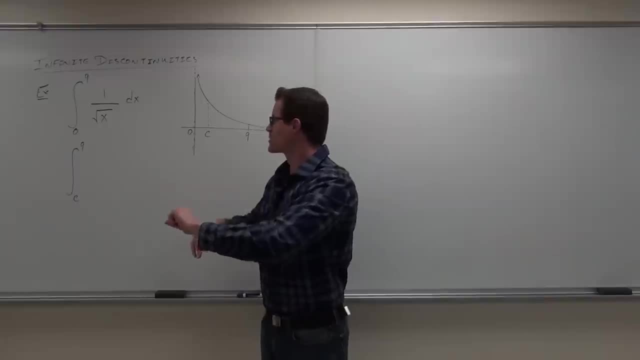 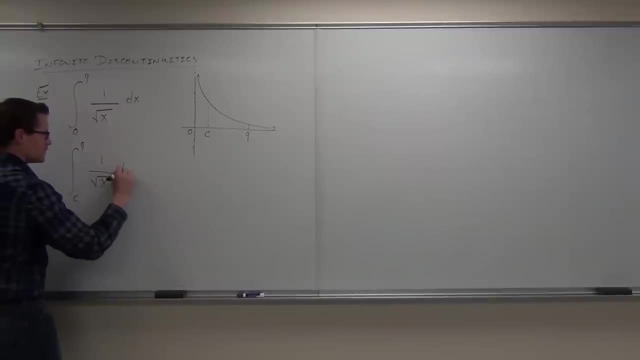 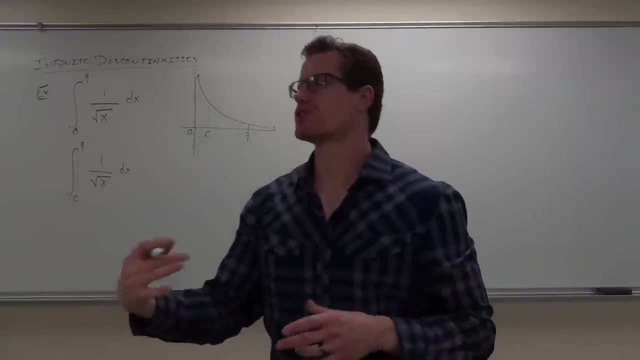 And then let that number go to infinity with a limit. So the idea here is all right. well, let's call it not 0.. Let's call it C. Now the question is, what do we want to happen After we're done with this thing? what do we want to happen to our C? 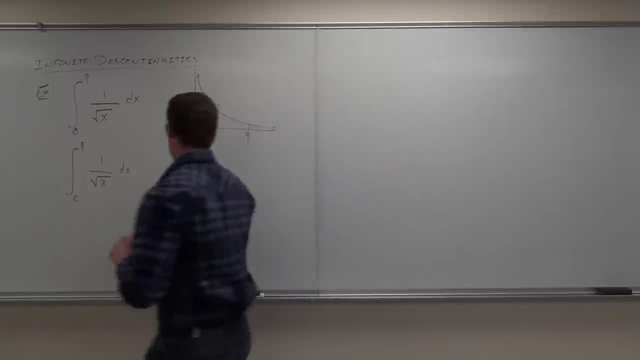 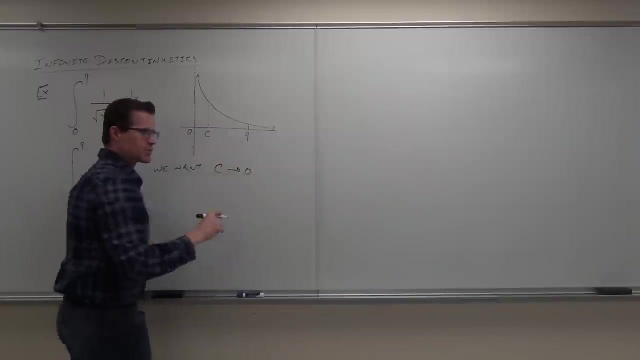 Where is our C supposed to go? Okay, our C. So we want our C to approach 0.. Yeah, that's right, We want C to approach 0.. Now, there's a problem with this, And this is why we talked about where the functions to find begin with. 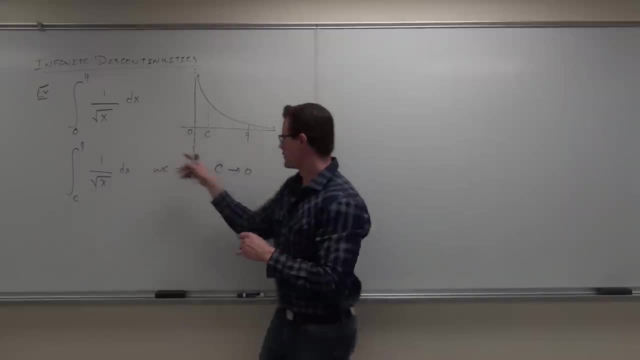 Is there any function on the left-hand side Or is there a function on the right-hand side of our 0?? So what this says, if you remember anything about limits, what approaches 0 means is that the function does this from both sides. 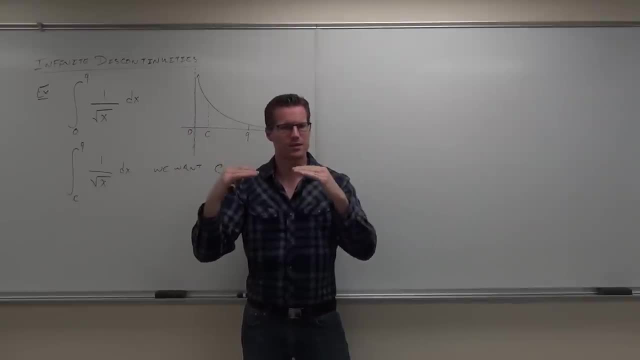 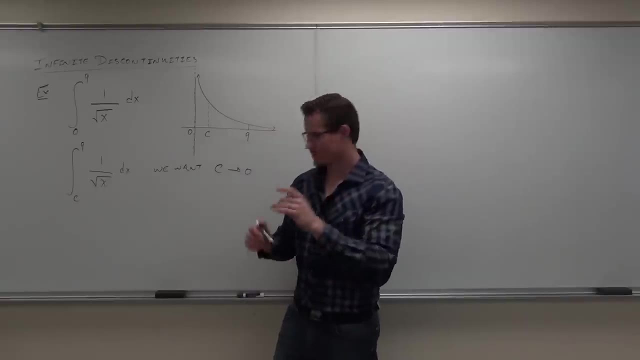 Remember that We have to make this not a both-sided limit but a one-sided limit, So we're going to have to approach 0 from a specific side, From the right side, From the right side. So would you use a plus or minus? 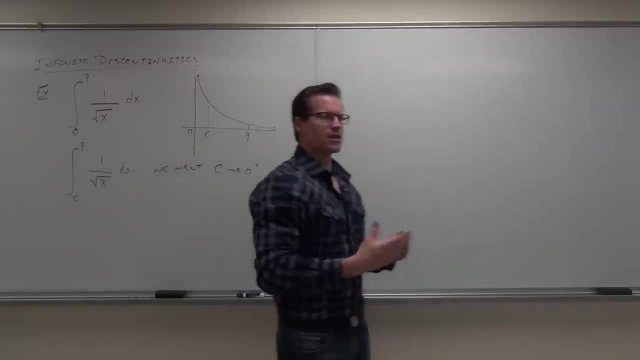 Plus Good. What we want is: let me recap this real quick so we understand everything about it, and then I'm going to give you the definition for it and we'll be good to go. The idea is well, you know what? 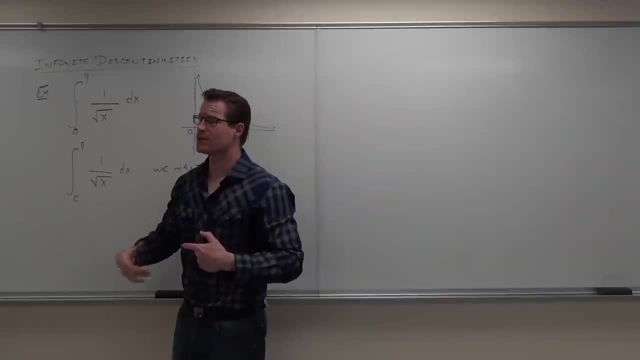 We're going to have a number 9.. That's fantastic, but our function's not defined for the whole thing. We have an infinite discontinuity. Wherever that happens, are you listening? Wherever that happens, change it to a C. 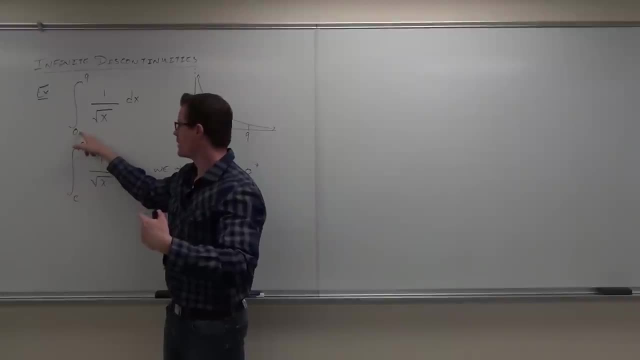 What we're saying is that, okay, I can't define the 0 here, It's undefined, So let's call it C. That way I can even do my integral. We're basically changing this to a definite integral right now, from a number to 9.. 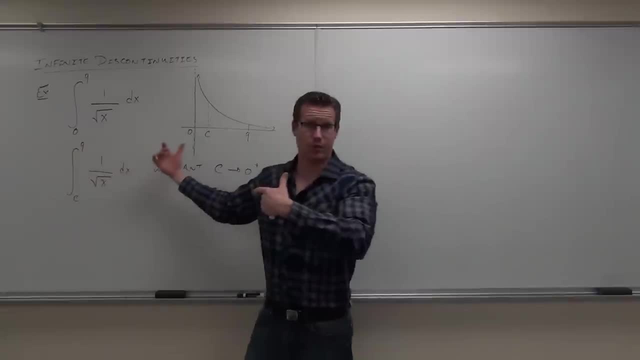 No problem. Can't you do a definite integral from a number to 9?? We just talked about how we could. After we're all done, then we'll say: well, what do we want to happen to our C? What happens there? 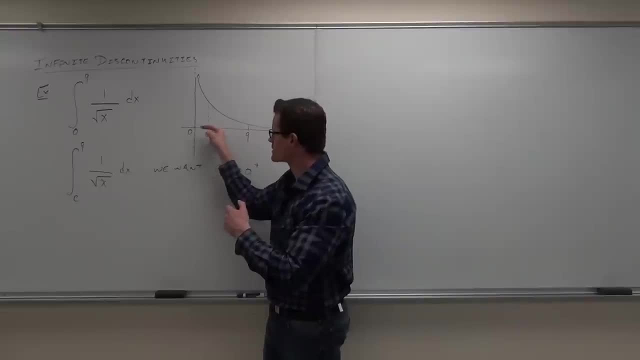 We don't want the C to be here, We want our C to be there. We're going to let that C goes to 0 from the right-hand side. This is the idea. Should I feel? okay with the idea? All right. 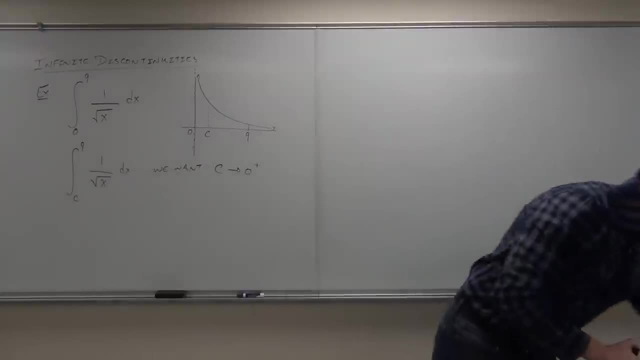 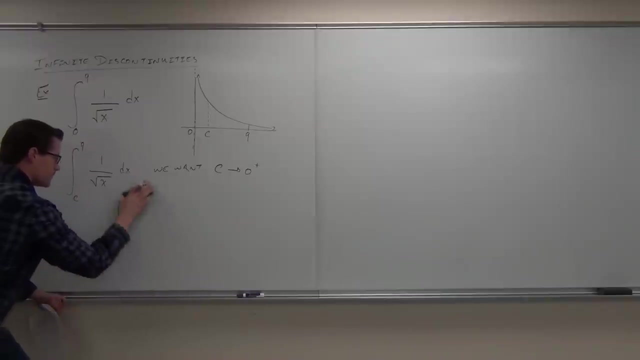 So basically, this is where we get our limit again, So we'll go all right. fantastic, I can do an integral from C to 9.. I just have to let the C approach 0.. 0 from the right-hand side of the same function. 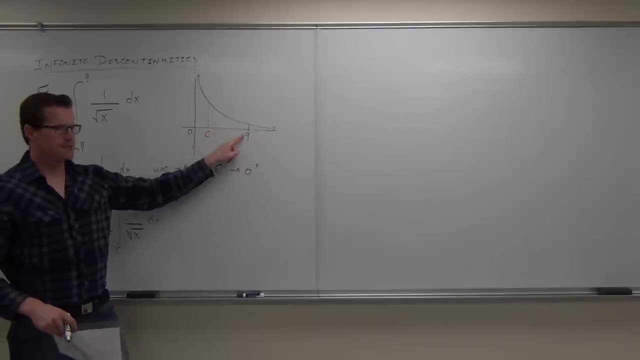 So we're saying 0 to 9? No, no, no, We'll go C to 9.. That's a definite integral. Fundamental Theorem of Calculus says we can evaluate definite integrals. That's why we're doing this right now. 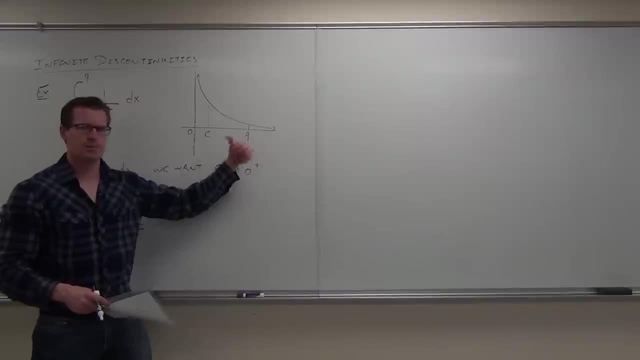 So we go, okay, C to 9.. Cool deal, Do the integral plug in 9,, plug in C, subtract the two values and then, at the very end, go wait a minute. let's trick it again. Let's say no, no, I don't want just C, a finite number. 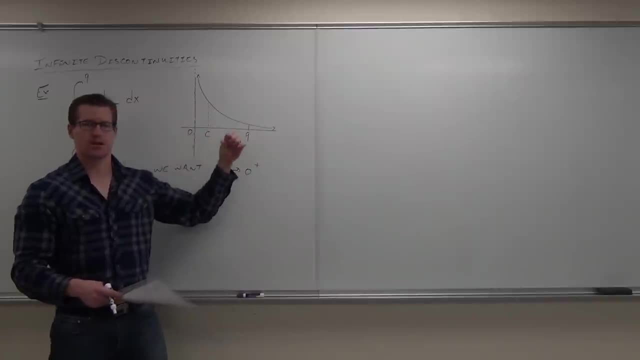 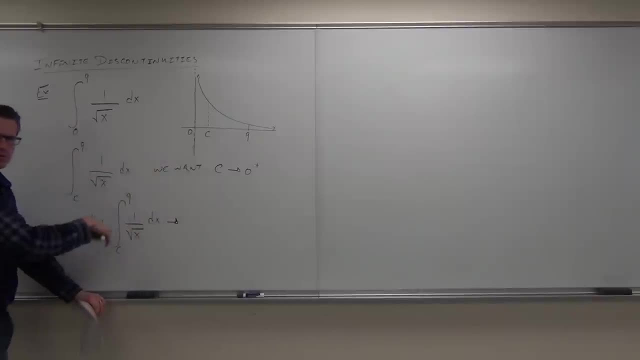 It's going to be a limit again. Can you guys evaluate this integral? What would you do with this? We could make it a 1.. Yeah, So C goes to 0 from the right. Remember we still have to write that. 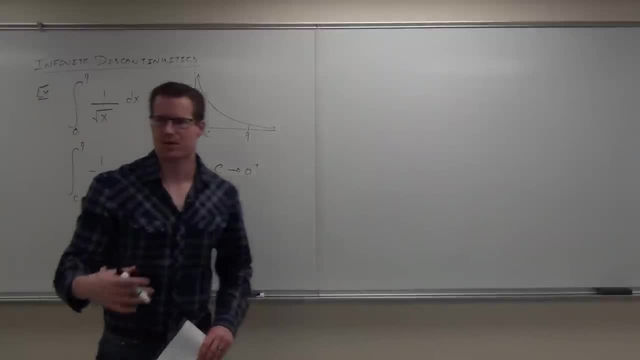 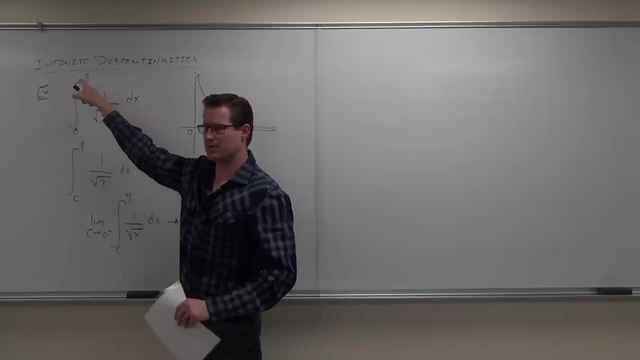 C to 9.. By the way, if you didn't catch where the C is coming from, A is typically called a lower limit, B is typically called a lower bound. B is your upper bound. So if we had negative infinity, we'd call that our A. 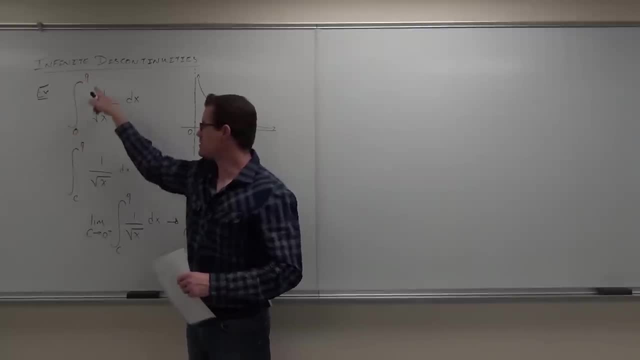 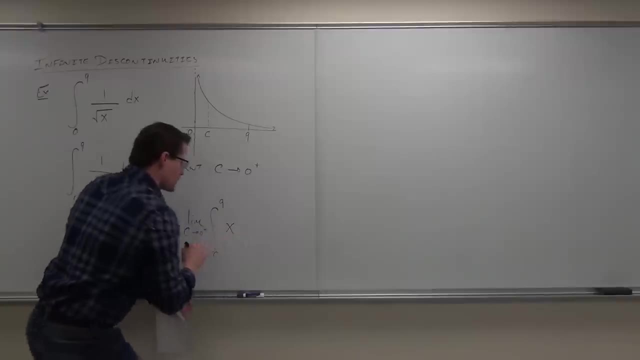 Our positive infinity would be our B. Anywhere in between these two numbers is typically a- C, So that's where the C is coming from. Okay, so you all said that this should be X to the. what am I going to do here? 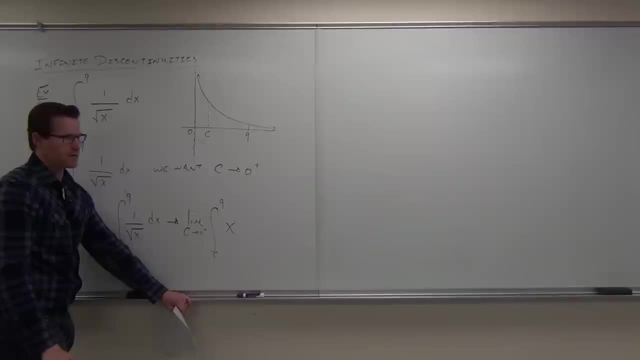 X to the what Negative 1 half. Oh wait, I'm sorry. 1 half or negative 1 half, Negative 1 half. Good, I'd move this up. That'd be X to the negative 1 half. 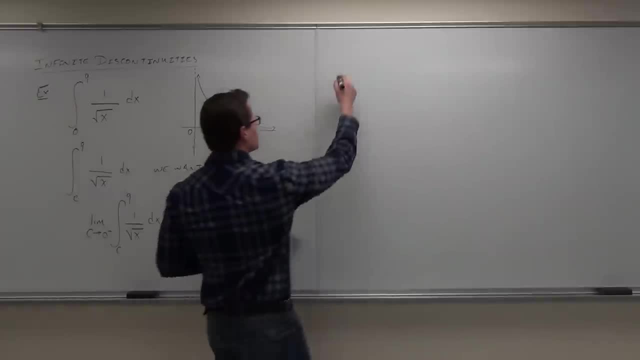 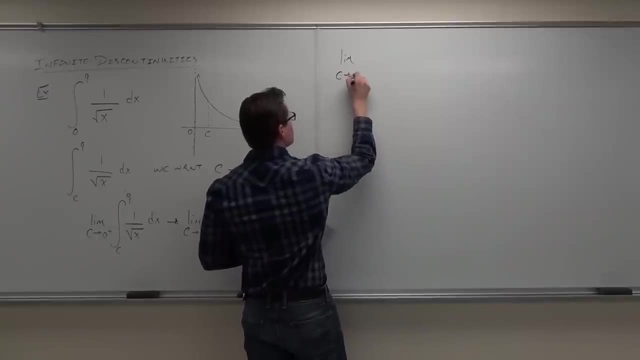 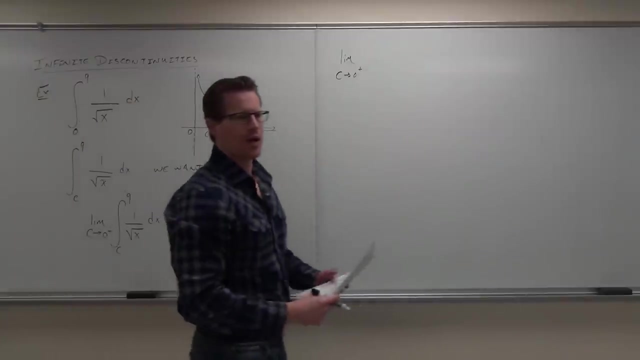 DX: Cool deal, Let's keep going. So this will be our limit. as C approaches, 0 from the right, Let's go ahead. let's do our integral. What's the integral of X to the negative 1 half? Tell me that one. 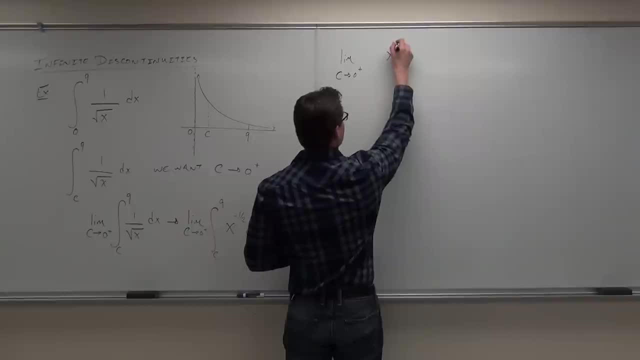 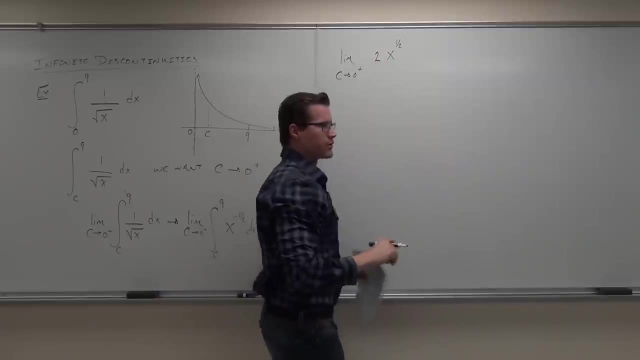 X to the 1 half. Okay, X to the 1 half. I like it. 2.. Over 1 half, So basically 2.. So I'm actually okay with that integral. I'm going to cut off the warning now. 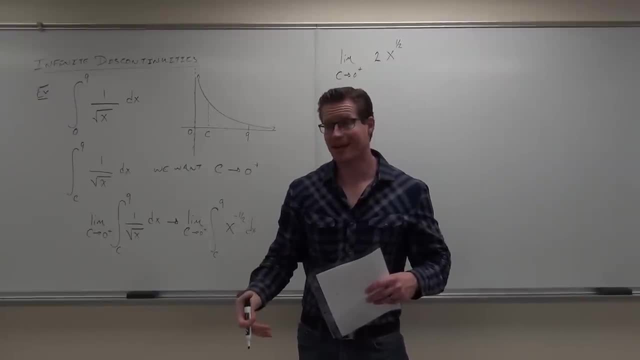 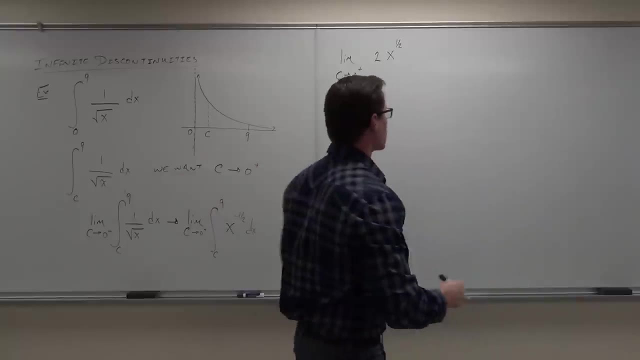 I'm going to go fast through a lot of these integrals, because the idea is no longer, hey, can we do integrals, It's let's look at how to do these improper integrals. Does that make sense to you? So the actual integration: we're going to go a little bit quicker. 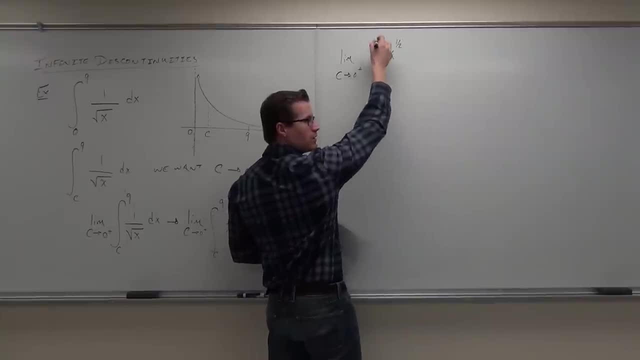 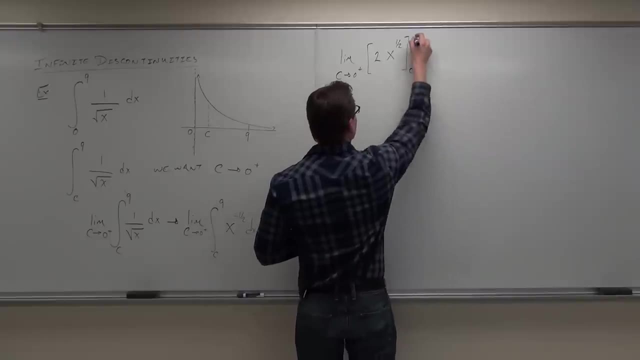 Now, do I still have an integration symbol here? No, You've already done the integral, So all we're doing now is evaluating. Where are we evaluating? from C to the negative 1 half, Okay, which way? C to the negative 1 half. 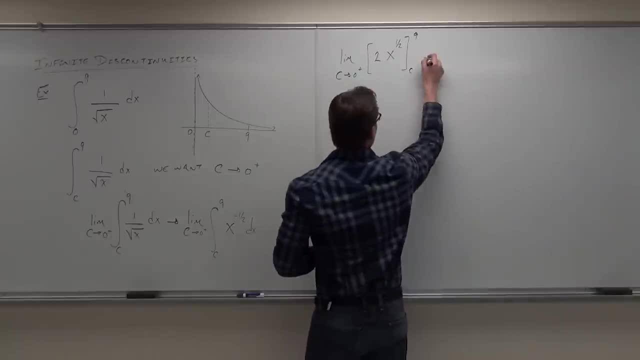 9 to C or C to the negative 1 half, C to the negative 1 half. Which one do we plug in first? C to the negative 1 half. So this would be the limit as C approaches 0 from the right-hand side. 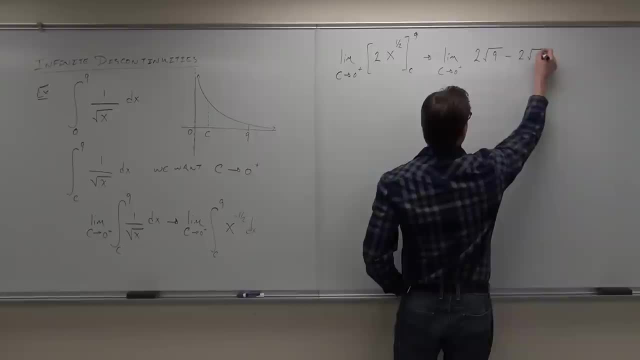 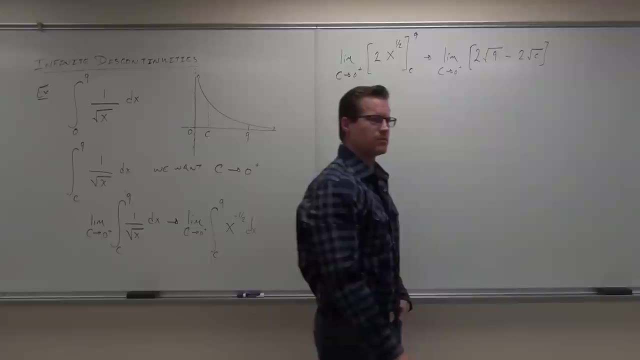 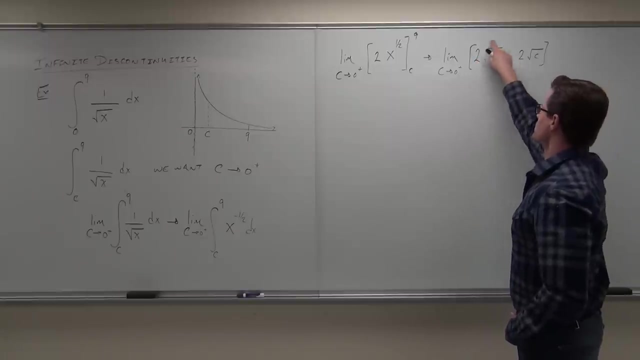 2 square root of 9 minus 2 square root of C. Still okay so far. Let's talk about these things. Let's talk about what happens as C approaches 0.. What's going to happen to this part? How much is that going to go to? 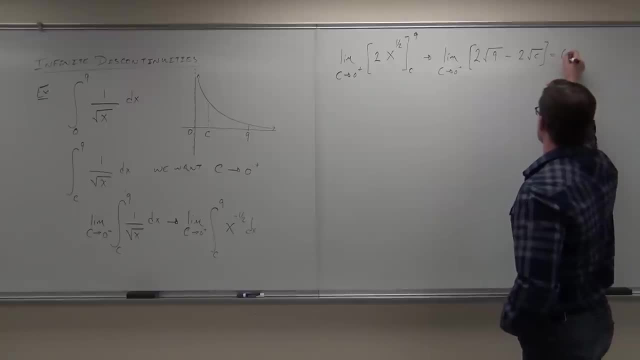 6 of it. Sure, This is 3.. That's 2.. So we're going to get 6.. Notice how we're stopping writing the limit Once we evaluate the limit, but before that we have to have it every single time. 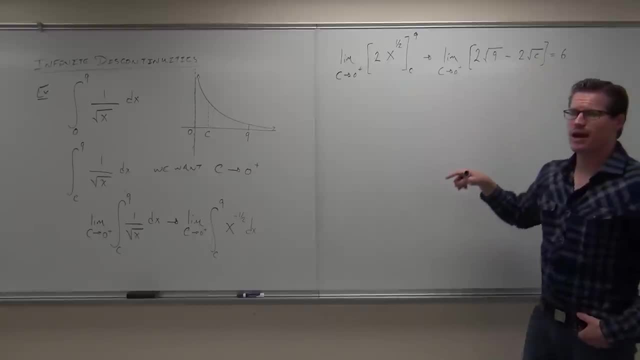 Now what happens to the square root of C as C approaches 0?? Notice, we don't have a two-sided limit here, which is why we had to go from the right-hand side only. It doesn't exist for both sides. So just think about what happens. 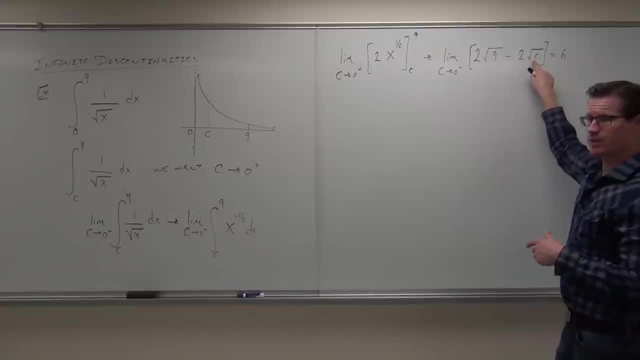 What happens to a square root of a number as that number gets really, really close to 0?? It gets really close to 0.. Does that make sense to you? If you plugged in 0, you'd get 0. So we have minus 0.. 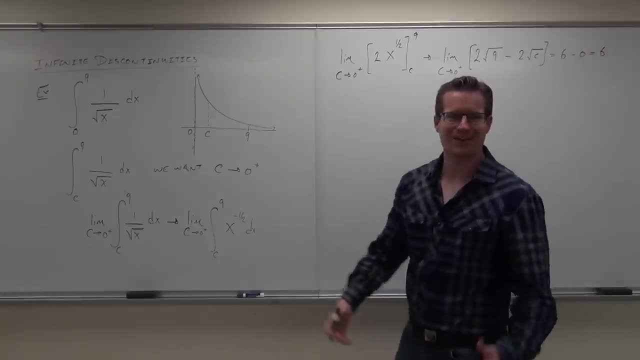 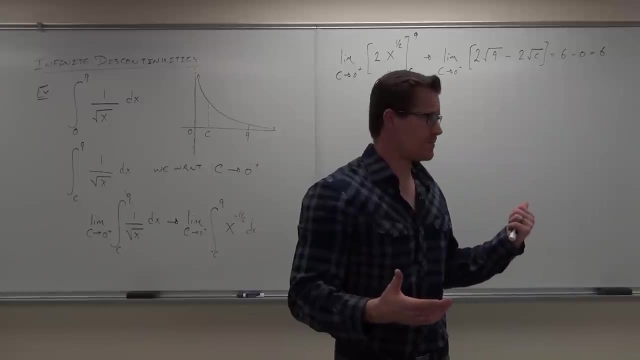 Therefore, what's really interesting- I don't know why it's so cool to me, but it's so cool to me- It says that what's an integral even mean? So this is a definite integral right Between 0 and 9, of something that's not even defined as 0.. 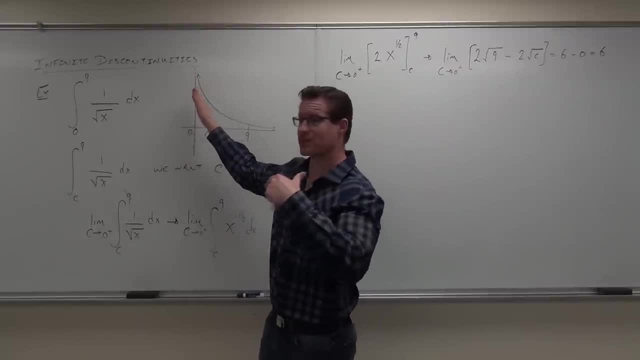 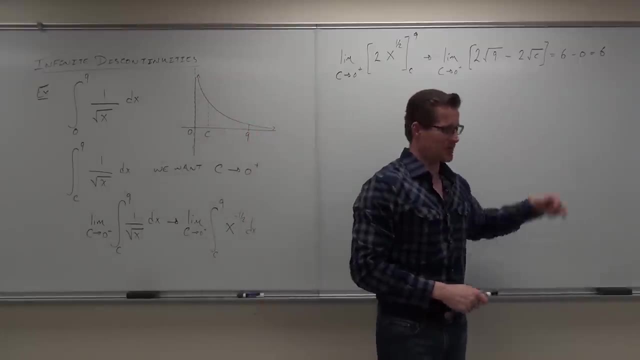 Yet what happens is that if I have the area, because of this, because of our limit idea, the area under this curve from 0 to 9 is equal to very cool idea, Very cool. So it makes me feel all right with this. 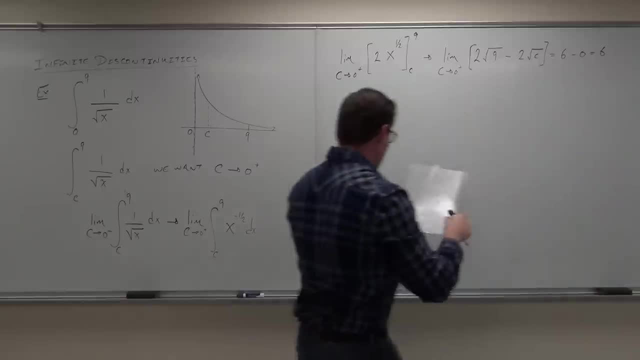 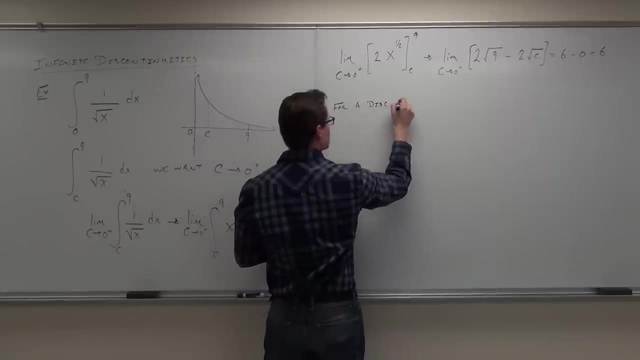 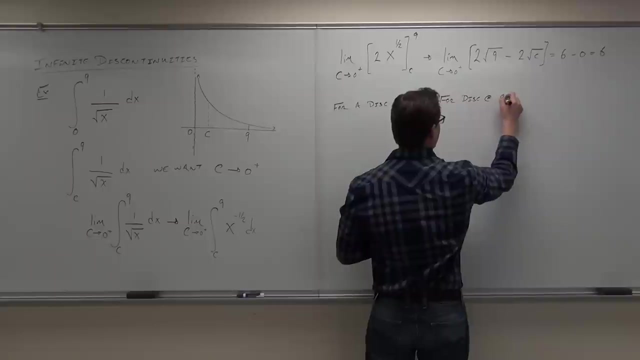 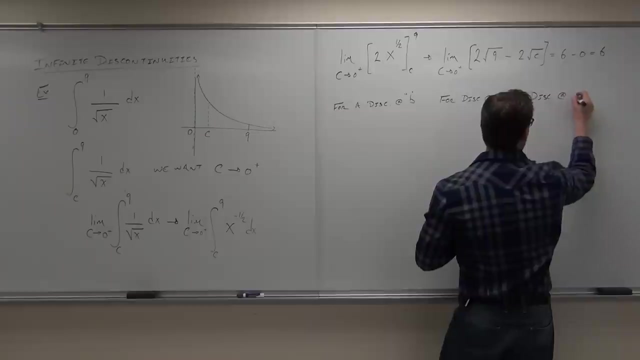 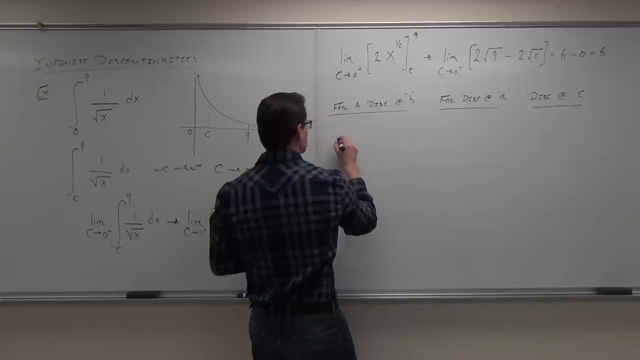 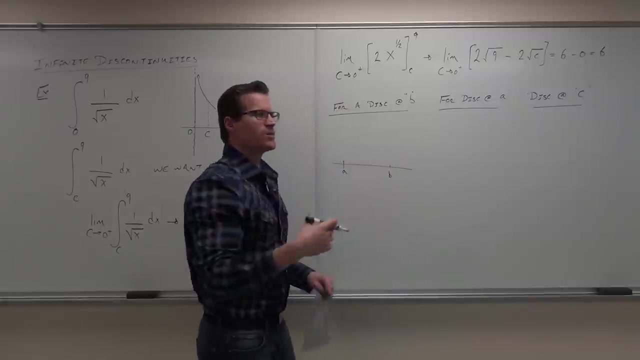 So there's a few scenarios I want to discuss with you. Let's say that we have so for a discontinuity at B, for a discontinuity at A or for a discontinuity at some intermediate value C. So let's say we have some function and there's going to be a discontinuity here. 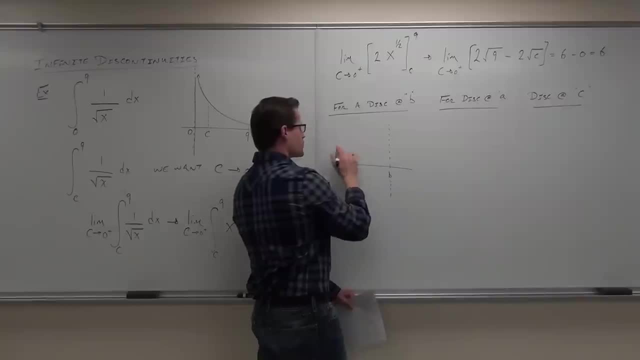 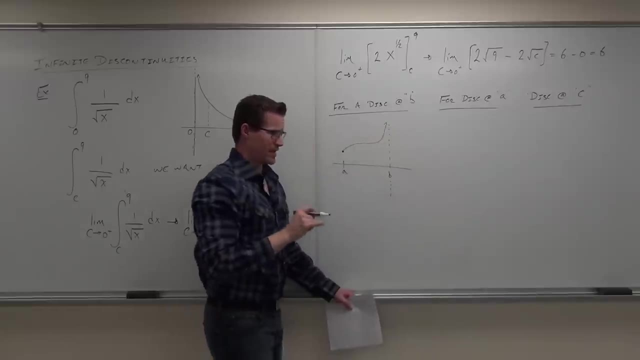 an infinite discontinuity at B. So our function is defined at A, no problem, It's going to do something. I don't know what it's going to do, but somewhere around B there's going to be an asymptote. Do you guys see what I'm talking about? the infinite discontinuity at B. 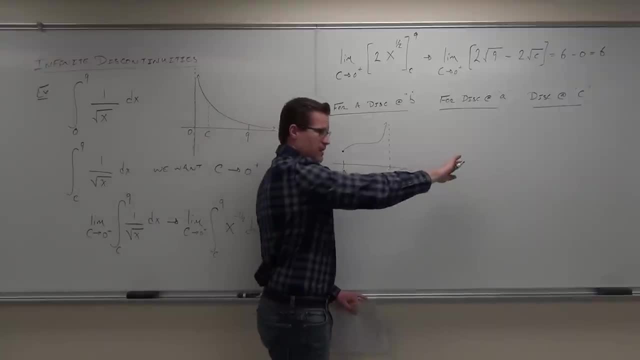 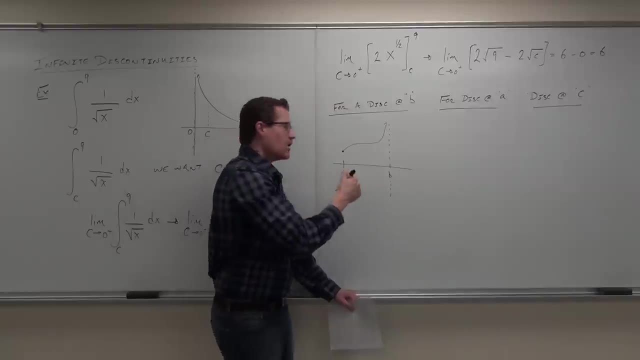 Hello, yes, no, I don't care what happens past it, my interval's going to be from A to B. I don't care what happens before it, my interval is going to be from A to B. Does that make sense to you? 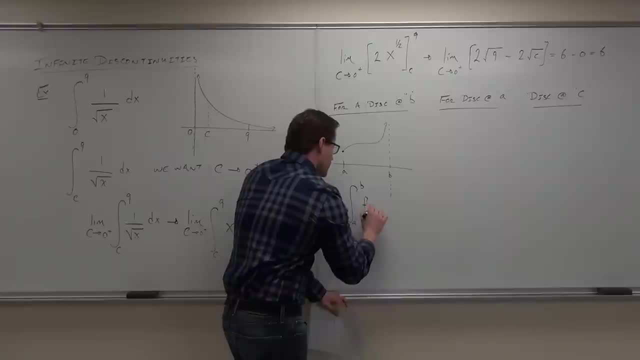 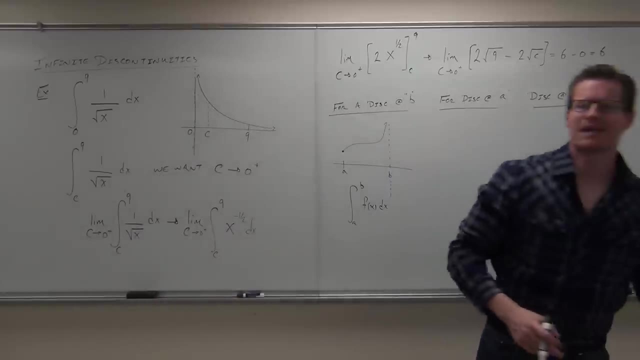 So if I tried to integrate from A to B of some function, then the idea is: well, let's look for the problem area. Let's look at what's wrong with our integral, what's making it improper? Now, clearly- hopefully it's clear to you- my integral is finite. 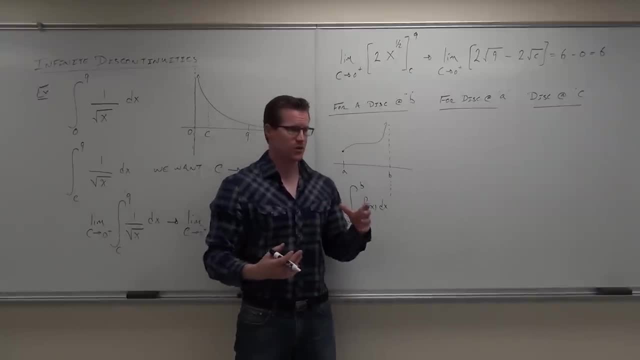 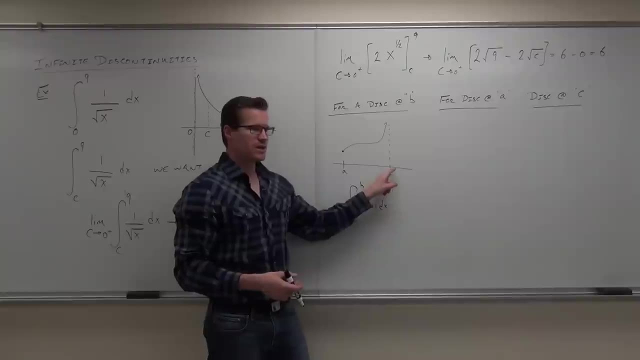 It's going from A to B. It's not an infinite idea, so I don't have to go to positive infinity or negative infinity. it's not a problem. but what is a problem is that while A is defined, B is not. 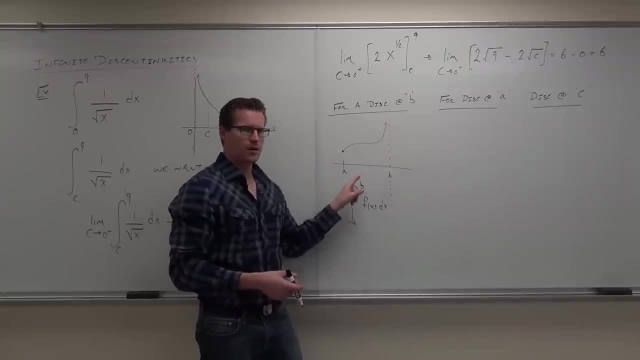 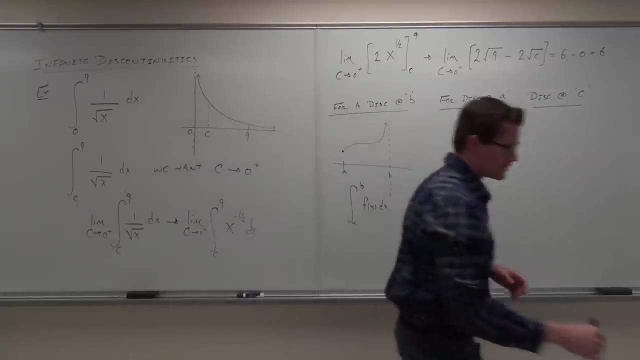 So my discontinuity would be where A or B, So wherever that discontinuity is, that's what we're going to call C or whatever you want to do. So you can call it any letter you want. we typically use C. 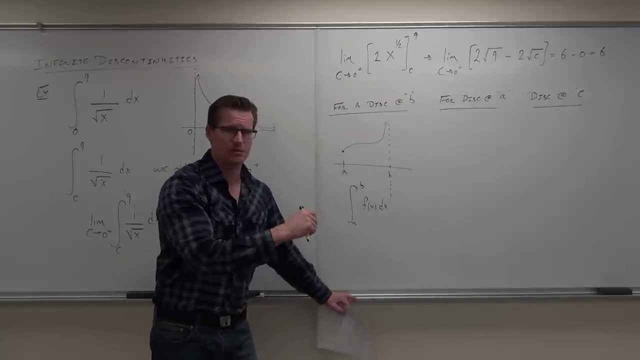 because it's going to be an intermediate value between A and B. Does that make sense to you? So for us we go all right. well, awesome, So we'll have. I'm sorry, which one would we change here? 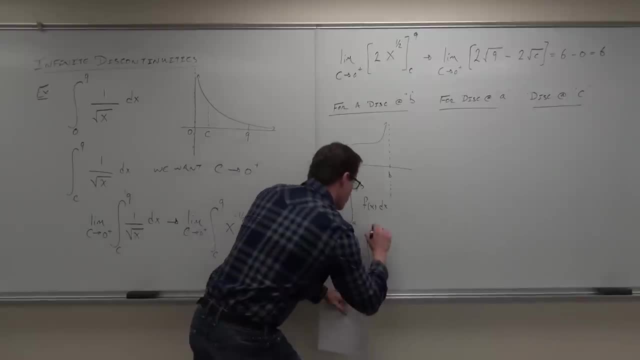 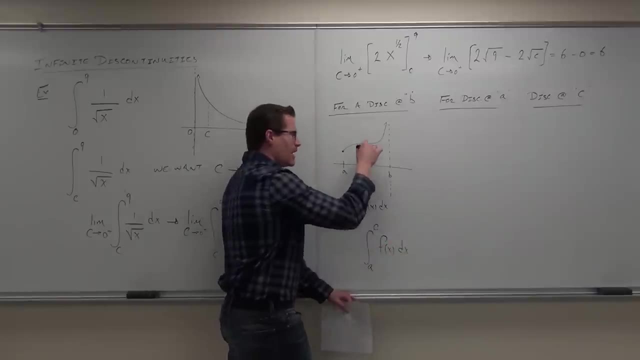 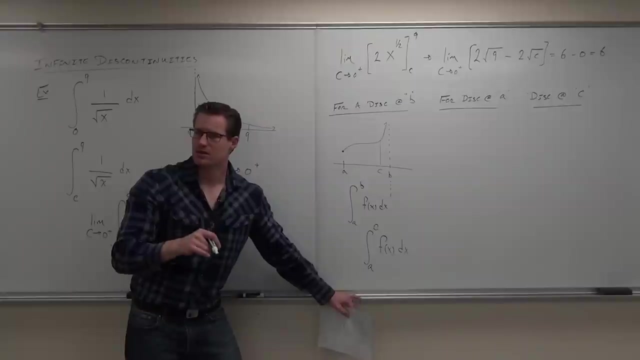 Would we change A or B, B? That would become a C. So we'd say no, no, no, no, not B, Let's make some point C, some intermediate value, And then where are we going to? let C go to. 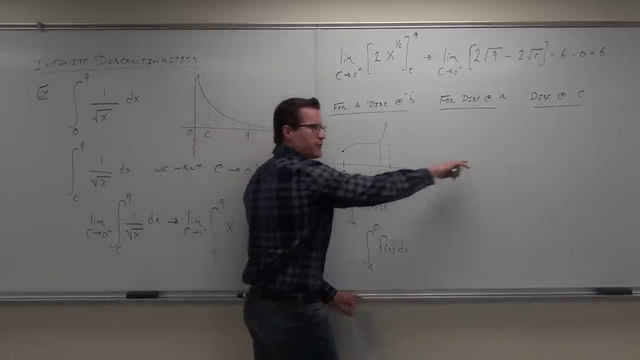 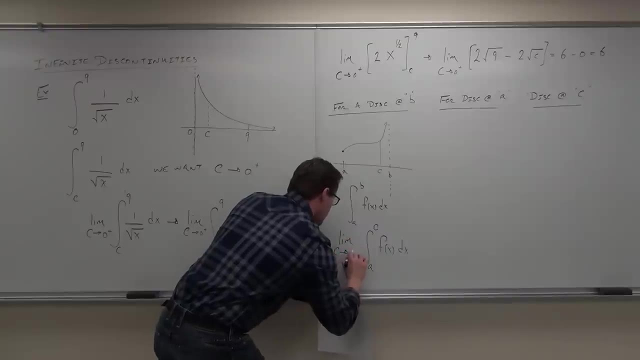 Oh, not infinity, because I'm not going to infinity anymore. I'm going to go to B. I'm going to go to B. So the limit would be: C approaches B. Now think carefully here. So here's the idea one more time, if I didn't cover this well enough for you, 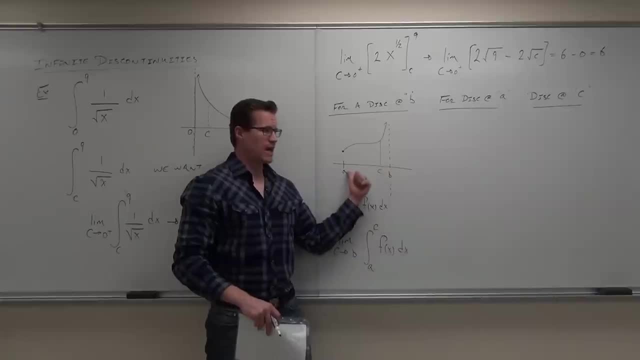 The idea is you're going to have a problem with an infinite discontinuity. It will either be at A or at B or somewhere between there. I'll show you that one last, If it's at one of your endpoints of your interval, A or B. 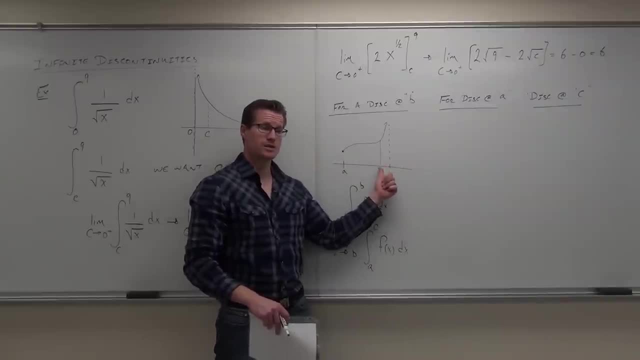 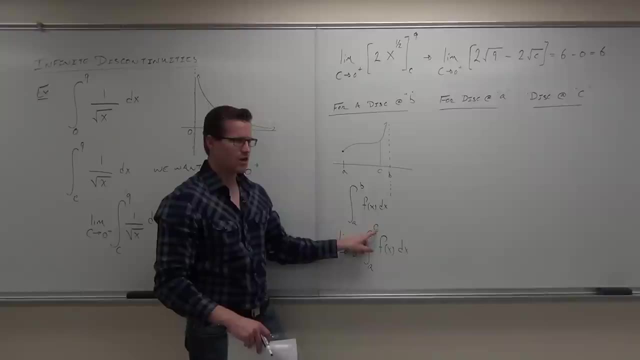 well then, define that endpoint as some intermediate value, C, So we go. no, we can't go all the way to there, So let's go to here. Let's go to C, not B. Does that make sense? Do our integral? because now it's a definite integral that's defined from A to C. 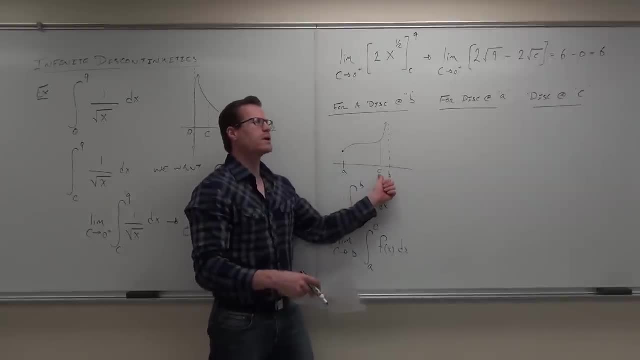 You got it. After that we go all right. well, where did the C really want to go? C wants to go this way a little bit. C wants to go this way a little bit until it hits B. Now, from which way? 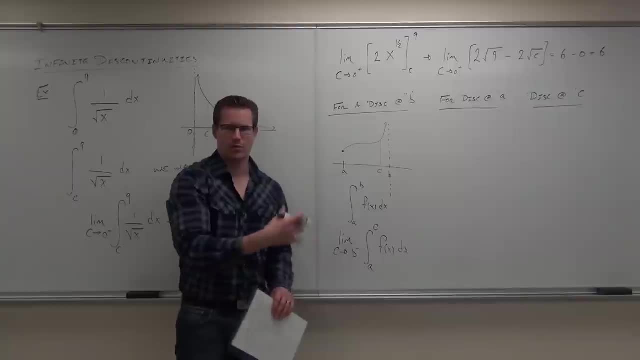 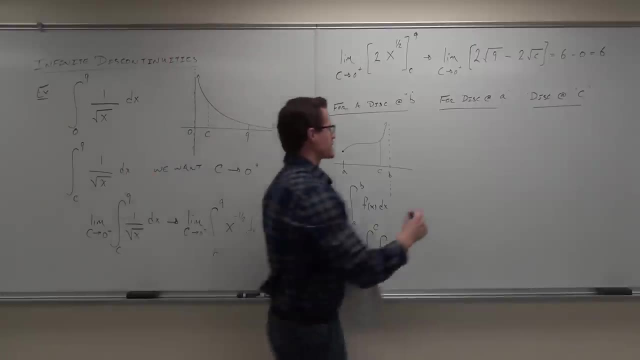 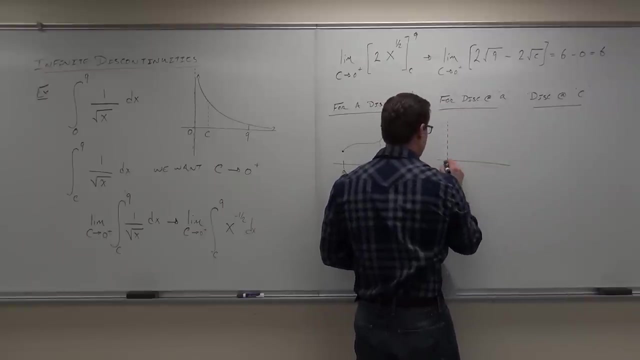 From the left, or from the right, From the left, From the left. That would be the idea I want to show fans to see if you're OK with with this one, Now let's reverse it. Let's say that we have some function that has a discontinuity at A but is defined at B. 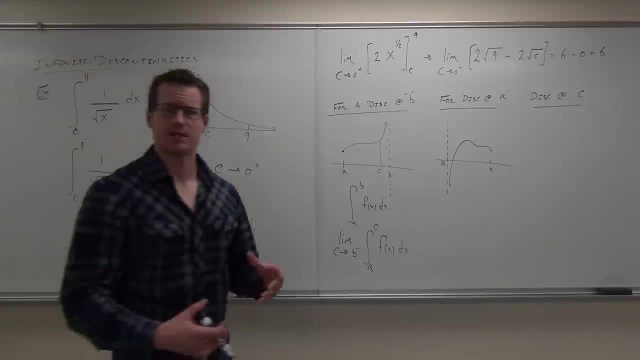 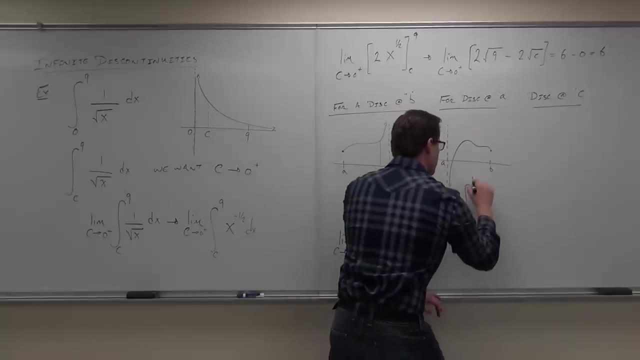 Can we do it the way it is? Well, no, We have an infinite discontinuity. The interval's great. It's from A to B, Not a big deal. So if we had an integral that says: I want you to integrate from A to B of whatever this function is, 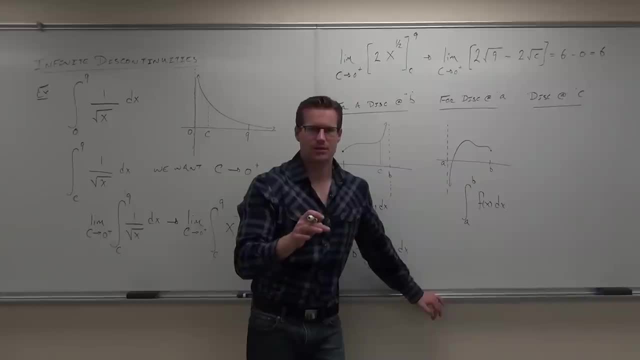 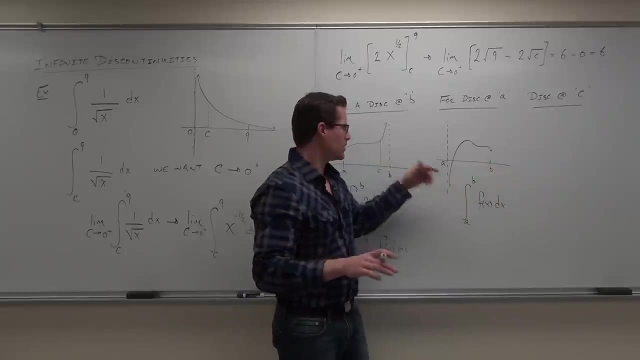 where is our problem here? Is our problem at A or is our problem at B? B, I mean A, yeah, It's at A. B is fine, right, B is defined, We're good to go. So what we go is- well, tell you what. I don't really care about going to B. 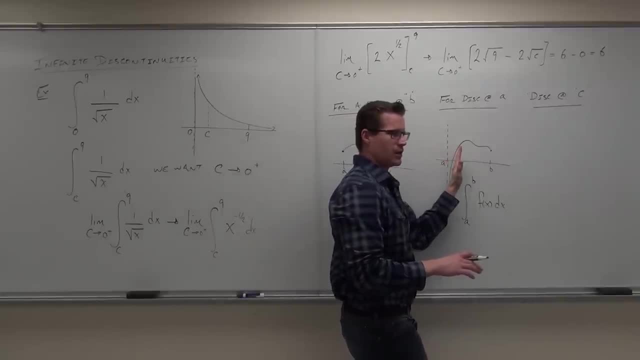 That's good to know, but I can't start at A. If I can't start at A because it's not defined, where am I going to start? C, Some intermediate value, C. So my B would stay the same, but my A would become a C. 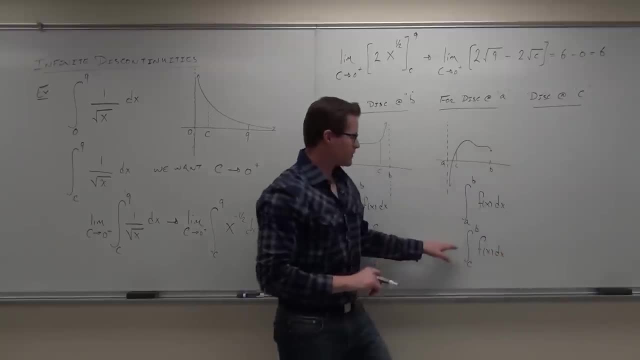 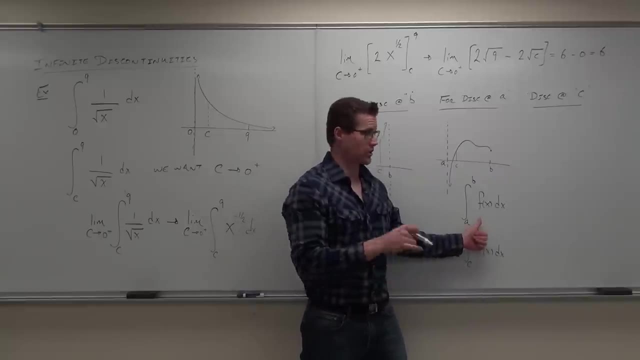 What that lets us do again what we did last time. that gives us a definite integral that we can actually evaluate. It says: now you're going from a finite number to a finite number that you can actually plug into your integral after you've already evaluated. 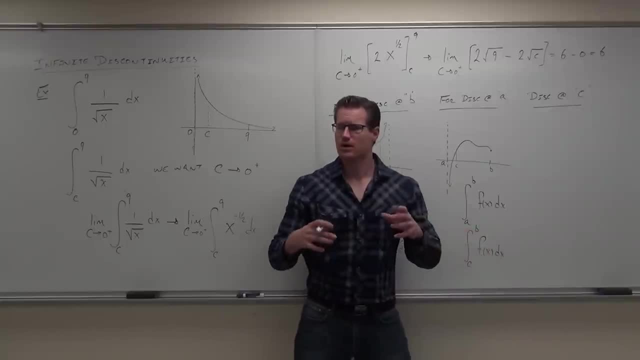 That's great, We go okay, plug in the B, plug in the C, subtract them. good to go. Calculus tells us we can do that. We can subtract that evaluation. We can plug in B and then subtract off and then plug in C, in this case. 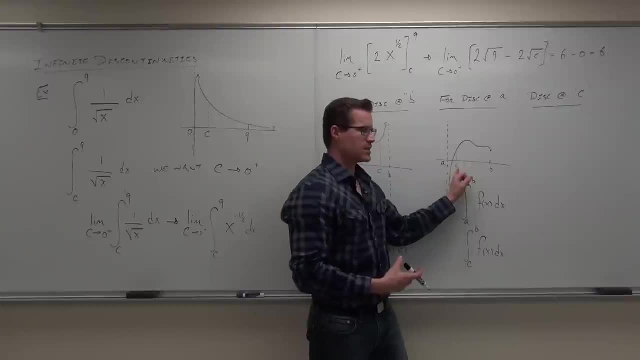 Now the problem is: well, I'm not really starting at C, I want to start where I want to start, at A. So yeah, this integral says from C to B, but now this limit can take the C and move it which way. 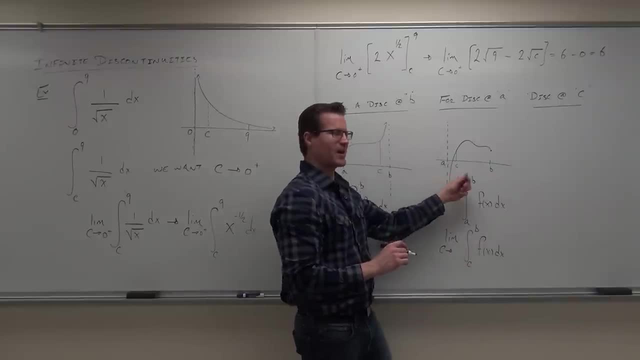 To the right. Okay, so let's just say to somewhere to where To A From the right side, From the right side. that's right. That's actually the first example that we had. that's right here. It said: okay, I can't start at 0, but I can start at C. 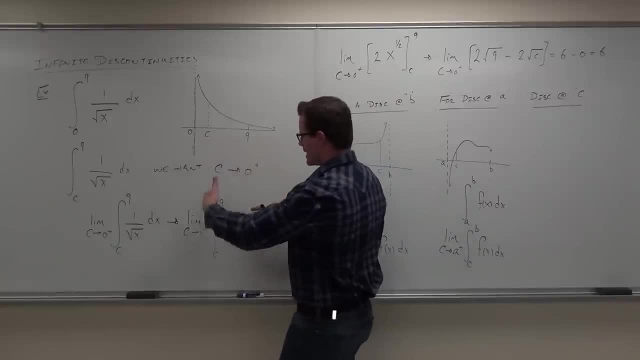 Now, at the very end, we go: okay, look at that, From C to 9. actually lets you evaluate it, Plug in the 9, plug in the C. that's great. That's what definite integrals are all about. 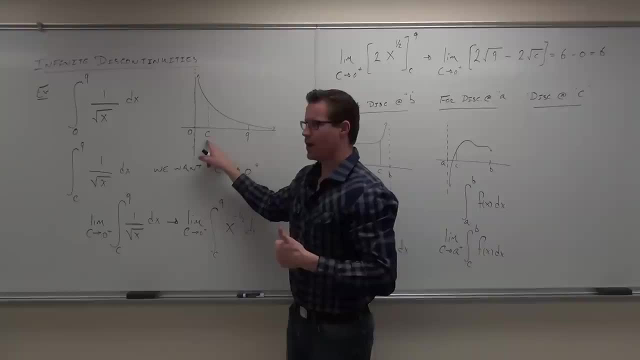 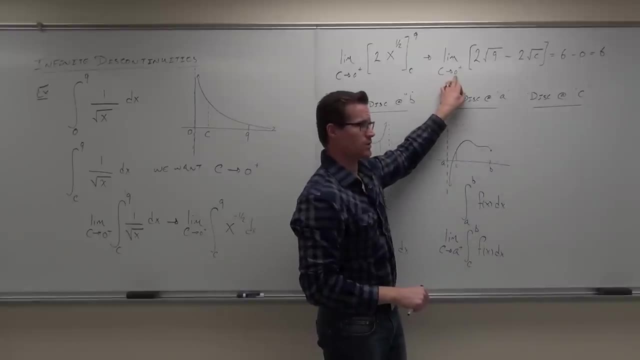 Then it says: well, I want that C to not start here, I want it to start really close to here, And that's what this limit idea says. I want the C to start really close to here. So towards 0 from the right-hand side. 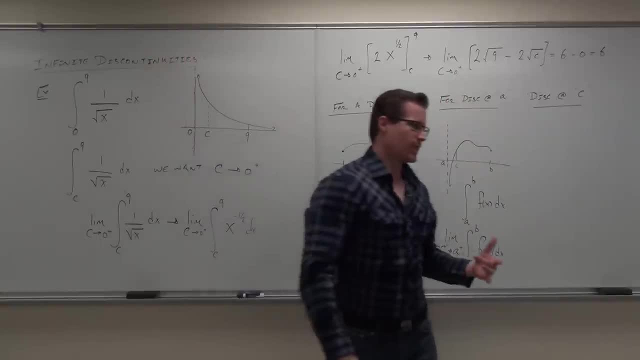 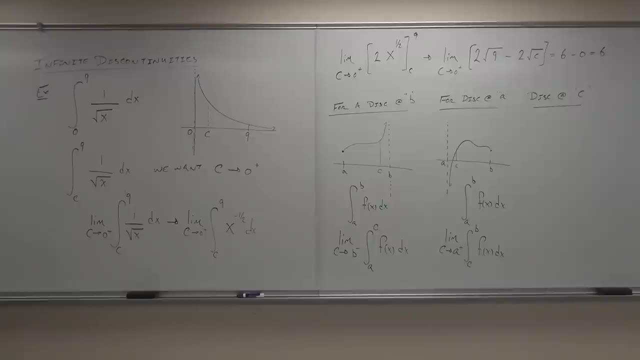 That's what this is. Show your hands if you feel okay with that one. Now there's one situation we haven't covered. What's the situation we haven't covered? Where there's a hole right in the middle- Holes I don't care about, because that's why they're called removable discontinuities. 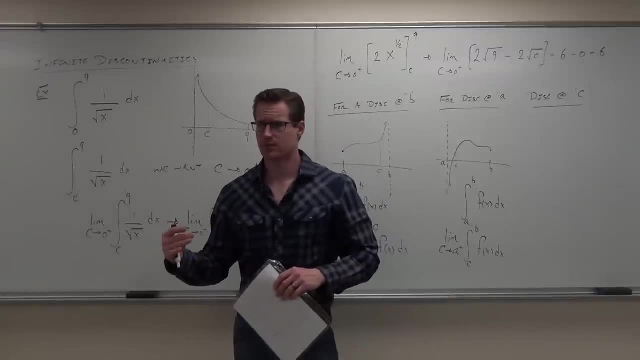 They're not going to affect us. It's still bounded correct. So if we have a hole, we can plug it with a single point. Does a point have any width to it? That's going to blow your mind. If a point has no width to it, then if I'm missing a point. 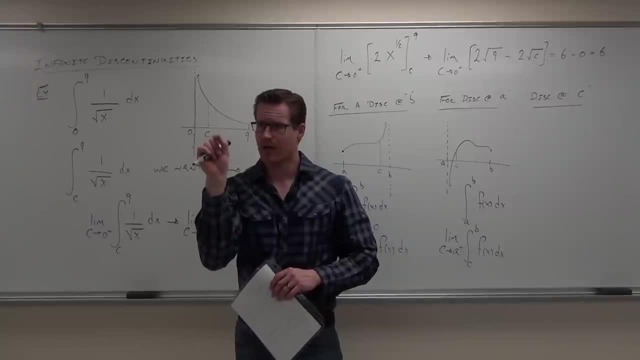 on my line, so a hole. basically, since a point has no width, it can't possibly have an area under that point. Does that make sense? This area is width times height. It has no width. I don't care how high it is, 0 times anything is still 0.. 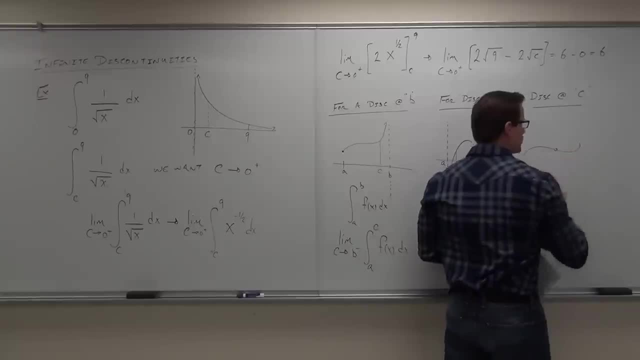 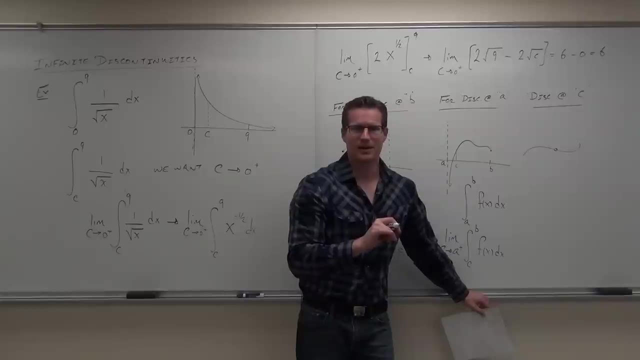 So for that reason, if I have a removable discontinuity that does not affect the area under the curve, Those points have no width. Crazy, right. What will blow your mind is you can have an infinite number of those on your line. 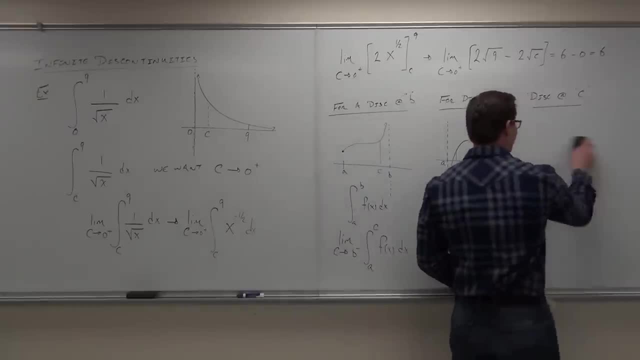 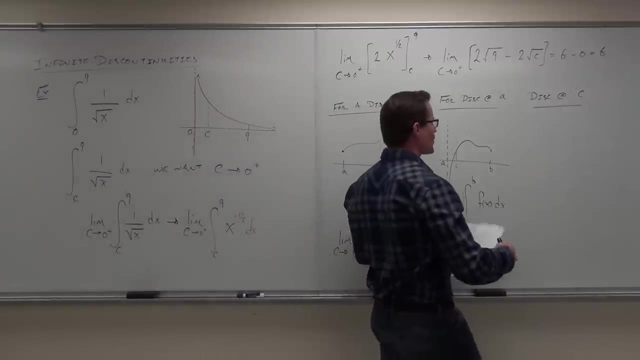 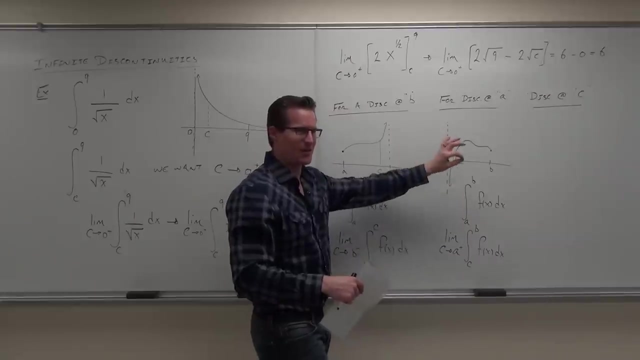 and still get an area. What Anyway? different class, Different class, Discontinuity at C. So what happens if it's not hit? Did I just completely blow your mind like a mine grenade? Do you see what I'm talking about? how that one point doesn't affect the area? 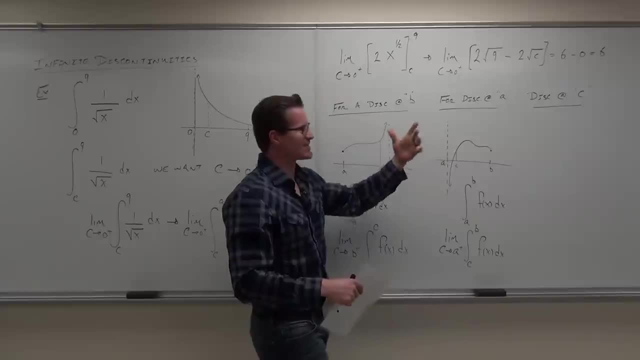 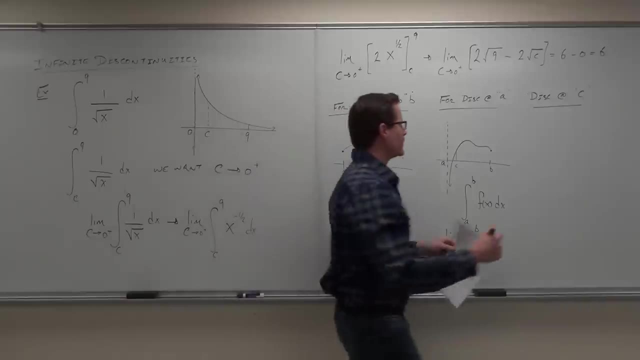 Yeah, That's so neato because there's no width. So therefore, we don't care about the holes, We care when it's not bounded right, because that's a problem. We need to define that a little bit better. 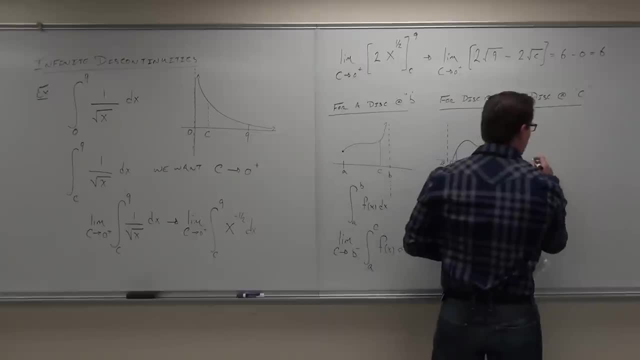 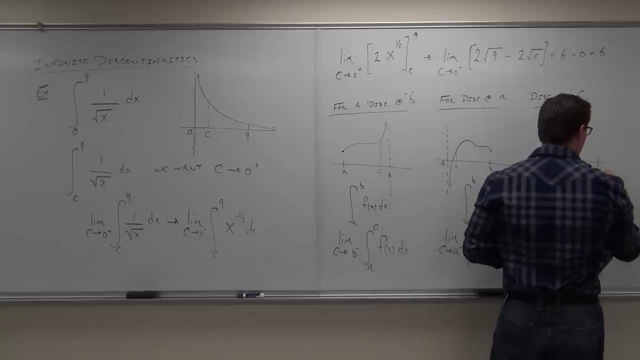 So it's not here anymore. It's not here anymore, It's somewhere in the middle. So here's our A, where we'd have something defined. Here's our B, where a function would be defined, But somewhere in here we've got a problem. 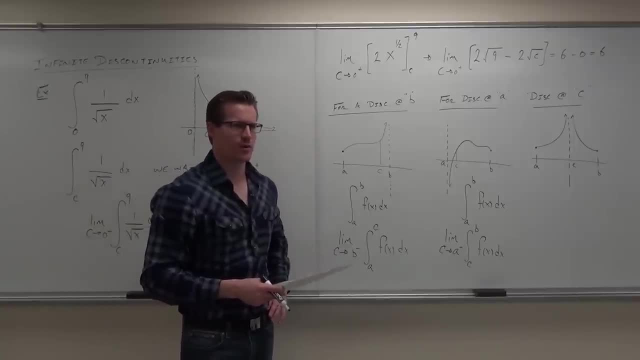 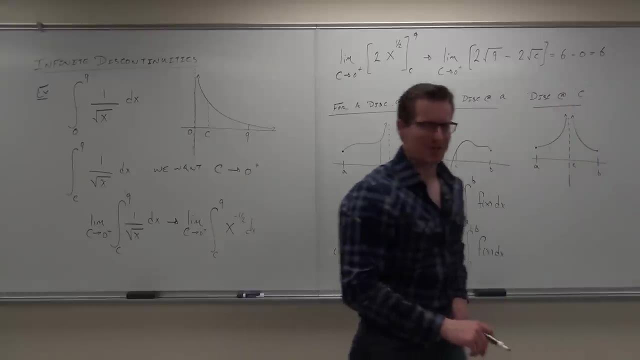 Oh, did I say infinite number of holes? I think I might have been finite, I'm not sure I don't remember anymore. It could be a finite number of holes. Let's see, That would be just a little bit of a problem if I don't know that exact thing. 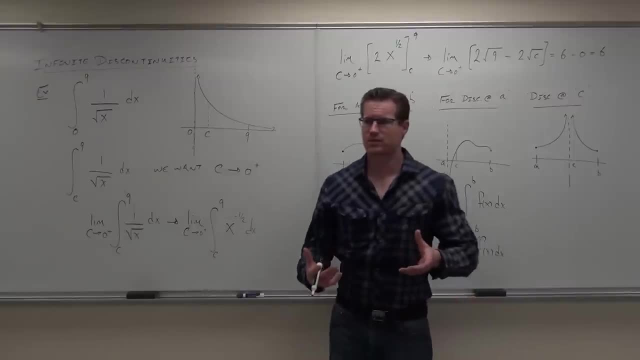 Well, what's the issue here? Are we defined at our end points of our interval, at our end points A and B? Are we defined Yes, So then our infinite discontinuity doesn't happen here and it doesn't happen here. 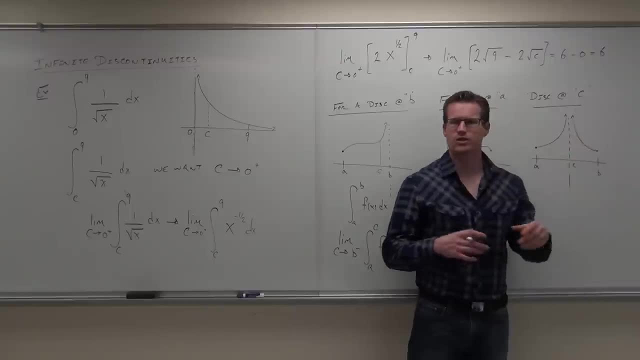 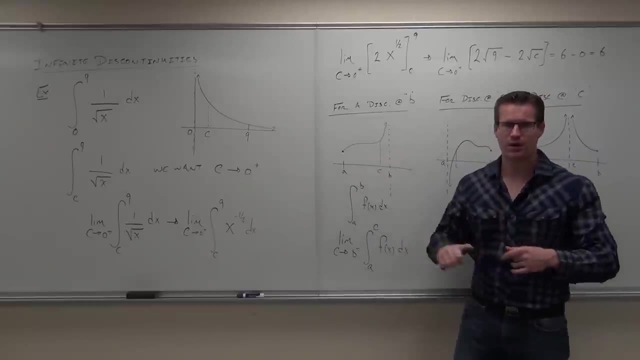 It actually happens right in the middle. Whenever you get this case, this is the worst case scenario. This one's kind of nice because you just go: okay, it's one limit. Does that make sense to you? One limit because we have one discontinuity from one direction. 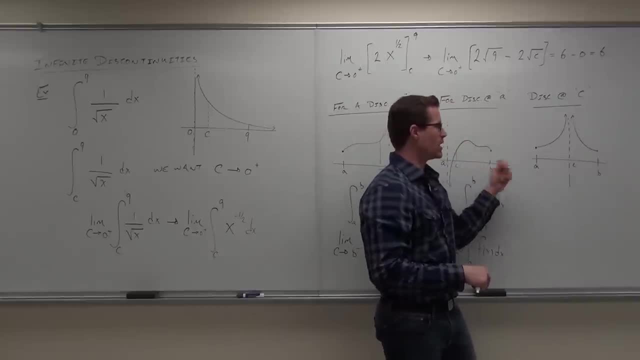 Here no problem. one limit, one discontinuity from one direction. Here one discontinuity, but it's from two directions. So whenever you have your infinite discontinuity between your bounds of integration, the A's fine, the B's fine. 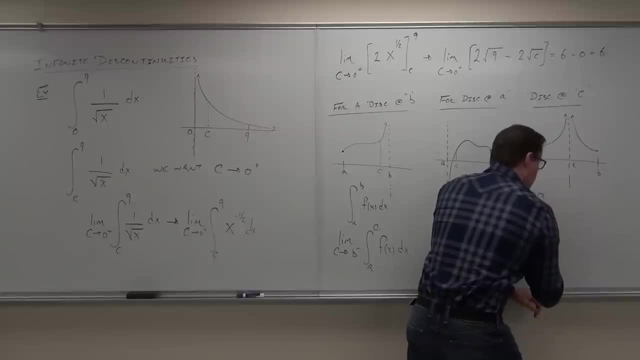 Somewhere in the middle we have a problem. So somewhere in the middle we'd say, okay, where would we go? where would we start from? if I want to do this, I'd start at A What's my problem at? 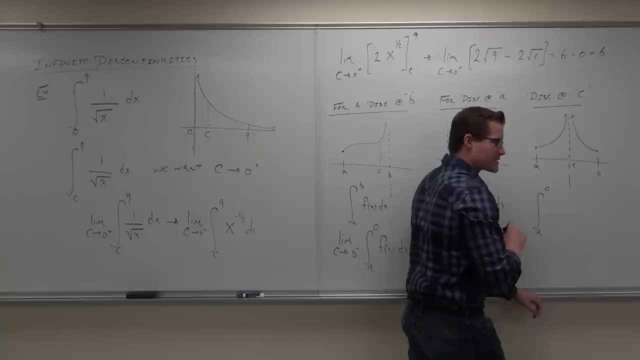 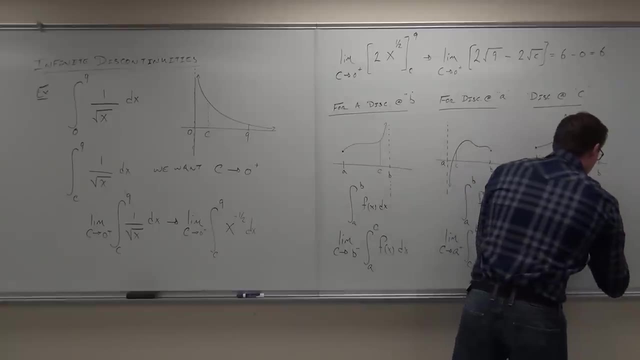 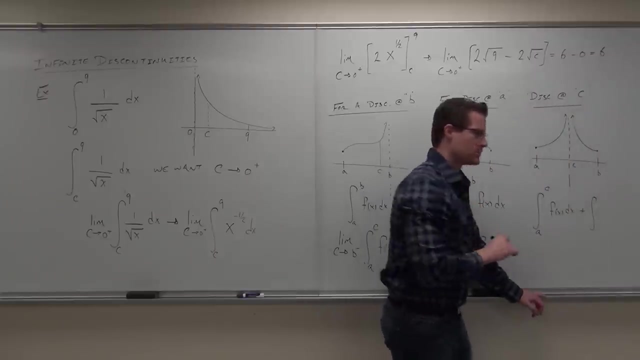 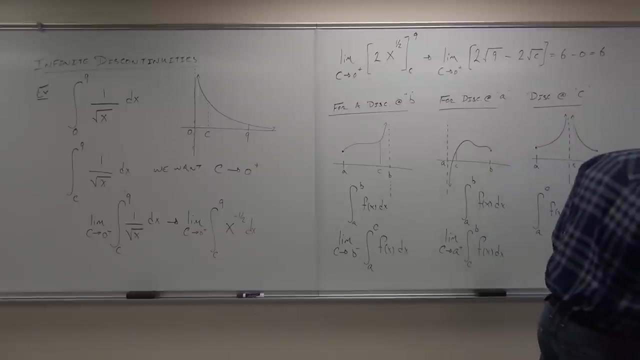 C. Yeah, I'd have C. I'd have to split that up, Then I'd have another integral starting from where C And going to B After you do this. so basically, here's the idea. If you have it at one of your end points of your interval, not a problem. 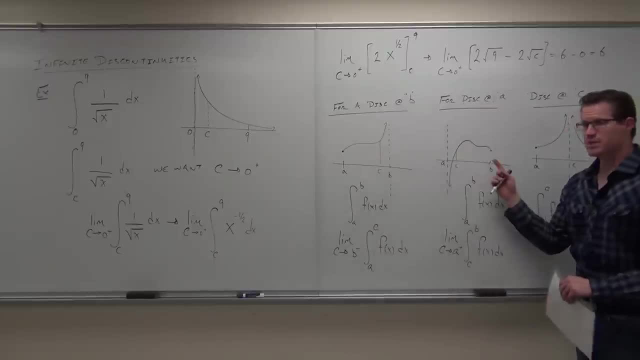 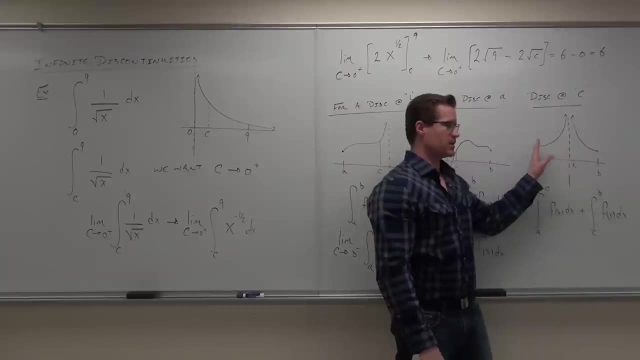 Just call it from A to C or from C to B respectively, and let that C go to the appropriate number. If it's in the middle you have to break that up. So the starting point to where C is, then C to where the ending point is. 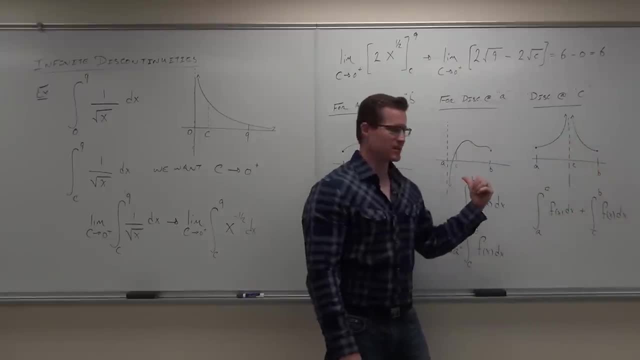 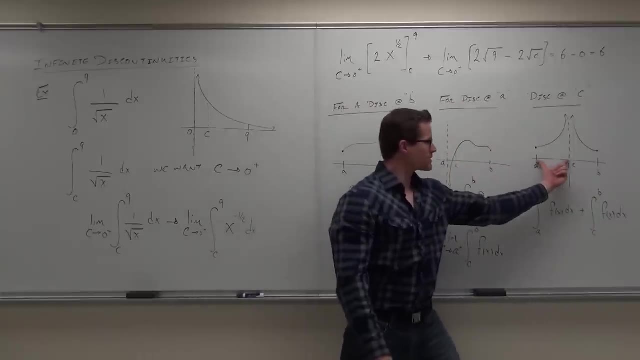 where your ending interval is, and then you do basically the above. So, basically, do you guys see that this idea is a combination of these two ideas? We get one of these and we get one of these. Basically, this integral is this one. 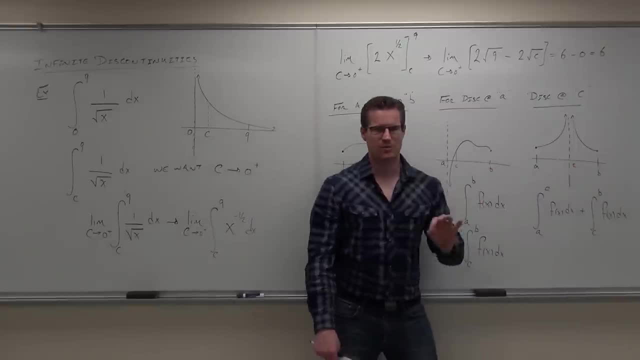 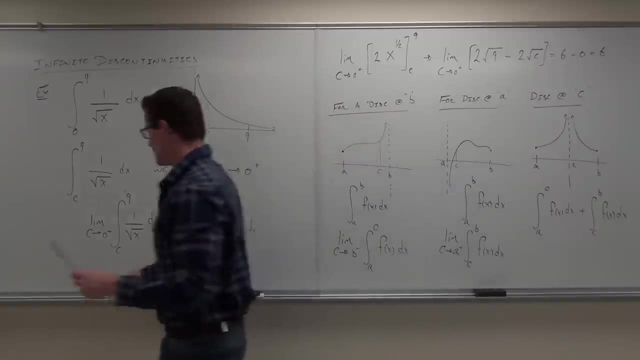 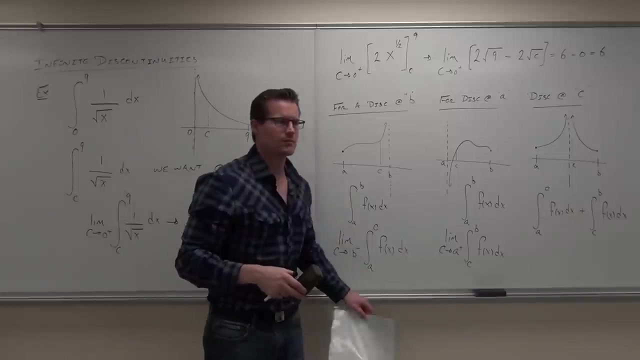 This integral is this one, And you do exactly the same thing. Make sense, Are you sure? You guys want to try a couple of them? Okay, probably, Let's do so. Any questions? Questions: What if it doesn't approach infinity on both sides? only one. 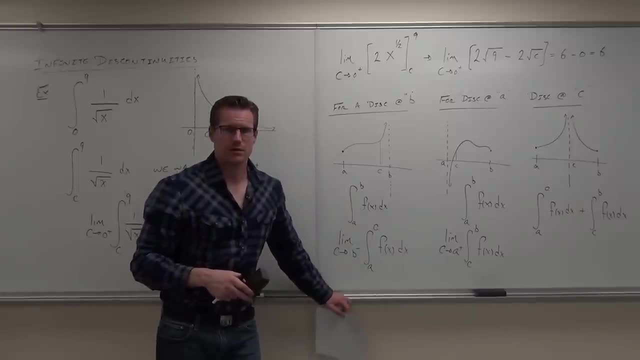 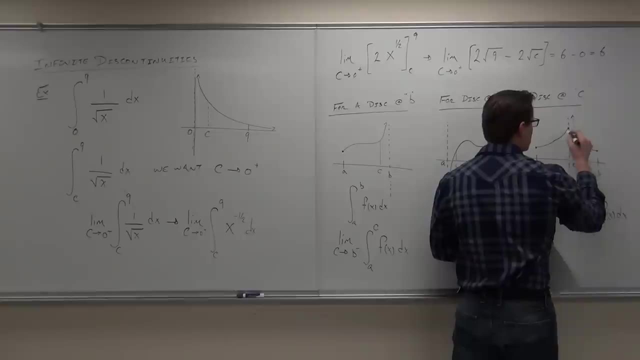 You can still try. It has a point, and then it comes down from infinity. What do you? oh, like a, like a piecewise defined function like this one? Yeah, That'd be great because this integral is defined, So this would be like easy, okay. 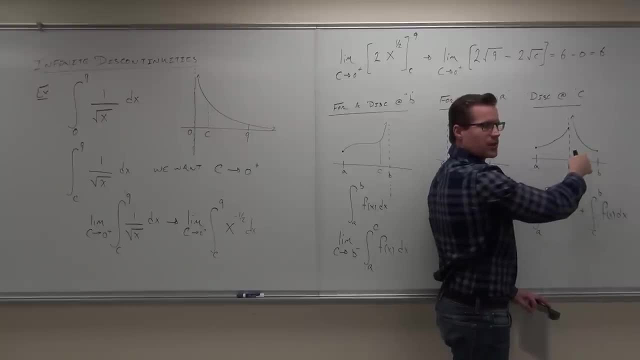 You say, hey, A to C, no problem. But then this side, you'd still have to split it up because it's not continuous. You have an infinite discontinuity, hence the not continuity part. okay, So this would be good. 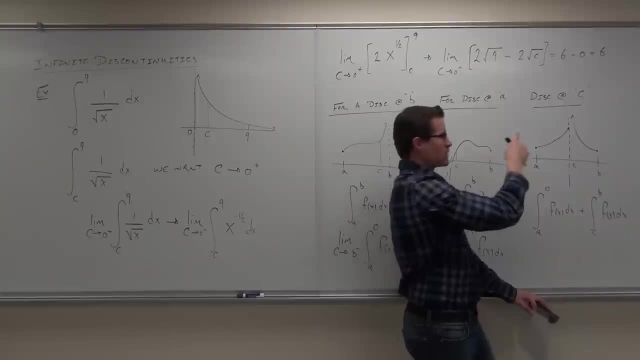 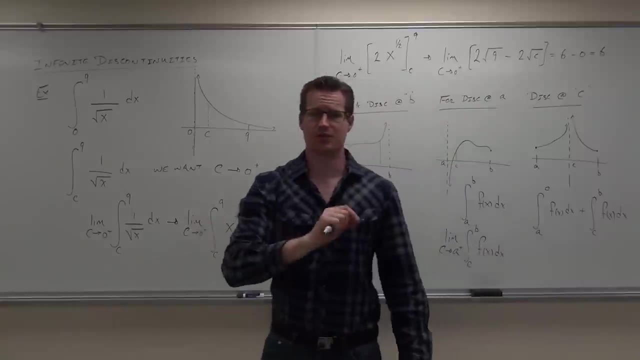 This part, you say: well, I got to do this one, That's a good question. So you just would skip the limit on one. You wouldn't have to do it for the left side. That would be easy because it's actually defined. 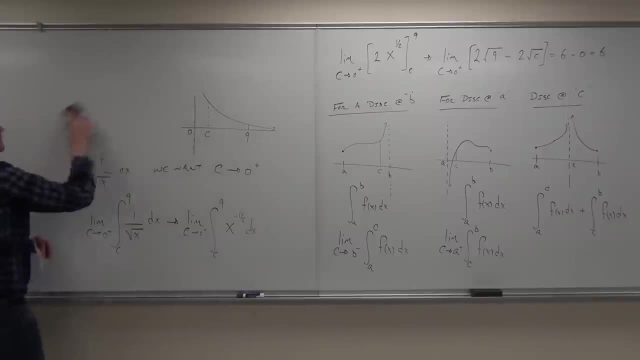 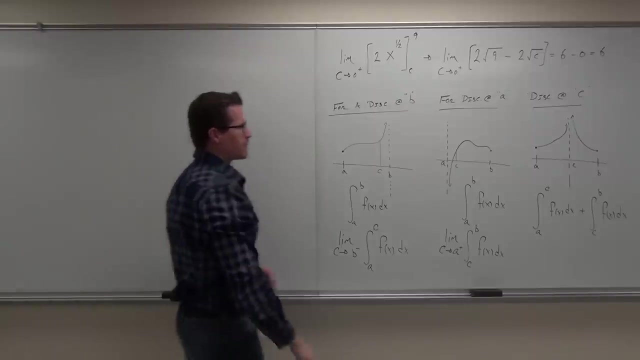 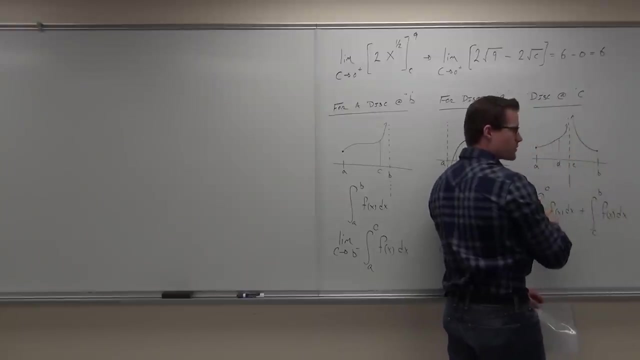 That's a good question. Any other questions? What would the limits look like for the A to C and C to D? It's easier to show you with actual numbers, But what you do is you call this intermediate point D And you say a limit as D approaches C from the left. 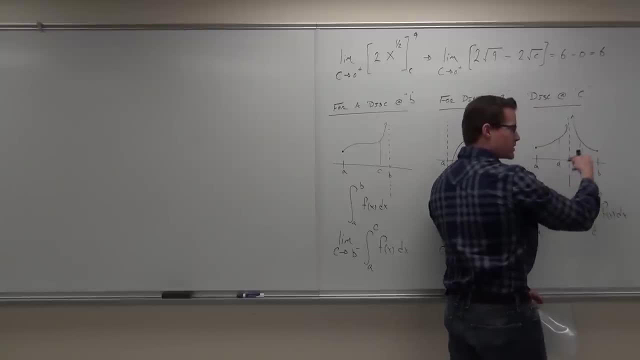 You'd say a limit, as maybe E, as E approaches C from the right, So you have to have. this is why I don't want to show you that many letters, because what in the world are you talking about here? But you go from A to some number D. okay, 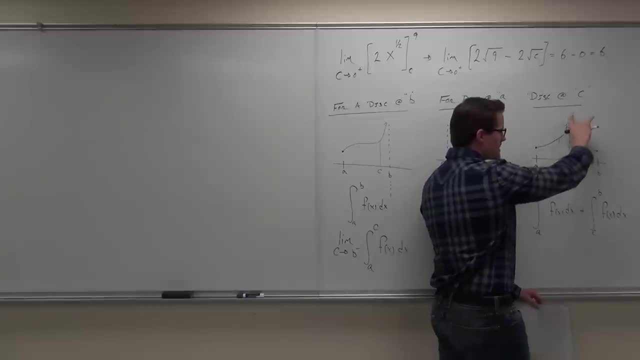 You do your definite integral and then you let D go to C, your undefined point from the left-hand side. Here you define some intermediate point E. You've already used C and D, so E. Then you do your definite integral from E to B. 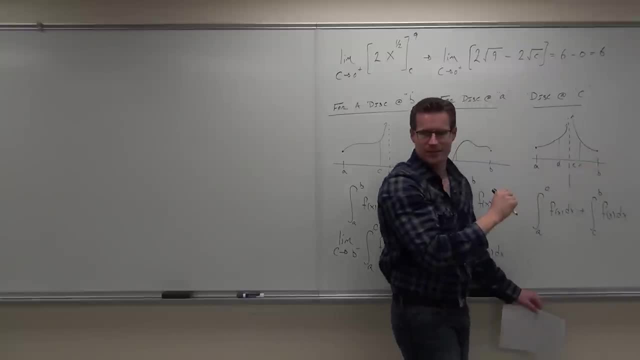 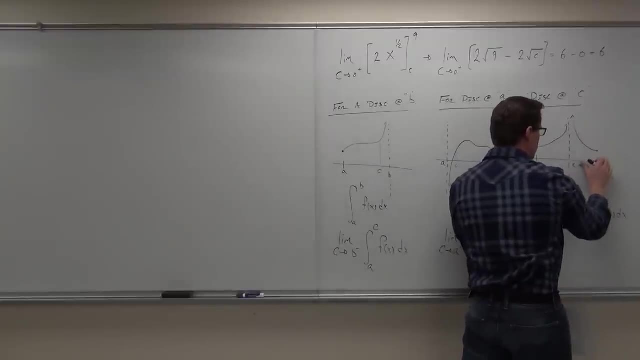 After that, you let E go to C from the right-hand side. Did you guys follow that Same idea? It works easier with numbers because I don't have all these letters floating around. Okay, so let's actually get to the nuts and bolts of this thing. 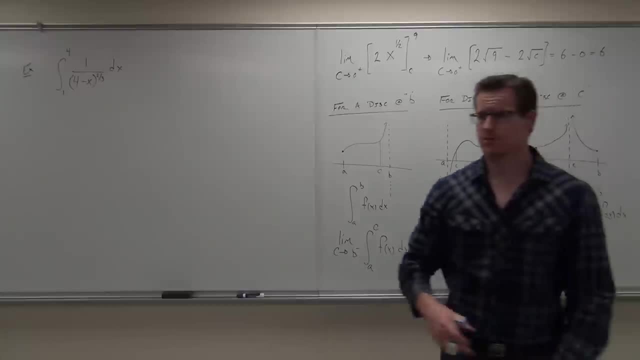 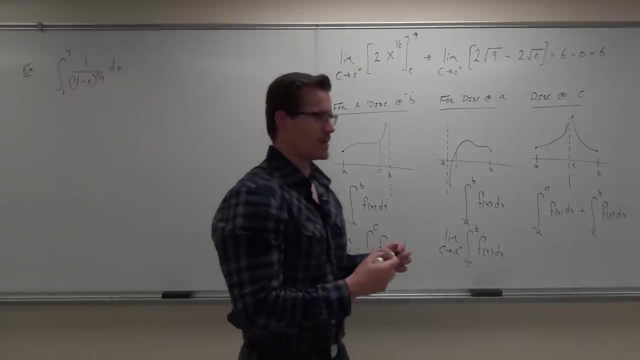 You know, one of the most important things we can do as integrators of these improper integrals is determine what we're talking about: whether we have an infinite interval or whether we have an infinite discontinuity. Which, in this case, do we have? 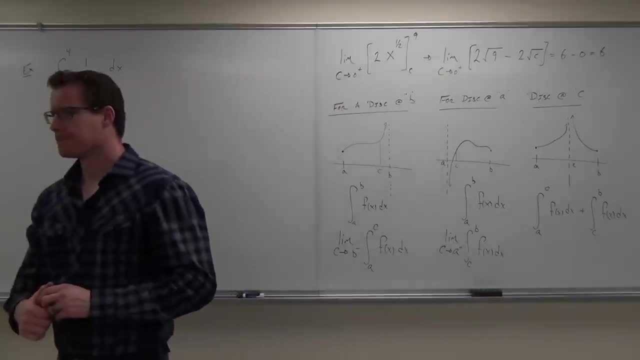 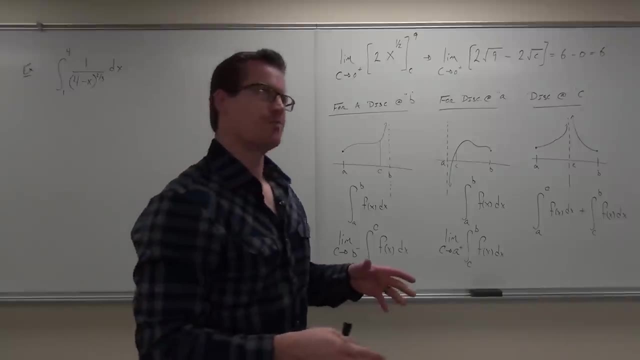 An infinite interval or infinite discontinuity. Infinite discontinuity Interval's great. We're going from 1 to 4.. That's a definite interval, It's finite. But within that 1 to 4, we've got a problem. 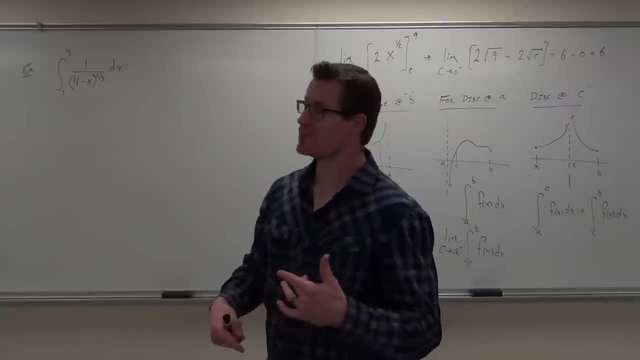 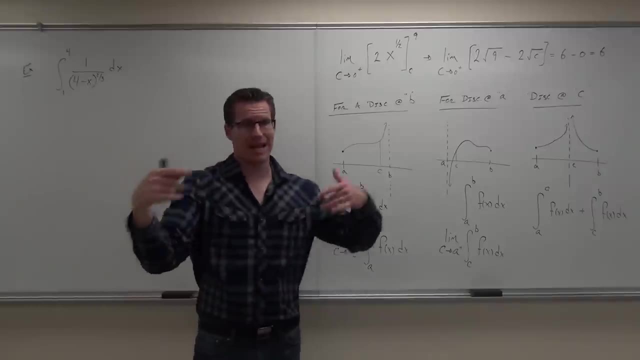 So you have to define all the problems you have, and there can be several of them. You could have a problem at an endpoint. You could have a problem at both endpoints. You could have a problem at both endpoints and somewhere in the middle or several places in the middle. 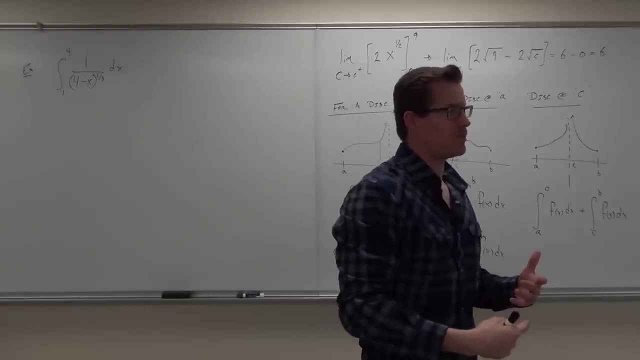 Now, of course, right now we're going to keep it kind of easy. right, There's going to be like one problem, But you could have many, many different problems. Does that make sense to you? So everywhere, your denominator is 0,. 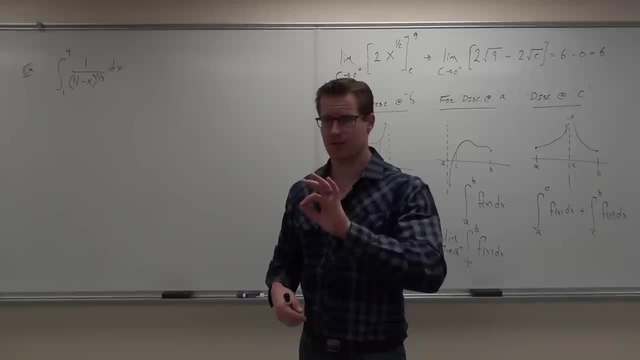 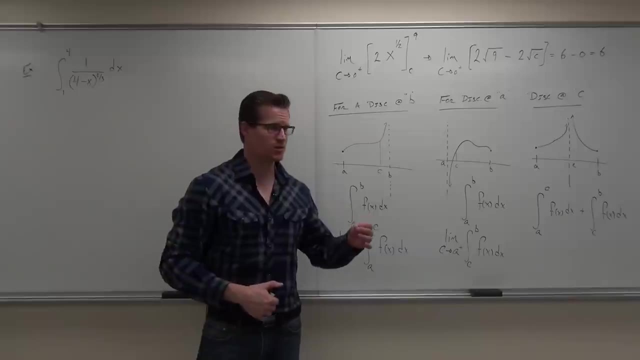 that's an infinite discontinuity, provided you can't simplify out the. The red's not a hole. basically, That would mean you would get from calculus 1 the difference between holes and asymptotes. If you had me, you should have known that. 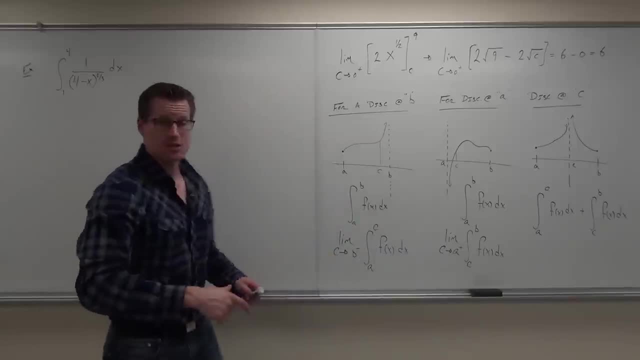 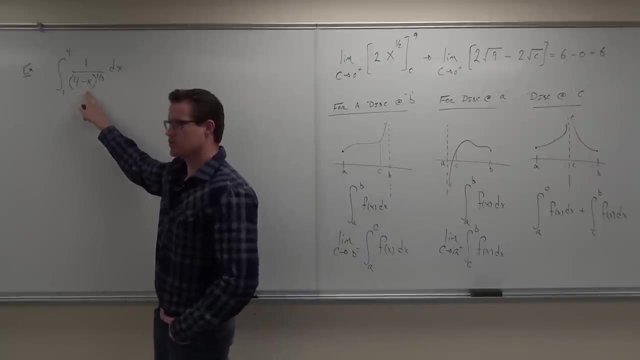 Exactly what the difference is between holes, removable discontinuities and asymptotes. So in our case, where is our problem? at 4.. It's not a 1.. You can plug it in, It's not a 0.. 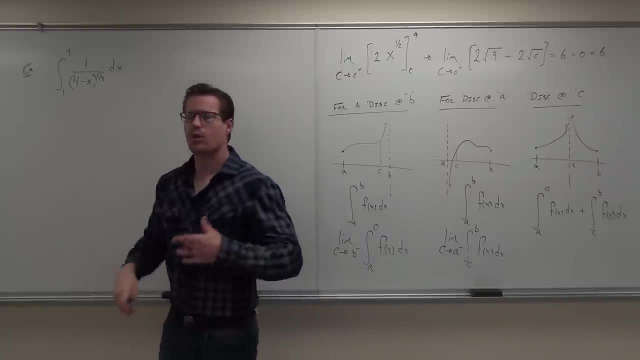 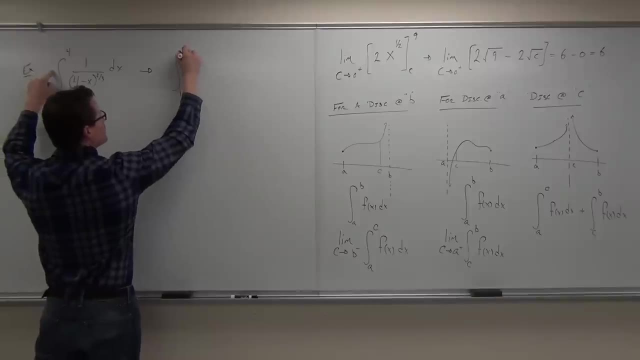 2, 3,, cool 4,. ugh, that's a problem. So what we're going to do is we're going to say: well, you know what, If it's not defined at 4,, let's make it be defined somewhere. 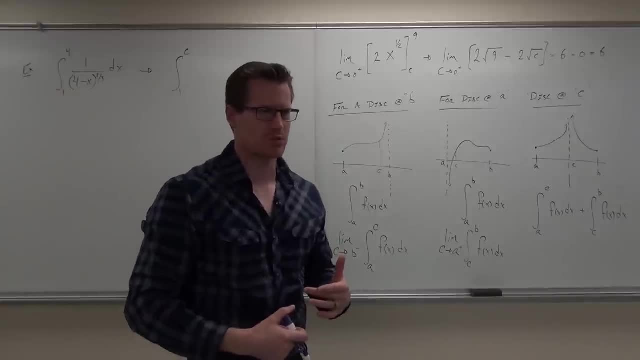 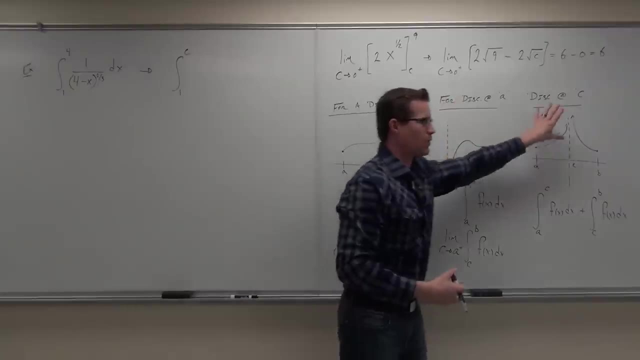 at some intermediate. point C: Are you guys with me on this one? Which case is this? Is this the case for 1,, 2, or 3?? Which case do we have? 1.. We have 1.. We have this one. 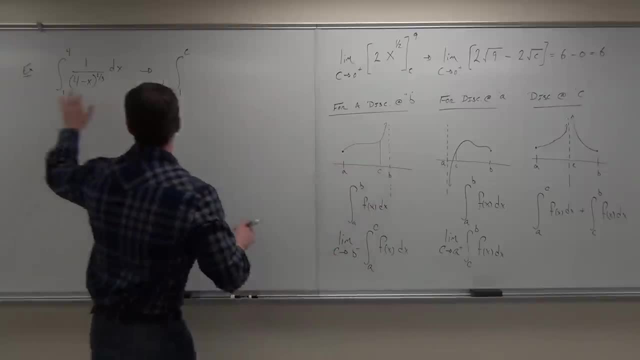 It's defined at A. It's not defined at B. It's defined at 1.. It's not defined at 4.. So we're going to call this some point, right before the B, Right before the 4,. we're going to call it C. 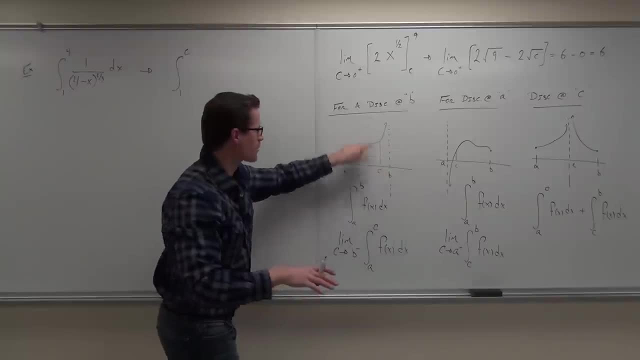 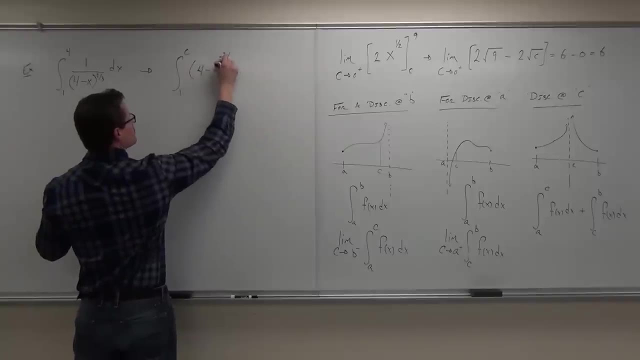 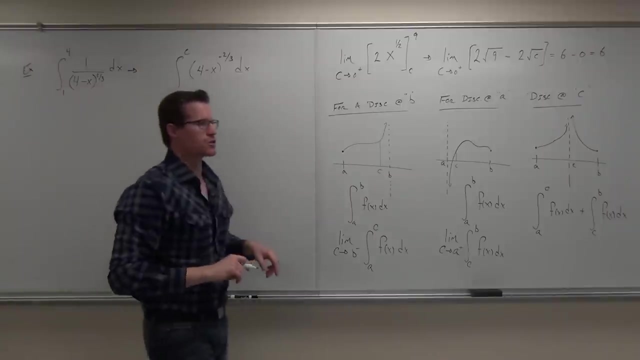 Maybe it's 3.999999 forever. I don't know what it is. We're going to call it C Now. we're going to have exactly the same function. We just have to say what's happening on my interval. So we have to say where C is going. 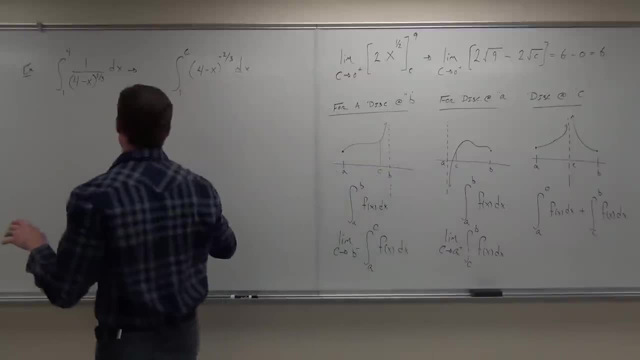 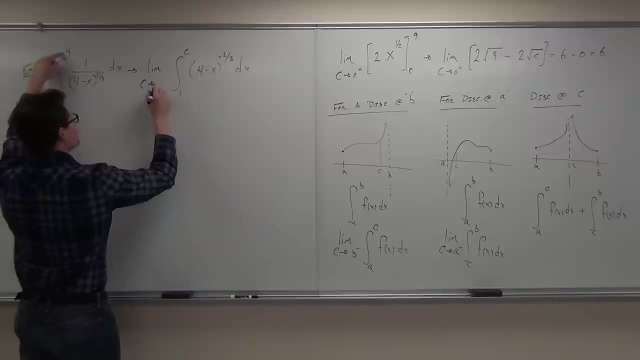 So how do we say where C is going? What are we going to use Limit? Yeah, limit is the way we say where a number is going, A limit as C approaches where 4.. It's always going to be this number or this number. 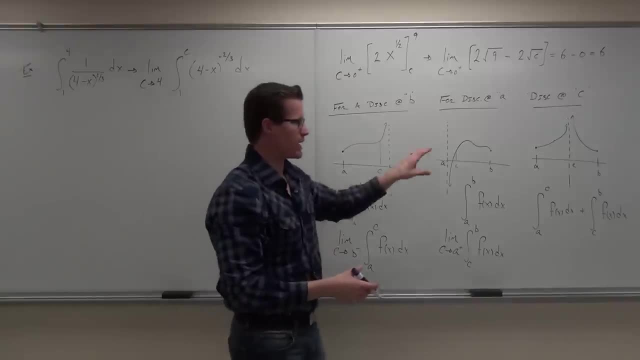 or some number in between. There's always going to be a number, So it's not going to be a random letter anymore. We're defining what's happening to the C. Now you've got to be good at this. Is this C 4 from the right or 4 from the left? 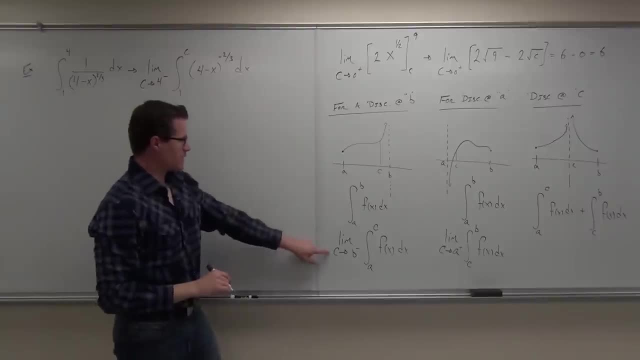 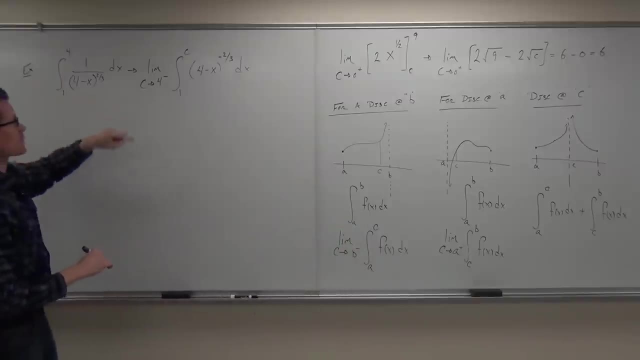 Left From the left. So let's see if it matches up. C is going to the top number from the left, C is going to the top number from the left. Hey, that looks exactly right. Can you do that integral? It should be pretty easy. 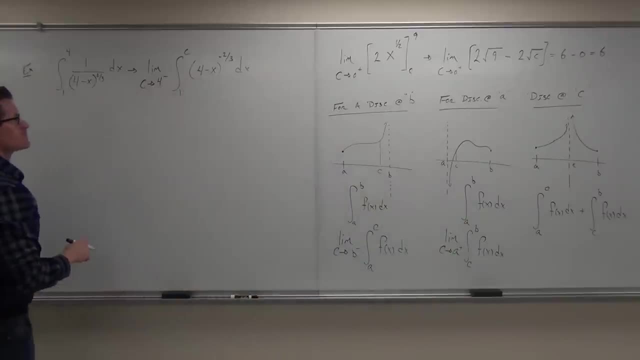 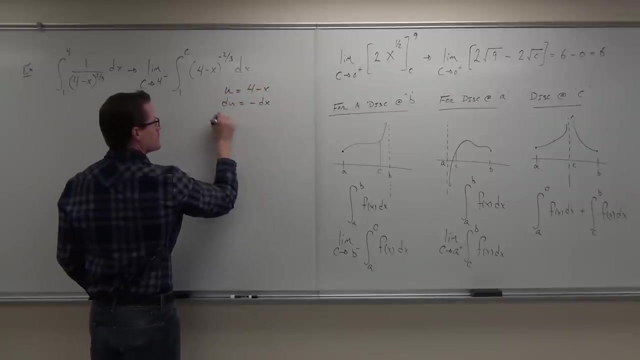 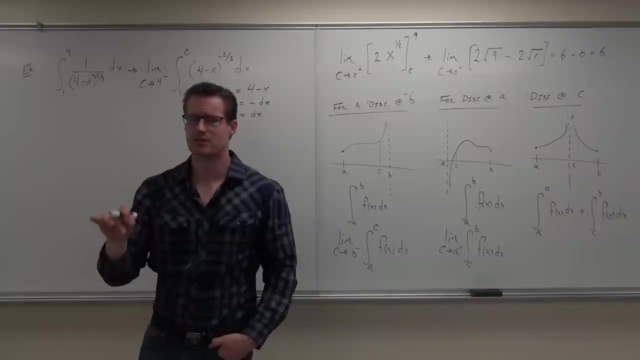 What would you use in order to solve this integral? What would the? u be? du equals negative dx or negative du equals dx. Again, I'm going to go kind of quick on this, but do not neglect your substitutions. Your signs are important. 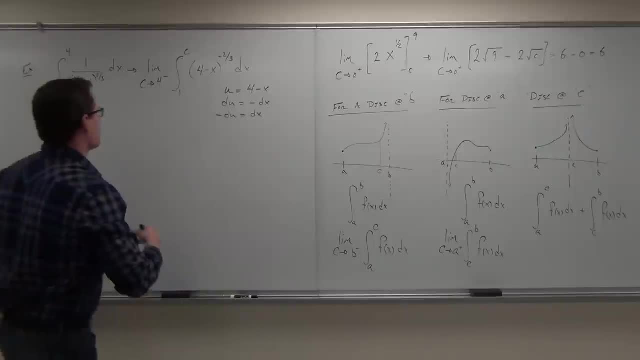 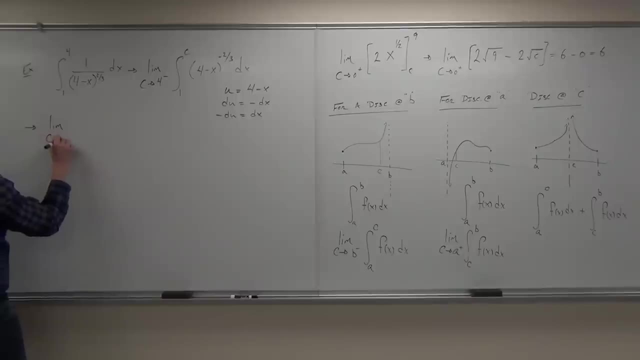 You guys see where the negative is coming from on that one. No, That's important. Okay, so we have a limit. as C approaches 4, from the left of the integral, from 1 to C? u to the negative, 2 thirds times negative du. 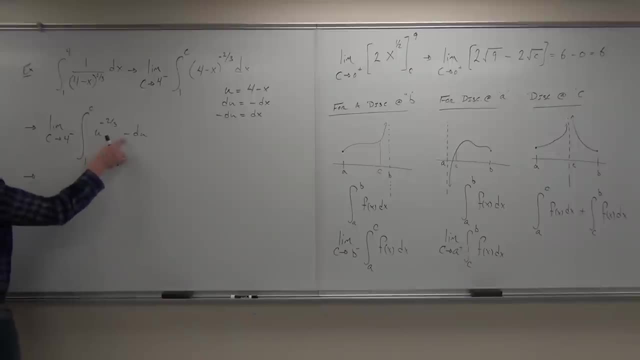 Tell me what I can do here. Okay, you can actually pull it all the way out front if you want to. You can pull it in front of the integral. It doesn't really matter. u to the negative 2 thirds. du Can you all integrate u to the negative 2 thirds. 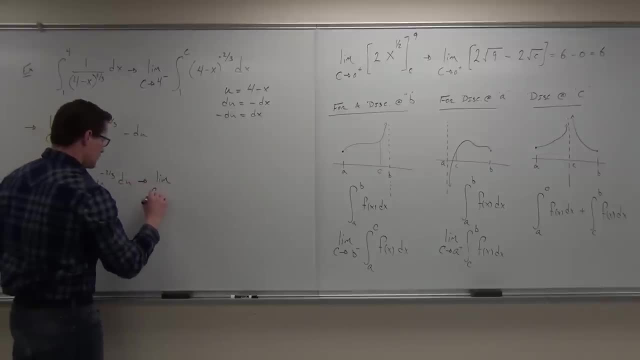 How do you do that? Okay, so we have our negative, We add 1, we get 1 third divided by what? 1 third? So this would be 1 third divided by 1 third. u to the 1 third divided by 1 third. 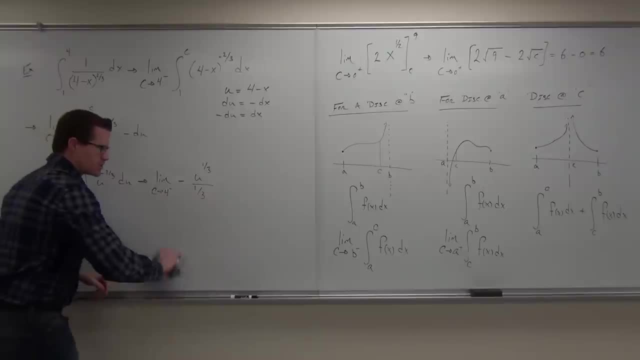 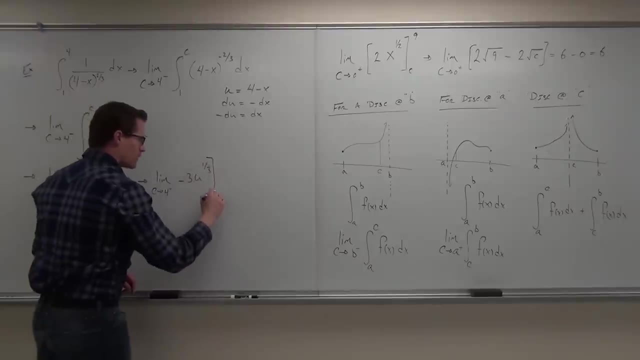 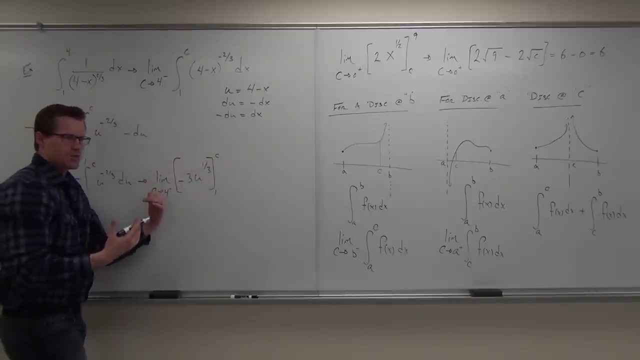 No more integral. We've already done the integral. What's the 1? third change to 3.. Now we can evaluate right now from 1 to C, or you can pull your negative 3 all the way out front. I might choose to do that just to show you that it's possible. 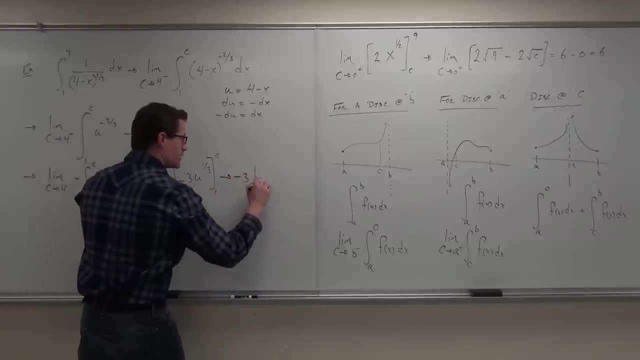 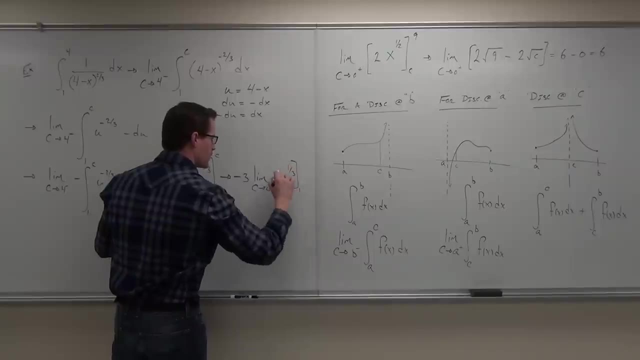 So from here I can pull that negative 3 out in front of my limit And do u to the 1 third from 1 to C. Now there's a big issue right now with plugging in the values. What's the problem? 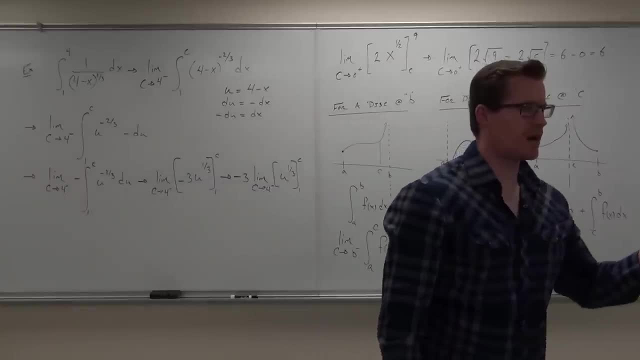 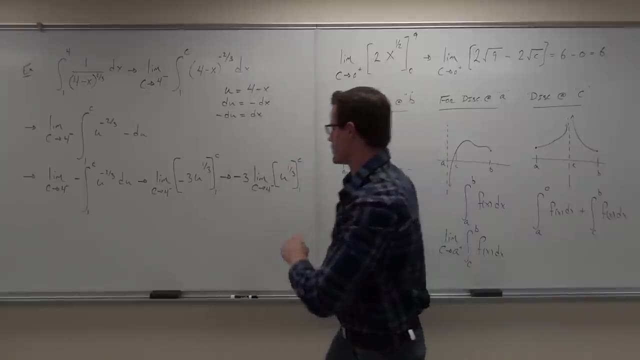 Changing bounds. We didn't change bounds. So if you didn't change bounds, instead of plugging it into u, what do you have to do? first, We've got to take this substitution and put it back, So we're going to have to do negative 3 times the limit. 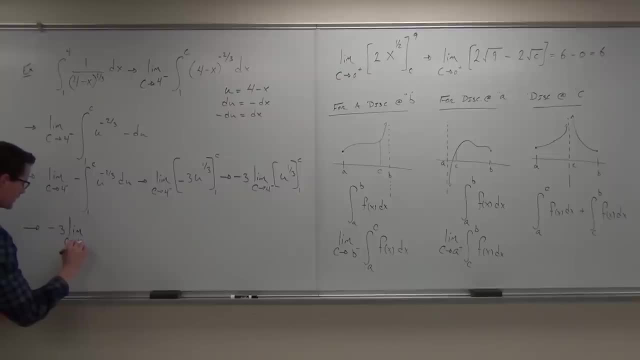 as C approaches negative 4.. Sorry, 4 from the left, 4 from the left-hand side. What's it going to look like? 4 minus x to the 1 third. Okay, so 10, 20-second recap. 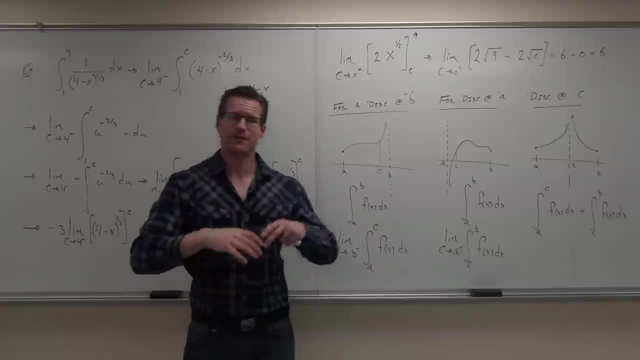 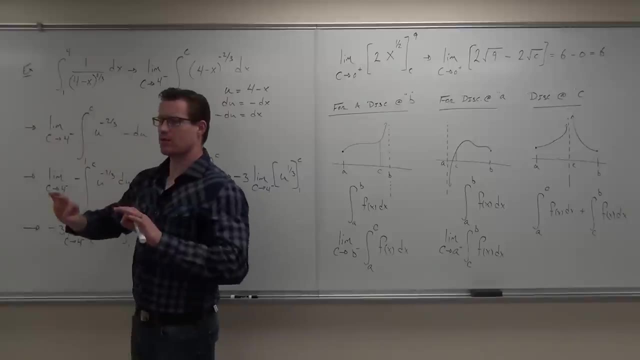 Here we go. We first identify what type of problem we have, whether it's an infinite interval, whether it's an infinite discontinuity, maybe both of them. Look for all your problems. We're good to go Here. we're not defining at this number. 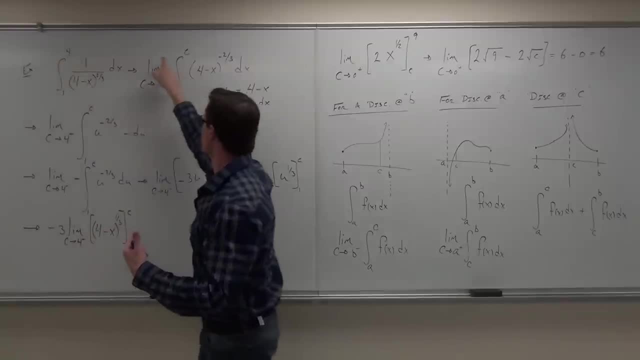 at that end bound, end point of your interval. We call that some intermediate value C. We say, hey, where's the C going? Well, it's going to go to 4 from the left-hand side. We don't care about the right-hand side. 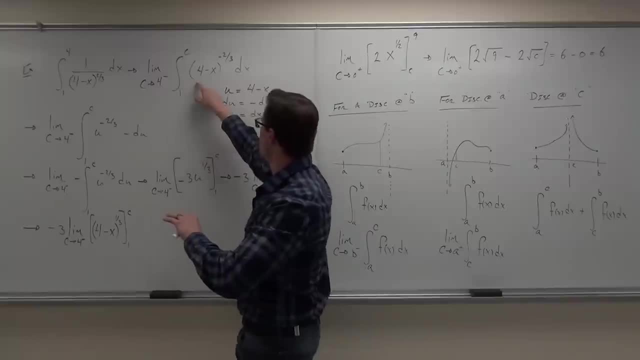 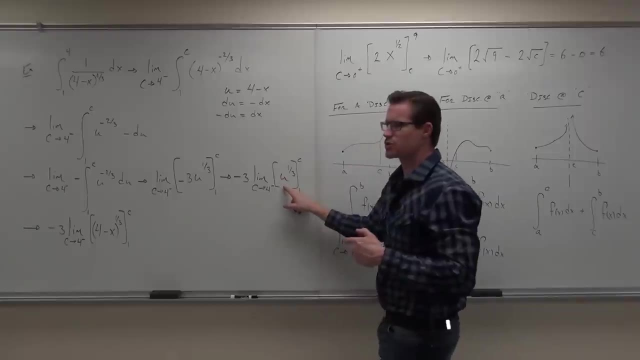 That function's not even there. We don't care, We're going to evaluate our integral any way that we can. We have lots of techniques to do that. Get all the way down to here and then, oh my gosh. well, if you use a u-substitution before you evaluate a definite integral, 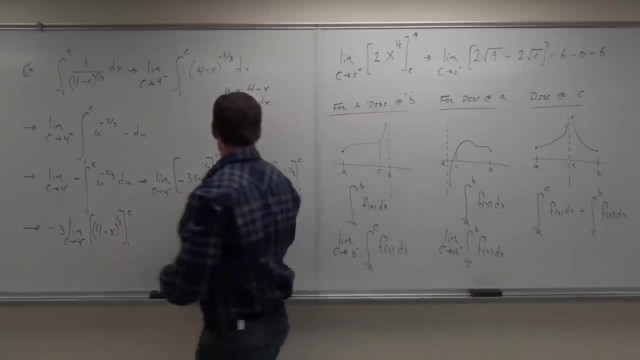 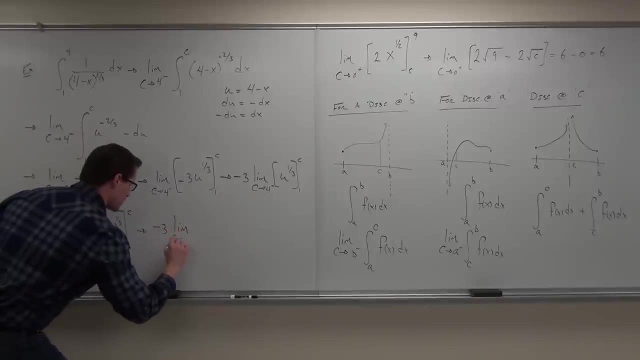 you definitely better plug back in your u. So we have a 4 minus x to the 1 third. Now we get to evaluate, So we've got negative 3.. Let's not forget that And limit as C approaches 4 from the left. 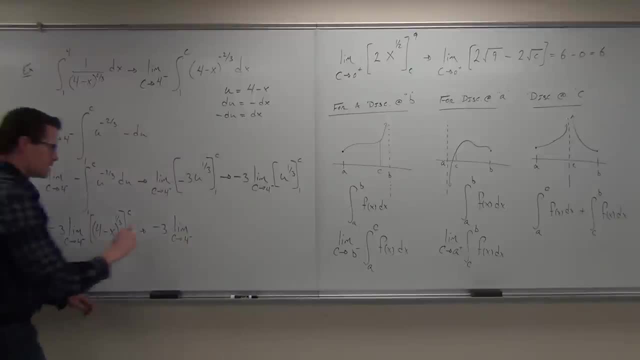 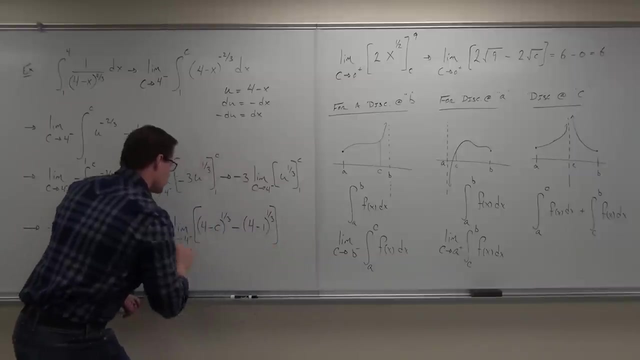 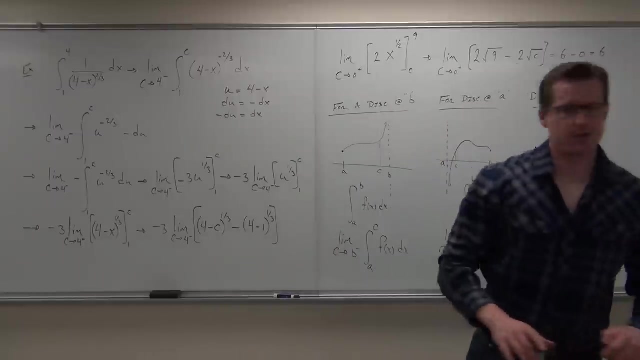 What goes in first, the C or the 1?? The C: 4 minus C to the 1 third, minus 4 minus 1 to the 1 third. This is the point where you can start to evaluate your limit. Notice, we've had to write limit every single time until we get right down to here. 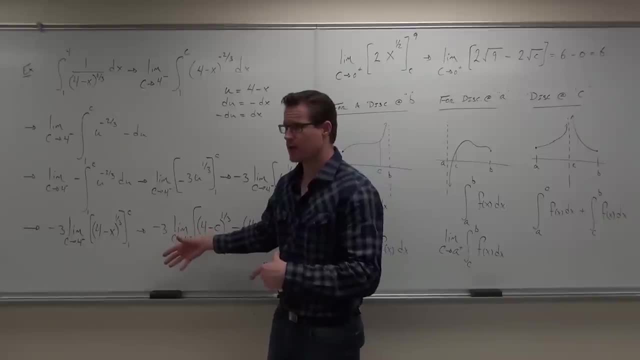 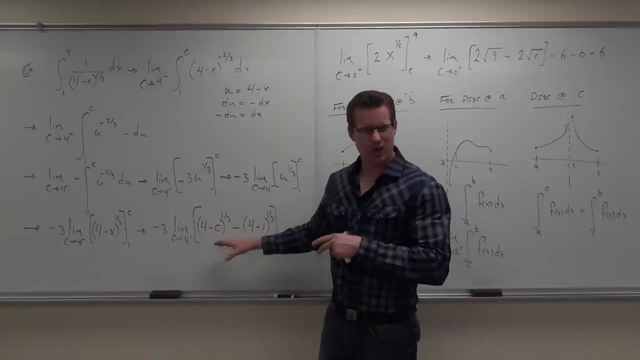 because we haven't thought about what's happening as C is approaching 4 yet. So this right here, look it. This is your definite integral. This is evaluated on your definite integral. Does that make sense? This is where you say: okay, now what was happening? 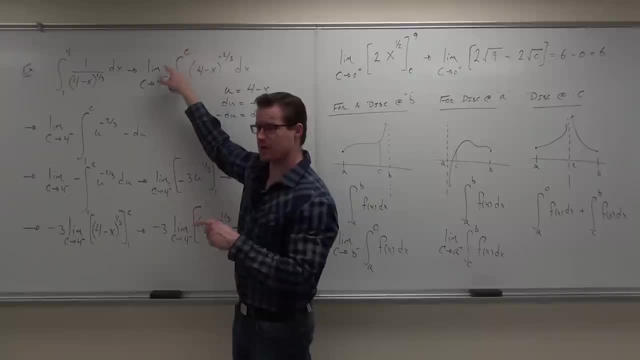 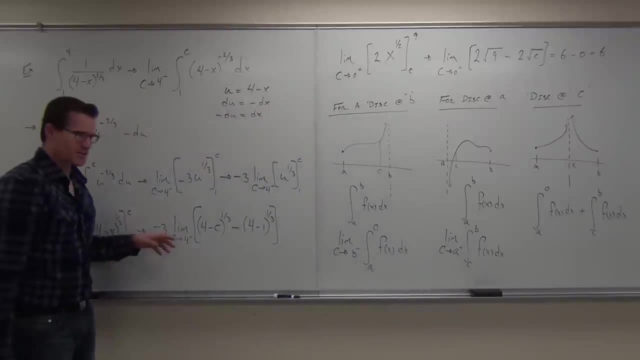 C really wasn't just the number I wanted to stop at. C was something I wanted to go to: 4 from the left-hand side. Does that make sense to you? So let's see about the C. What's happening to the C? 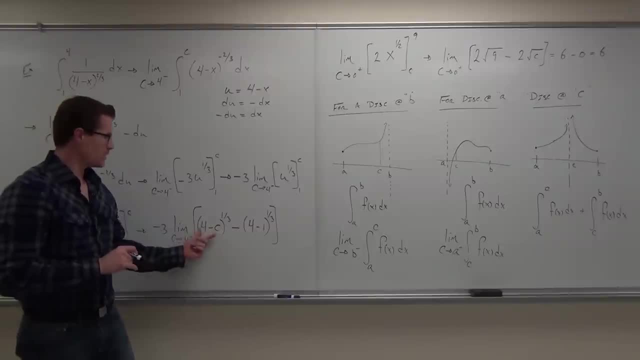 It's getting really close to 4.. Really close to 4.. What's 4 minus something, really? and when I mean really close, I mean it gets to 4. practically speaking. How much is that? 0.. So this thing is going to go to. 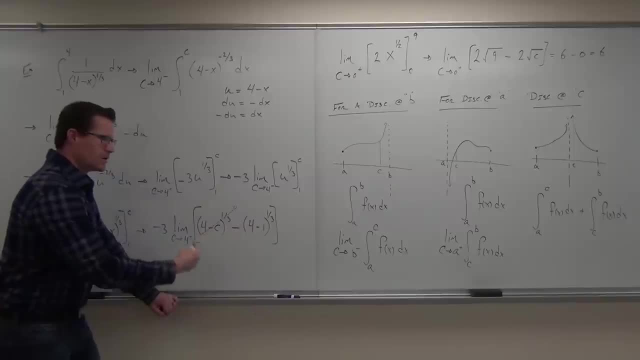 0.. 0.. Since C is going to 4 from the left-hand side, this thing is getting really close to 0.. 0 to the 1 third is still 0.. So we're going to have- don't forget about this negative 3.. 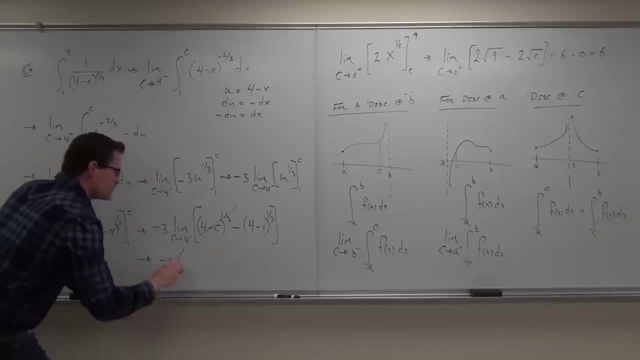 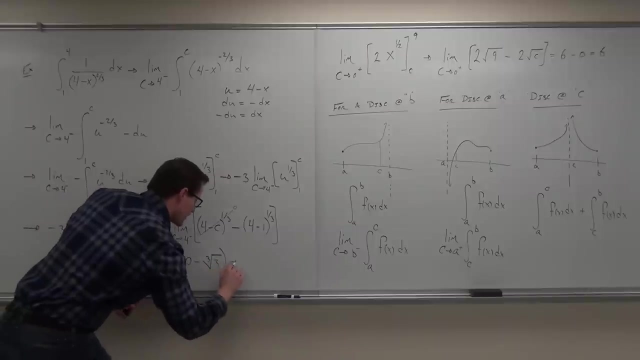 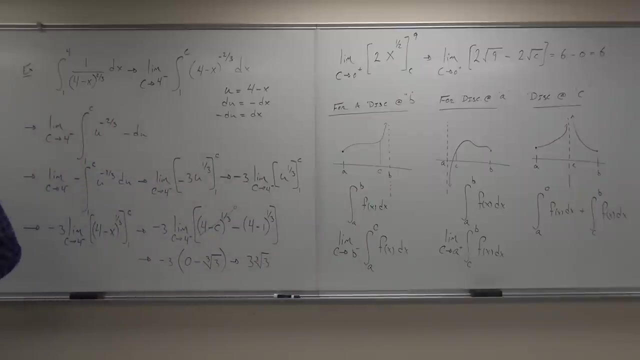 It's still there. So we have negative 3 times. this is 0, minus. how much is this going to be? Cube root of 3.. Cube root of 3.. Cube root of 3.. Altogether we have 3 cube root of 3.. 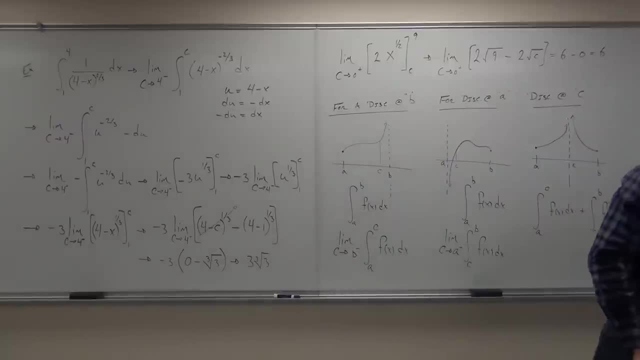 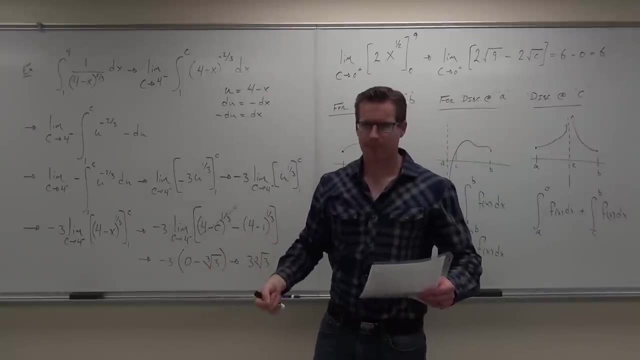 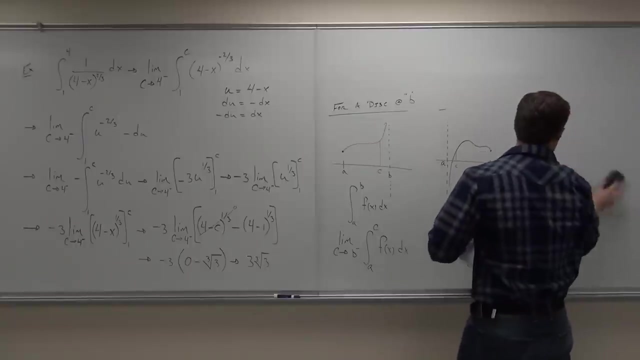 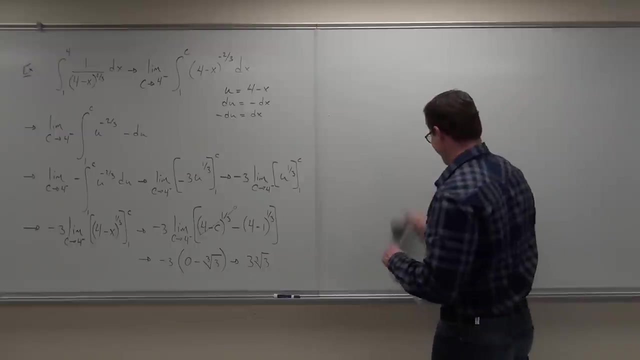 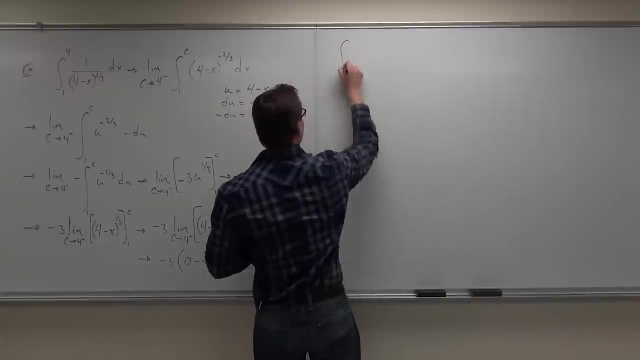 This part should be pretty easy. Chopin should be okay with this stuff. Can we move on just a little bit? Okay So moving right along. Questions All gone. already Have I taught you what the integral of L and X is. 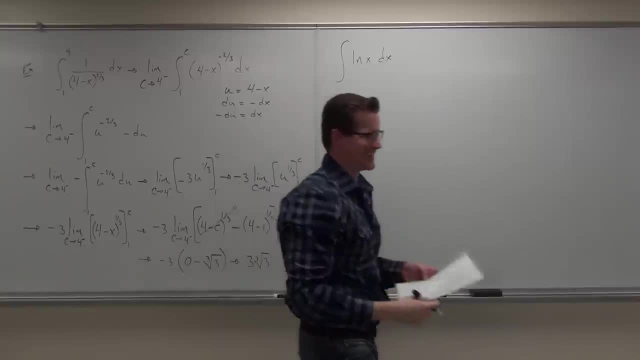 Have we done that in this class before? 1 over X, right? Oh no, we haven't. The integral of 1 over X, not the derivative of L and X, The integral of L and X. Have we done that? 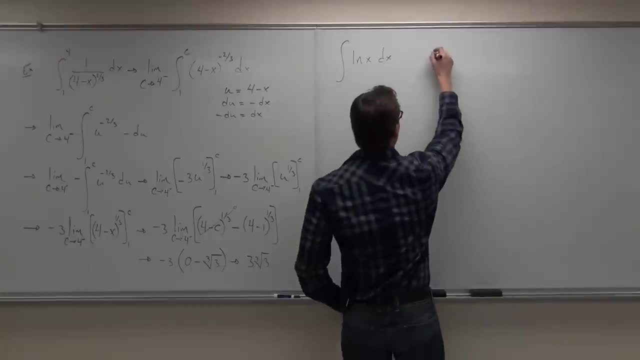 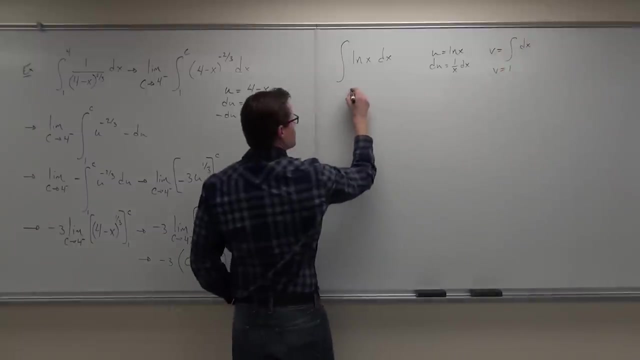 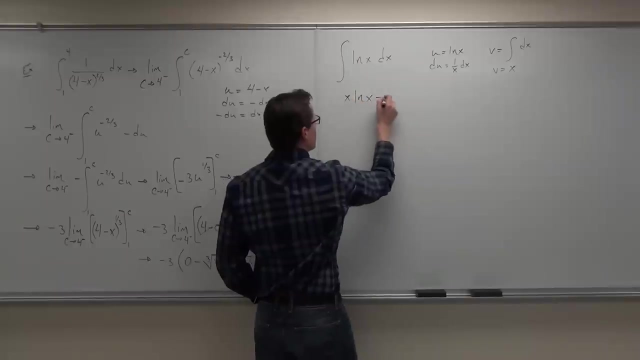 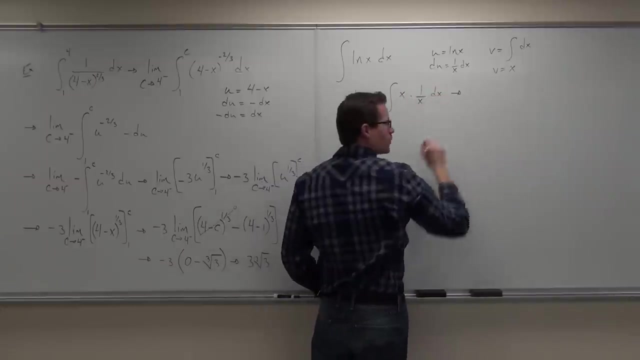 No, I think we've done it once. Yeah, Yeah Sorry. U times V minus the integral of V du. What am I doing up here? Magic Partial. We should do magic Integration by parts. U times V minus the integral of V du. 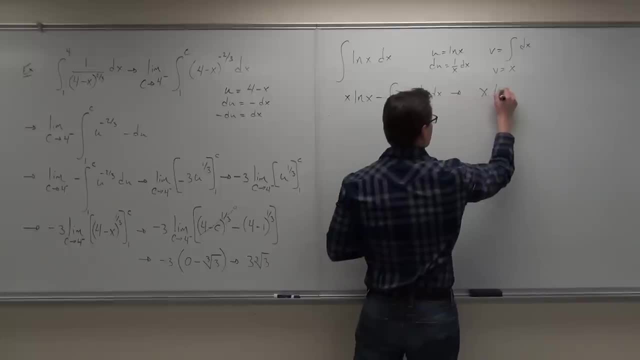 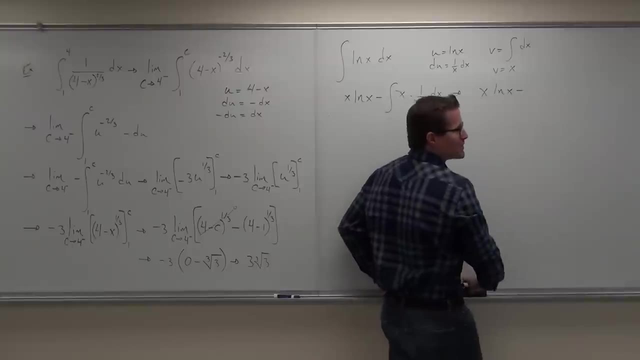 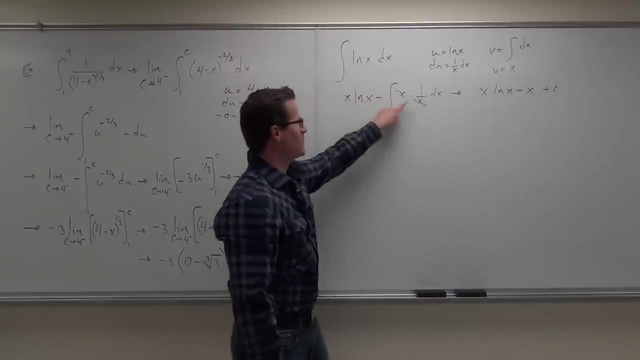 This is 1. You know I never miss those C's. Sometimes I do the wrong thing, but I never miss those C's. We get X, L and X minus X. Do you guys see where the X is coming from? It's just basic integration by parts. 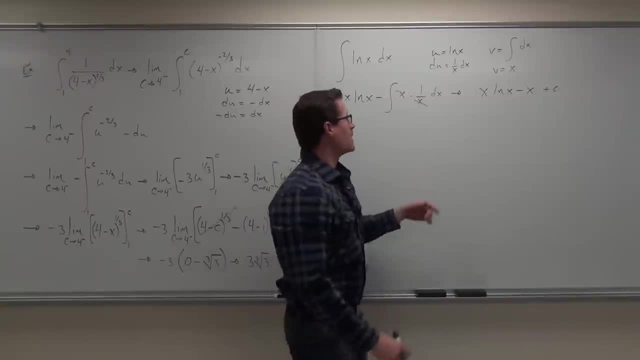 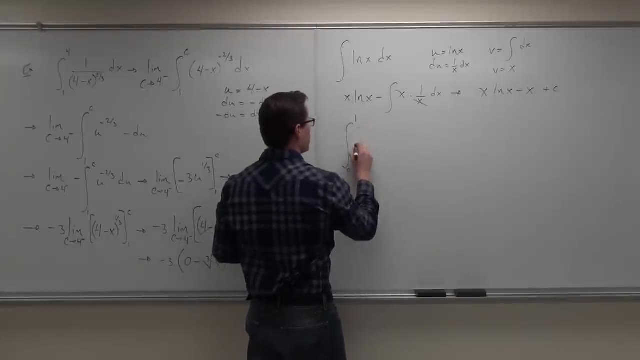 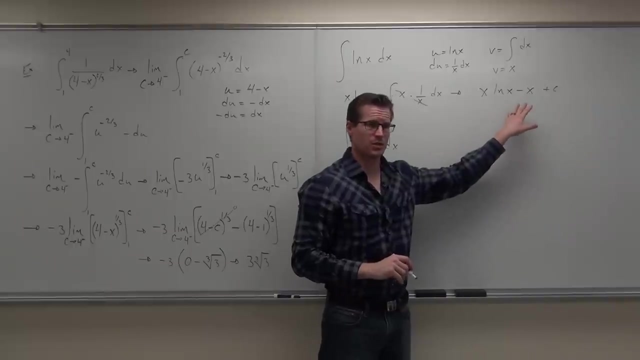 I know we've done it at least one time before, But what that means is that if I wanted to evaluate this limit from 0 to 1 of L and X dx, now I can use this formula. basically I wouldn't have a C, but now I can use that. 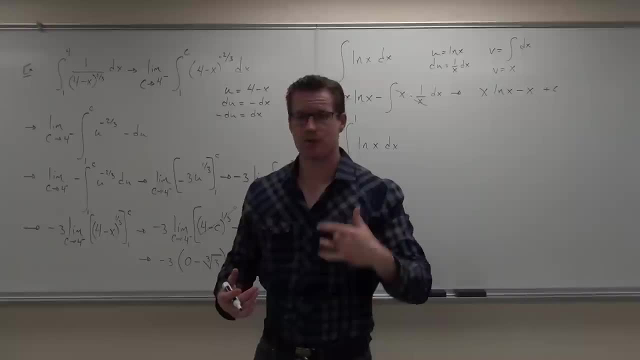 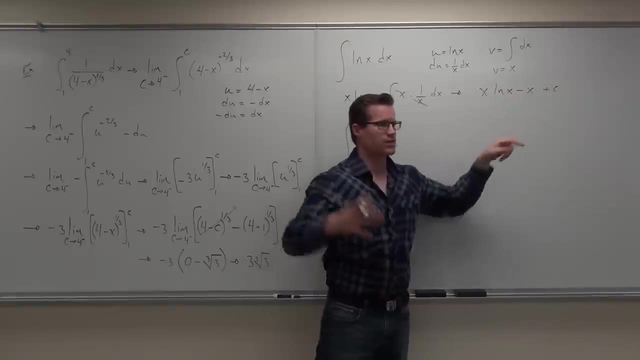 So whenever you see the integral of L and X, if you want to memorize this, that's fine. Integral of L and X is by integration by parts X, L and X minus X. I know I did it fast, but we've done it one time before. 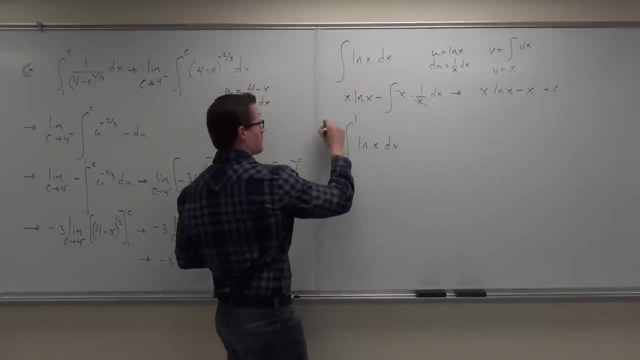 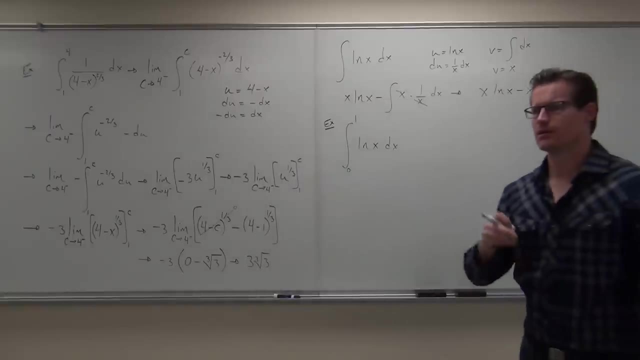 So let's look at the integral from. let's look at the integral from 0 to 1 of L and X. Firstly, is this an infinite interval or is it an infinite discontinuity? Infinite discontinuity? Very good. Where is the discontinuity? 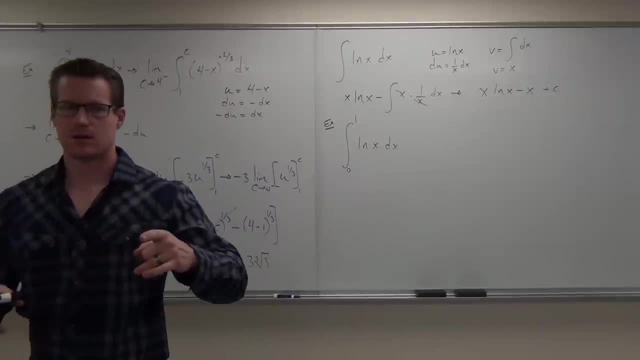 0, 1, or somewhere between 0. 1.. 1. What's ln of 1? 0.. Then it's defined: Oops, What's ln of 0?? Error Syntax. error Syntax. My calculator won't do it. 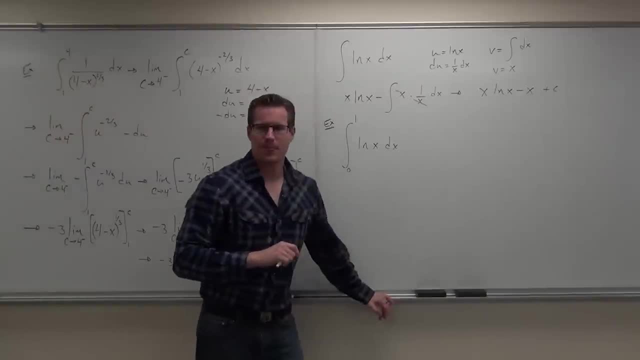 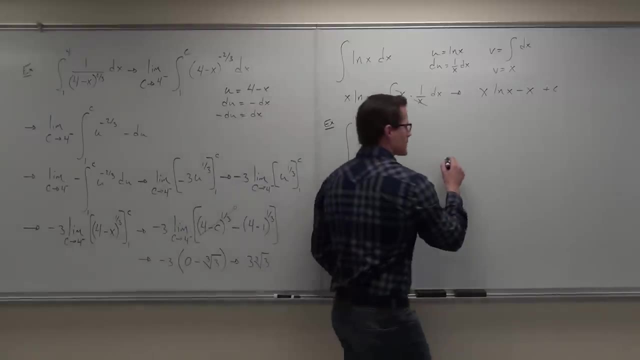 I don't know. Do you know what ln of X looks like You better? Yes, It's the inverse of e to the X. So if e to the X looks like this, ln of X looks like that. Now you all think that it's undefined at 1. 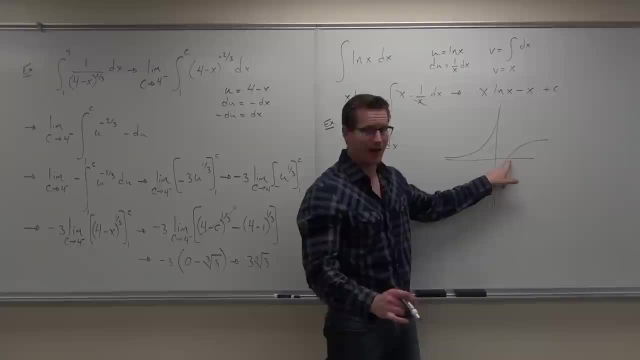 because when you plug in 1, you get 0. That's not something that's undefined, It's actually defined. But the definition is ln of 1 is 0. That's not a problem, It's at 0. What our problem is is at 0 from the right-hand side. 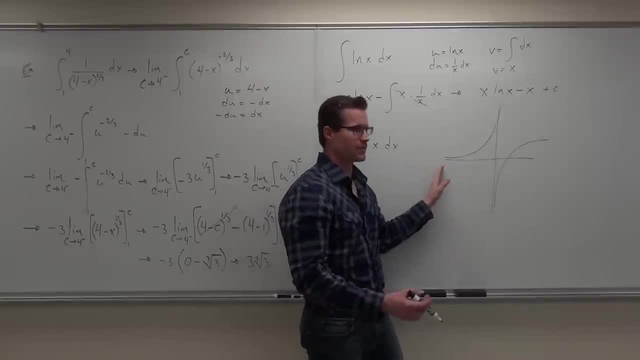 That's not a problem. ln isn't even defined on this side, Not even defined at all. OK, So our problem here is: Oh, your problem here. I don't got a problem here. I'm good, All right, But it's not at 1.. 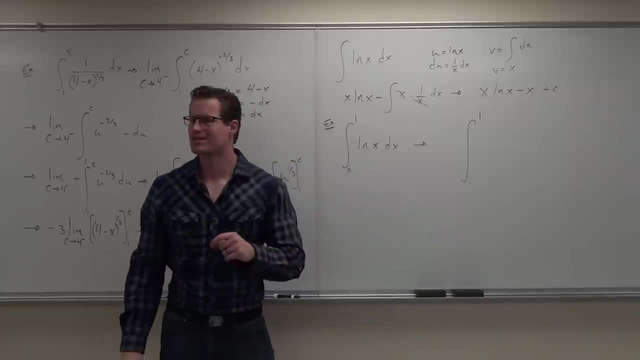 1's good. We're good at 1.. We're not good at 0. So help me out with it. What do I call the 0?? What am I going to make it? Make it C, Make it C. 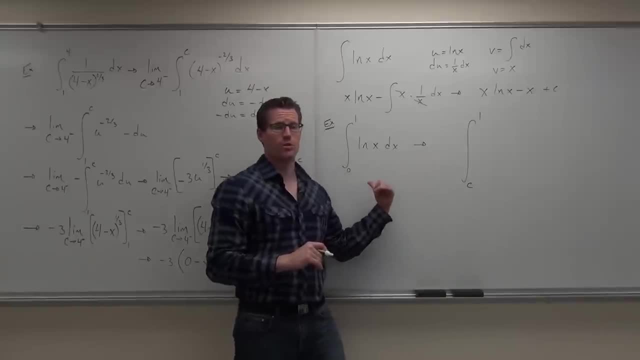 Yeah, I'm not making it A because I'm not letting this number go anywhere. I'm not letting it go to infinity or anything. I'm calling it C because I have a number between 0 and 1 right now. Does that make sense? 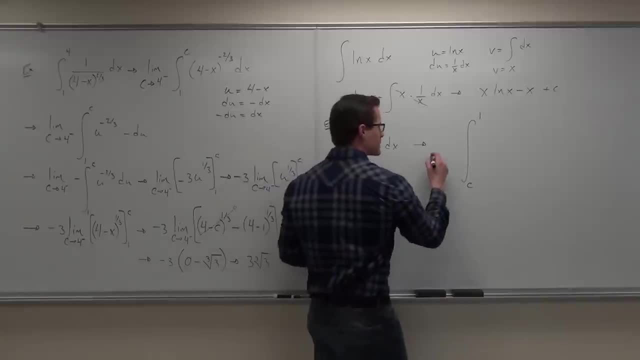 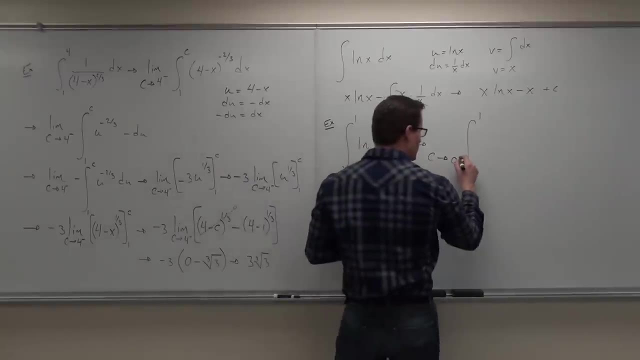 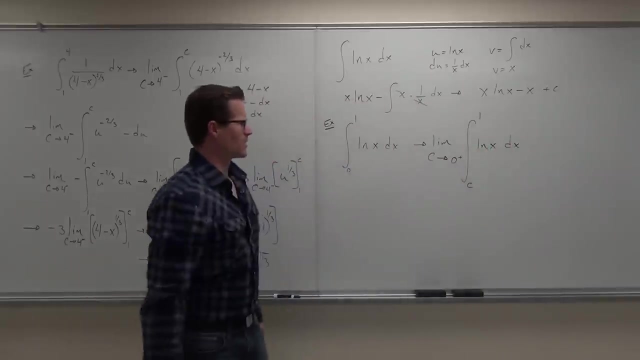 It's between 0 and 1.. Now, where do I want that C to go From? the right, Right I mean correct, And the limit lets us do that. I made a really big integral, didn't I Make sure you know that's an integral. 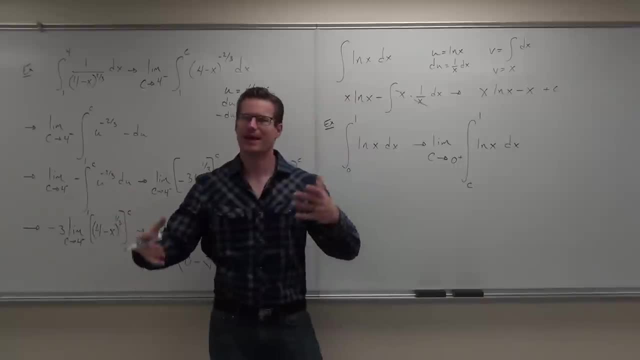 Quick show of hands should be OK with that one so far. So 1's good Man. it'd be kind of worse in this case scenario to pick the wrong thing right Go. oh, this is completely undefined at 1.. 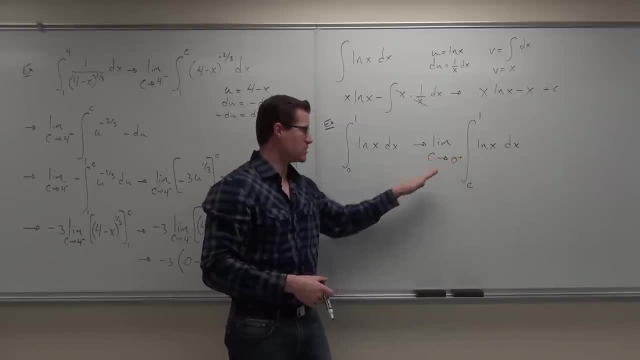 No, it's not. It's greater than 1.. It's not greater than 0, because it goes to negative infinity. That's a problem. So we say: hey, 0 to 1? No, no, no, Call it a number. 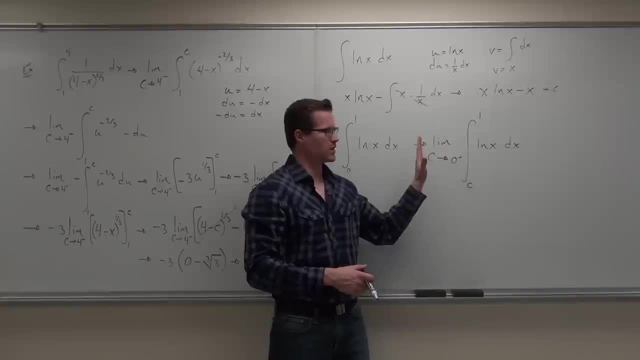 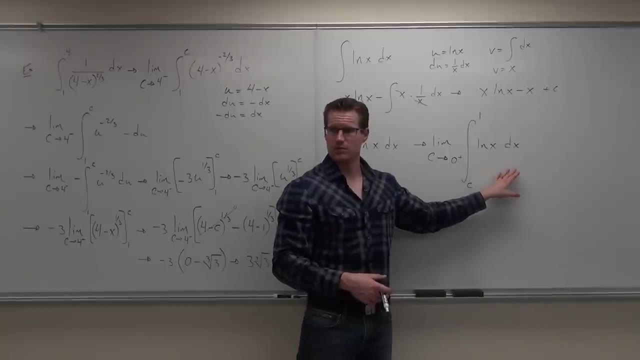 C to 1.. Somewhere just before 0, as we're going from the right Just before 0.. Do your integral, because we have a definite integral now. After that you go. OK, cool, After you've done your definite integral. 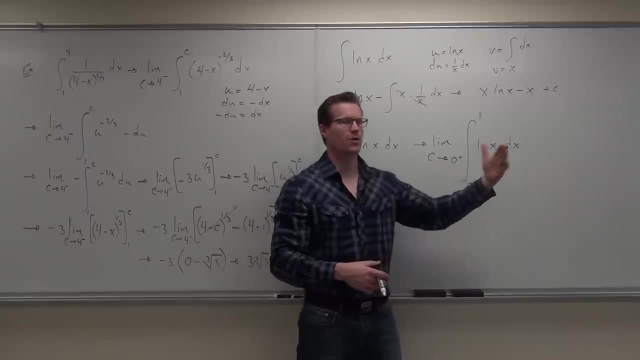 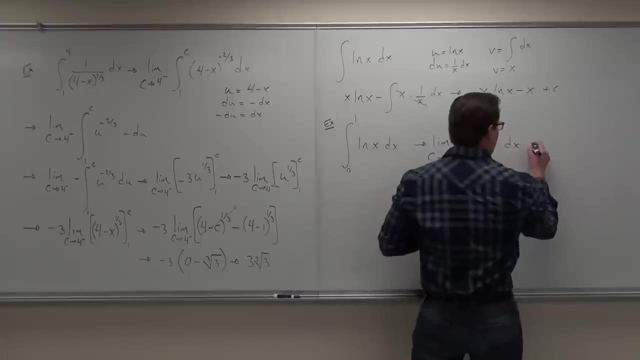 where do you want the C to go? Now? we want the C to go to 0 from the right-hand side. This is the idea. Do you get the idea? Are you sure you get the idea? Yes, All right, So now that I've shown you. 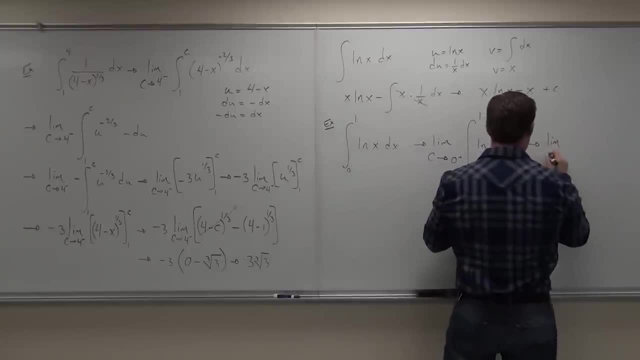 how to do this integral. no problem, You've got a limit. as C approaches 0 from the right, The integral of ln x is x, ln x minus x. We do not need the plus C because it's a definite integral. Where is my bounds of integration? 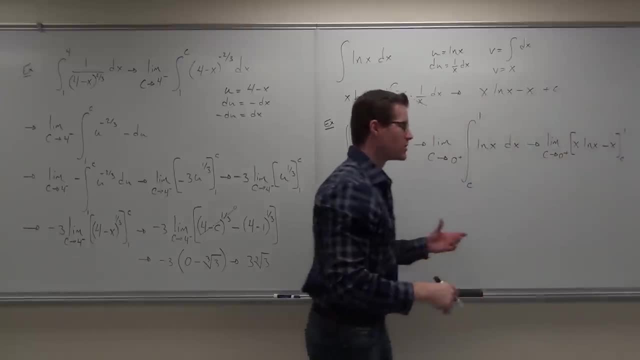 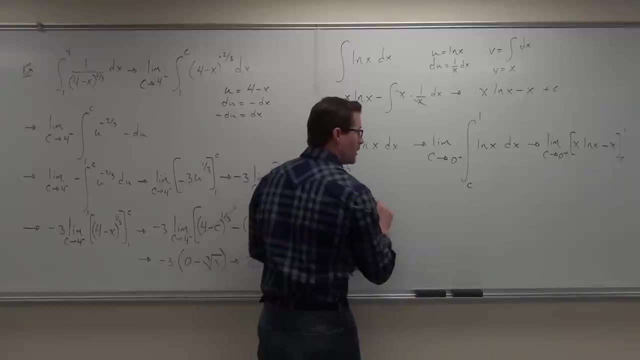 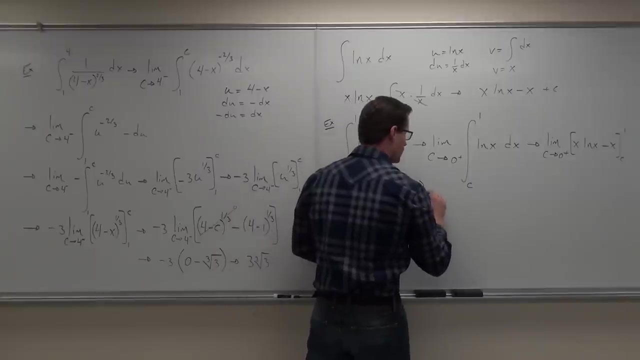 From where to where? C to 1.. Which one do I plug in first, 1.. Very good, So this will be a limit. as C approaches 0 from the right of C times ln, C minus C. I was just checking to see if you were paying attention. 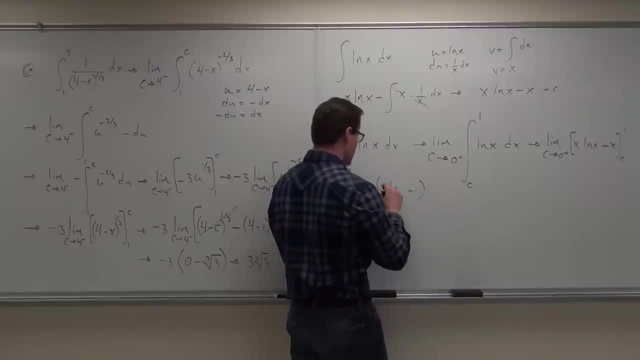 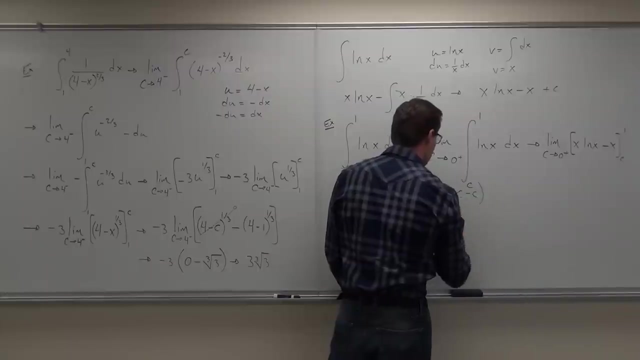 I didn't even write the C's, I wrote the x, for some reason not the 1.. 1 ln 1 minus 1.. I even asked you that question, didn't I, Silly old Leonard. Okay, Now we'll have C ln. C minus C. 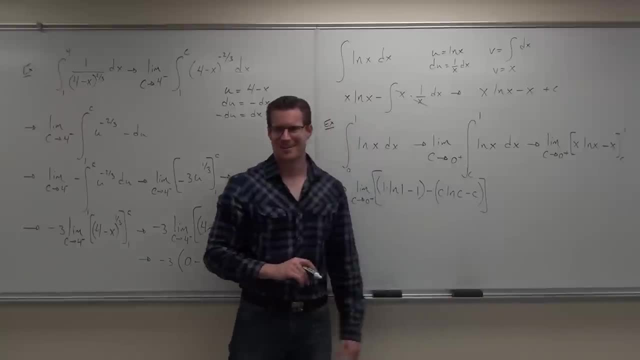 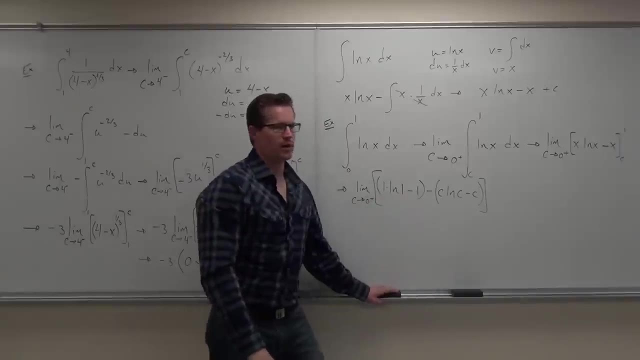 Can you see why this is correct, Anyway? So can't you be all right with that so far? Now let's start simplifying this thing. What happens with ln 1? 0. That's 0.. What happens with? Oh goodness gracious. 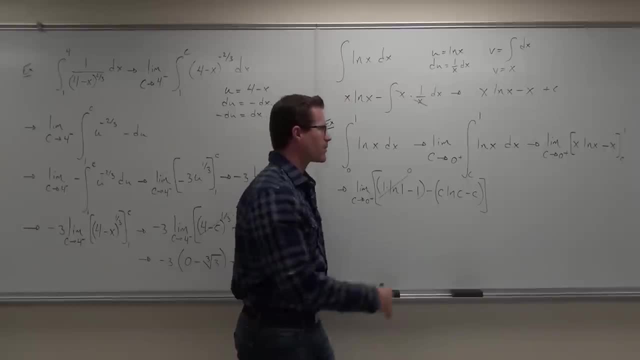 You know what We're going to do. one more thing with this. So we know that's 0.. I'm going to rewrite this just a little bit. I'm going to write this as limit as C approaches 0 from the right of. 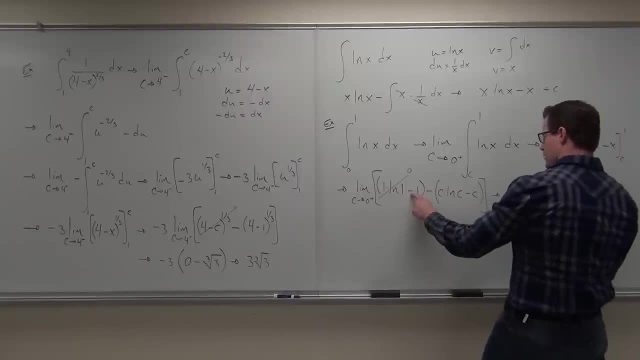 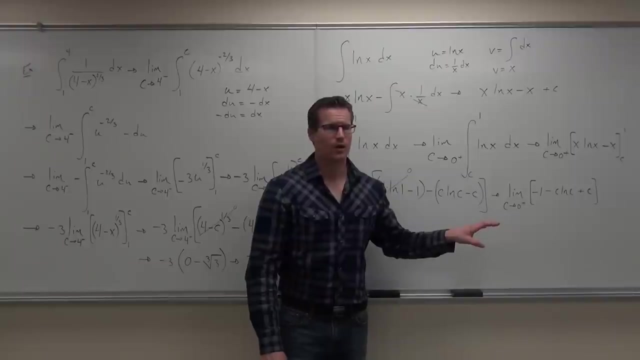 Let's do this. Let's do negative: 1 minus C, ln C plus C. Are we okay with that? so far, Hello, Yes or no? Yes, Okay, Now you can't make up your own math on these things. Some are going to be easy little parts. 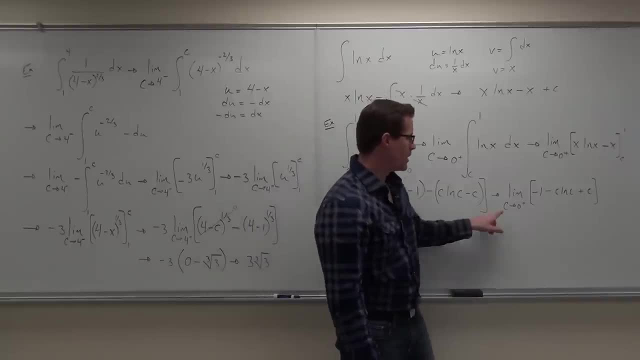 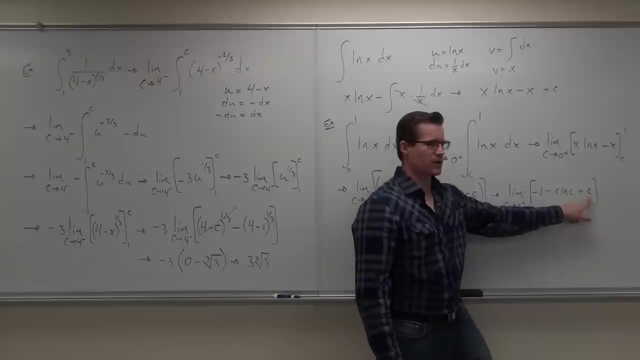 Some are not going to be so easy. You're going to have to do some things with it. So let's look at this. What's the limit of negative 1? Easy. What's the limit of C, as C approaches 0 from the right? 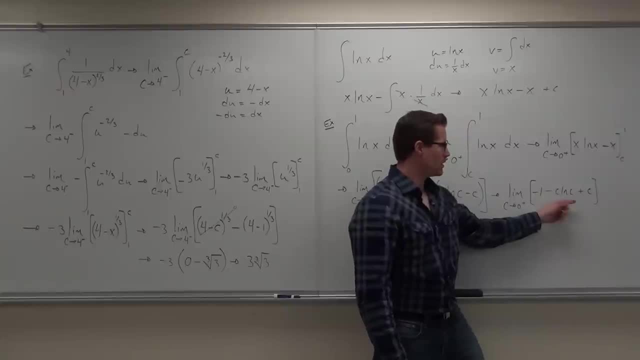 That's 0.. This one, Oh, This is 0 times negative infinity. That's an indeterminate form of 0 times infinity. We'll have to rewrite that one. You guys follow me on that one. You can't do 0 times. 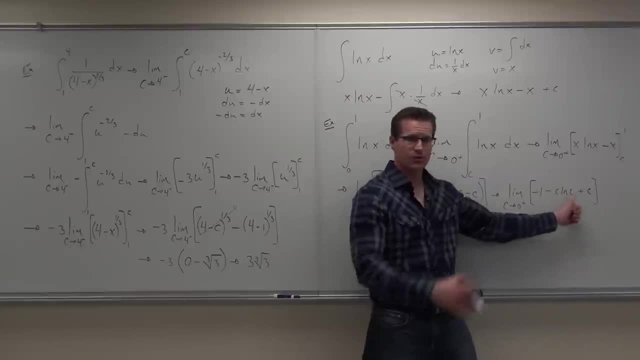 You should know that ln of C, as C approaches 0 from the right, goes like this to negative infinity. You can't do 0 times infinity and know what that is without doing this. You've got to actually go through it. Am I getting through to you a little bit? 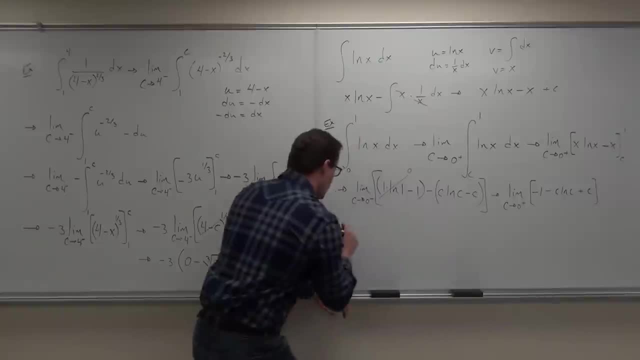 You've got to do the indeterminate forms like we've been practicing. That's why we did that was to get here. So we're going to have This is still negative 1.. This goes to 0.. We're going to have negative 1. 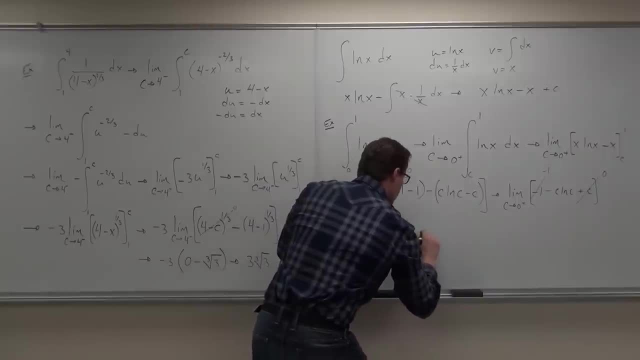 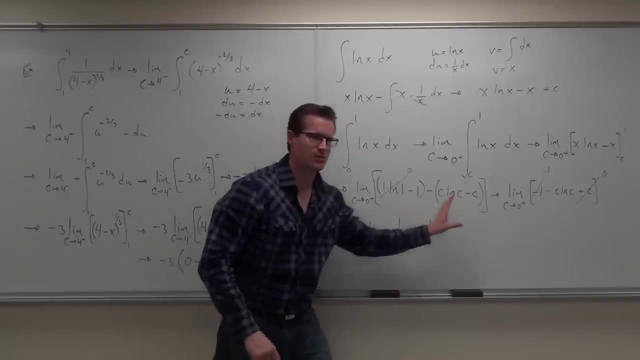 minus the limit as C approaches 0 from the right of C, ln, C, and then well, plus 0.. That's gone. So really I just need to focus on this thing. I'm going to take it off to the side here real quick. 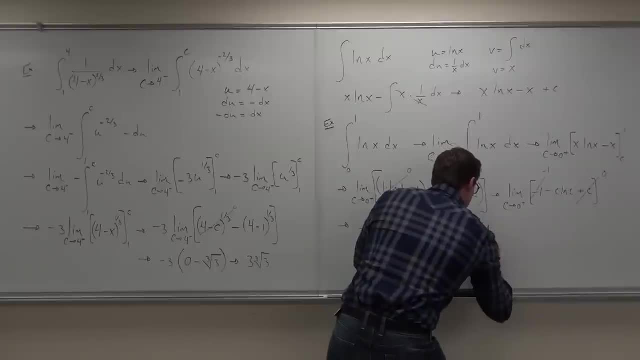 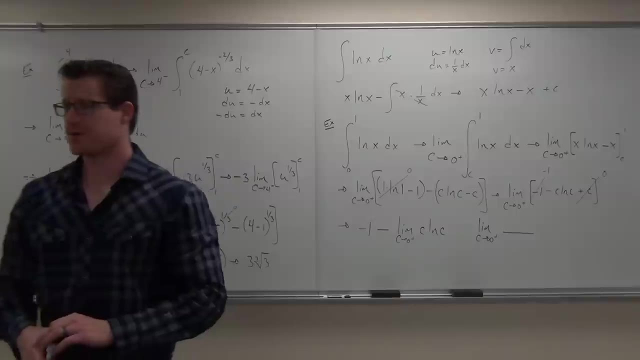 Use a different color here. The limit as C approaches 0 from the right. If you remember anything about indeterminate forms like 0 times infinities, or 0 is 2, the whatever. we're trying to make a fraction out of it. 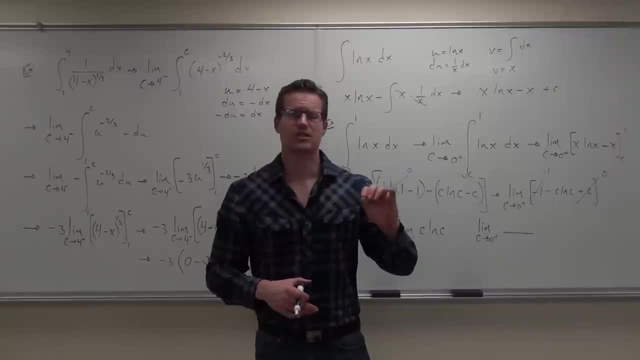 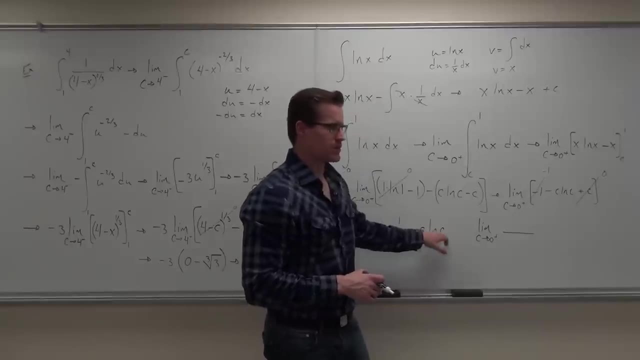 of 0 over 0 or infinity over infinity. Explain to me why we're trying to make a fraction out of it. Very good, So never want to move ln to the bottom. We found that out when we Remember doing E to the ln of the bunch of junk. 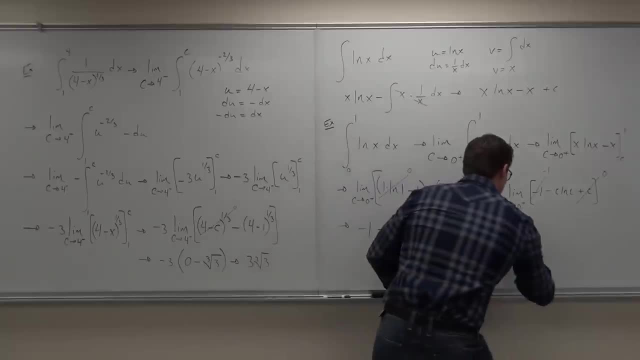 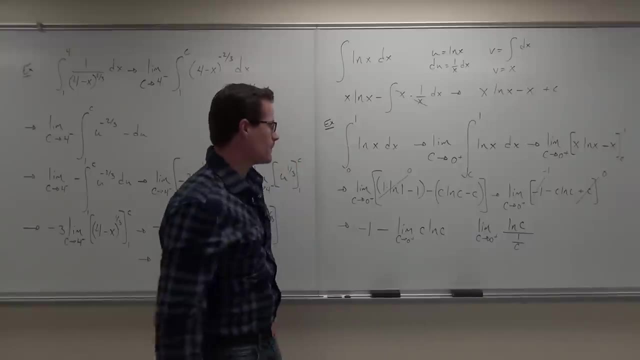 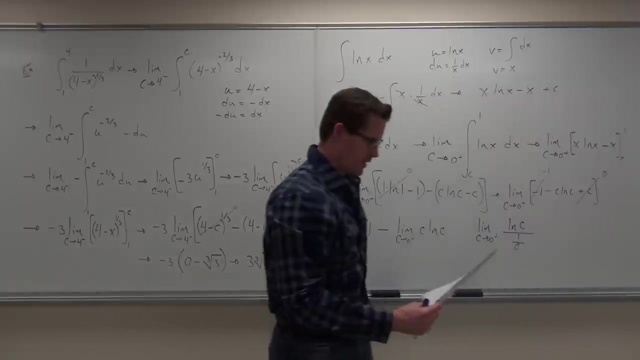 We never move ln, We always move the other thing. So this: you leave this as ln C over 1 over C, which was the idea. You can, but you're going to be doing a derivative right now. Now let's identify this. 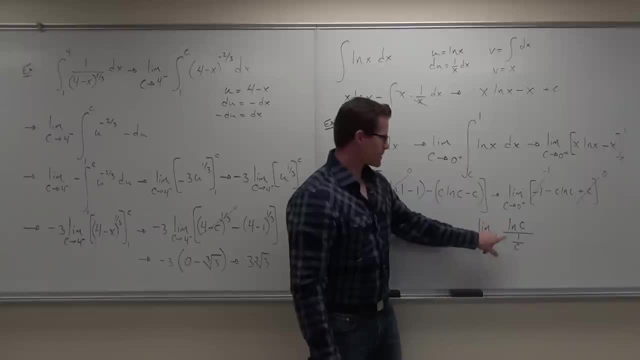 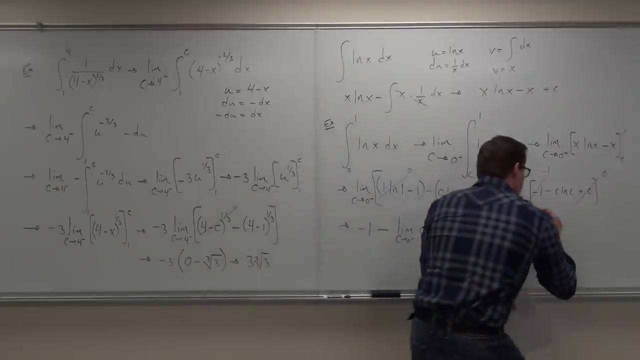 What is, What is this as we go from? This is infinity. This is negative infinity As we get really close to 0, this thing's also infinity. If this is infinity over infinity, we can use. So this was infinity over infinity. 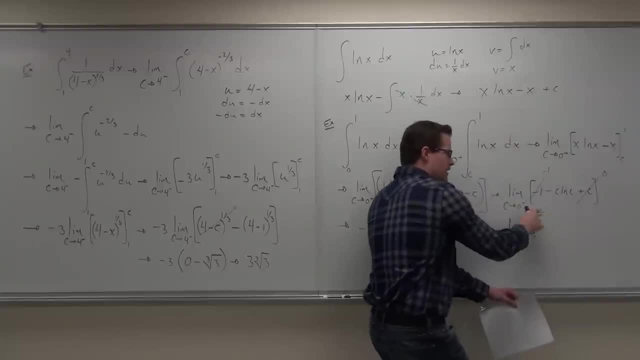 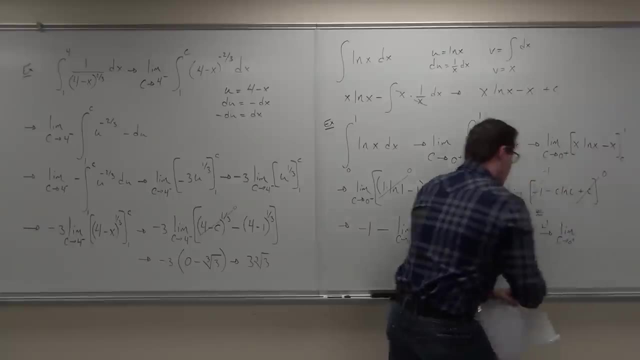 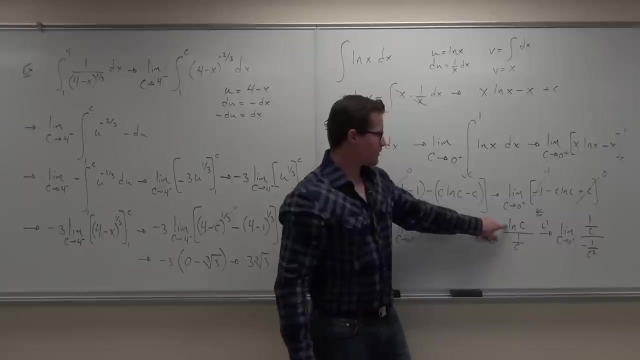 A weird infinity. This was infinity over infinity. So with a L'Hopital's rule- I'm going to do L'Hopital's really quick- We get 1 over C over negative, 1 over C. squared Derivative of ln C is 1 over C. 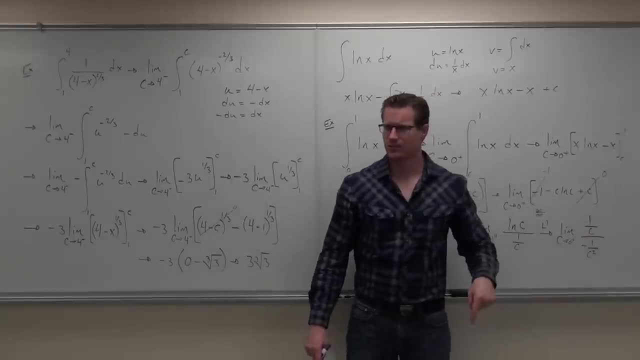 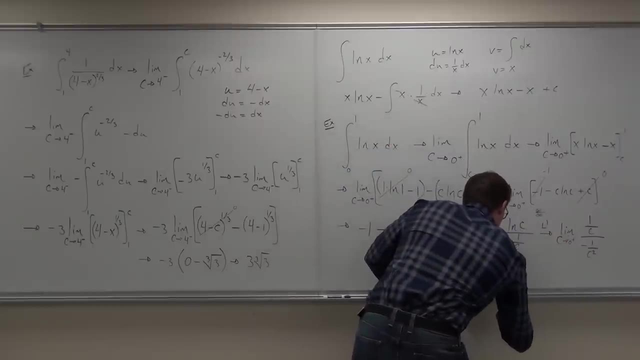 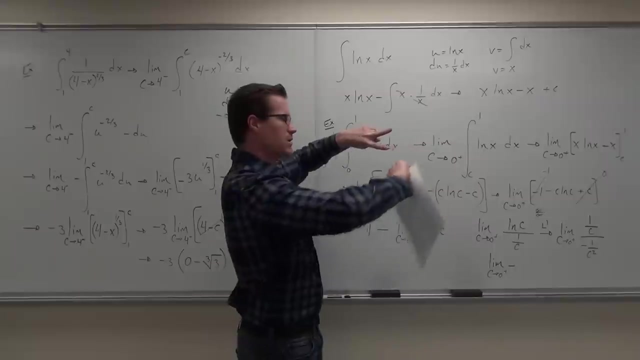 Derivative of 1 over C is negative: 1 over C squared. You guys, okay with that one. Can you simplify that? Of course you can. Let's see It's going to be negative. 1 over C over 1 over C squared. 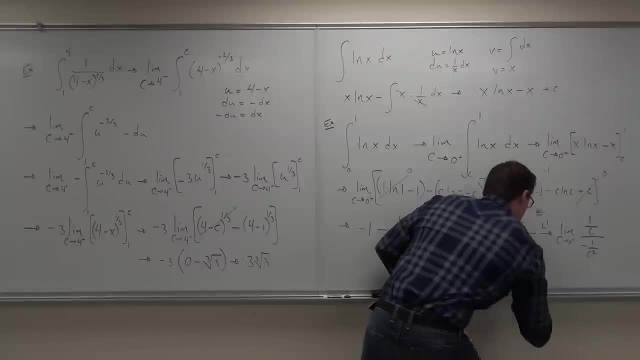 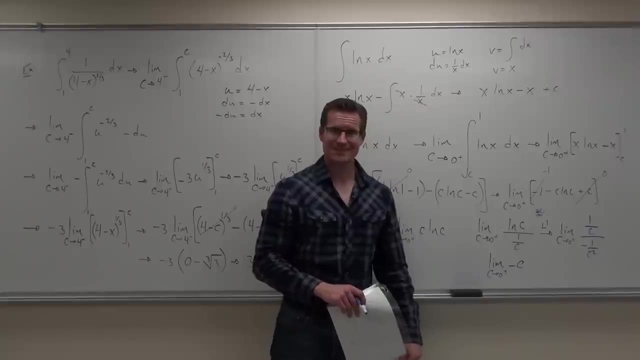 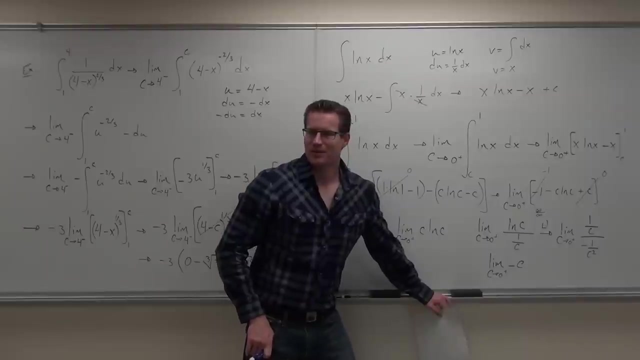 Simplify and multiply C. If you simplify this, you're going to get negative C. Got it. C, C, C. Now what's happening Are we really okay with? Can you see Those three different C's? 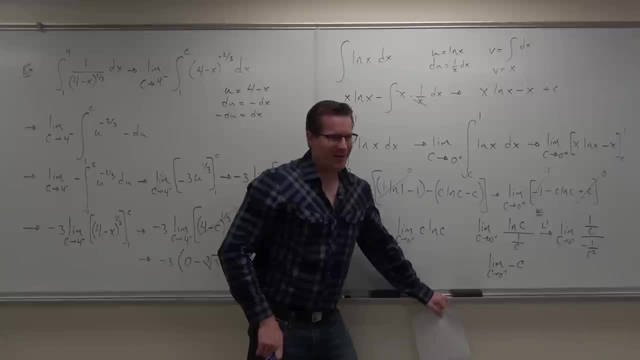 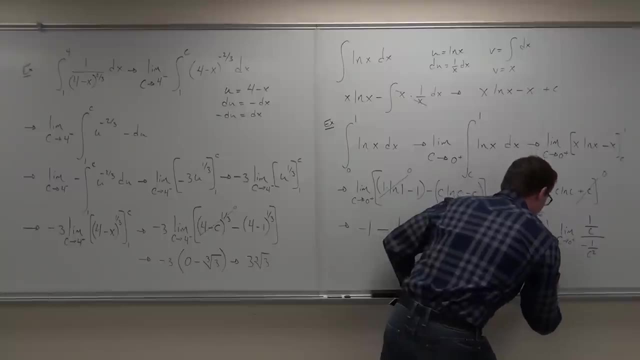 I see what you did there, Thanks. So what's happening to our C? as C approaches 0 from the right, This thing is going to negative 0. Well, I don't care about negative 0. 0. So this whole thing is 0.. 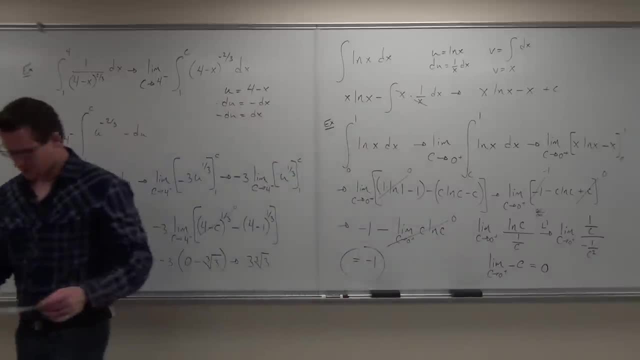 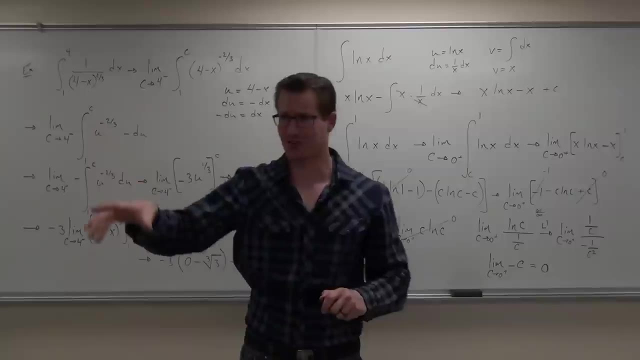 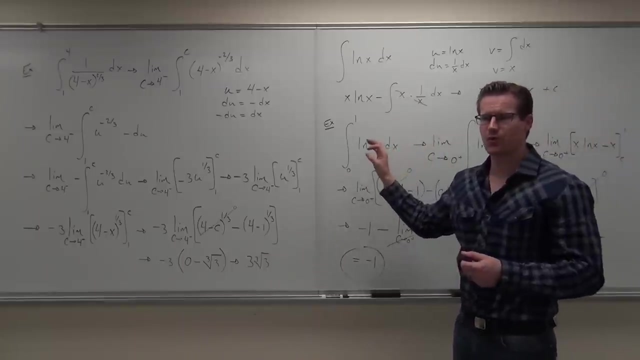 And we get negative 1. Crazy. Could your hands feel okay with that one, Are you sure? So the idea is, man, you can do all these intervals. They're pretty easy. Be careful with how you set it up. Identify where the infinite discontinuity is. 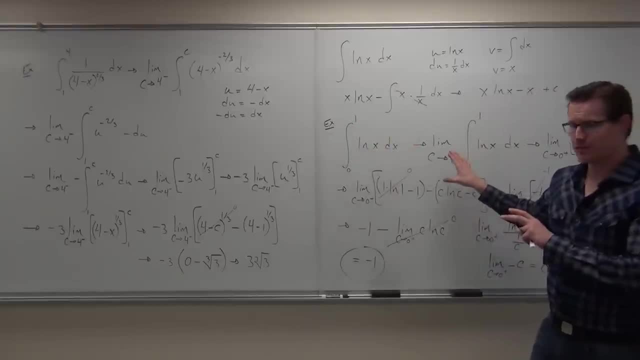 That's important. If you can do that, you get your correct limits. Okay, After that, man, you can't cheat at your limits. Don't make up your own math. Do them the way I showed you, with indeterminate forms. 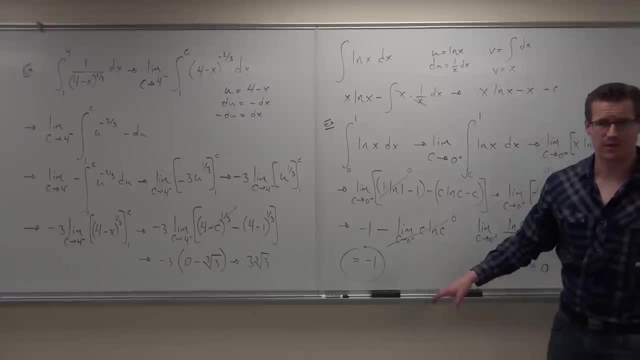 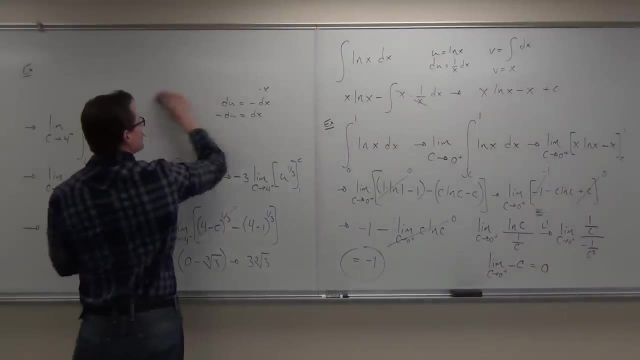 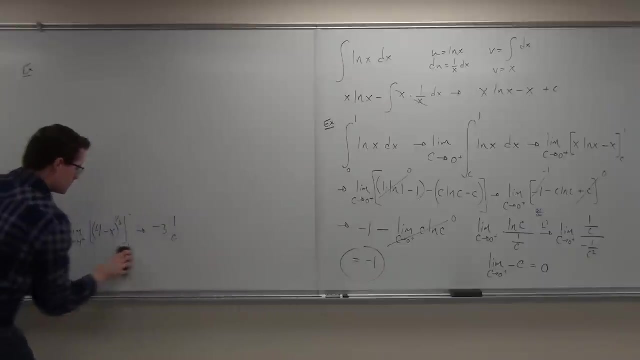 Okay, Really, make sure that you know how to do those limits and refresh your memory on the section of indeterminate forms. So let's do two more. We'll talk about one, We'll actually do another. See if you're really really with it here. 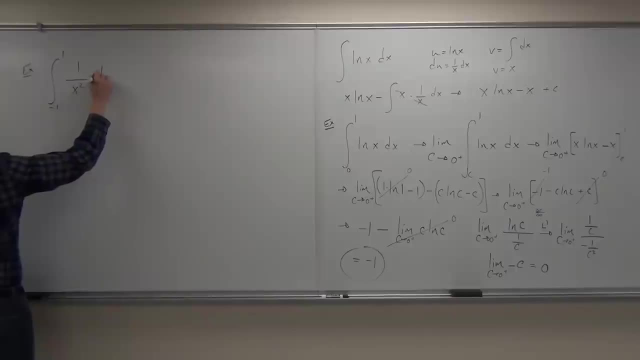 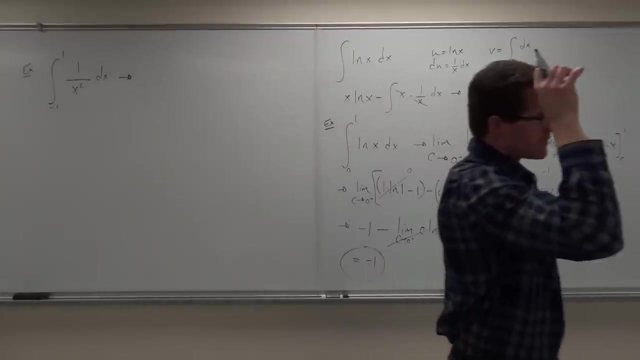 We're not going to finish this, but I want to see if you understand what to do. Integral from negative 1 to 1 of 1 over x squared is x. Integral of negative 1 to 1 of 1 over x squared: dx. 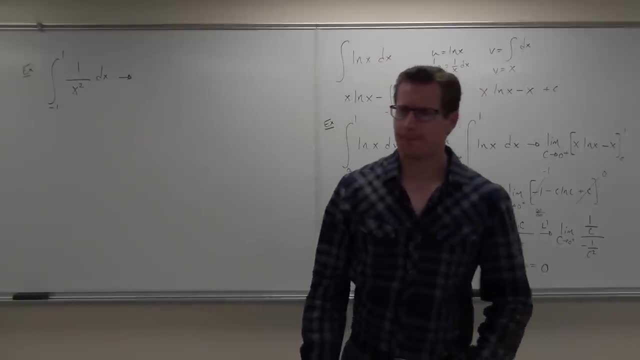 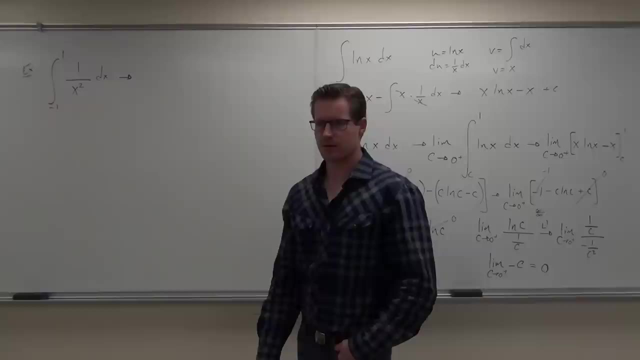 Infinite interval, Infinite discontinuity. Neither Both. Infinite interval, Infinite discontinuity. Is there a problem in our function Where Zero is a problem? Do you see what I'm talking about? The zero, Zero is a problem. This is what I'm talking about. 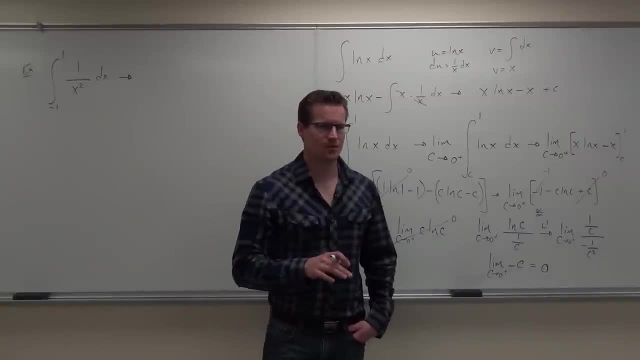 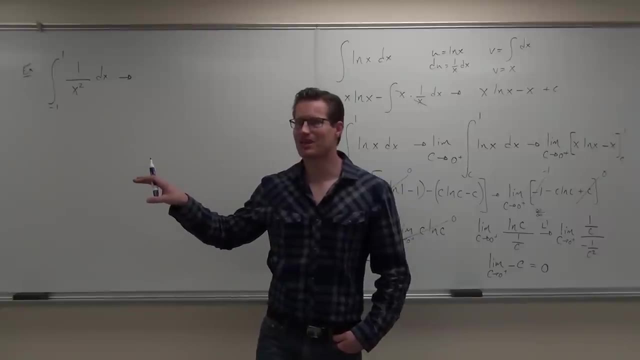 You can't just blindly integrate with definite integrals In calculus 1, you can, because you don't cover this idea, You go: okay, I'm just going to assume I can do it, But here you can't do that. 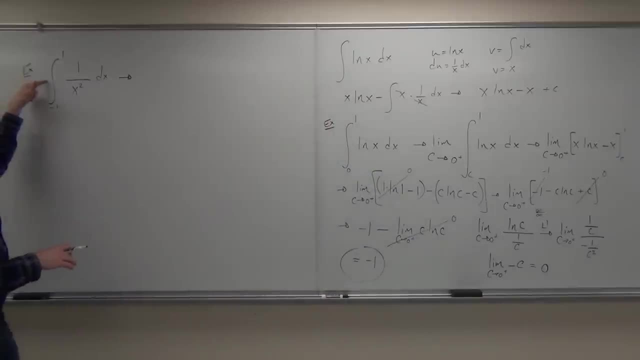 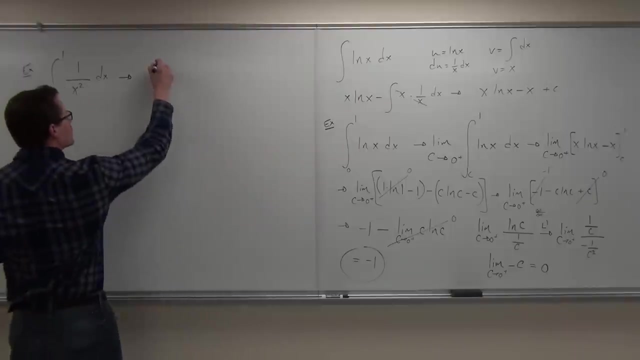 Because now, well, can you plug in zero? Goodness gracious folks, we're going over an interval where this function is not even defined. What that means is that we have this third situation, where we've got a negative 1 to 0. 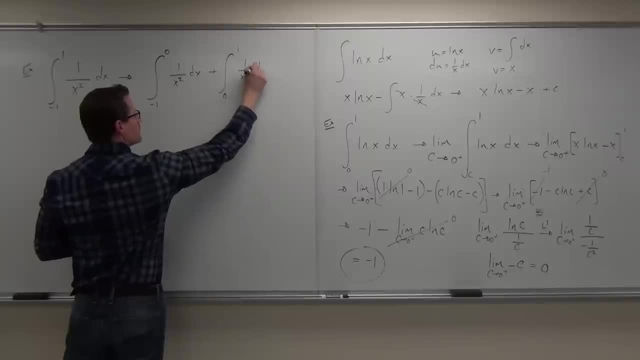 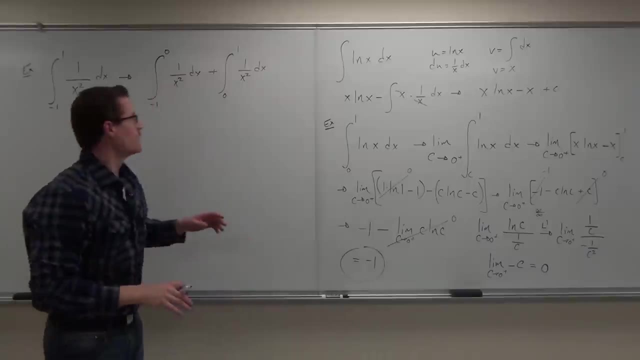 plus a zero to 1.. Chopin, do you feel okay with that idea? I'm not going to finish the problem for you. I think you can do it. Check it out. Ignore this side. Could you do this? Yeah, this would be. as c approaches, 0 from the left. 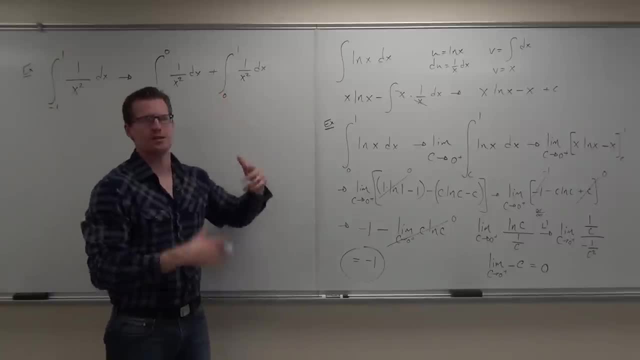 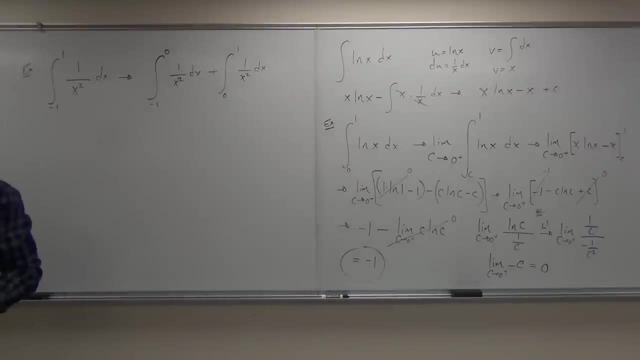 As c approaches 0 from the right, And then you do both of them and add them together if they both exist. Thanks for the emphasis on that one. Okay, last one: I have 84%. Last one, Integral from 0 to infinity, of that bunch of junk. 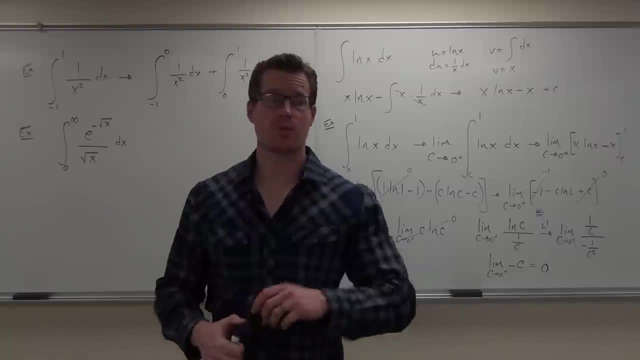 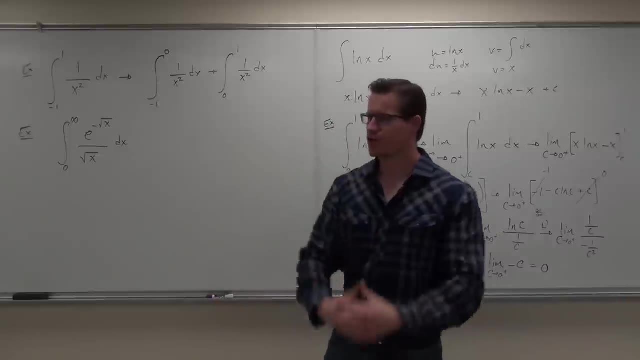 Oh my gosh. One of the most important things you can do is actually identify what is going on and what is wrong with your interval or your integral, or both of them. So what's wrong with this picture? Infinity, Infinity, Right off the bat, it smacks you right in the face. 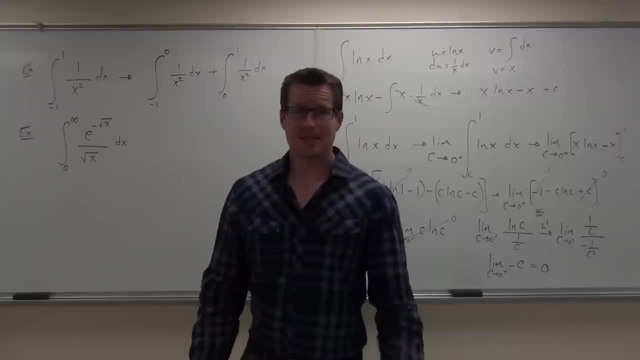 Boom, Got an infinity. Did that wake you up a little bit? So that's an infinite interval. We're going from 0.. 0 is great, all right. Well, 0 is great as far as the interval being defined. 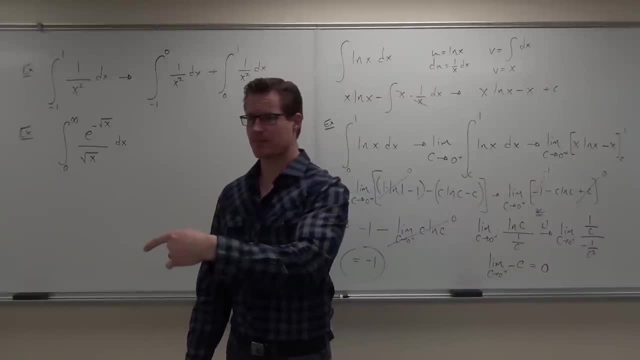 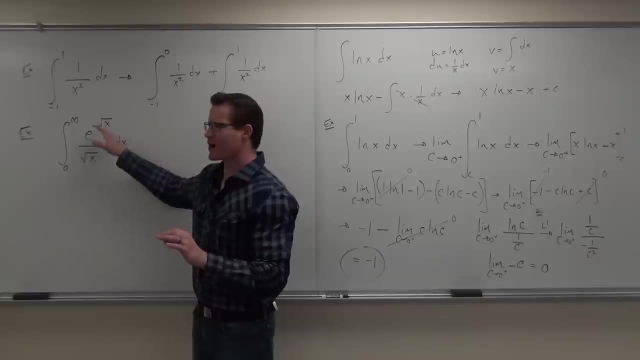 To infinity. that's going to be a problem. We're going to have an issue there. Does that make sense? Now there's another problem. What's the other problem? We're defined everywhere except at 0.. 1,, 2,, 3,, 4, boom, boom. 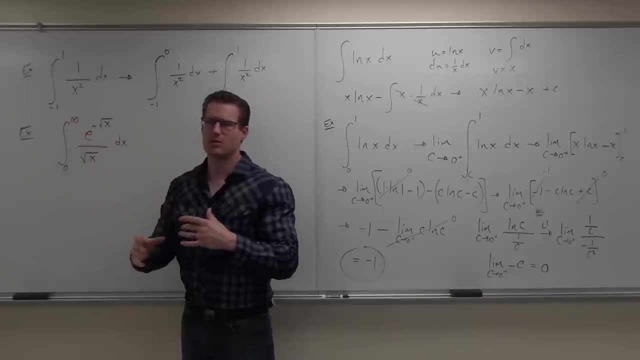 All the way to infinity is perfect, except with a 0. So here's how we can. You can take these ideas and roll with it. okay, I'm giving you kind of the basics here. So if you had started like, 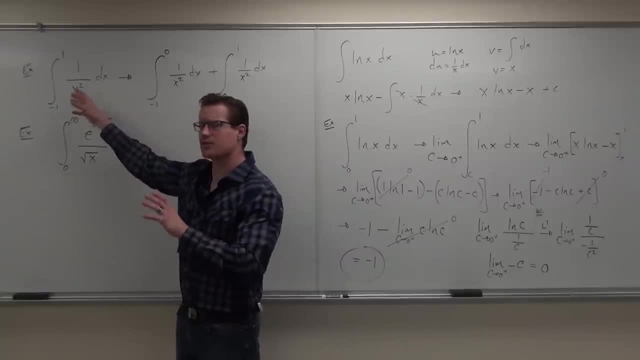 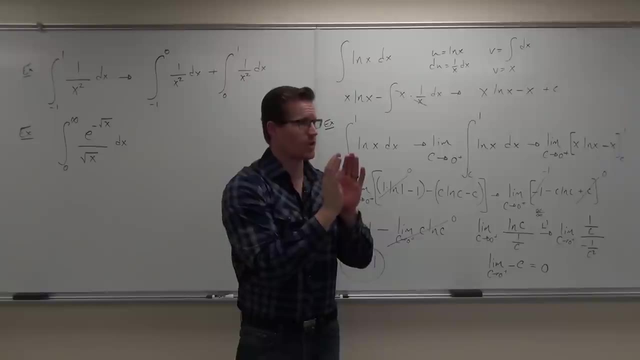 You couldn't start anywhere negative. but, like on an example like this one, if you had other scenarios, you got to break them up to where your interval is defined and do limits for where you are not defined. Is that clear? So in our case, we're going to say it's not a problem. 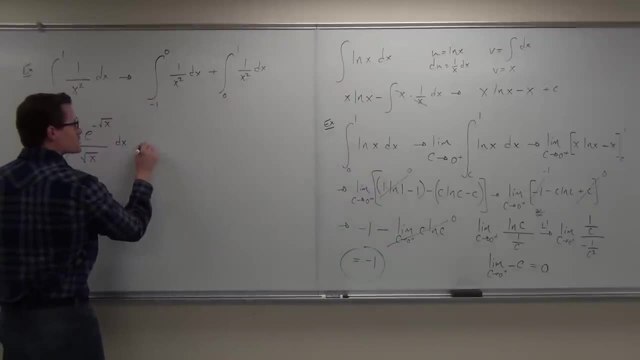 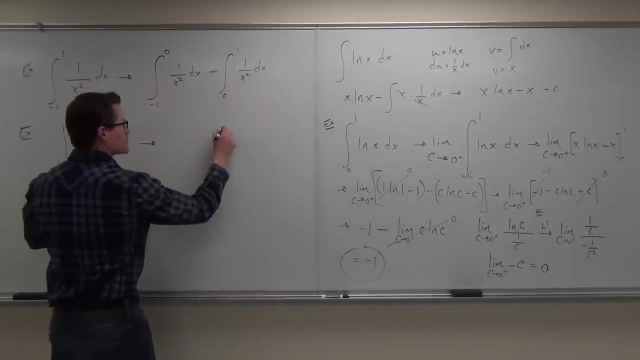 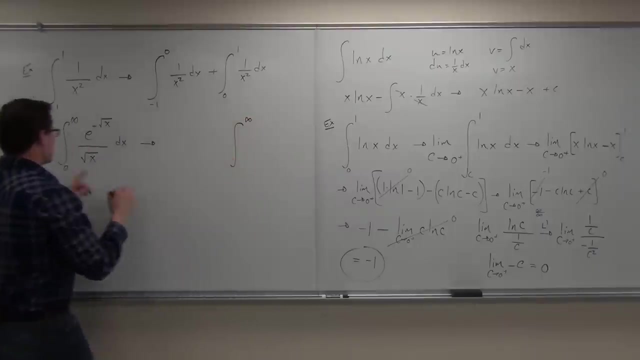 No, but we can do this, Not a problem. But here's how to split it up. If you have an infinite interval, we're going to have to have somewhere where we can start at a finite number and end at an infinity. For here, for our infinite discontinuity, 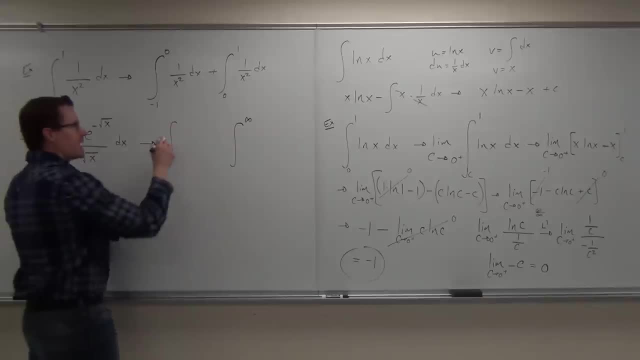 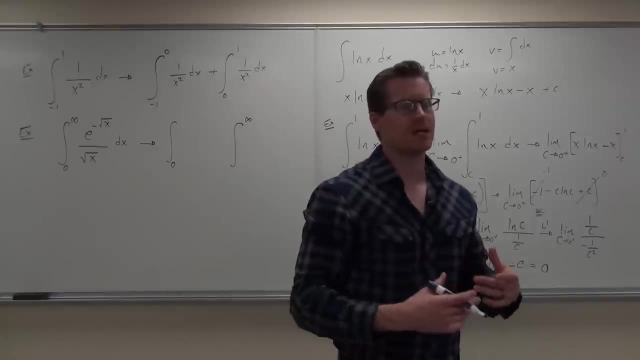 we're going to have to have somewhere where we start at 0 for sure, but we end at a finite number. So what we're going to do here is we're going to split up our integral with some intermediate value that's relatively easy to plug in. 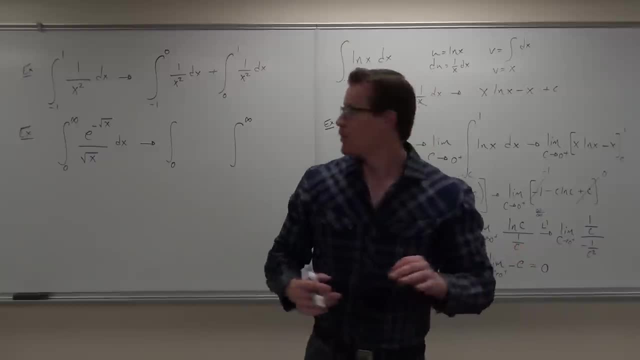 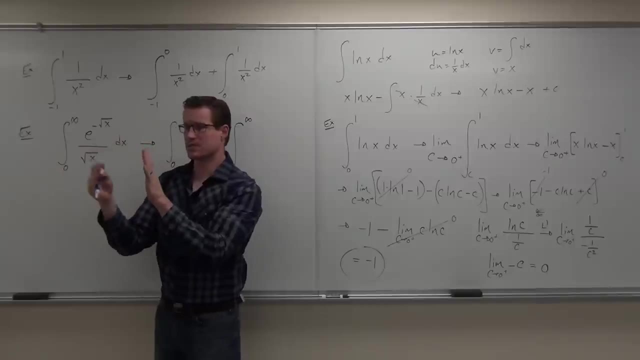 So are you guys with me on the idea? We know that we can separate integrals as long as they're well continuous, or as long as we separate and make a discontinuity with our limits? now We can separate them anywhere we want to. 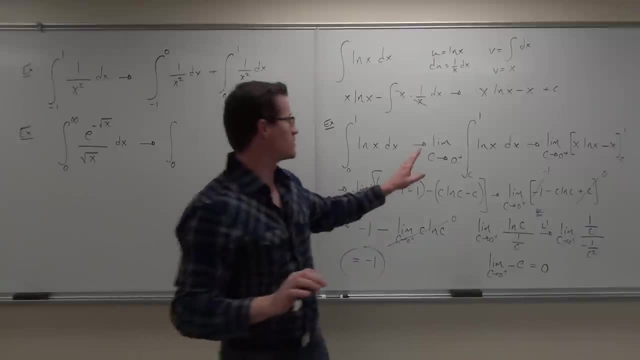 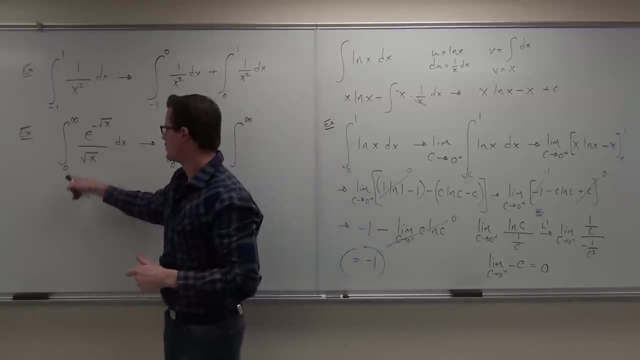 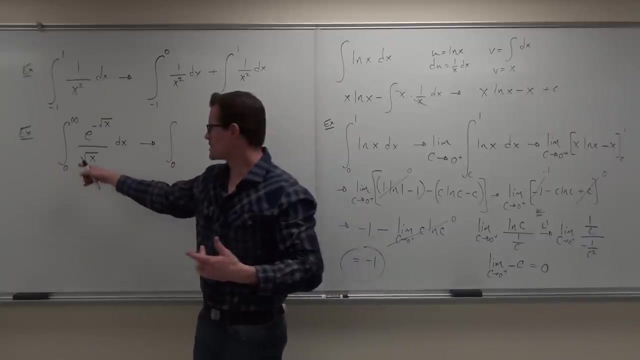 We typically will separate at the discontinuity if one exists between our ending bounds or interval. However, if we have no infinite discontinuities between the bounds of our interval, just pick a random number or pick one that's easy to plug in. What number is easy to plug in between 0 and infinity? 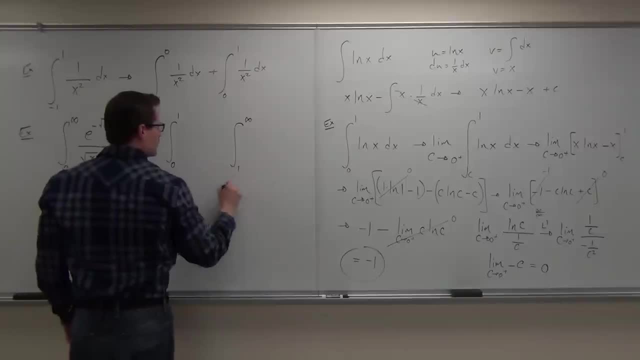 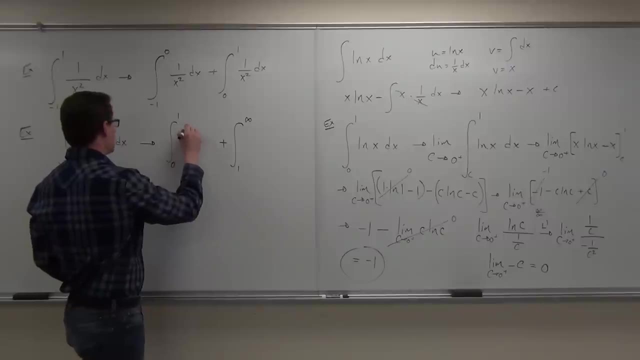 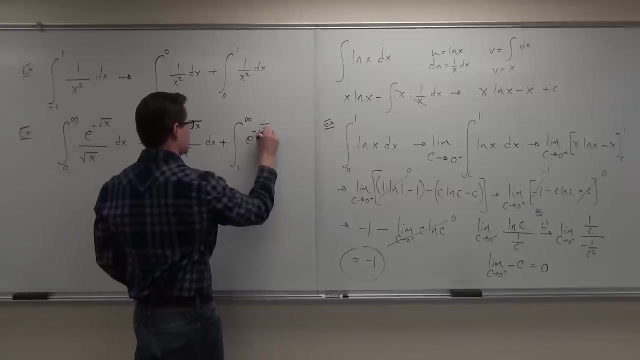 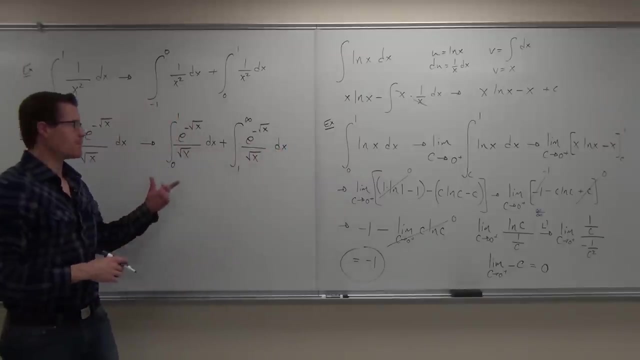 1. Does that make sense? Add them together. Now tell me something. Now that you've broken it up, can you do this integral? This is improper. It's definite interval here. It's just undefined at that point. So we could write a limit as: 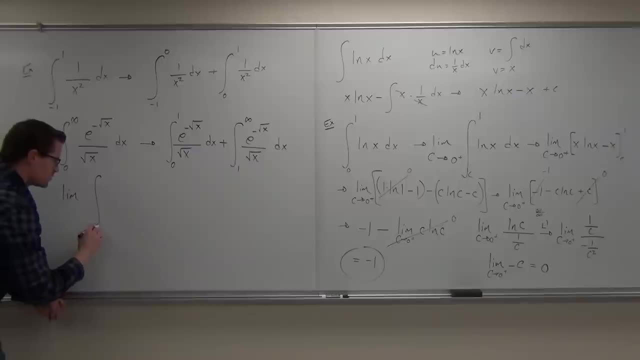 What number is going to change. Look what number is going to change: 0. To a thing, 1.. C, C. Wow, Third time's a charm. Okay, now where's that C going to go From the right? 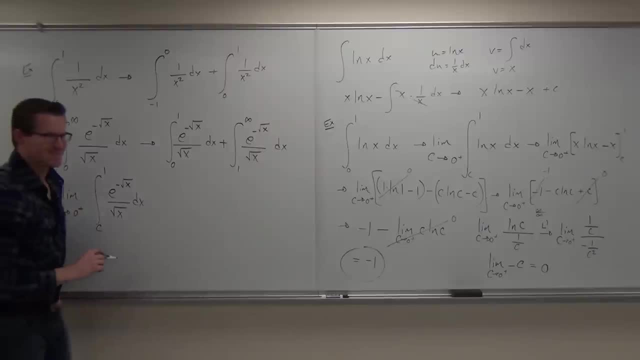 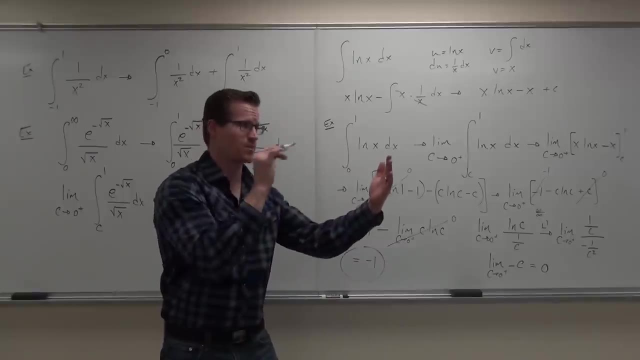 From the right, From the right. Listen, if it's a left-hand bound, you're going to have to get there from the right. If it's a right-hand bound, you're going to have to get there from the left, Because there is no other side of that. 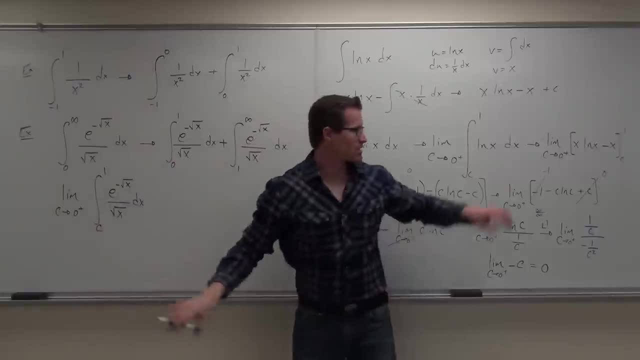 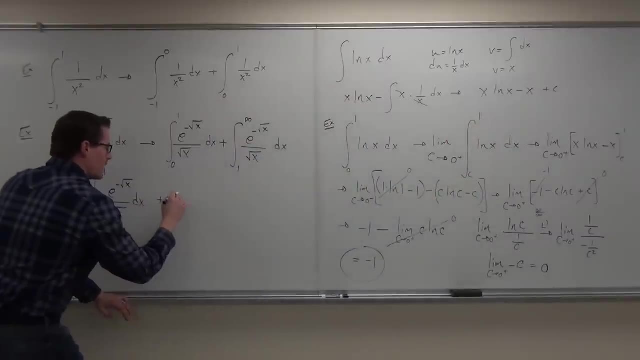 Show of hands if you feel okay with that one. Do you guys see how this idea is the stuff that we literally just covered? It is this. All you've got to do is break this thing up. So now, next one: We're going to have a limit. 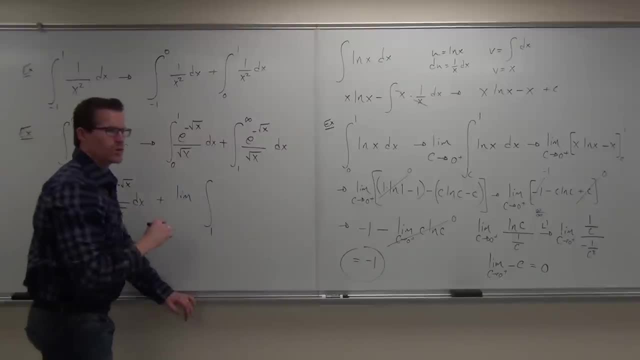 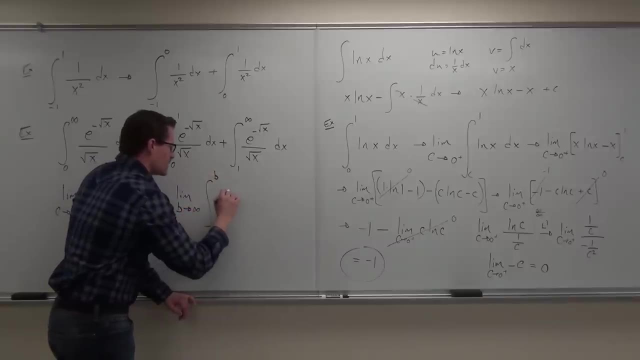 Okay, let's see if you remember this from last time. The 1's not going to change. What's the infinity going to be? E As B approaches E to the negative square root of X over square root of X. Now be smart about this. 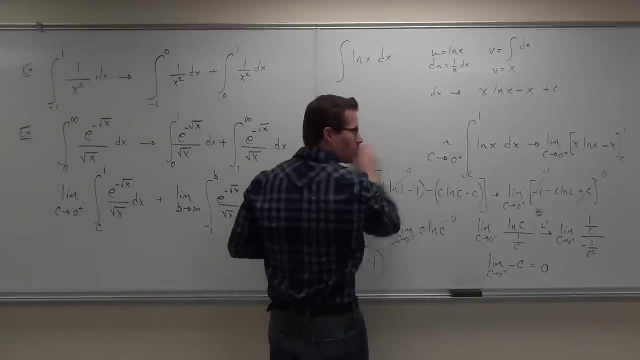 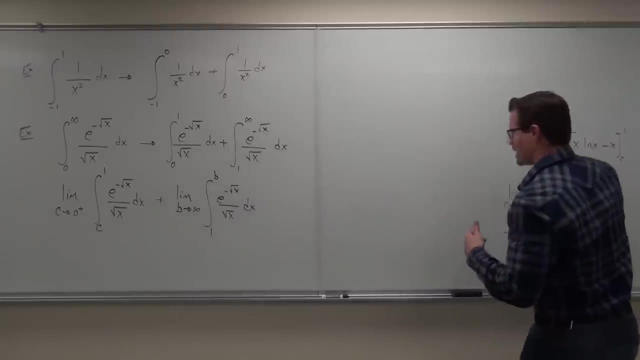 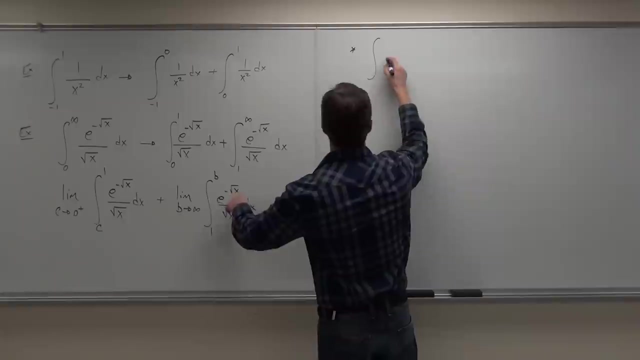 Don't do the same integral twice, two different times, Just do it once and use it for both cases, okay, So for us, I'm going to really rip through this thing very quickly because I have about a couple minutes left And I'm going to assume that you know how to do this. 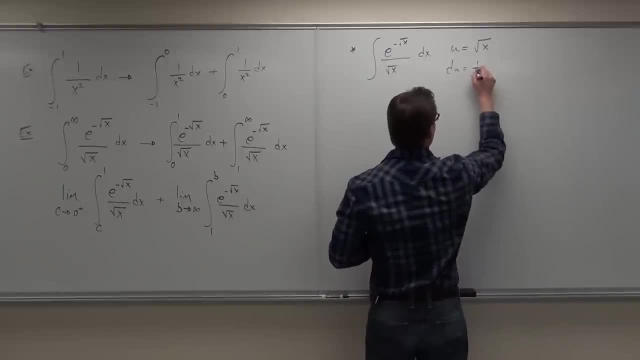 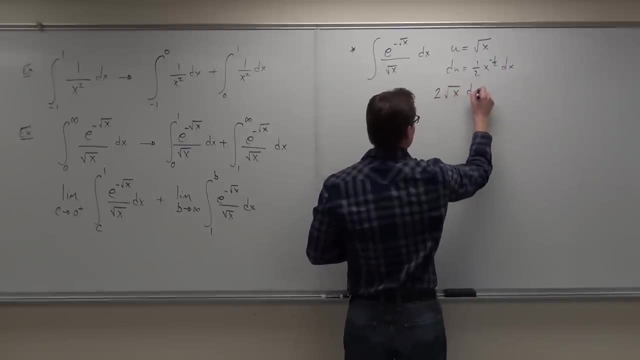 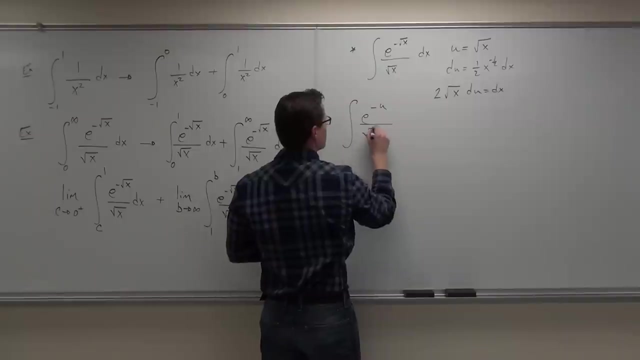 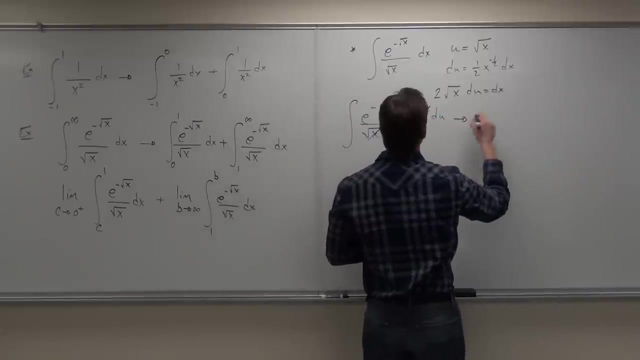 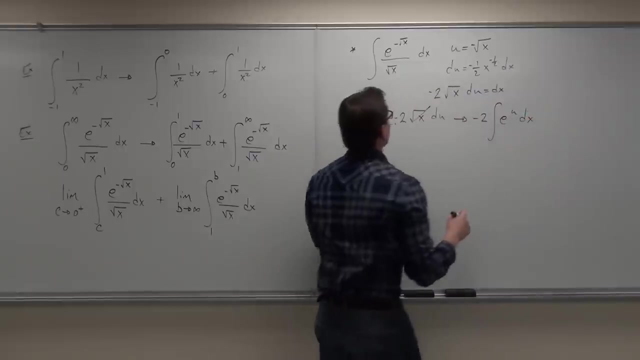 I guess you could have made that negative 2.. Now, let's do that. So U is negative square root of X. You get negative 1 half. X to the negative 1 half. Move over to the negative 2 square root of X DU. 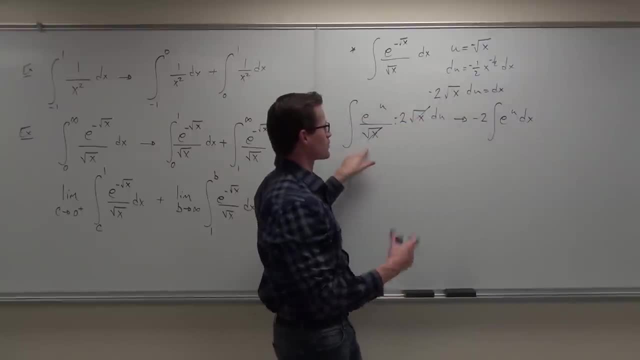 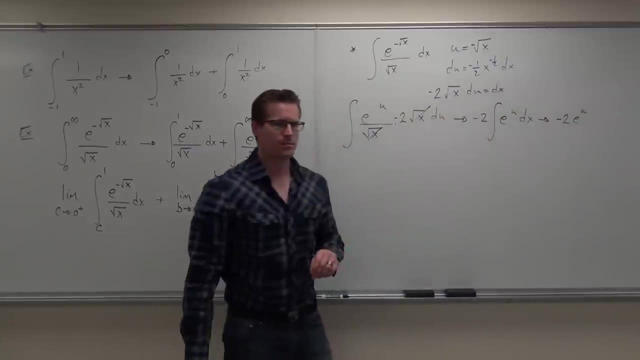 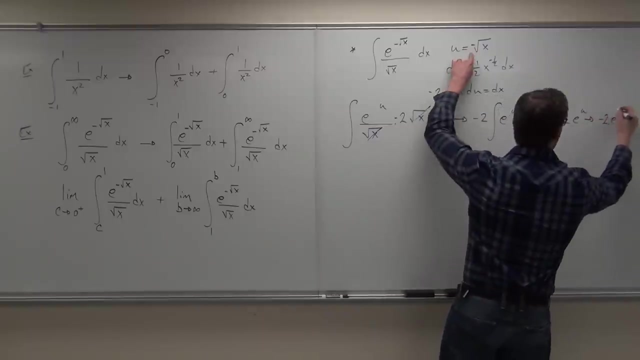 That is our DX. Bam, square root of X's are gone. Pull out our negative 2.. Our integral becomes negative 2, E to the U. So far, so good. Now, of course, before I start evaluating this, I'm going to want to make sure that I have my function in terms of X and not U. 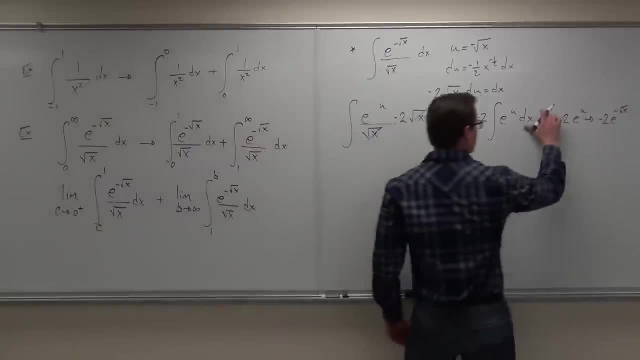 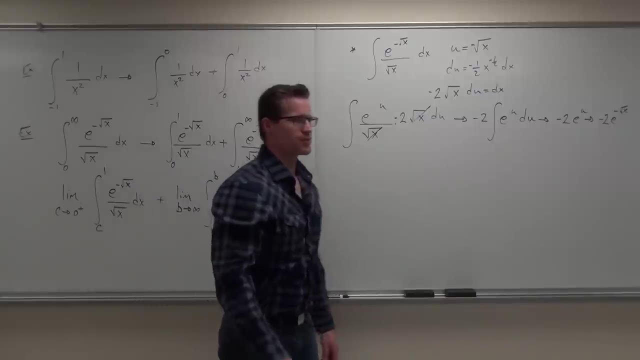 It should be DU, not DX. Oh yeah, thanks, Thank you for that. So negative 2 E to the U, negative 2 E to the negative X Show of hands. if you're okay with that, one Basic use of it, okay. 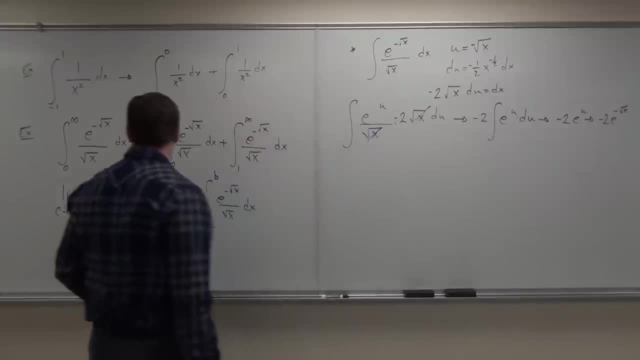 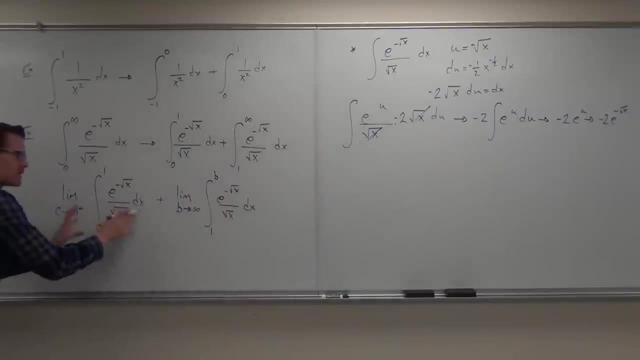 If you need to watch that again, watch it again. Now we've got both of these pieces. So what we end up doing is, once we've done this integral, now take that idea and put it here. So we have from this side. 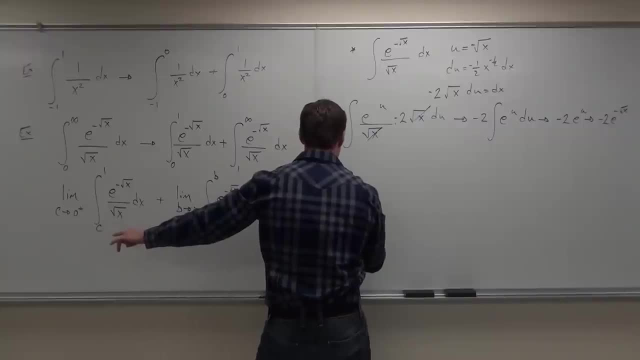 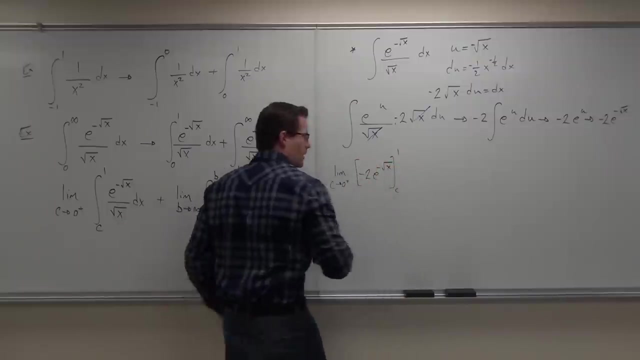 we've got a limit as C approaches 0, from the right. This integral is this negative 2 E to the negative square root of X. It's just that we're evaluating from C to 1.. Okay, I really want to make sure that you guys get this idea. 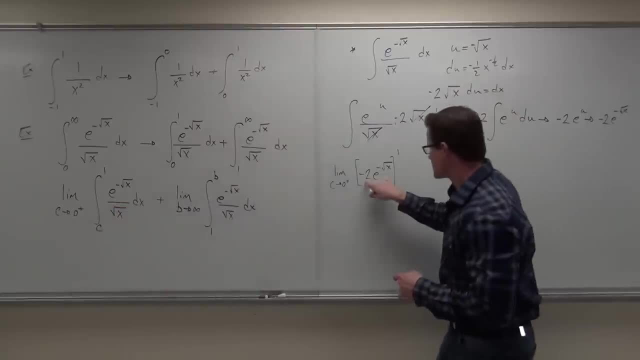 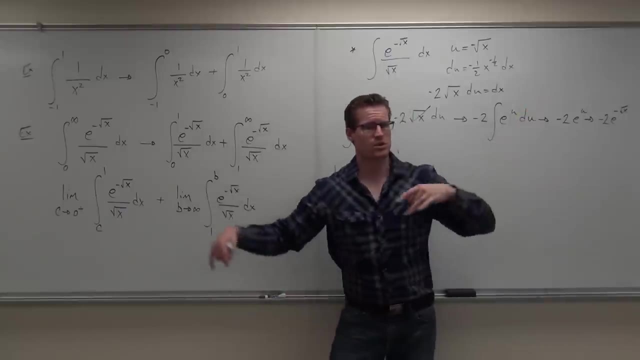 Are you okay that this integral is this piece, and I'm just going from C to 1?, Yes or no? Yeah, Are you sure? Is everybody sure on that one? That's a big deal. So we integrate once and we use it twice, because we're just splitting up the same integral. 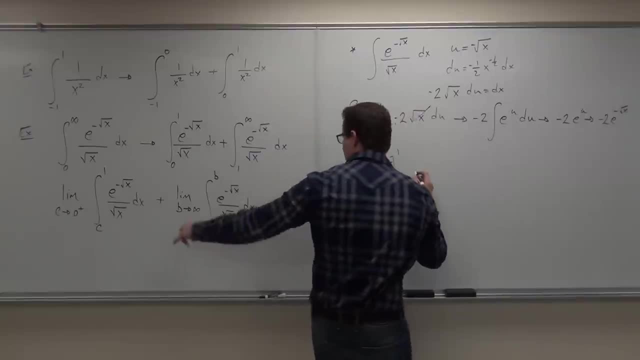 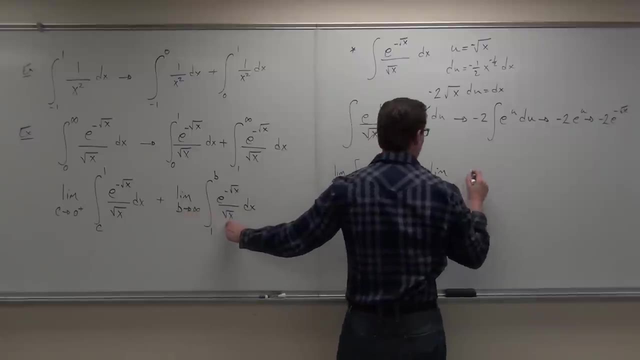 Show of hands if you're okay with it. Okay, fantastic. Now we're going to add on to it a limit, as B goes to infinity. This integral is this piece, Only on this particular integral, I'm going from 1 to B. 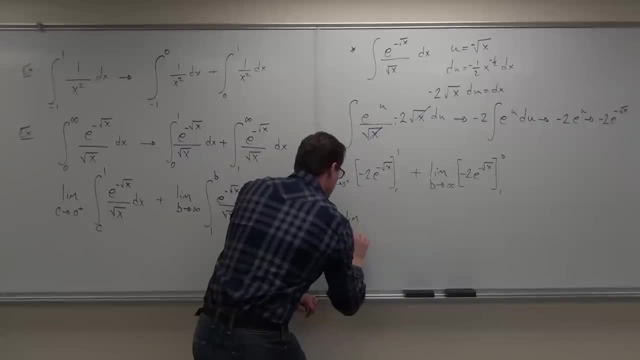 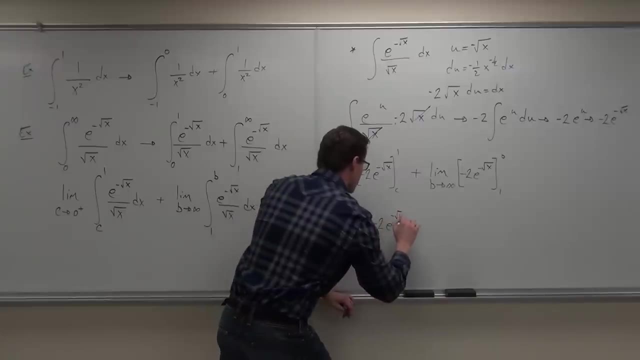 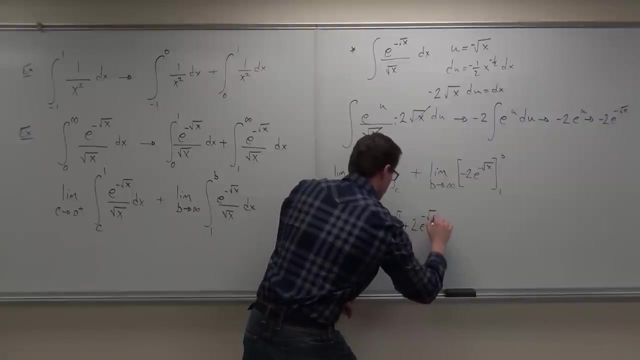 So we evaluate Limit as C goes to 0 from the right, Which one do we plug in first Negative 2 E to the negative square root of 1, minus negative 2 E to the negative square root of C, This minus this. 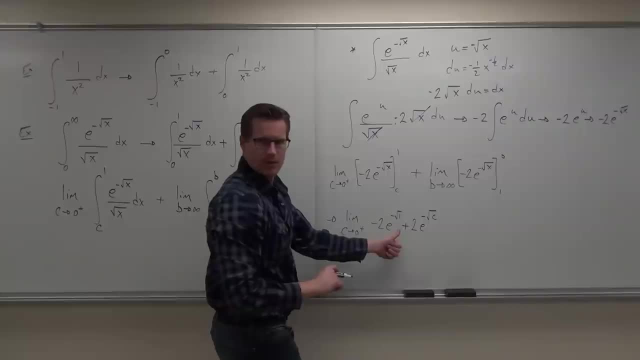 So I'm doing the plus here. Do you guys see where the plus is coming from? I don't want to blow you out of the water, but I got to go quickly here on this one. So this minus a negative, That gives us a plus. 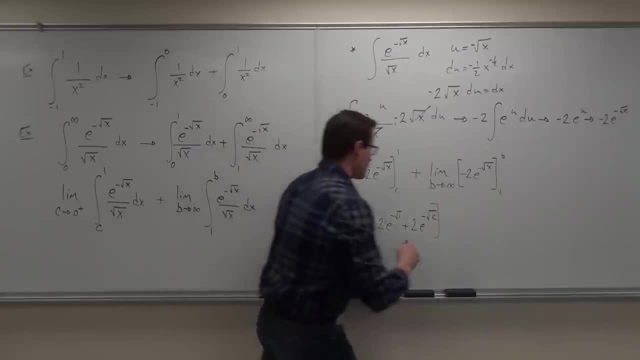 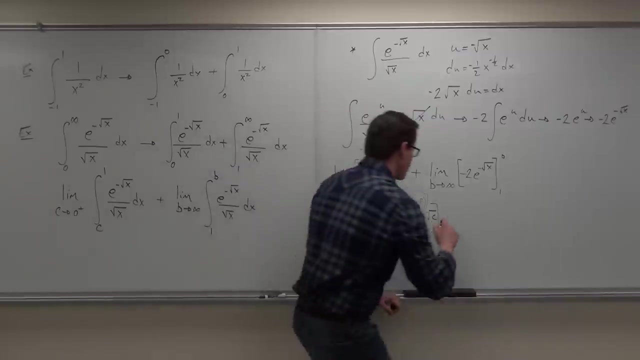 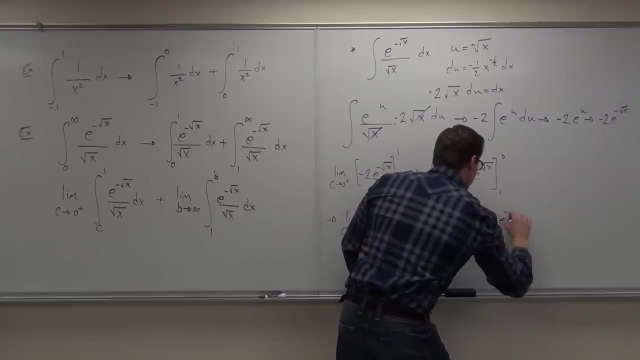 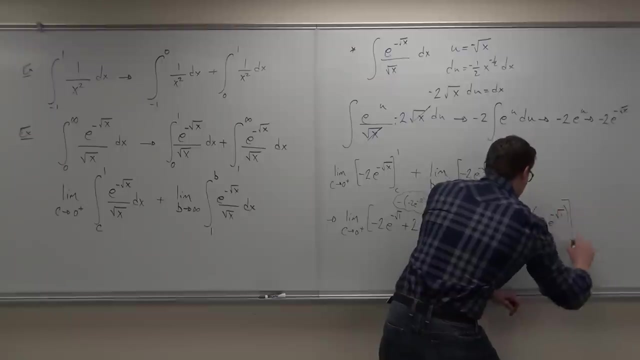 You okay with that. I swear I wouldn't have missed that Little piece Minus and negative. I'll do it over here if that bothers you. Negative 2 E to the negative square root of B, minus negative 2 E to the negative square root of 1.. 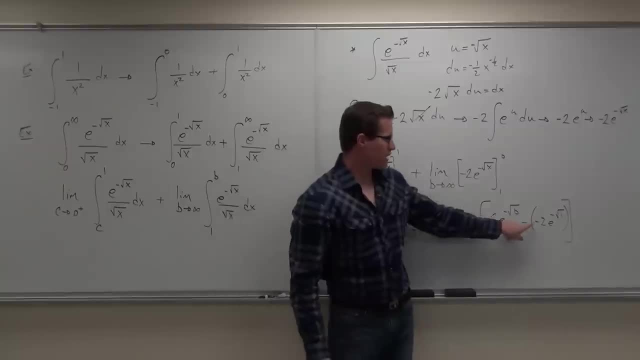 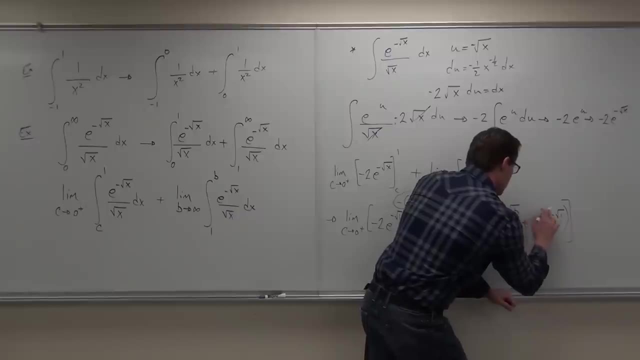 Here's what I'm talking about. This is what we did here. So, when I subtract a negative, what does this become, ladies and gentlemen? A power? Okay, now we're almost done. Tell me what is. what's the square root of 1?? 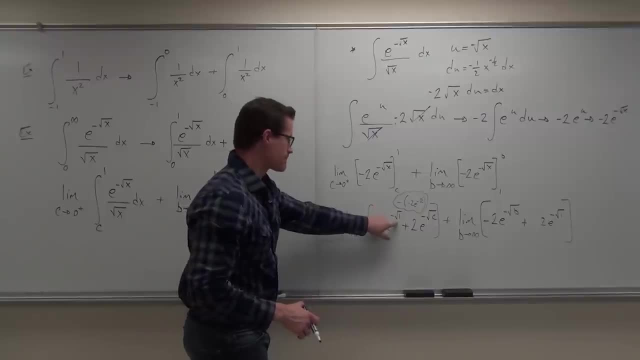 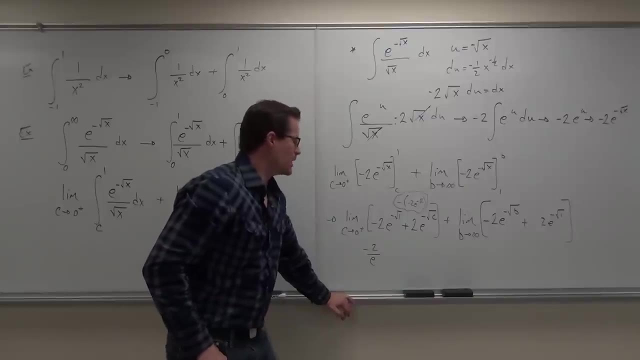 1. Negative 1.. So this is negative 2 over E. Does that make sense to you? Negative 2 over E. Now what's happening to the C? It's going to 0.. It's going to 0.. 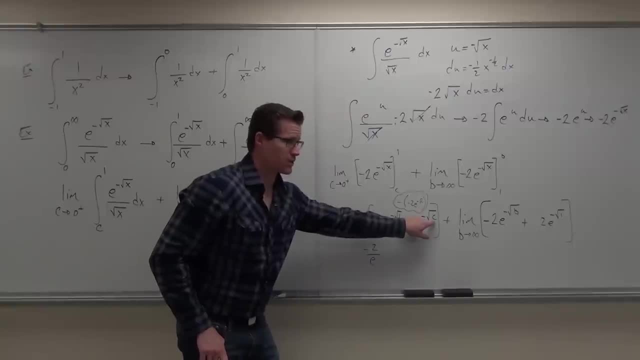 What's the square root of 0?? So look it, this is getting really close to 0.. Are you with me? Square root of 0 is Negative 0.. Negative 0 is 0.. E to the 0 is. 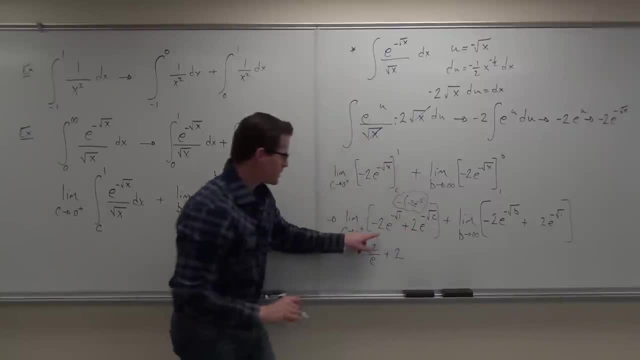 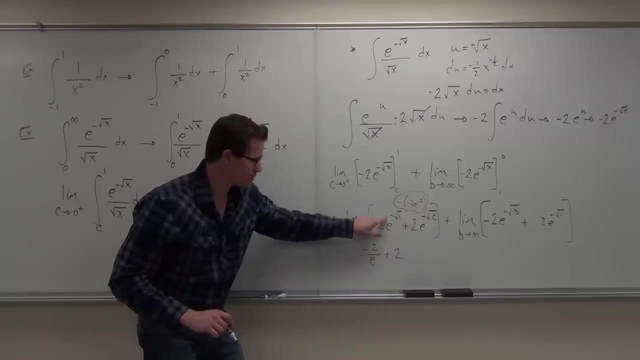 1. So this goes, This goes to well. E to the negative: 1. E to the negative: 1 is over E. So negative 2 over E. This is 0.. E to the 0 is 1.. 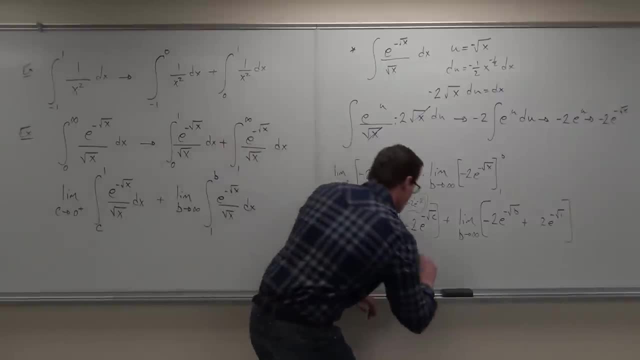 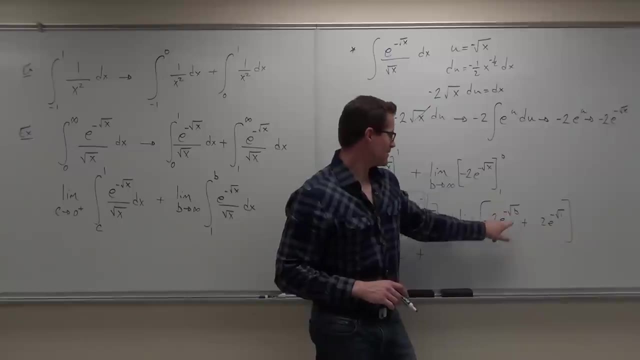 This gives us 2. Are you guys with me on that one? Yes, Plus, Let's go to infinity. What's the square root of infinity? I'm going to go from negative to infinity. What's my problem? This is right, right. 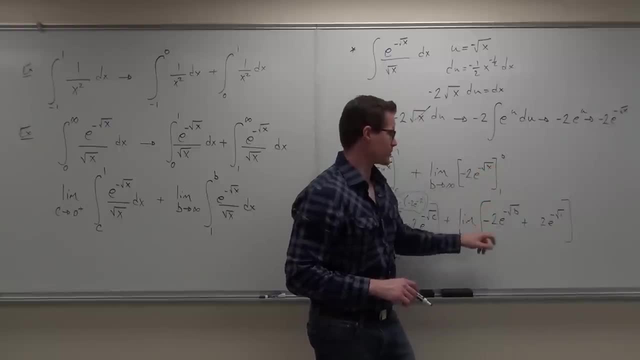 Yeah, B comes first. Plug in the B and then plug in the 1.. B comes first. What's the square root of infinity? Infinity, Still infinity. This is negative. oh think careful. Do you guys see what I'm talking about? negative infinity. 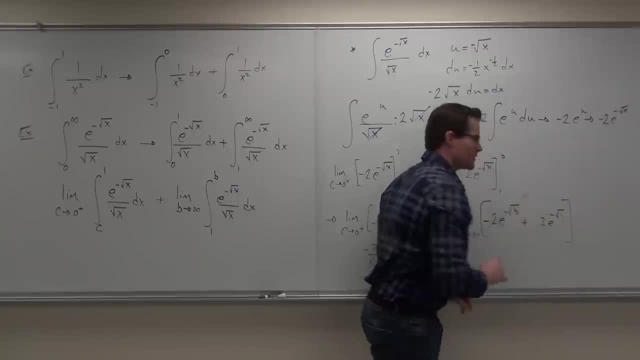 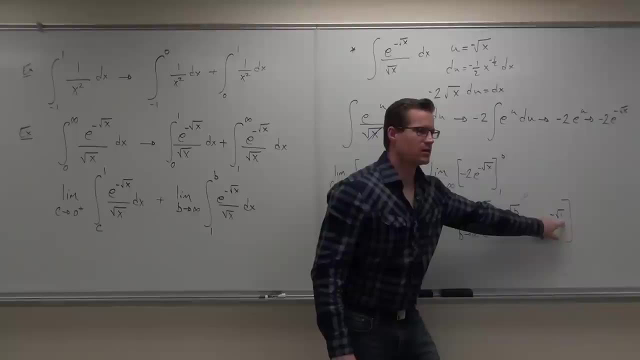 E to the negative infinity is 0.. Thanks for the Okay. now how about this one Square root of 1.. 1. What's E to the negative? 1?? 2 over E, 2 over E. 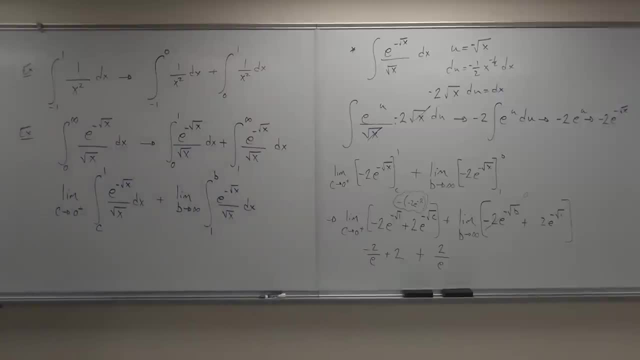 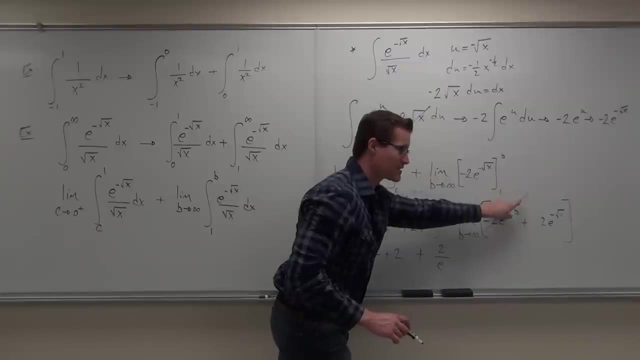 What happens? What's our area 2.. So this was this. This is 2.. This is 0, because E to the negative infinity is 0.. 0 times E to the negative infinity is 0.. This gives us this again. 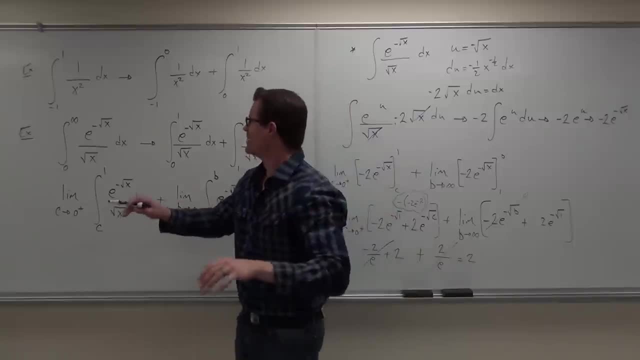 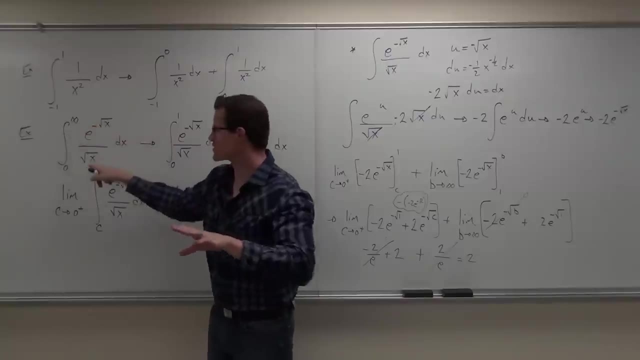 Bam, bam, we get. oh my goodness, This is crazy, okay, crazy. So we do all this work From 0,, where it's not even defined, to infinity, where we're going forever of this function. 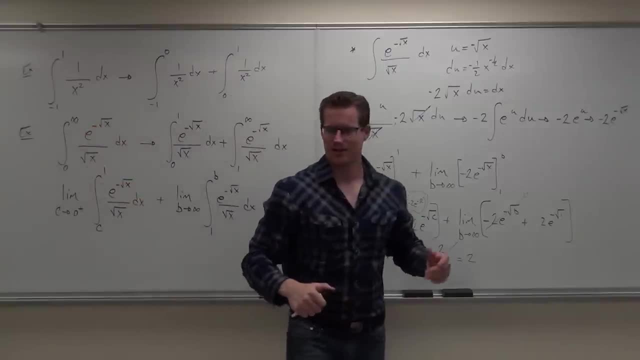 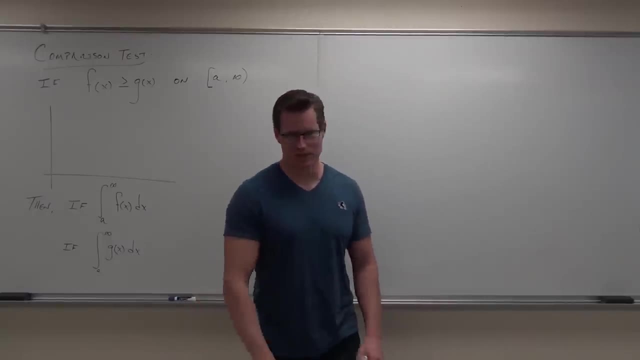 and because of our limit idea we figure out this area under that curve is 2. Bam, Our last little bit of session. 7.6 of this section is dealing with something that's a little bit of a kind of a nice application that we can use improper integrals. 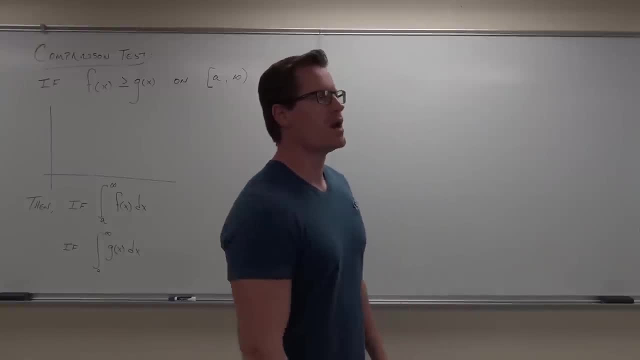 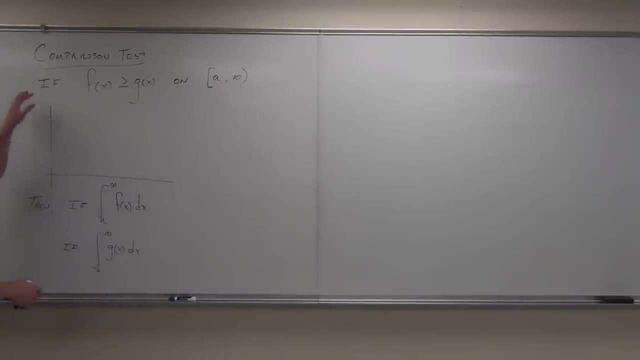 use to our advantage with improper integrals. Here's the idea. Let's suppose that we know something about two functions. Specifically, we know that if we compare two functions, one is always greater than or equal to another graph on this interval, or one is always less than or equal to another graph or function on this interval. 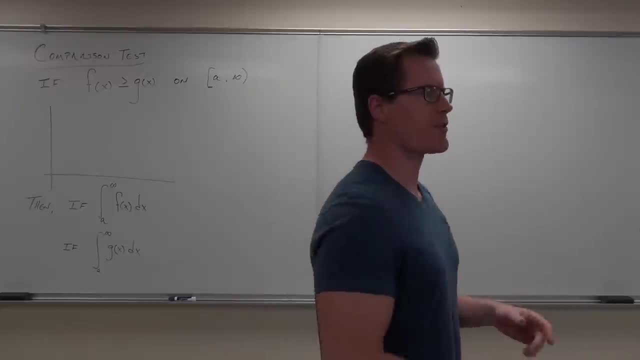 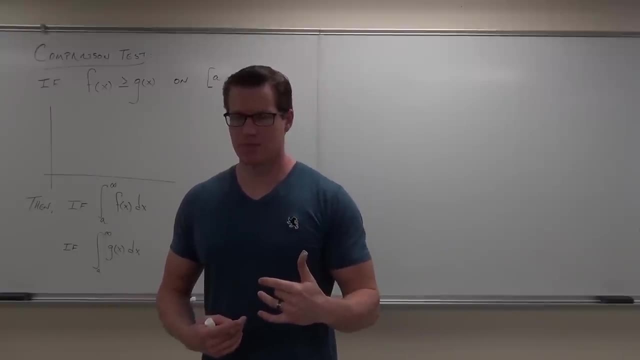 If we know that, then sometimes we can say something about the convergence or divergence of these integrals without even doing them. Did you hear that? Without even doing them? And the reason why that might be nice is because there's some integrals that we can't do. 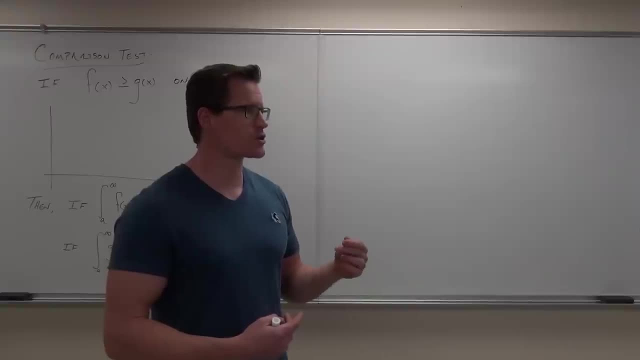 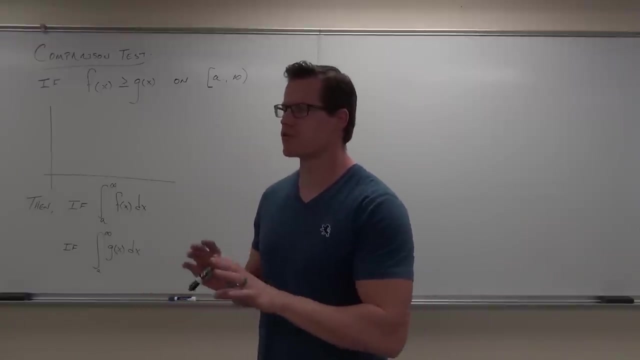 There are some non-integrable functions, so if we compare them to some that are possible, we can find out some nice things about it. Does that make sense to you? Let me give you a picture of what I'm talking about, okay. 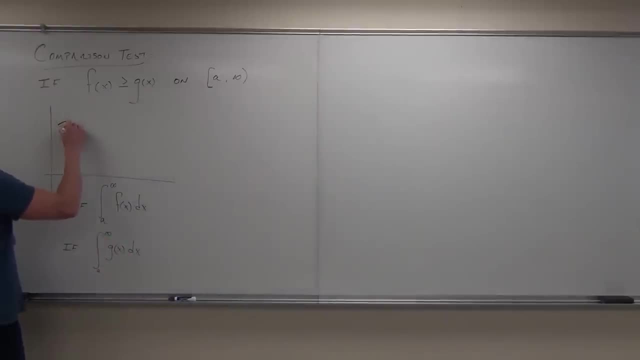 So let's say that I've got some function f of x, And I don't care what this function looks like, it's just some function- And it goes forever. And I've got some function g of x And it goes forever. 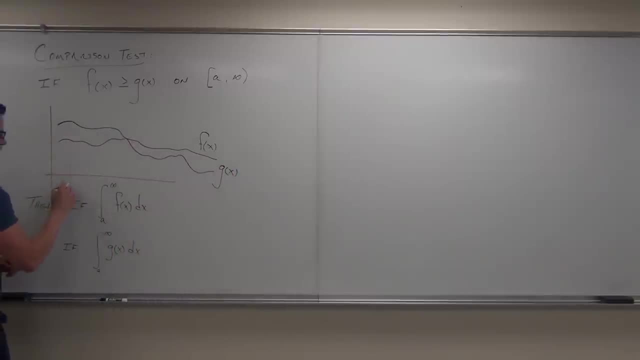 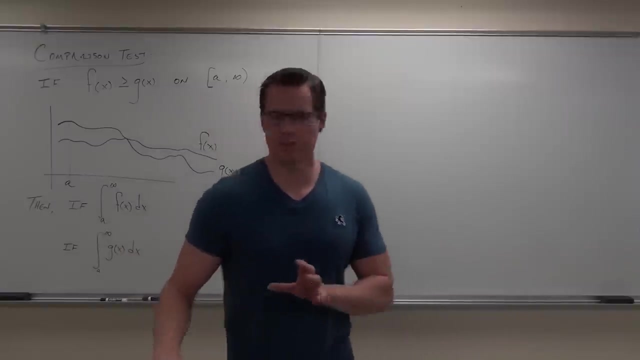 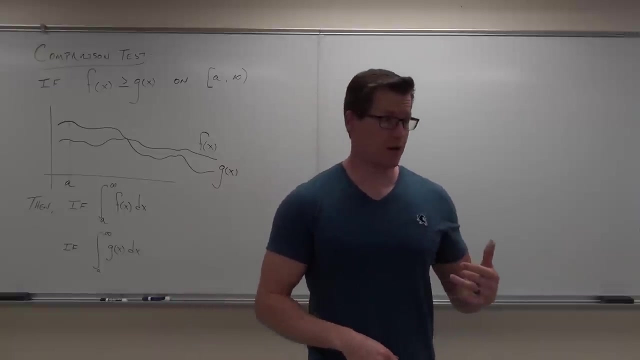 And it goes forever. Now here's the thought process I'm going to try. It's a very simple, and what I have right here is very simple. It's going to be like one little statement, one little statement, But I want to make sure that you guys understand the concept. 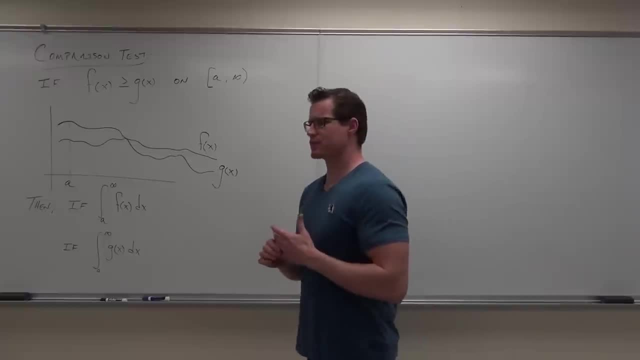 That's what this class is about, right? It's understanding the concepts here, So think about this for a second. Firstly, do you see that f of x is always greater than g of x for any number that I give you from a? 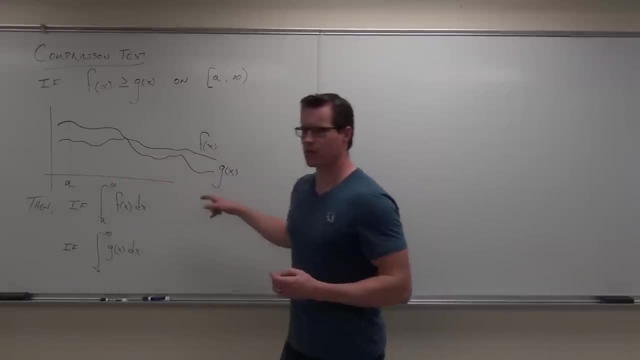 and let's assume this goes like this forever. okay, From a to forever. Are you guys with me? Always greater than or possibly equal to it? Let's look at it. The black line is f of x. the purple line is g of x. 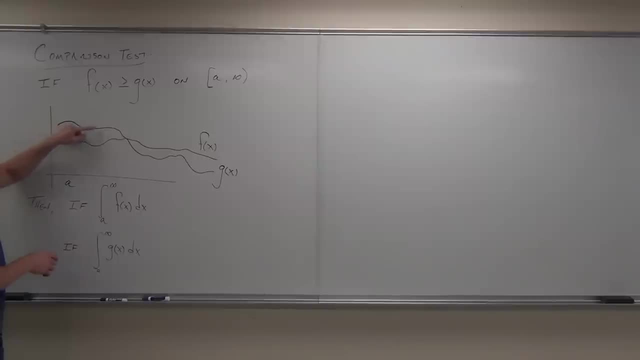 Is the black line above the purple line? Yes, Is the black line above the purple line? Yes, How about? right here? Oh, it's equal. right there, Does that matter? No, It can be equal to it, That's fine. 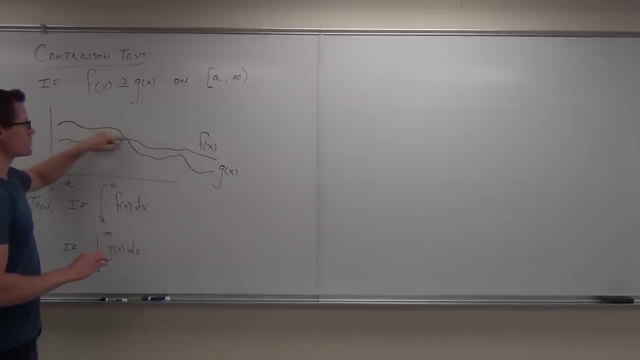 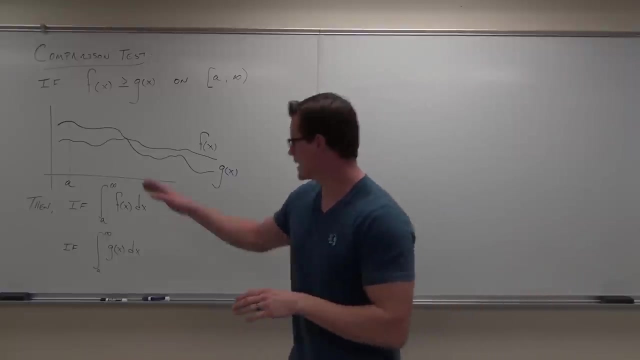 As long as it doesn't jump above it, that would be a problem, But there's always equal to it or less than that. So would you agree that f of x is always greater than or equal to g of x for any number from a to infinity? 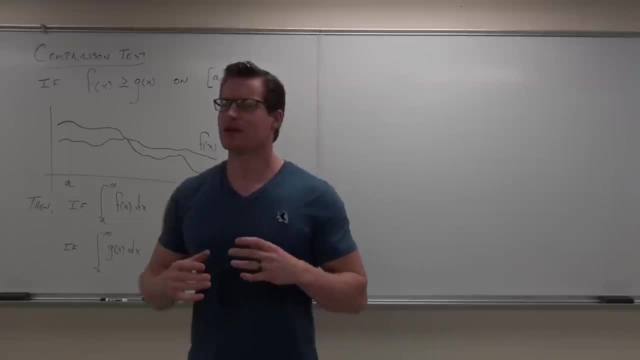 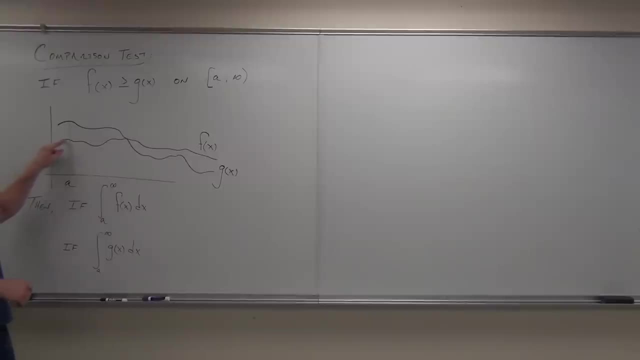 Show of hands. if you understand the concept. Okay, now here's the plan. Think about what would happen for these scenarios. Let's say that we take an integral of g of x. Let's start with f of x. Let's say we take an integral of g of x. 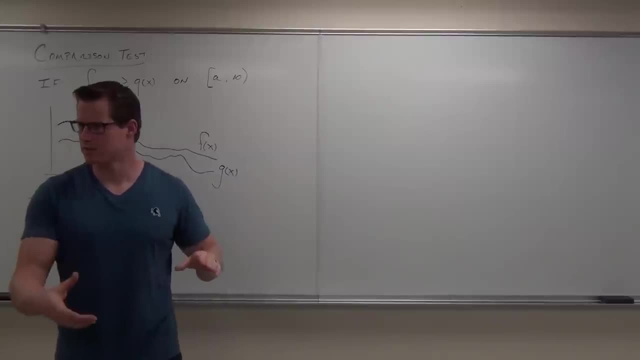 From a to infinity. Remember the improper integrals that we've been doing. Watch the video from the beginning if you don't remember that, If we go on this indefinite interval from a to positive infinity, we go. okay, let's take the integral of f of x. 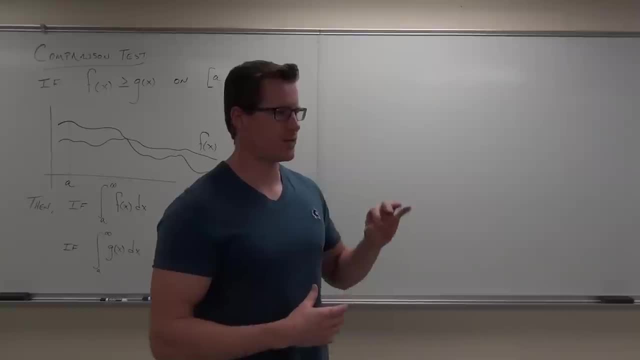 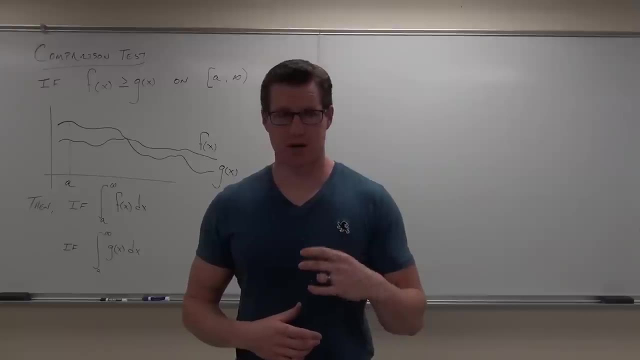 Let's say that we can find it. So the integral of f, of x, from a to infinity, is actually convergent. Remember convergent, Remember the word convergent. It means the area exists, the limit exists, So the area exists. So we do this and we say: oh, you know what? 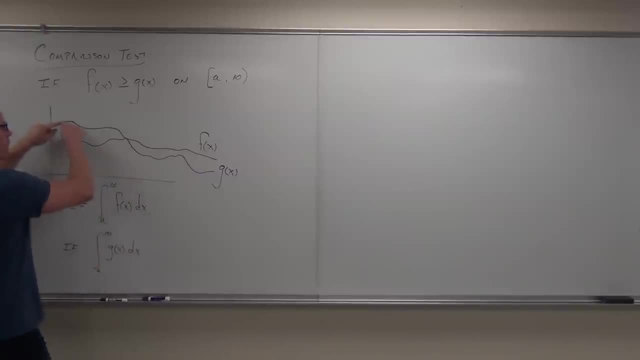 I can find. Here's the key thing, so focus. right now I can find the area of f of x from a to infinity. You get that. Therefore, the integral of f of x from a to infinity would be called convergent. 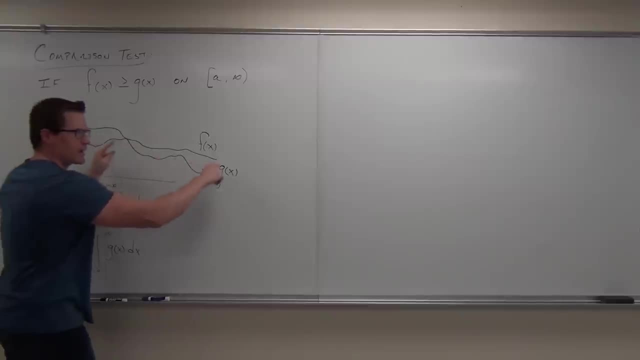 Now here's a thought. If the integral of the black line is convergent, what would that tell you about the integral of the purple line, of g, of x? Convergent, It has to be convergent. If the big one converges, this one's bounded. 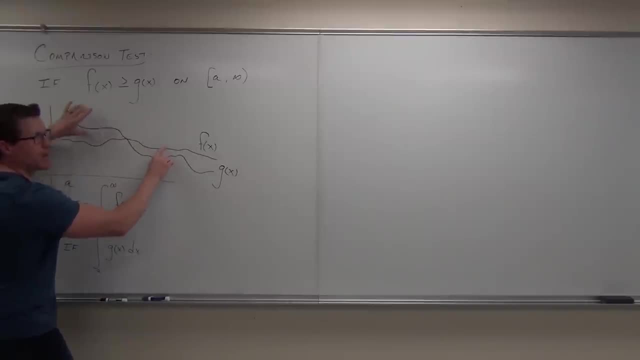 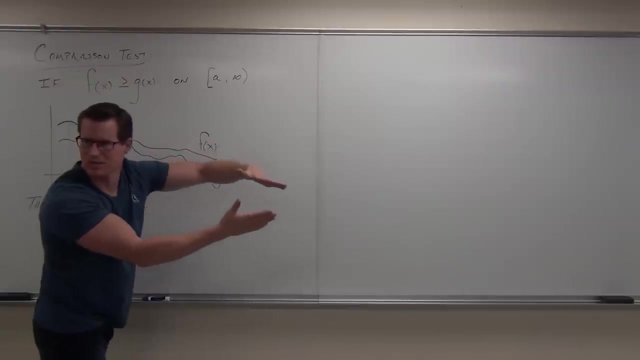 It's bounded by this, and that's what this says. It says that f of x is the upper bound for g of x. It's bounded so if this converges, this one has to. It's like it's squeezing it, almost like it's squeezing it down there. 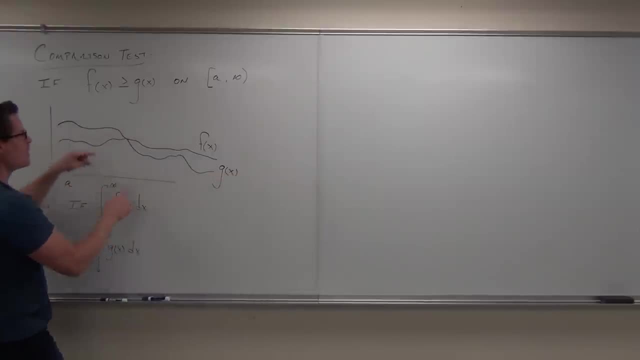 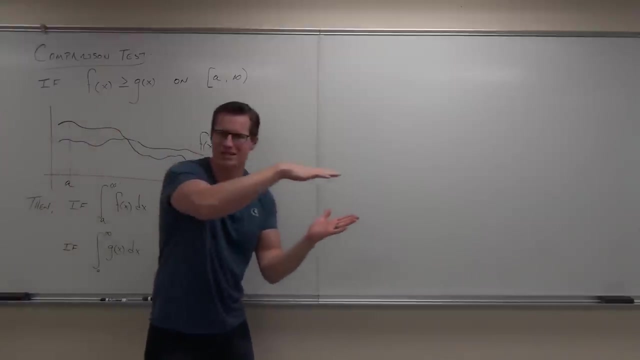 Does that make sense to you? So it's bound by the x-axis and by f of x. Well, this is always above this. If this one converges, a smaller function would also have to. It's like it's getting squeezed down even more. 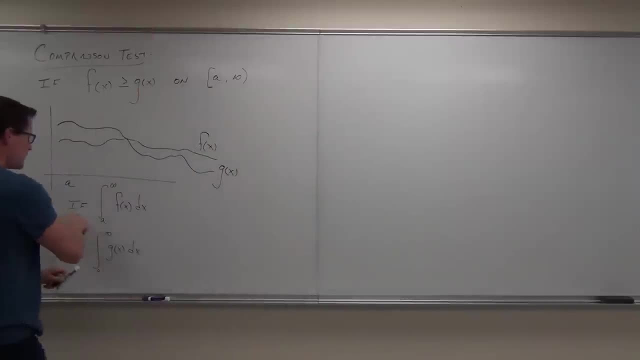 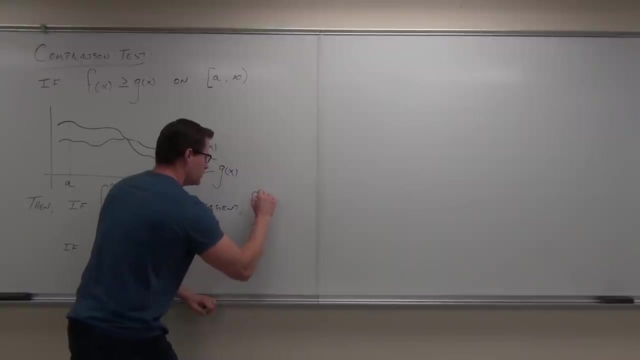 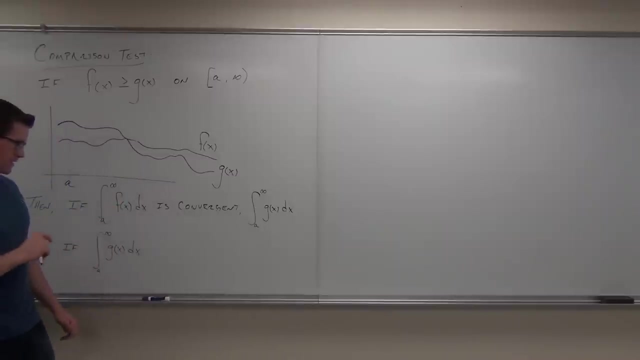 Show me if you understand that one. So that's what we're going to say here. If this integral is convergent, then so is this one. If integral from a to infinity of f of x dx is convergent, then the integral from a to infinity of g of x dx is also convergent. 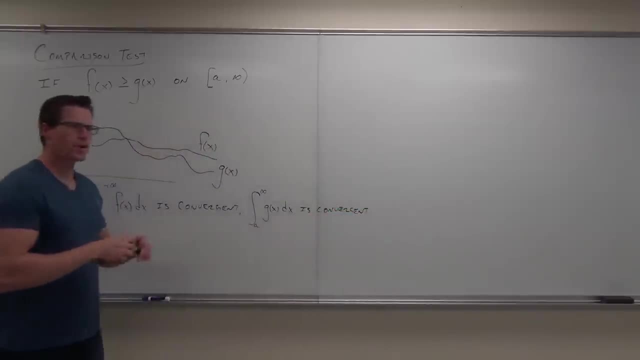 I really do want to make sure that makes sense to you. Do you understand that concept? So if the f of x converges, that area exists, then g of x has to. It's smaller than that Question. So g of x just can't go down forever, or does it have to stay above some point? 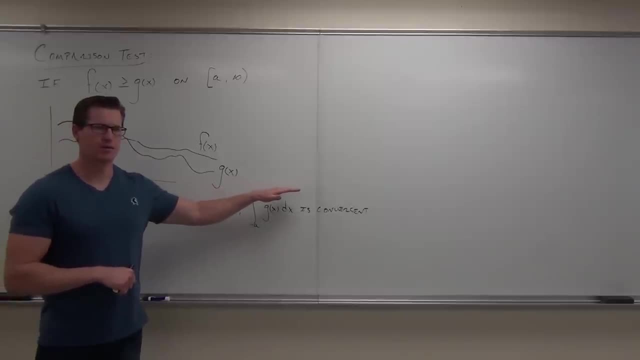 Yeah, we're going to assume that it's bounded by this. But even if it isn't, even if it's not x-axis, if this went down below it, as long as f of x is on top of it, you can still do it. 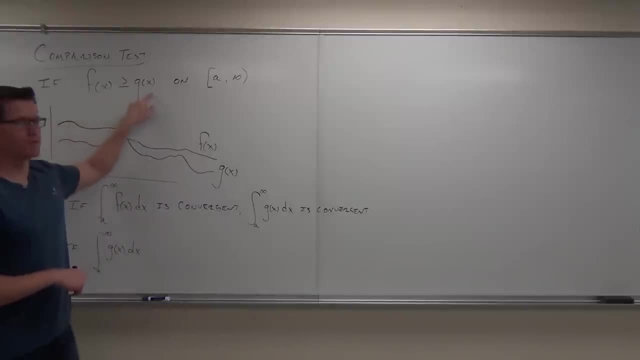 Does that make sense? This is the only condition we have to have. This has to be above that. What can't happen, it can touch, That's fine. The difference in areas between there for the interval where they touch is zero. If it goes above that, that's a problem. 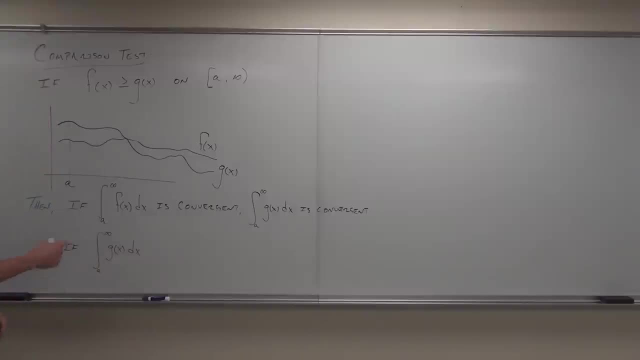 Does that make sense to you? Okay, so now next one. Think about it the backwards way. Let's say we know something about g of x. Let's say that we calculate the area of g of x and it's divergent. 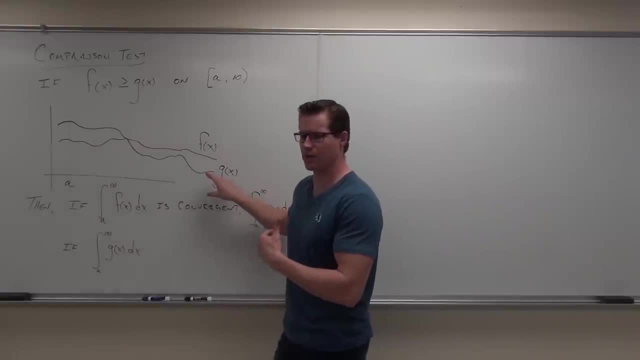 So that means that we go: okay, the area under here, oh, it keeps growing without bound, or we can't find it. What would that tell you about the area of f of x or under f of x? We don't know. 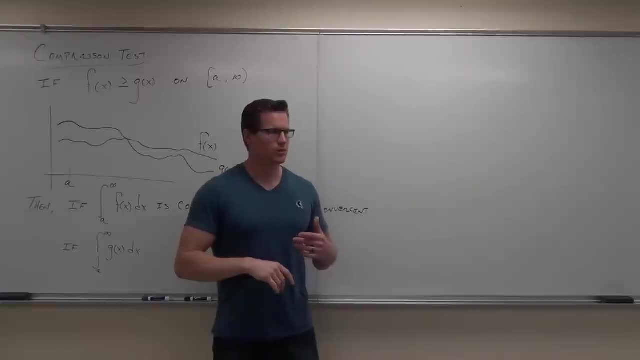 What means? We don't know. Is it possible for the integral of g of x to diverge and the integral of f of x to converge? No, No, If this one grows without bound. remember we're saying this is bigger than that. 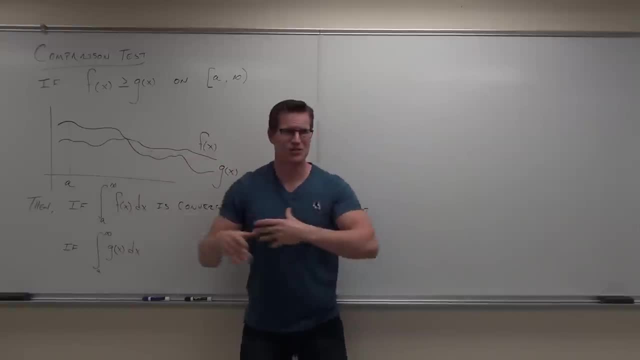 Does that make sense? If this one grows without bound and f of x is always bigger than that, how can f of x converge? if g of x grows without bound, It's not convergent. So if g of x is divergent and we know f of x is bigger than that, 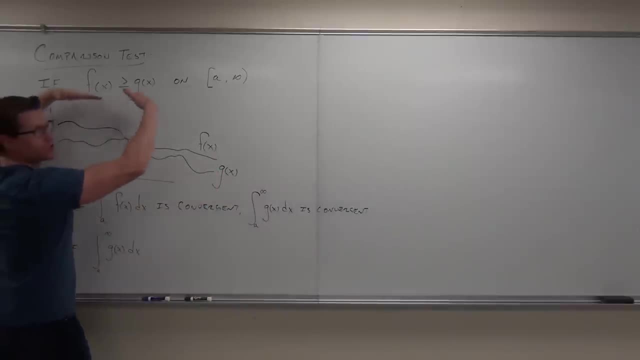 so if g of x goes mm-mm, can't do it. f of x is larger than that. can't f of x also converge? No, So if g of x diverges and f of x is bigger than g of x, then integral of f of x also diverges. 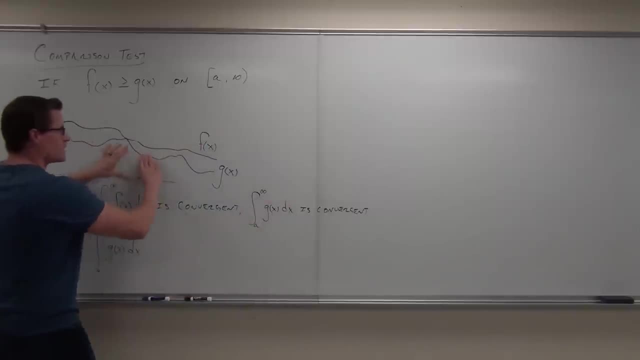 I used f of x instead of integral of f of x, but hopefully you get what I'm saying. If the area of g of x diverges, the area under f of x is bigger than that. It must also diverge. So if the integral from a to infinity of g of x, dx is divergent. 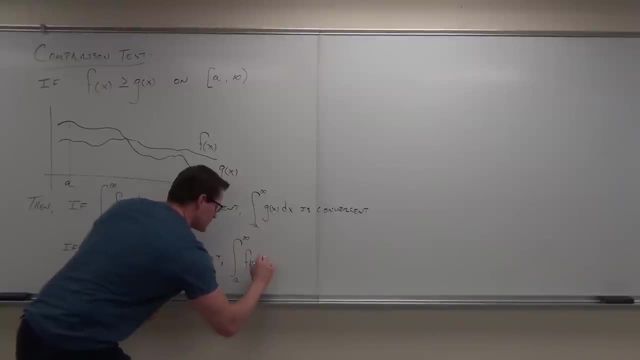 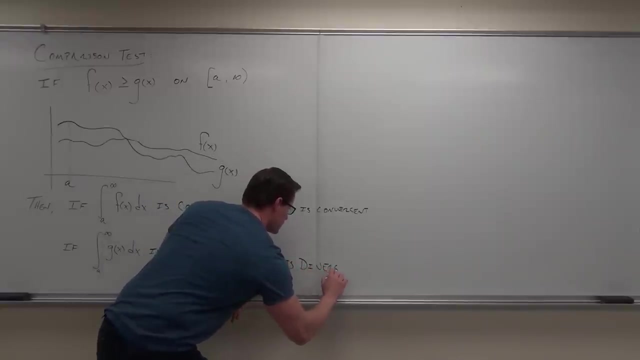 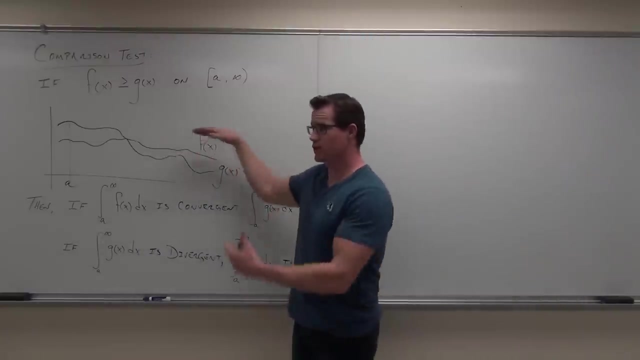 then the integral from a to infinity of f, of x, dx is also divergent. Quick show of hands if you feel okay with that. Basically it says, hey, if the big one goes somewhere to a specific number, g of x also has to do that. 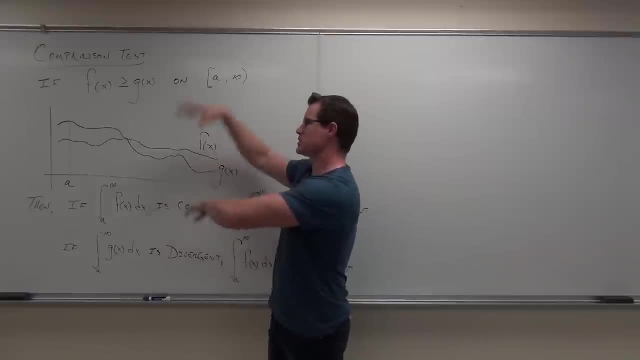 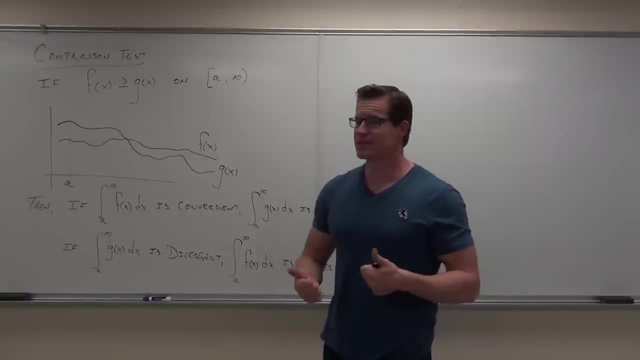 It's kind of squeezed between them, it's bounded. If g of x goes to infinity, then f of x also goes to infinity. That's the idea here. Sure, you're okay with it? Okay, would you like to see an example? 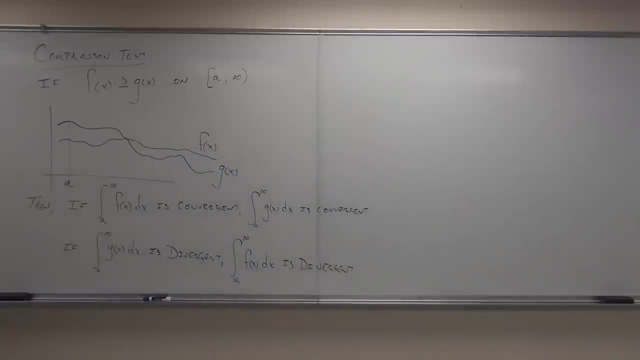 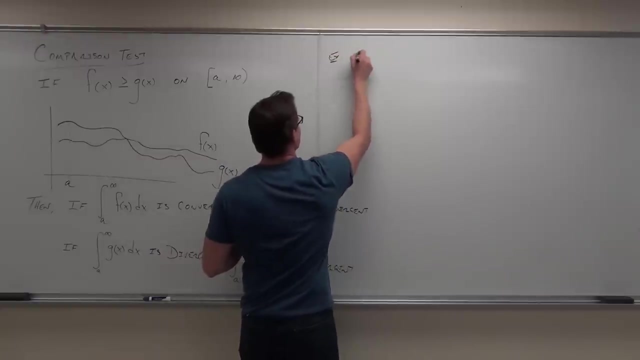 We'll give you one example here, because it's honestly just this idea, But here's why we would use this. So let's say that I give you an integral from 1 to infinity, 1 over x plus sine squared x, dx. 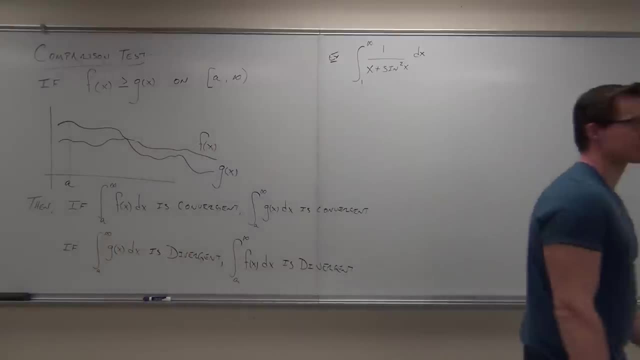 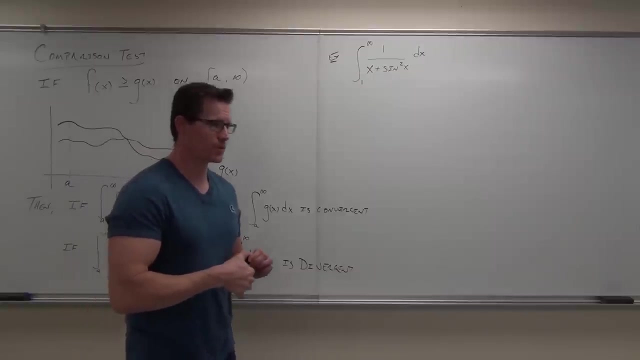 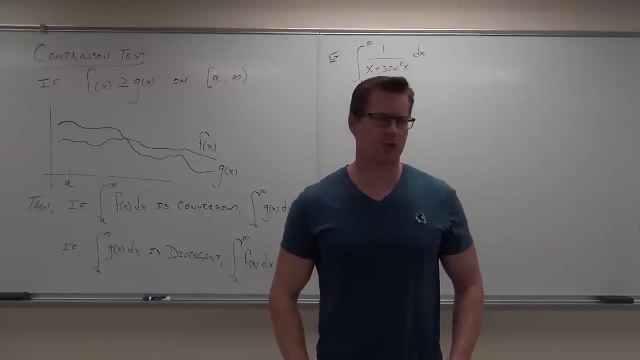 And again, here's why you might want to do this: Integral from 1 to infinity of 1 over x, plus sine squared x, dx. Is there anything that you know that will take care of that integral for you? It's not a sub, for sure, because there's no cosine anywhere to be found. 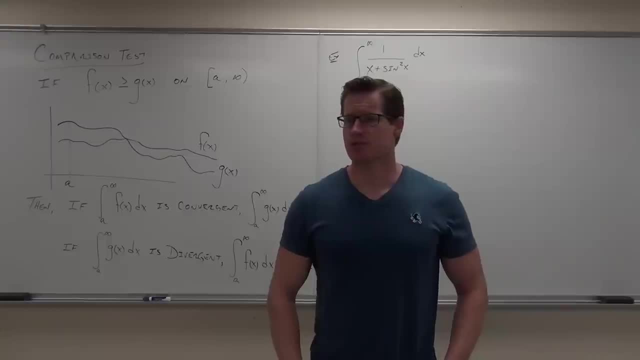 It's not a sub. It's not a by parts, because you have a plus there. It's not a separate y product. It is not partial fractions, because those are not polynomials. It's not a trig sub. You can't complete the square with that. 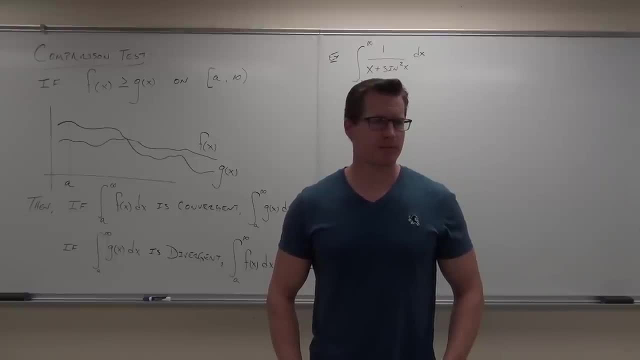 And there's an x, not an x squared. No, No, There's nothing you know how to do for this integral, Some things you can't directly do, Some integrals you can't do. So I know that's a shock to you. 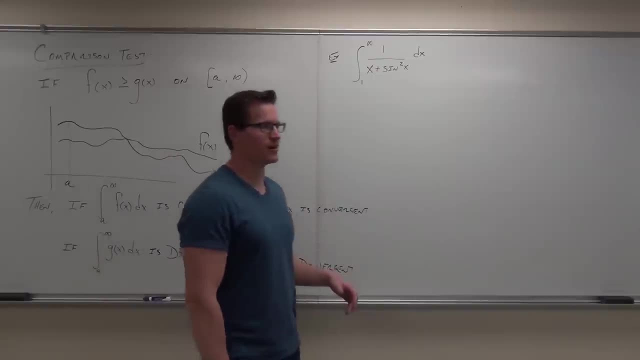 Wait a minute, This is math, Man. sorry, Right here there's nothing that we know how to do for this integral, Maybe somewhere else, numerically or approximations for sure, okay, There's other things that we can do. 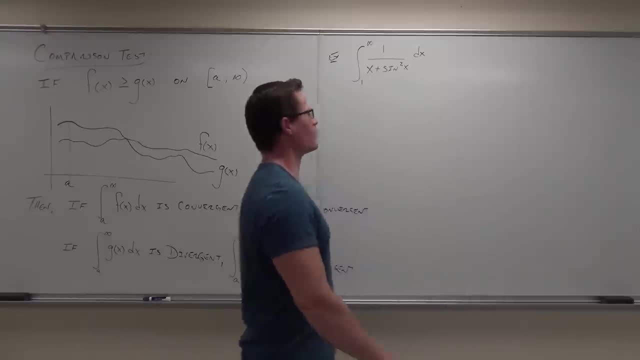 But here? no, We can't do anything with this in our class right now. So what in the world are we going to do? Well, the most we can say about this is whether it is convergent or whether it is divergent. 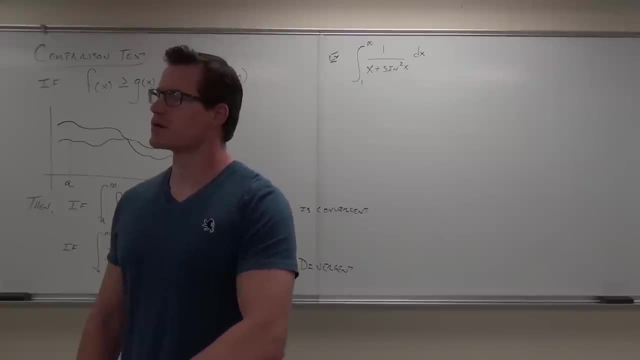 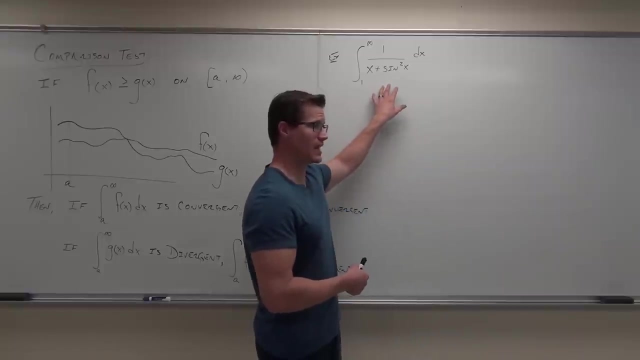 That's something we could probably do, So we're going to make a comparison to another function that we do know how to do something with. Now, we might not be able to find the actual area of this, but we can tell whether it actually goes to a number or whether it doesn't. 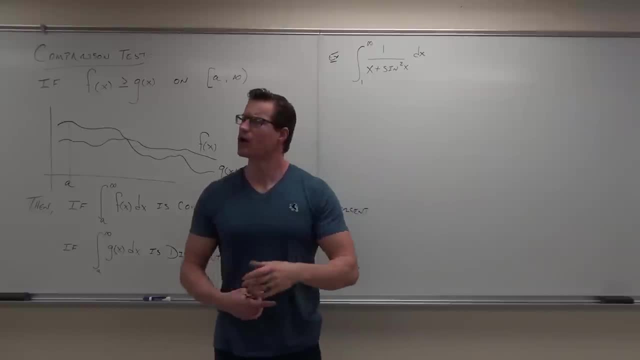 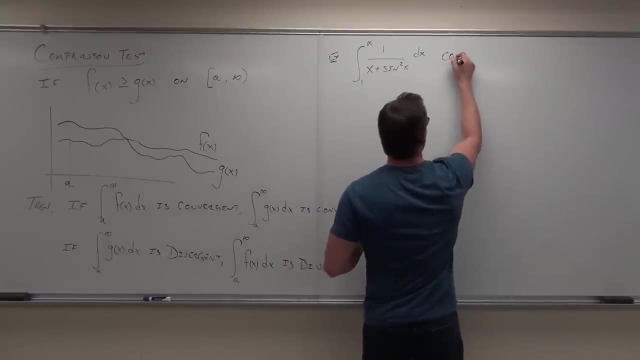 Does that make sense to you, Whether we should spend time trying to find it or whether it's a waste of time. So here's what we're going to do. We're going to compare this to another function, Something that is going to be easy to do. 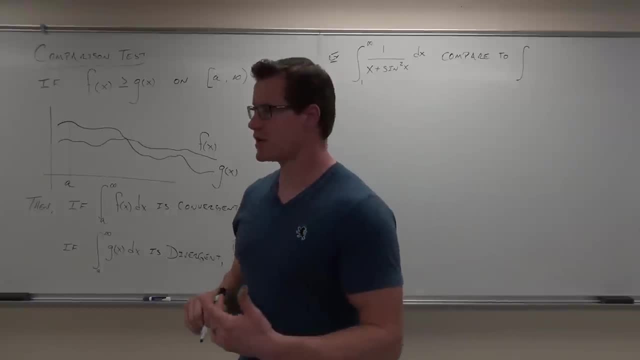 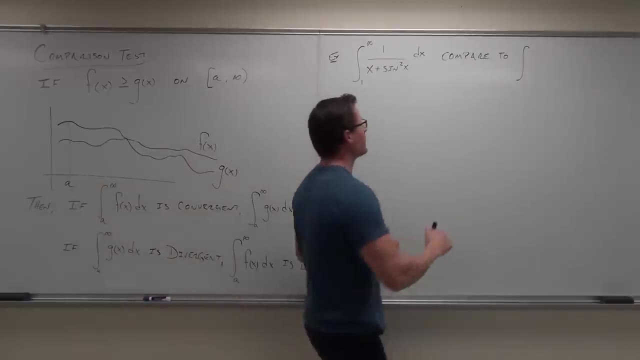 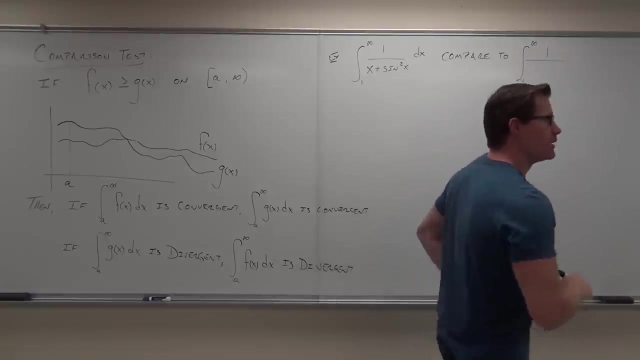 Now keep in mind that if we're going to do this, we do have to keep the bounds of integration the same from here to here, just so that we match this up. So notice that our a and our a- they match up. Perhaps we think of this. 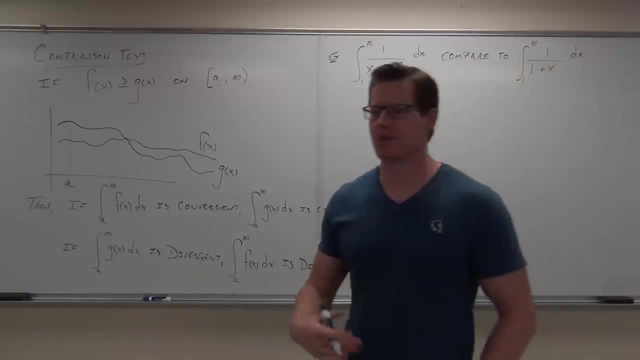 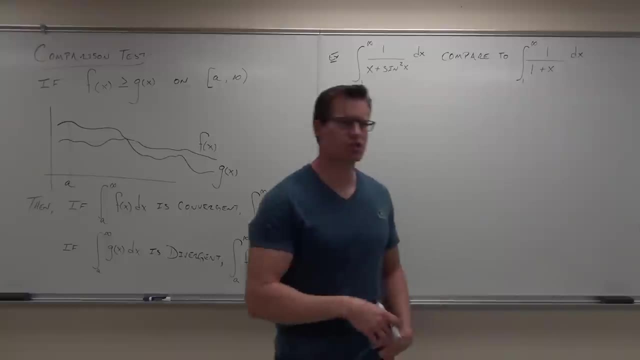 We're going to try to compare it to that. Now. here's how we're going to compare it. Now, where did I come up with that? Well, I'll show you in a second how I came up with that, But a lot of times when you're just learning this stuff, it's going to be given to you. 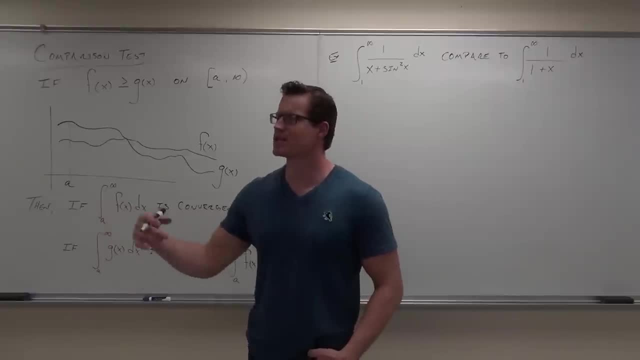 It's going to say: hey, compare this function to this one, Just to get you guys in the habit of seeing how to make that comparison. Does that make sense? So it'll typically be given to you. I would say, like on one of my tests I'd say, hey, you know what? 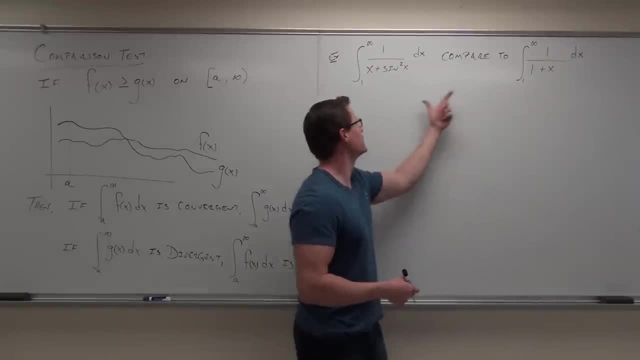 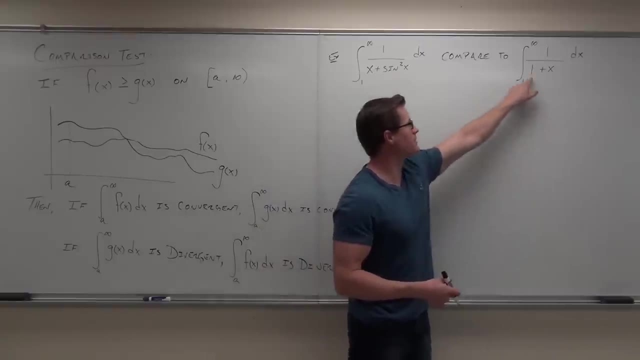 Take this thing, compare it to this. So what am I doing here? Well, I'm getting rid of at least the sine. I'm trying to limit that. Also, I'll show you why the sine gets limited to this and the x. 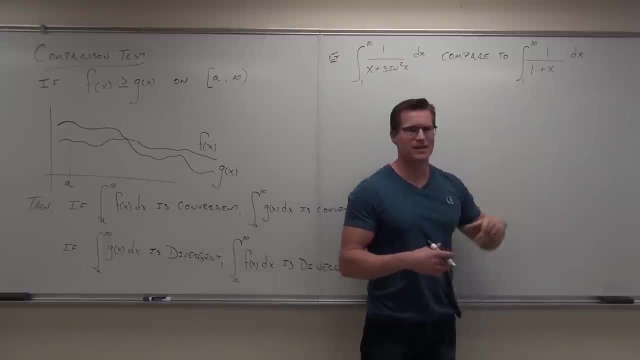 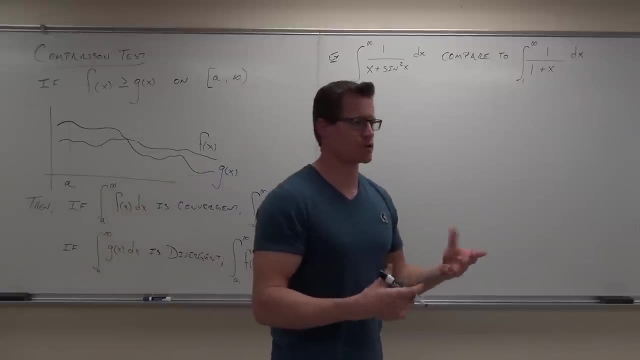 I don't have to change that. I'll show you that in just a second. OK, But the idea is, let's try to find something that is going to contain all the times it'll be bigger than this function, or all the time be smaller than this function. 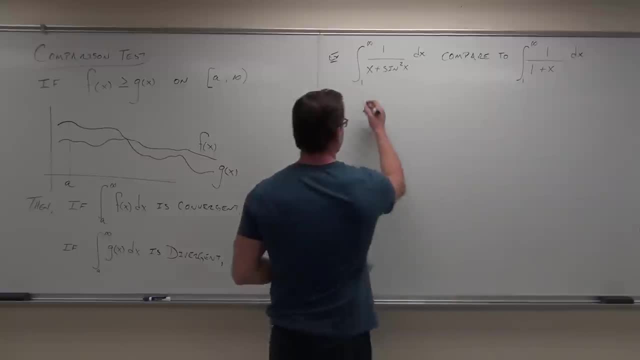 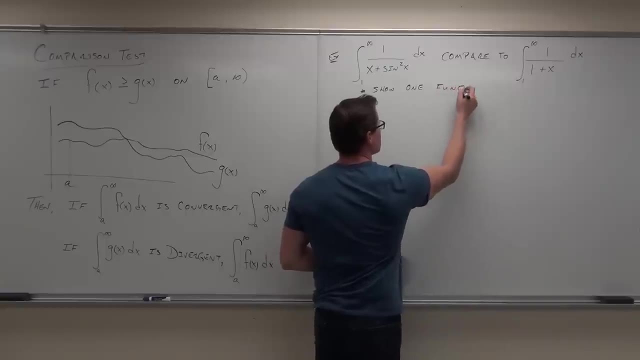 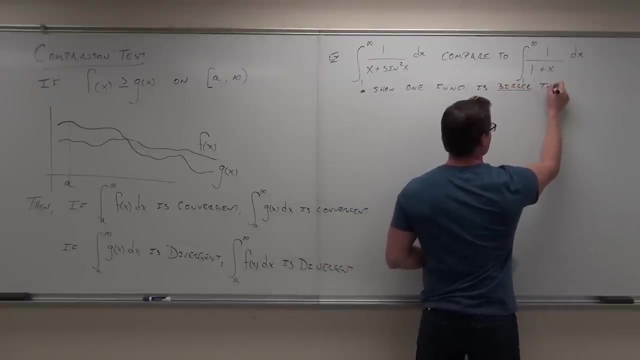 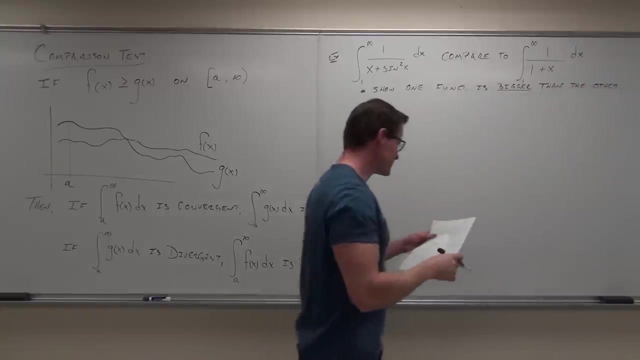 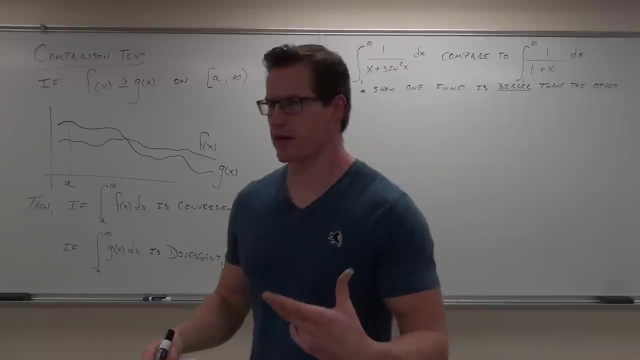 Let me show you. So the first thing we've got to do show one function is bigger than the other. We start with something very basic, just the idea of what in the world these things look like. Are you guys with me so far, on the idea at least? 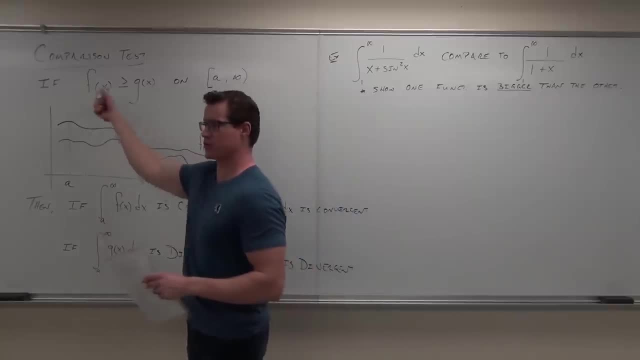 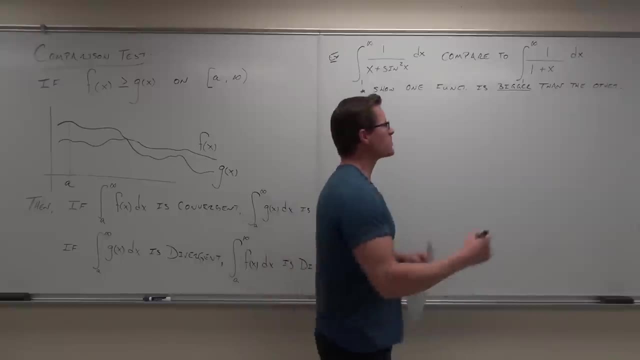 Hello, yes, no. The idea, of course, is we've got to show this first. That way we can make some determination as whether this is happening or whether this is happening. Does that make sense to you? So we start with something very basic like this: 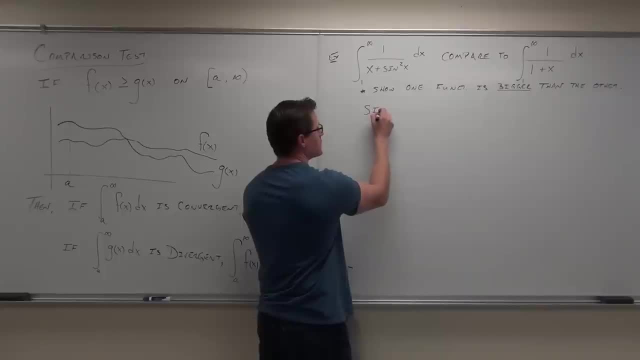 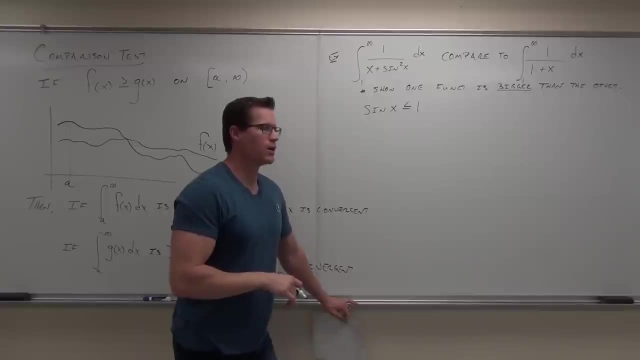 I know just from my trigonometry that sine x is always less than or equal to 1.. I know that, Don't you know that? OK, now here's what's interesting. If I square both sides of this inequality, it should not change that inequality. 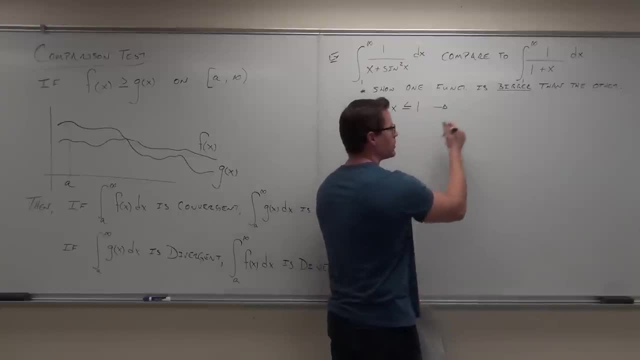 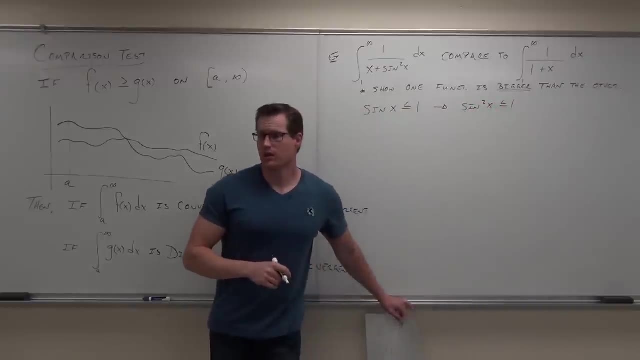 So what this implies is that if sine x is always less than or equal to 1, then sine squared x is also less than or equal to 1.. When I square a number less than 1 or equal to 1, it gives you a number less than or equal to 1.. 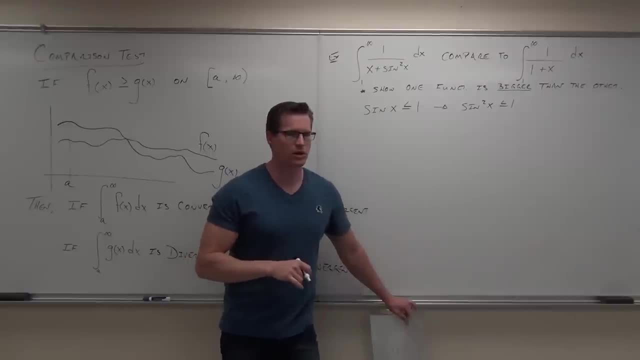 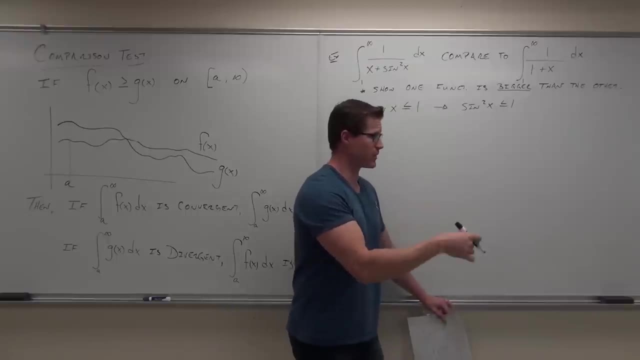 Does that make sense to you? Cool, OK, You sure you're OK with that one, right, Cool? Well, let's just do something really easy. You know we can do anything we want to, as long as we can do both sides of an equation. 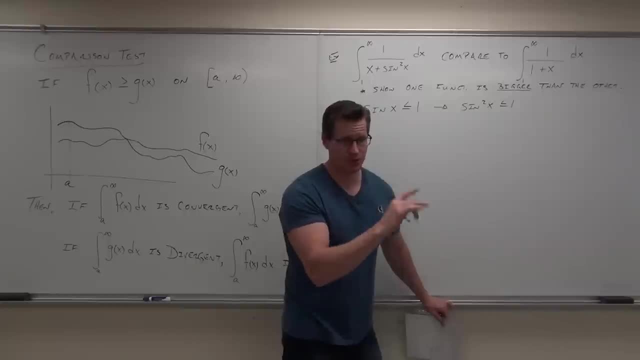 And same thing with inequalities. Unless you divide or multiply by a negative, then it flips inequality around. So what I could do basically is say, hey, if this is true, then what I can do is let's just add x to both sides. 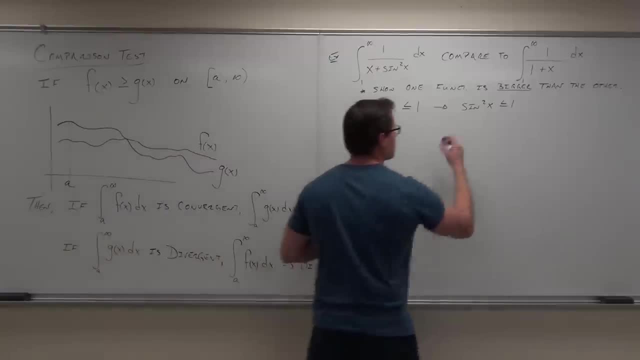 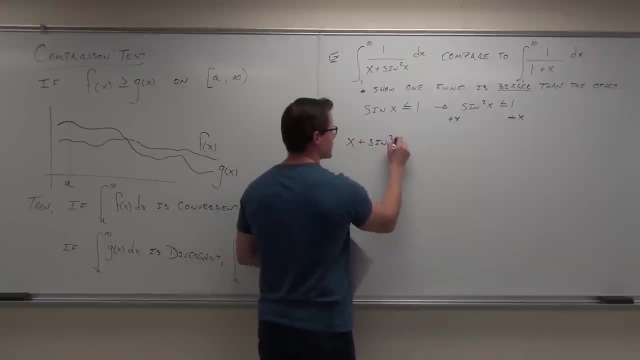 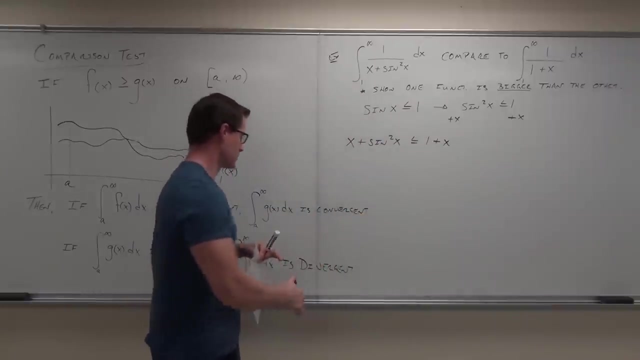 So if I add x here and I add x here, I'm going to get x plus sine. squared, x is less than or equal to 1 plus x. Put your hands, if you can follow the algebra, on that one Now. do you see the way I came up with this function now? 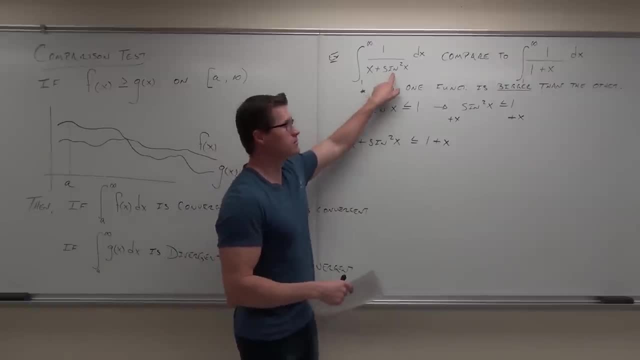 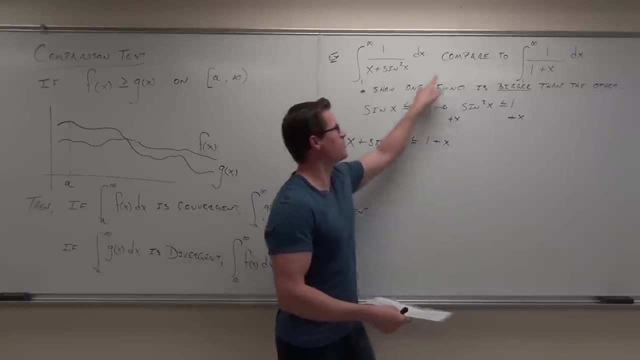 I thought about it like this: OK, you know what? Sine is always less than or equal to 1. Sine, squared is always less than or equal to 1.. So I'm trying to build something from this one. So I'm saying, hey, how can I make this function from here? 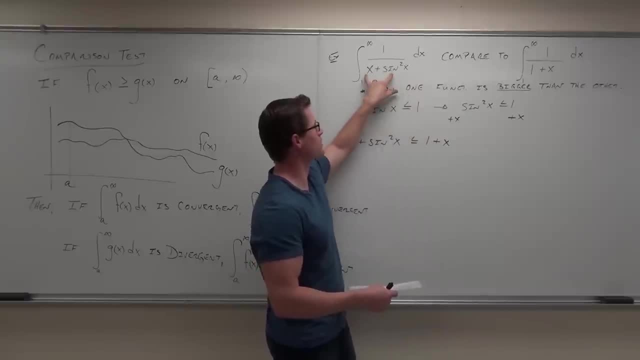 Well, hey, that's bounded by 1.. Therefore, this thing is bounded by 1 plus x. That's the idea. Now, of course, what we're going to want to do is we're going to reciprocate these two things. 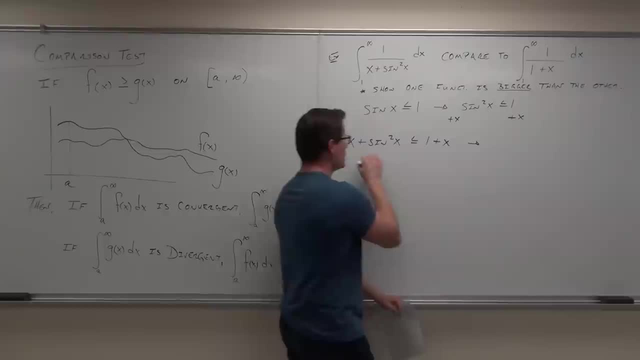 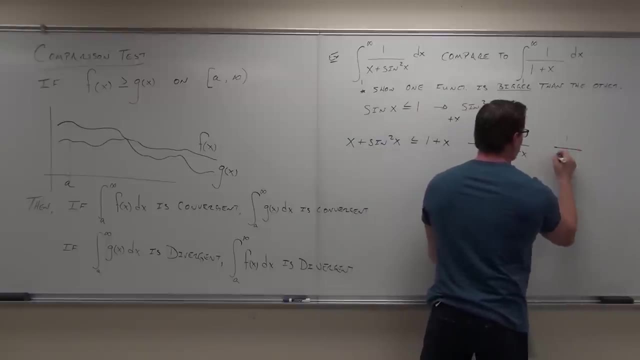 Put them over 1.. If you do, if you reciprocate your inequality, if I do 1 over x plus sine squared x and I do 1 over 1 plus x, tell me what happens to an inequality when I reciprocate both sides? 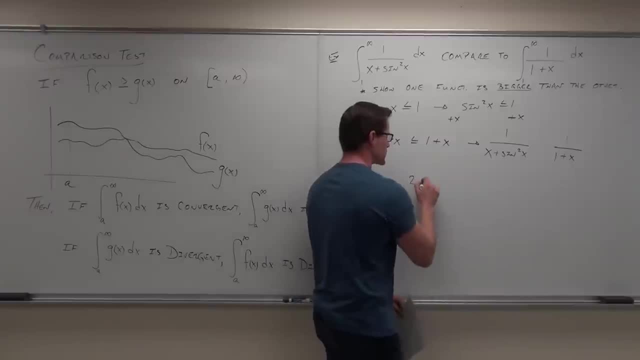 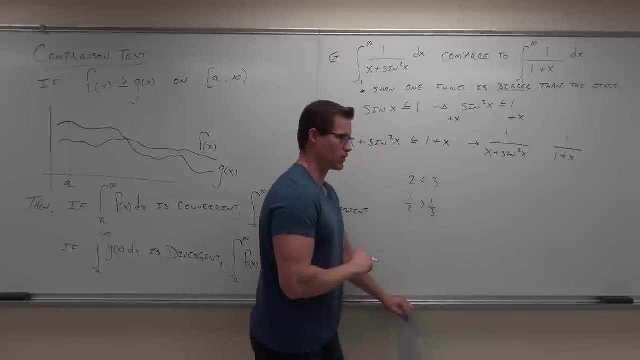 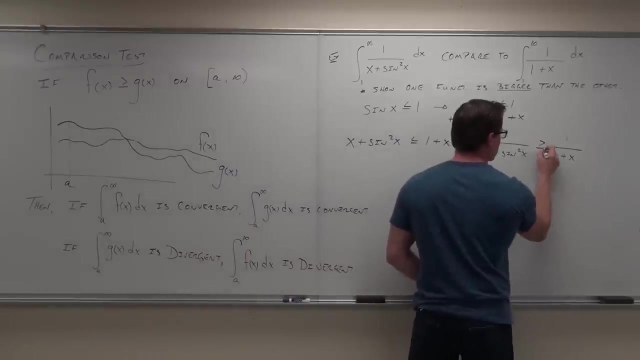 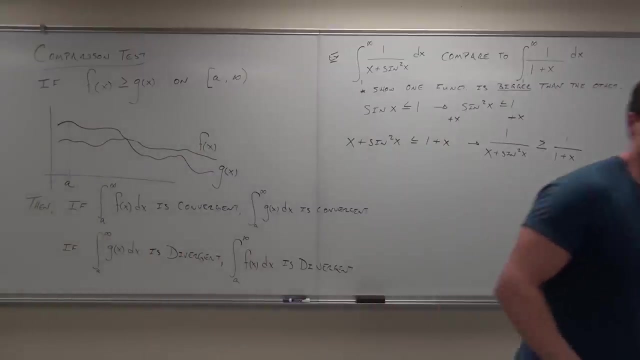 Do you know? 2 is less than 3.. If I reciprocate, 1 half is greater than 1 third. The inequality flips around. We reverse that inequality. Does that give us the relationship that we want to see? It tells us that, yeah, cool, OK, we know that something's happening here. 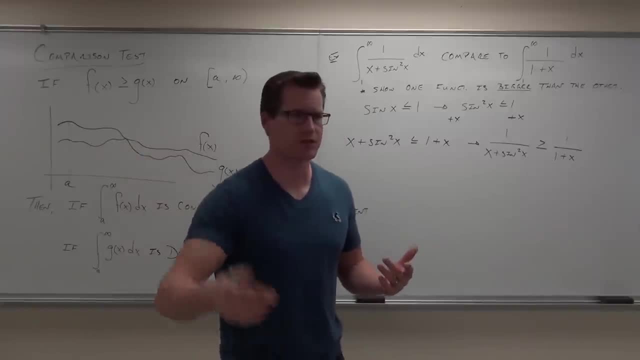 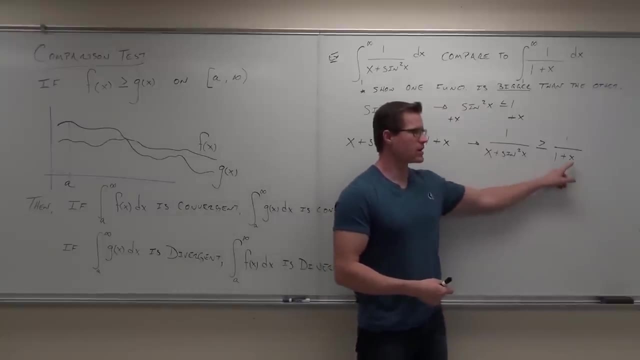 that one function is always greater than, or possibly equal to, another Show of hands should be OK with this one. That's the idea. You need it to be all the time too, So we always know that, yeah, these could be equal at some points. 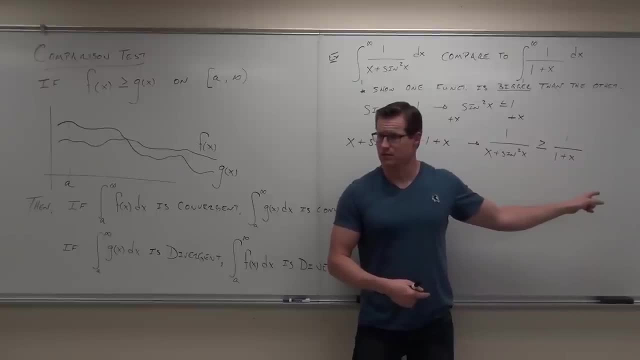 but other points. this is going to be greater than this function. Does that make sense to you? You sure? Any questions or comments? before we go any further, I need to make sure you guys get with this, OK. So the first thing we show is that I don't know right off the bat whether one's bigger or smaller. 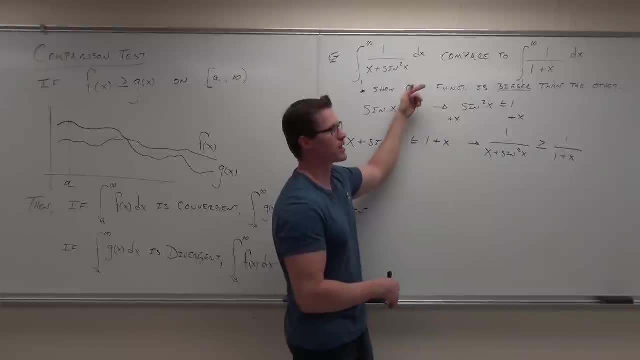 I do because I'm doing the problem. OK, but we're not going to know that right off the bat. We've got to look at it and go: OK, how am I going to get this thing from this thing? Well, figure it out. 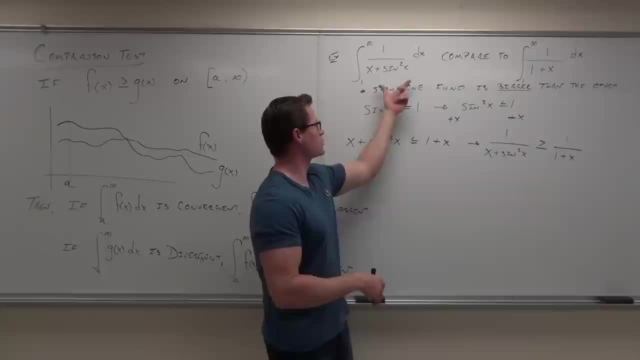 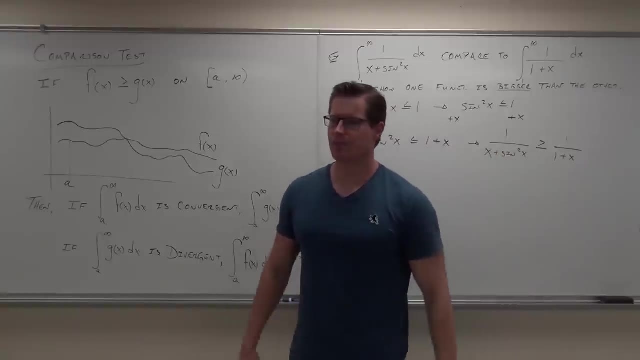 Figure out some relationship. start small, grow your function, grow it to what this side is. then compare it to what this side is. Well, this one turned out to be always bigger than that. So what are we going to try to show? 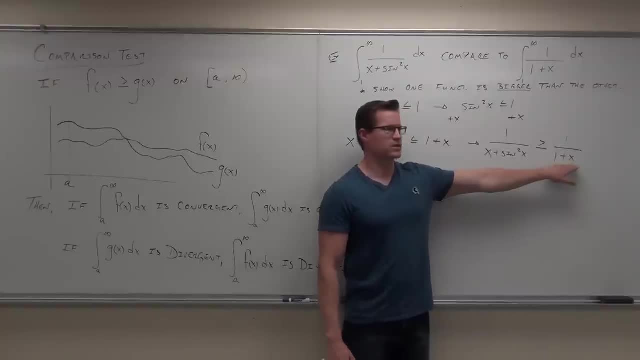 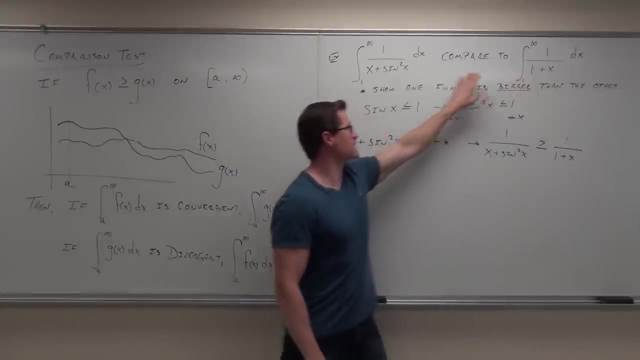 Let's think about it. If this thing- please listen carefully and think carefully on this- If this thing converges, if this, well, actually this, if this thing converges, does it tell you anything about this thing? No, If this converges, does it tell you about this? 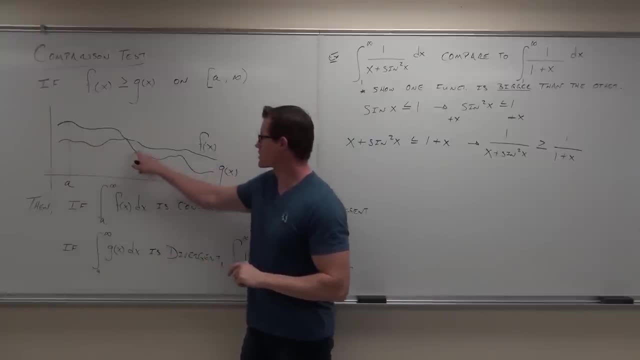 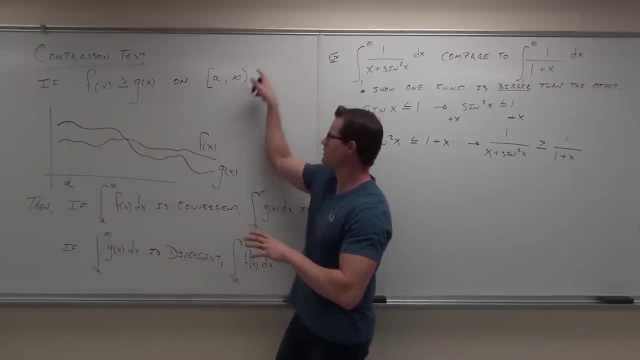 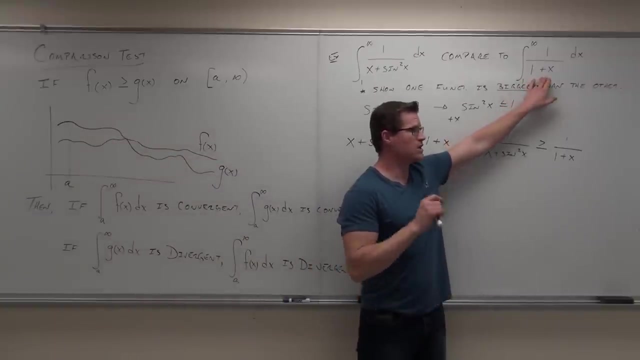 No, Here's a scenario. It says: hey, suppose that g of x converges. g of x is a small one. If this converges, could f of x diverge. Possibly, Absolutely, You don't know. So if this small function converges, we've said nothing about the big function. 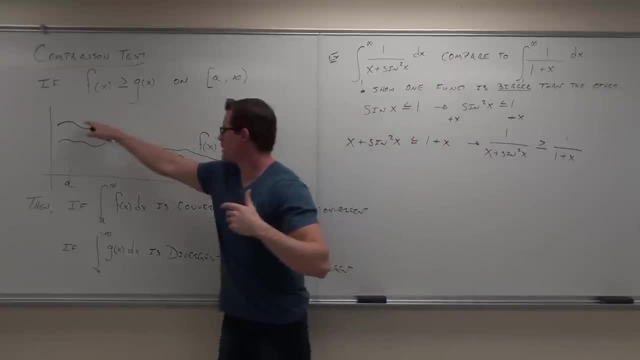 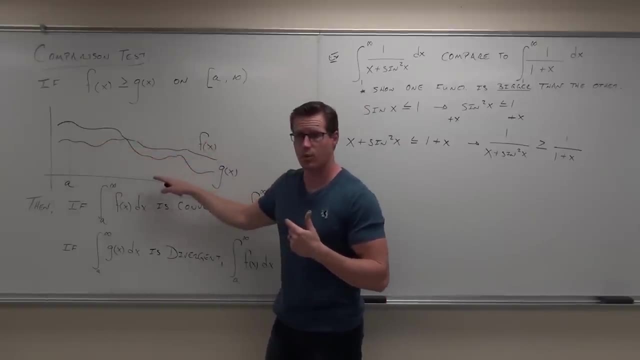 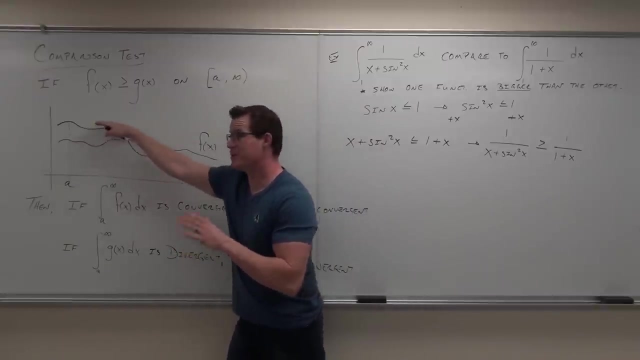 Does that make sense? Contrapositively, If the large function diverges, does it tell you anything about the small function? No, No, it doesn't. This could easily diverge and the small function could converge. What happens is, if the big function converges, the small one has to. 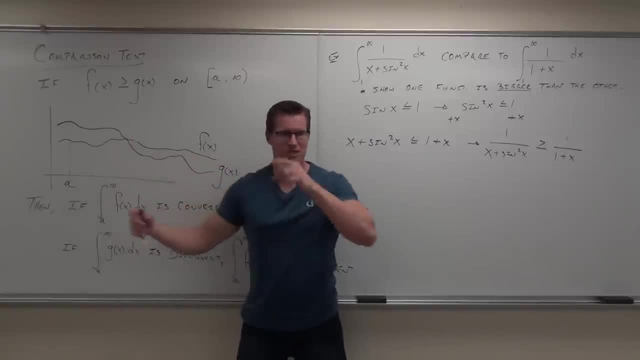 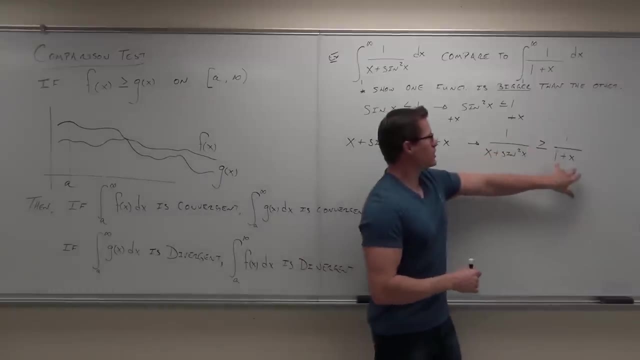 If the small function diverges, the big one has to Maybe watch that about 14 times so it actually sinks in there. okay, Because that has to happen. So in our case, if this one converges, nothing, Nothing Got it. 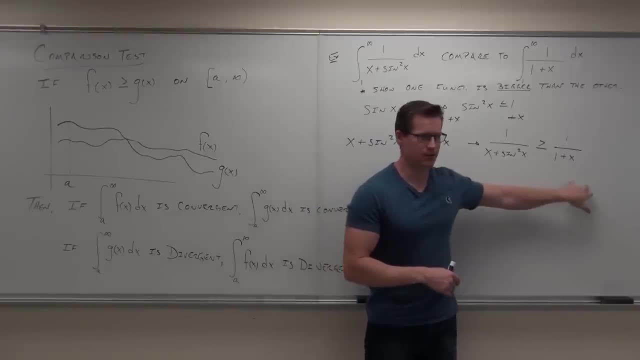 If this one diverged, nothing. Now, of course, we can't do this integral, So we're going to do this one and then make the comparison If this one diverges. now think of here: If this diverges, what does it tell you about this one? 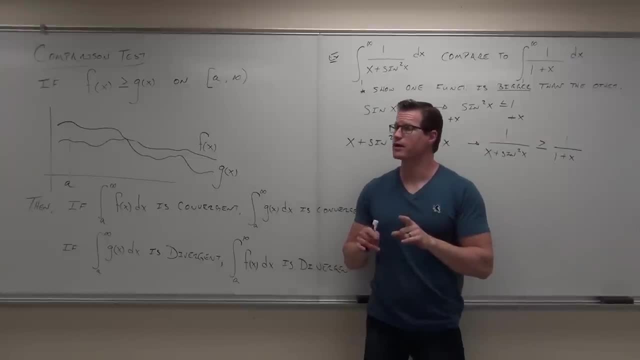 It diverges. That's where we can make the jump. So we can only show one thing here, if at all: If this converges, it's smaller than this one. It doesn't say anything. It says, yeah, your small function converges. 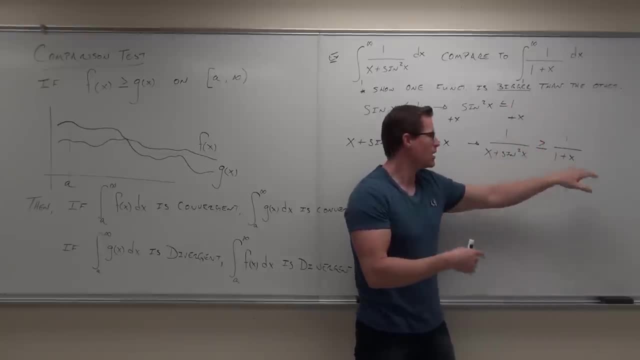 The bigger one is obviously bigger than that. I don't know where the convergent diverges, But if this diverges, if the small one diverges, the big one also has to. Does that make sense? at least a little bit? 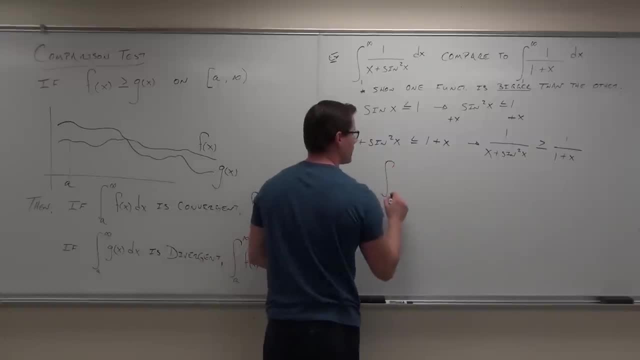 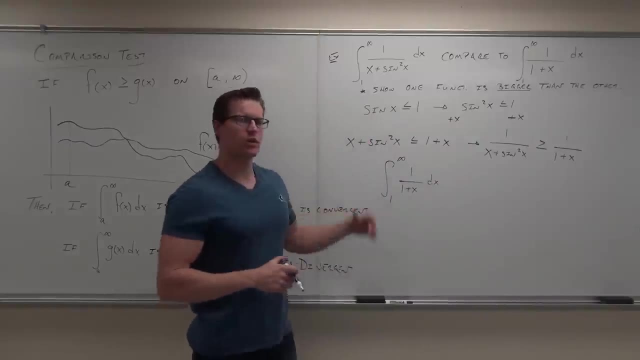 Okay, so let's go ahead. let's see if we can do this integral From 1 to infinity of 1 over 1 plus x dx. Now that's something we know how to do. What would I do? first, You've got to change your limit. 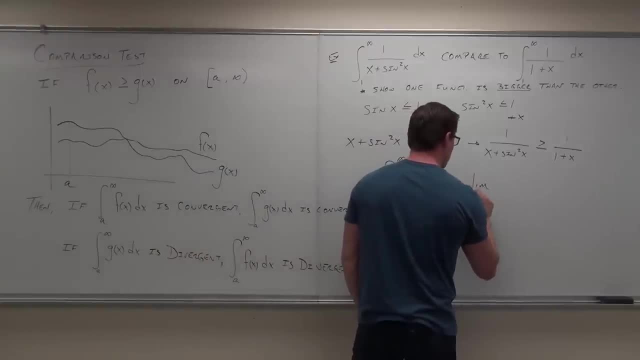 Yes, I would say this is an infinite interval. As b approaches infinity, I can change it to 1 to b, 1 over 1 plus x dx. Yeah, you can do u sub. We're going to keep this pretty simple because we're past all this stuff. 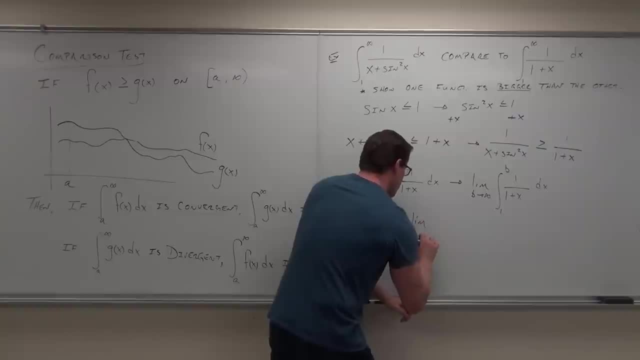 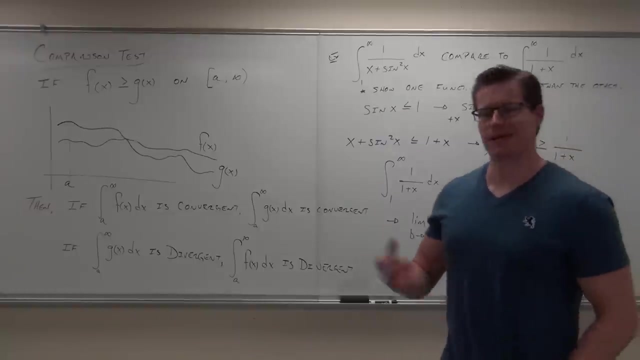 What this changes to is a limit, as b approaches infinity, of ln absolute value. 1 plus x From 1 to b. Yeah, of course you can do a u sub on that one. You just say u equals 1 plus x. It would be 1 over u absolute value of u. plug in the 1 plus x before we start evaluation. 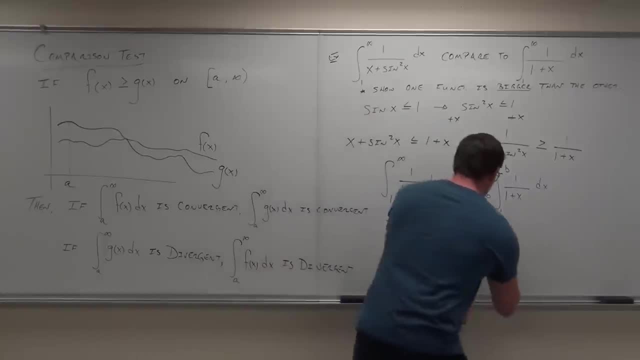 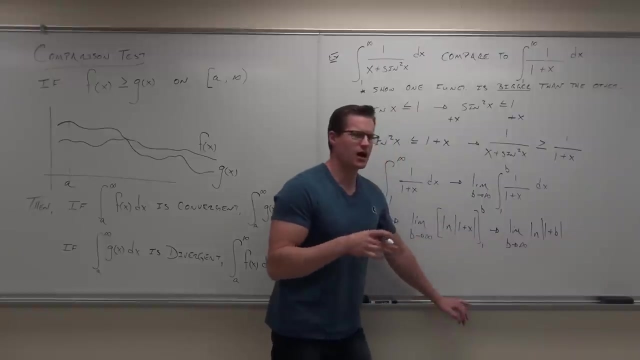 Should we be okay with that one. Let's evaluate. So this would be limit as b approaches infinity ln absolute value. 1 plus b Absolute value here really is not that relevant. Can you explain to me why the absolute value here is not relevant for us? 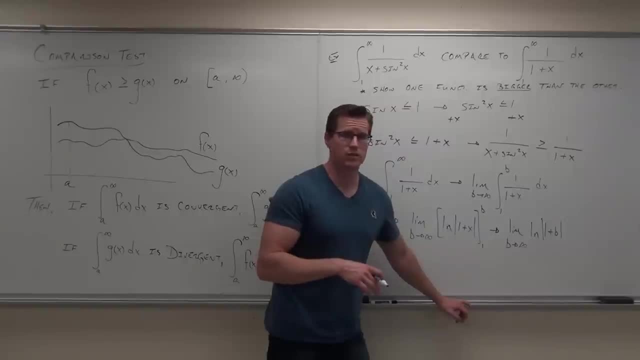 Never be negative. Say what now? It won't be negative, Never. Our interval is 1 to infinity. We can't get a negative if we're adding 1 plus a number, that's positive, okay. So really here kind of irrelevant. 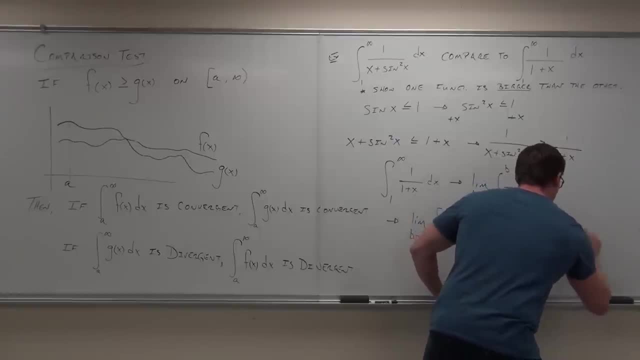 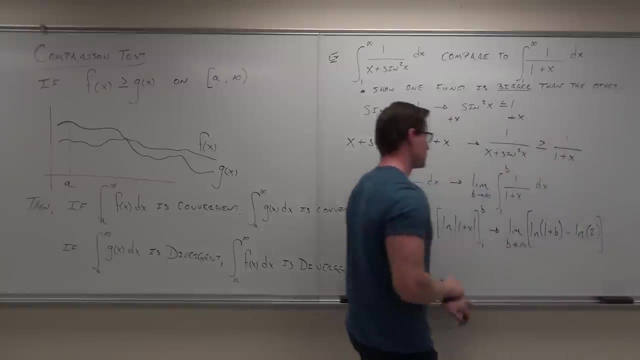 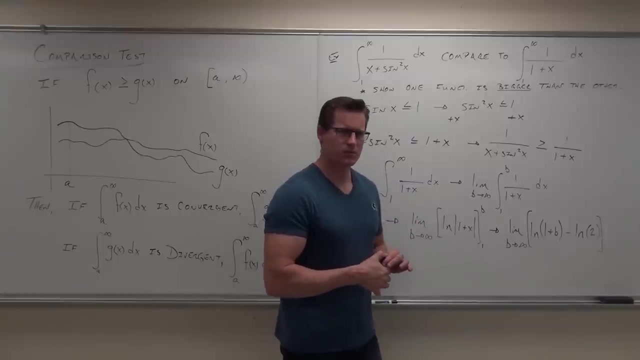 It doesn't really matter. Minus ln 2. Quick head nod if you're okay with where those numbers are coming from. Just some evaluation. Now let's think about it. Where's b going? Infinity- Okay. What's infinity plus 1?? 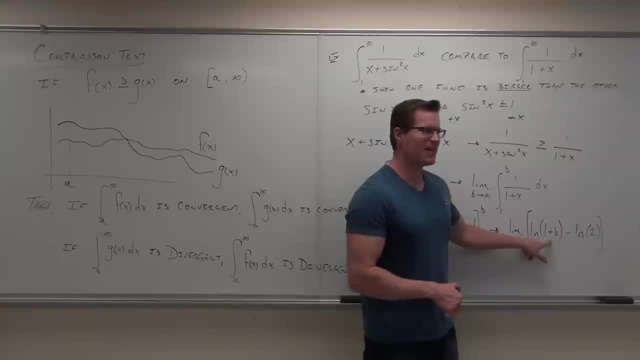 So when you're a little kid, I hate you to infinity. I hate you to infinity plus 1.. It's still infinity, stupid kids, Anyway. so infinity plus 1 is still infinity. What's ln of infinity? I always argue with you. 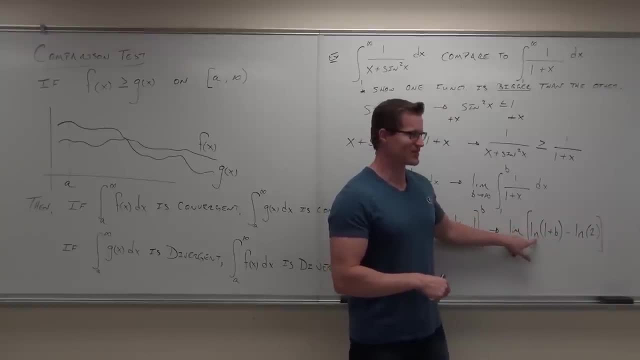 I'm stupid, I really don't. I ignore the little kids, just like they shouldn't be ignored. That was a joke, by the way. Totally love kids, Anyway. Infinity- That's right Back to math. ln of infinity is: 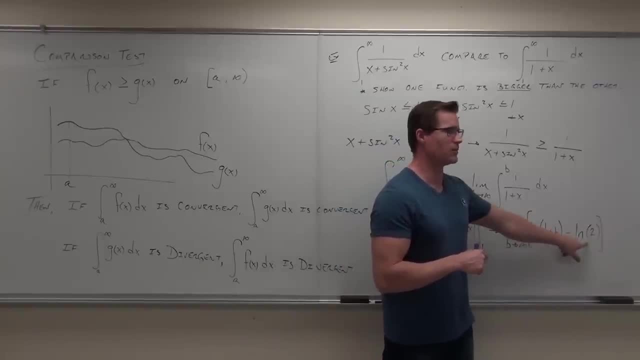 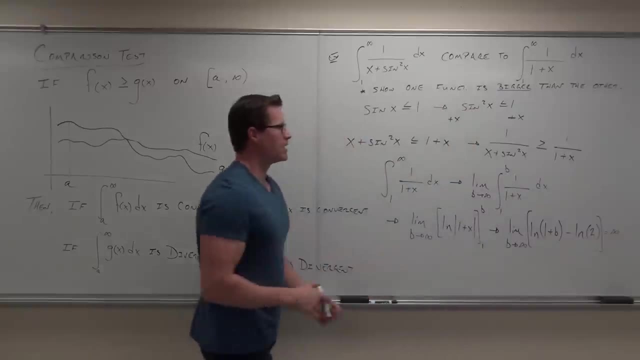 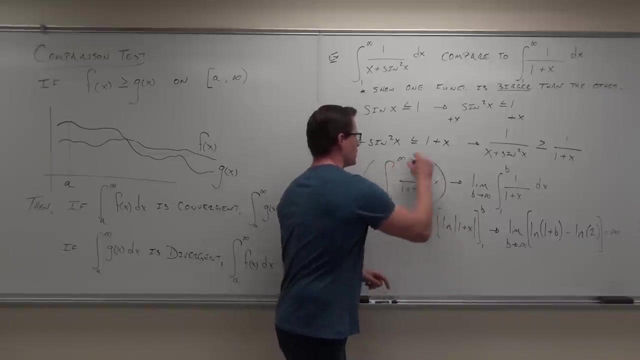 Infinity, So this goes to infinity. What's infinity minus something really small? Infinity? So this whole limit goes to Divergent. So you tell me something. Tell me something Now that we've done this integral: is this integral convergent or divergent? 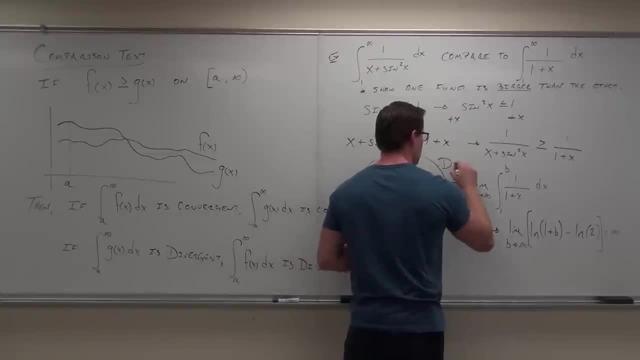 Divergent. Now we think back to why we did this whole thing right here. If this function is always bigger than this function- I'm going to go through this one more time- If this had been convergent? Not convergent, just not convergent. 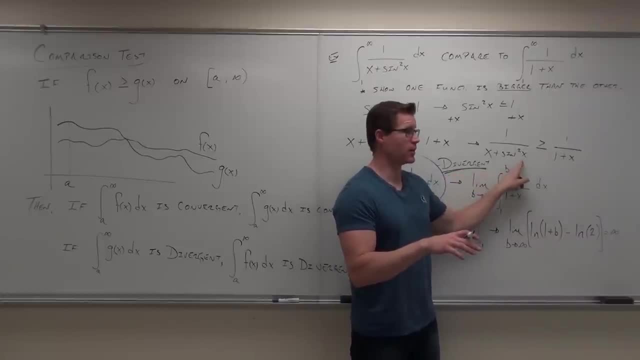 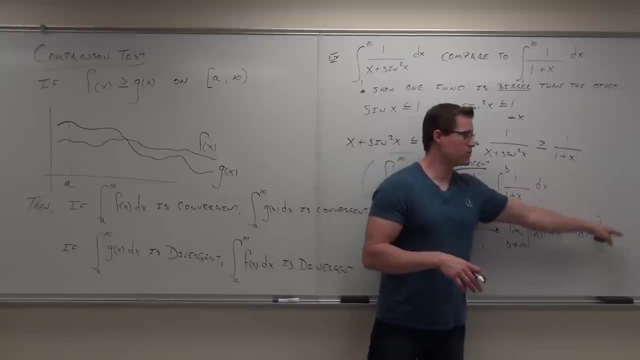 But if it had been convergent, it doesn't say a thing about that, Don't know. Inconclusive, But if this is divergent, This says that this area goes to infinity, or we can't find it, or something like that. 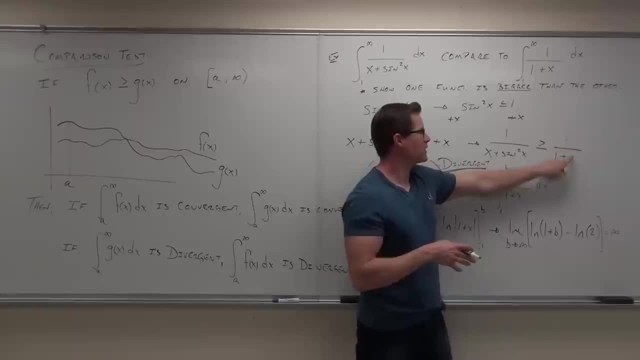 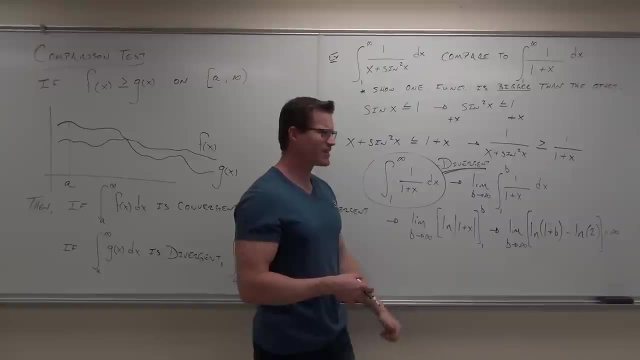 This area is infinity Area of this. What say about that one? It has to be So. should we even bother doing this integral? No, Heck, no, I know that if I did it, If I was able to somehow magically do this right now, 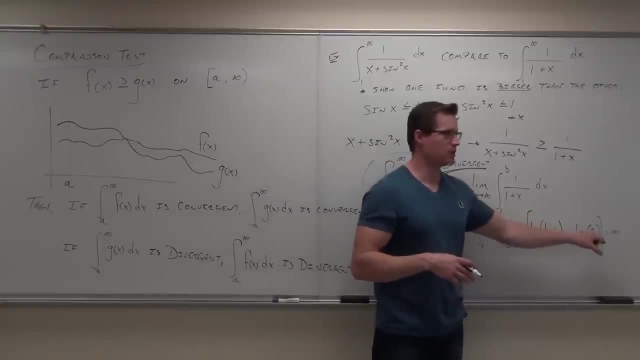 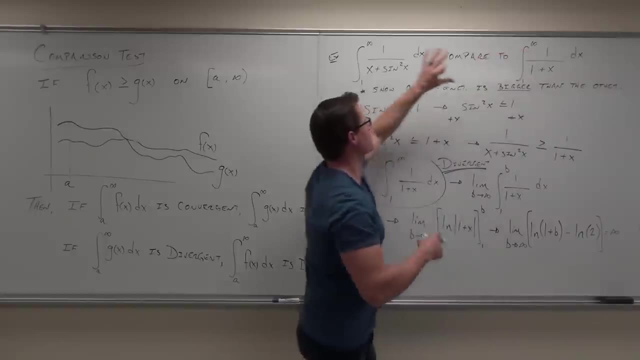 Our limit would also go to infinity, Since this function is always bigger than this function. The area under this curve is always bigger than the area under that curve. So if this is divergent, this also has to be divergent, So that's infinity plus bigger.